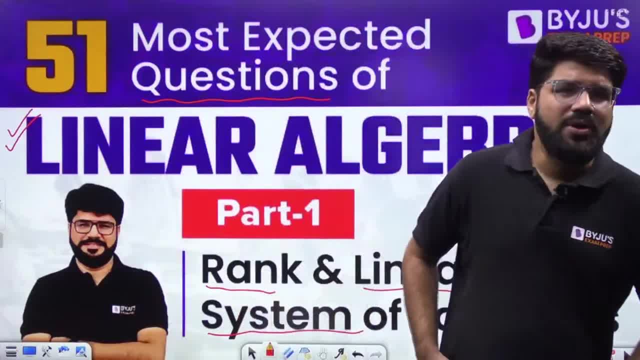 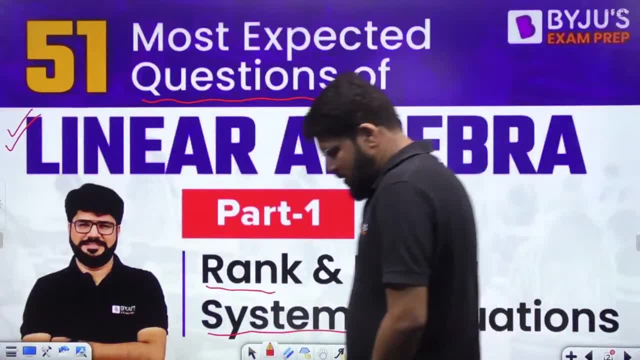 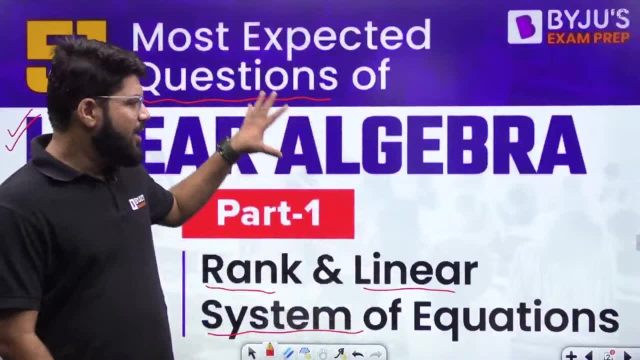 you know, we have rescheduled to 11: 30. yesterday i informed you about 11 am but it has started 11: 30 due to- again, i repeat, due to power issues. right, but yeah, whether it starts at 11, 11, 30 doesn't matter. do we have the same energy? and, of course, we are going to content. we are going to 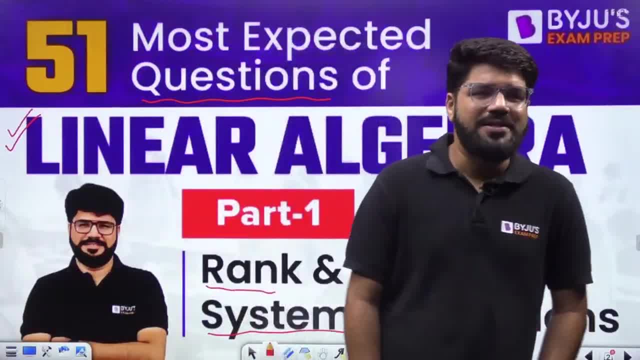 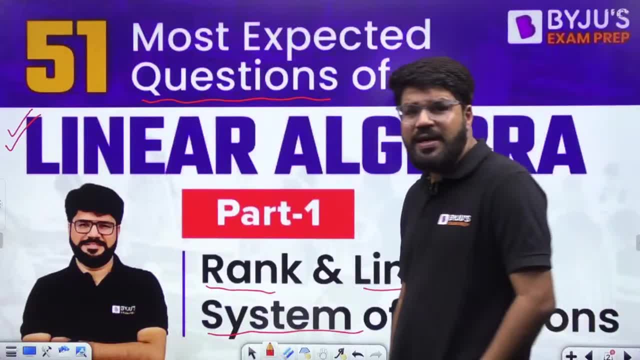 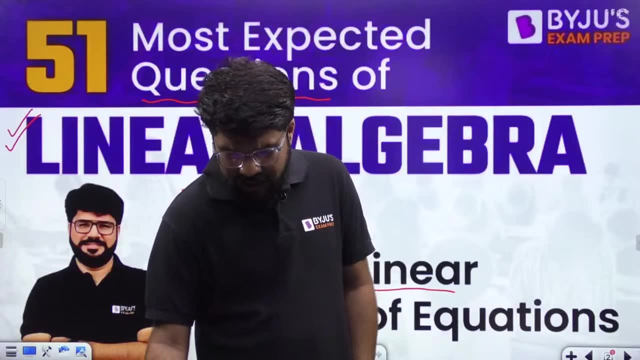 cover the similar content and, as i planned for 11 am also, there is no difference in the content. good morning, akbar sagnika satish. very, very good morning. let everybody join quickly, right? so, since the session was rescheduled, everybody quickly update your friends. okay to join using the new link. this is a new link. 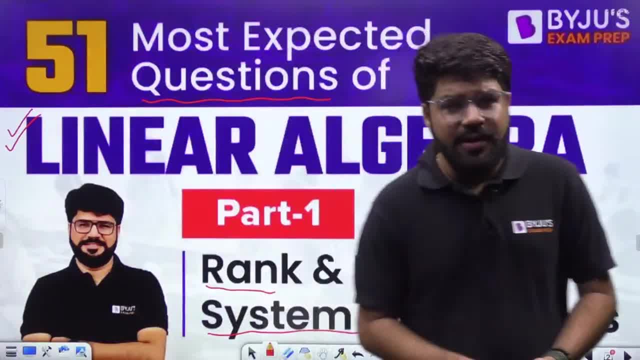 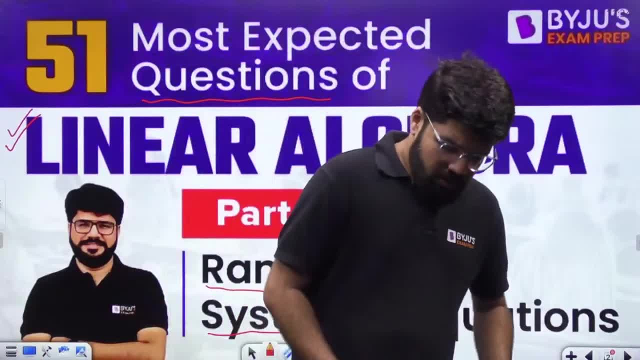 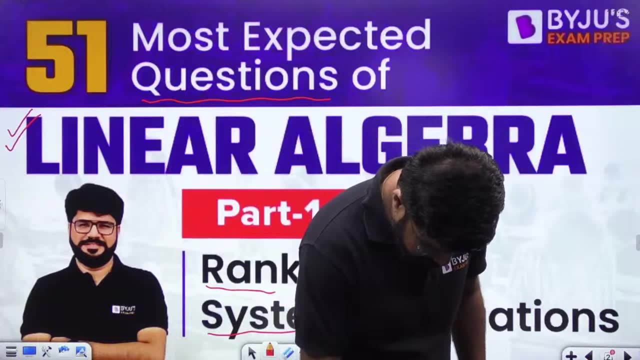 created to share this link upon everybody, because this is the newly created link. everybody share the link of this particular session to all your friends. good morning, shiva. okay, so that all others who were in plan to join they could join, also join this session. just a second. 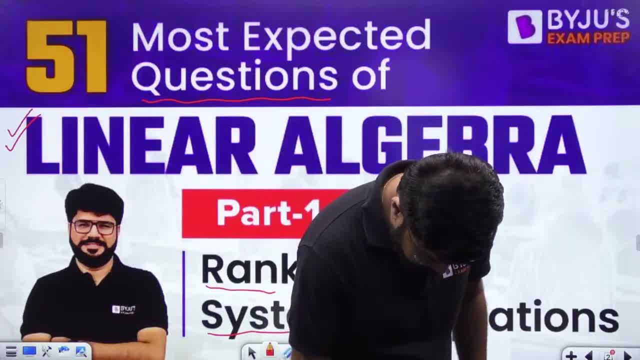 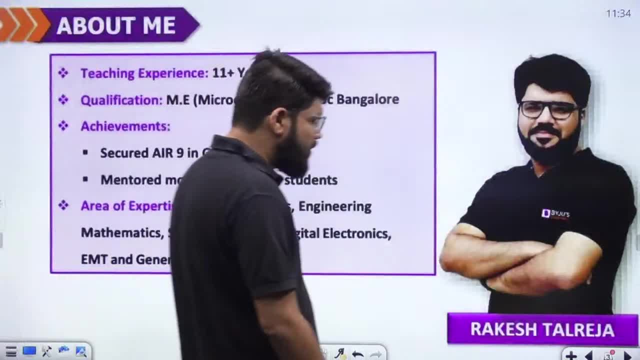 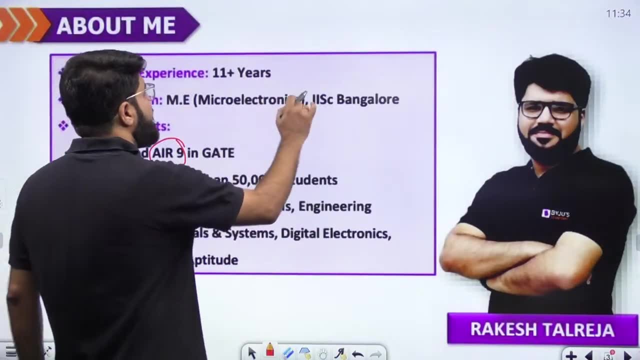 okay, chalo, cool, let's get moving ahead. then let's get started, okay, guys. so this is a brief intro in case somebody new to my session. this is your mentor and educator, rakesh, and i have secured all india rank ninth in the gate examination, completed my master's from indian institute of 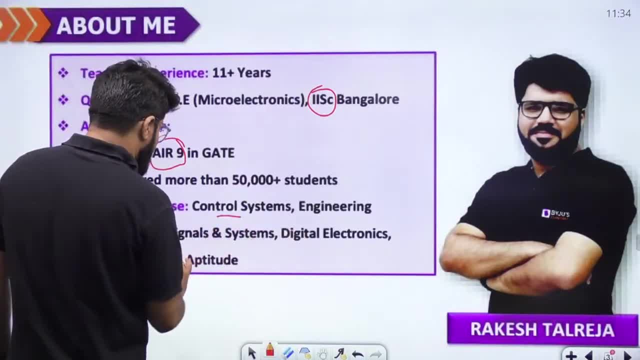 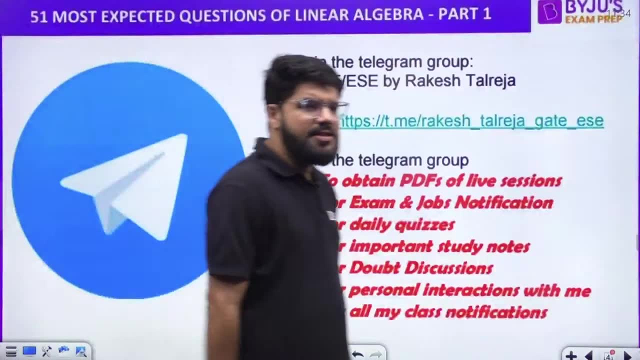 science, bangalore, and these are my major area of expertise. right in the technical, i deal with control signals, digital and emt, and the general ideal with the maths and aptitude, and this is the engineering math session. right, this is the engineering math session. you can also connect. 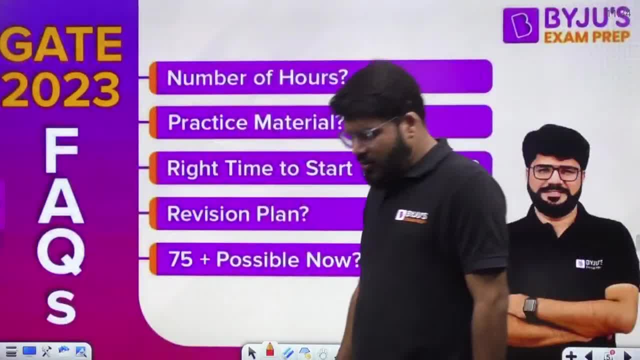 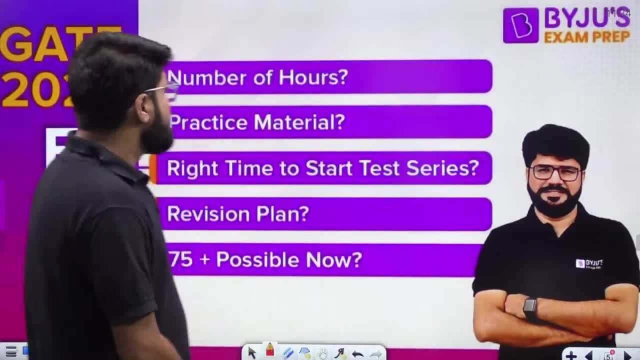 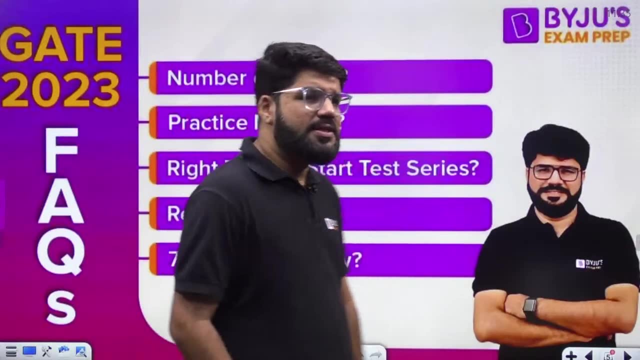 me through the telegram. i'll share you directly the link of the telegram. okay, i'll directly share the link of the telegram. very, very good morning, trb akshata. okay. so, guys, one more session for you i'm bringing, and i just want to give you a small update about that particular session, and that is: 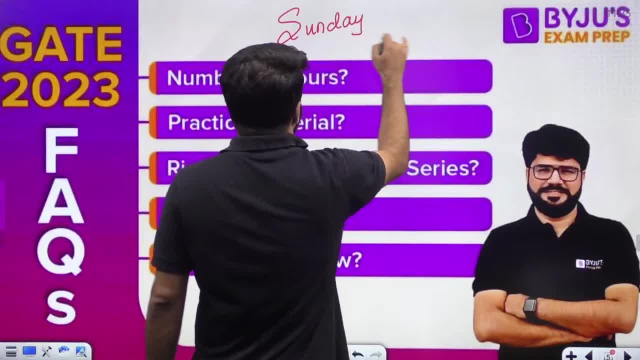 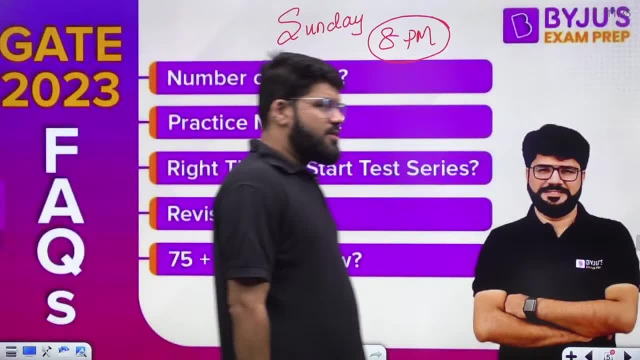 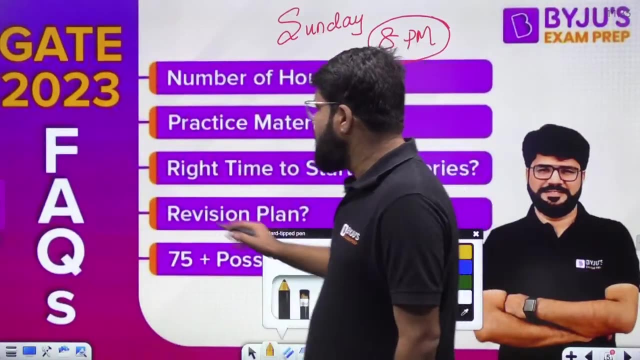 coming on this sunday night, 8 pm. this sunday night at 8 pm. last three months, three and a half months are left for the gate examination. clear any of your queries, if you have, and what are the, you know, main queries that are students, that the students will have at the last moment. what are the frequently asked questions by 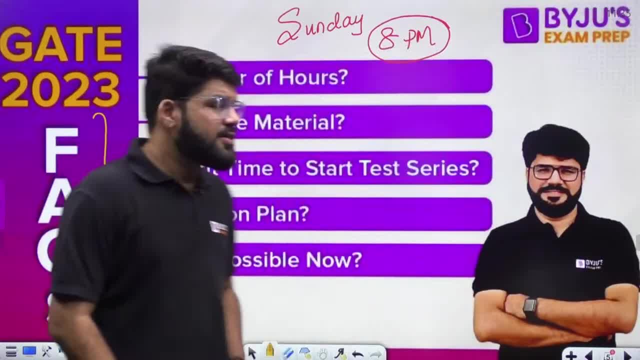 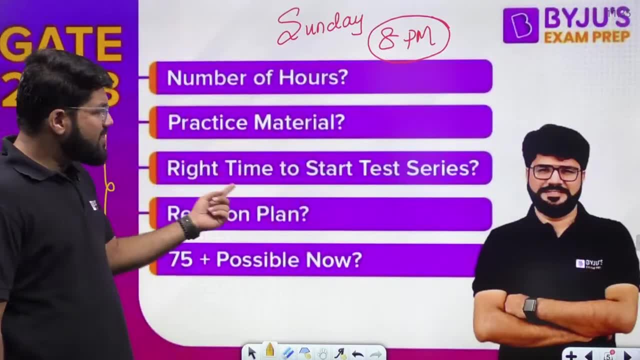 the students. i'm going to come and answer for all of you. that is now, in the remaining time. what should be the number of hours from where you should practice intensively? now, right? what is the time to start test city, especially the mock test? what is your revision plan? what is your? 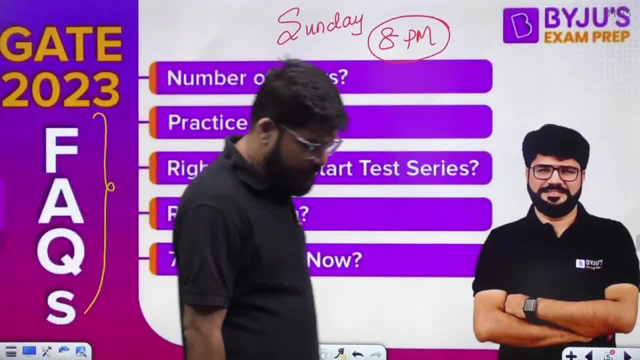 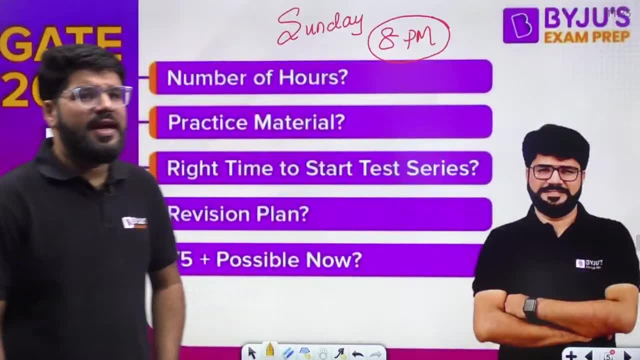 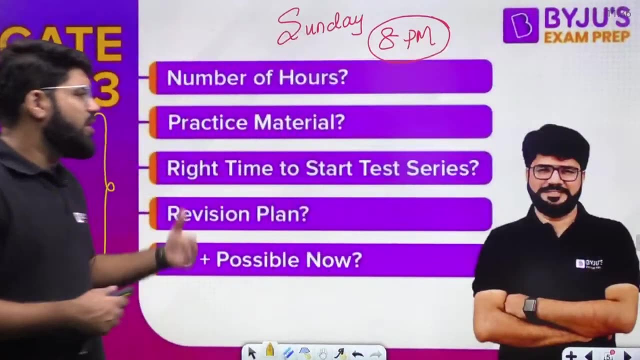 revision plan and is 75 plus possible now. is 75 plus possible now, okay, we are going to come live tomorrow, sunday, at 8 pm with this session. it's going to be a small session to give you a general idea, to give you a general idea about the last three, three and a half months left for the gate. 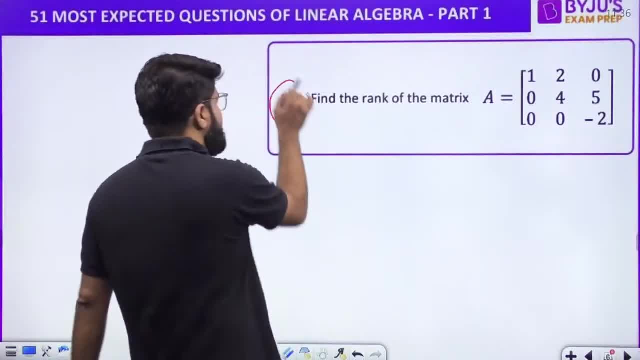 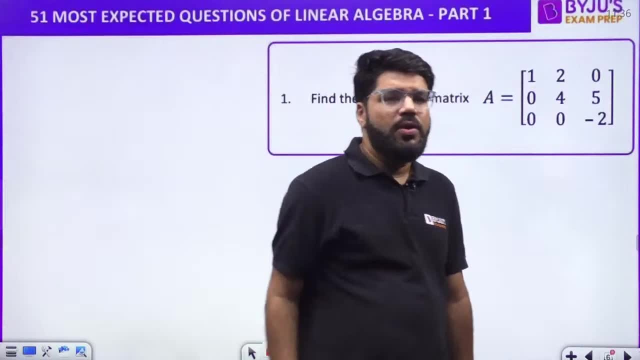 examination. and guys, this is the question number one. we will keep maintaining the sequence as well, so that you will know by tomorrow. tomorrow also you have the class at 11 am for the linear algebra, part number two, and you should know that we are going to cover all 51, as i promised. 51 means 51 questions. 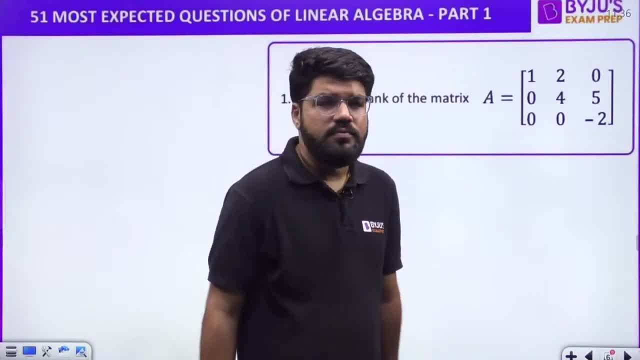 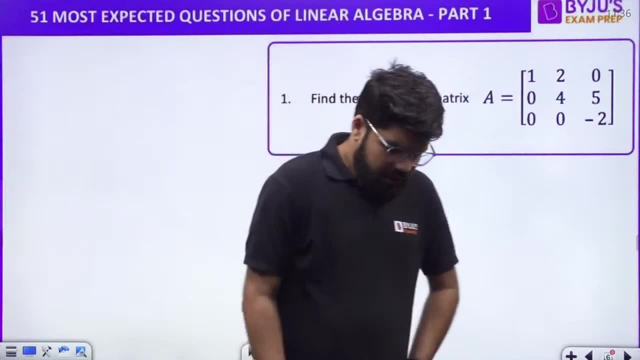 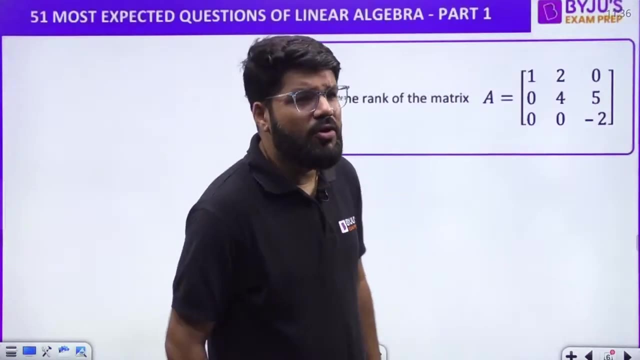 we are going to cover, isn't it guys? chalo, good morning, good morning. all keep joining and guys come on all right. first question: answer this, and do not forget to like the session. i see very less number of likes right now. maybe the session was newly created. do not forget to like the session. 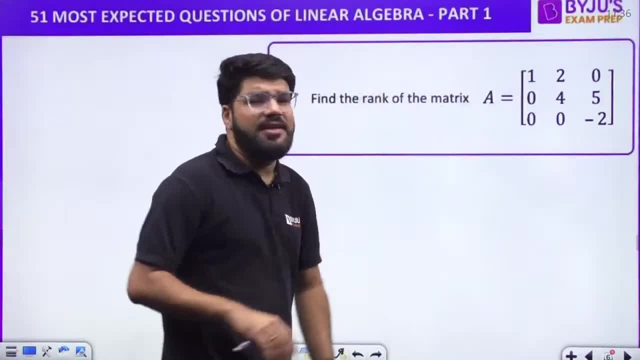 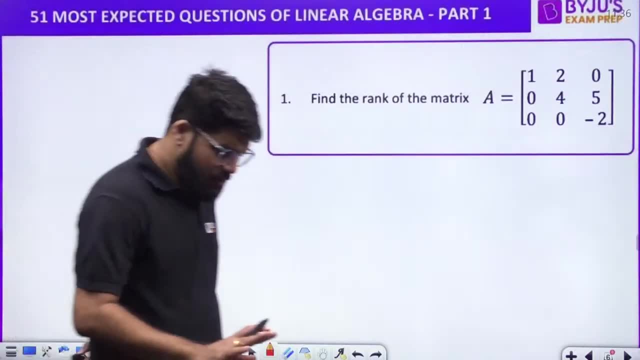 start with a positive motivation. start with a positive motivation. start with a positive motivation. everybody, show your love, show your response and like and answer the question: what is the rank of the following matrix? what should be the rank of the following matrix now? now we will start with all possible cases and i'll 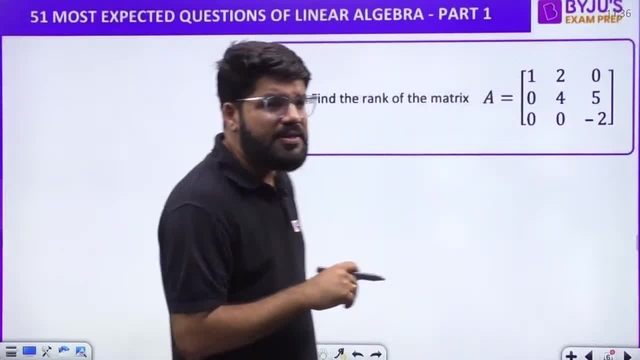 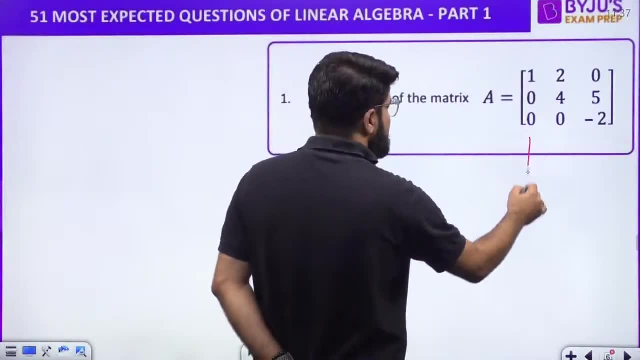 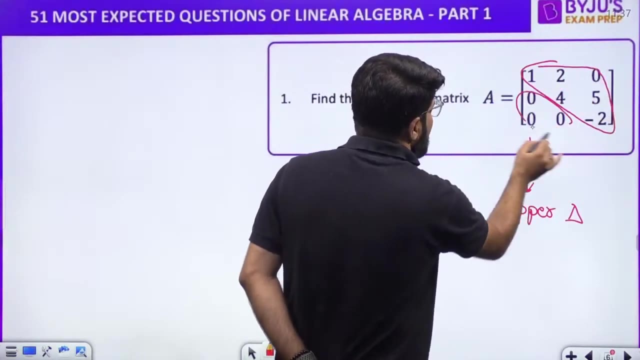 tell you the echelon method, determinant method, shortcut method, all possible methods. i am going to tell you, uh, if you have a look into this matrix, what is this type of matrix? what is this type of matrix? it is clearly upper triangular, isn't it? the elements below the diagonal are 0. Hence it is a upper triangular matrix. Now, what is the? 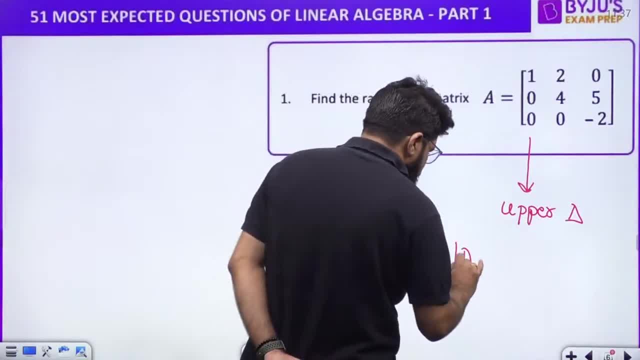 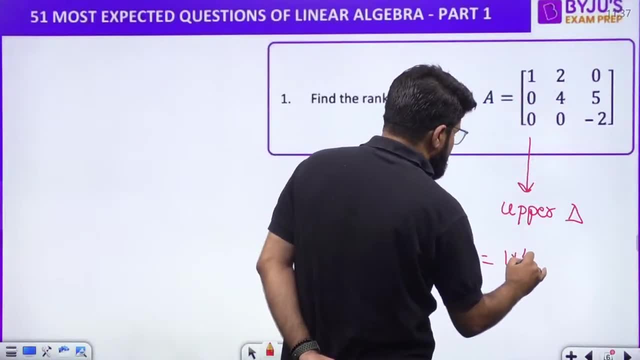 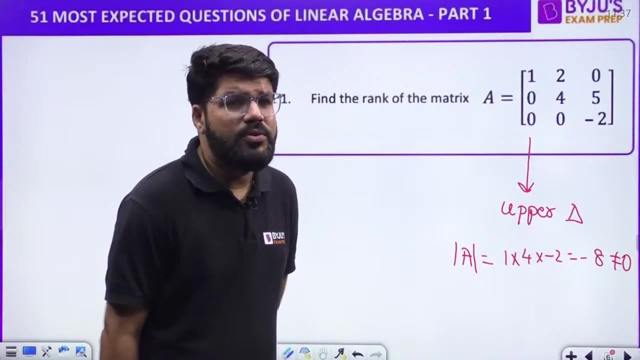 determinant of upper triangular matrix. What is the determinant of any triangular matrix? It is the product of product of diagonal number. So that is 1 cross 4 cross minus 2, which is minus 8, eventually not equal to 0.. So what is the determinant of this matrix? It is not equal to 0. 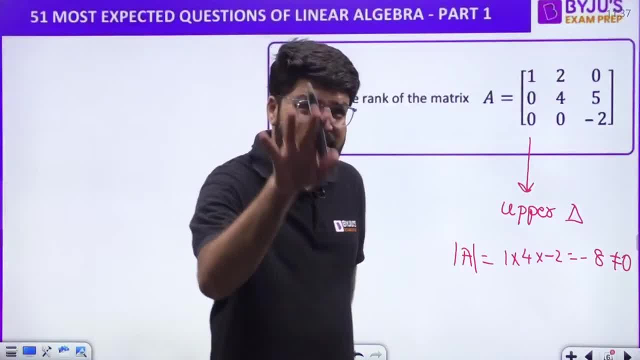 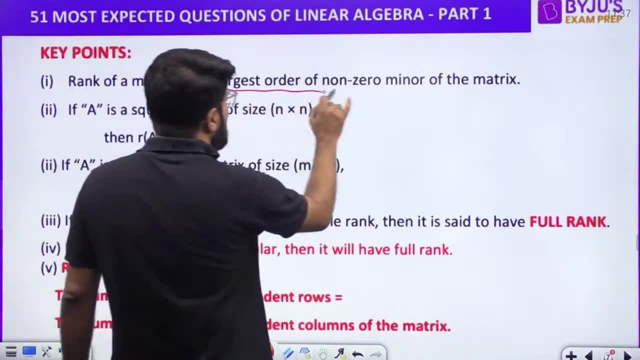 Now one of the way of understanding rank. I will tell you several points about rank. We will discuss several things about the rank, But first thing you can notice, rank is the largest order of non-zero minor of the matrix. It is the largest order of non-zero minor of the matrix. So this is 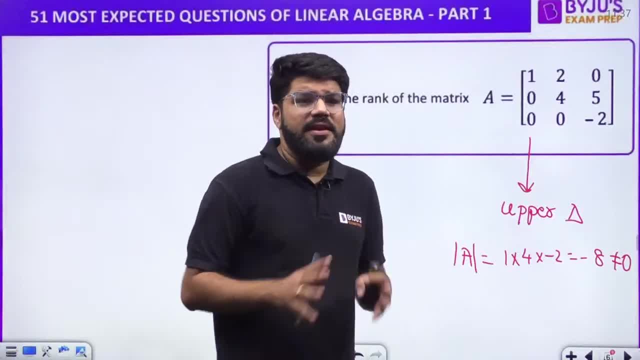 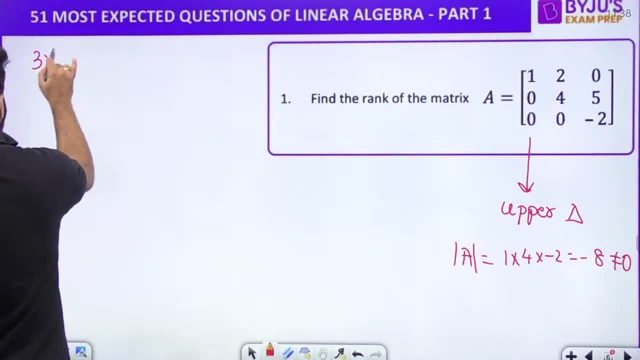 a 3 cross 3 matrix. This is a 3 cross 3 matrix and how many minors you can make. Number 1 minor you can make is a 3 cross 3 minor itself. So if I want to talk about, let us understand in the 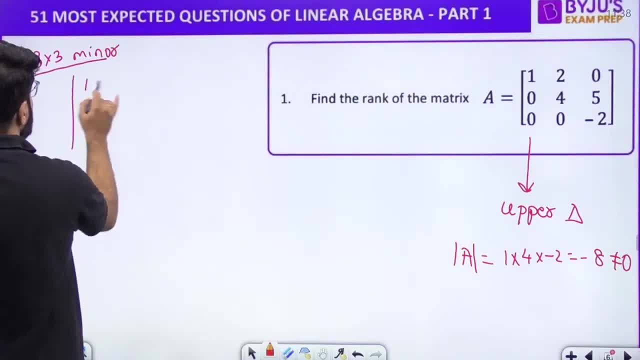 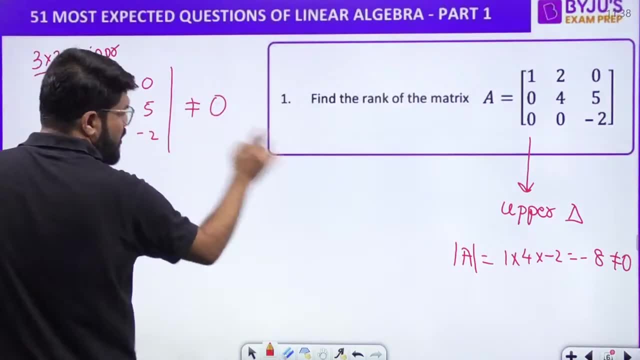 first question: If I want to talk about a 3 cross, 3 minor, so that is itself the matrix determinant. Let me call it, Let me copy the numbers. And this itself is not equal to 0, as we have noticed, And that is why. 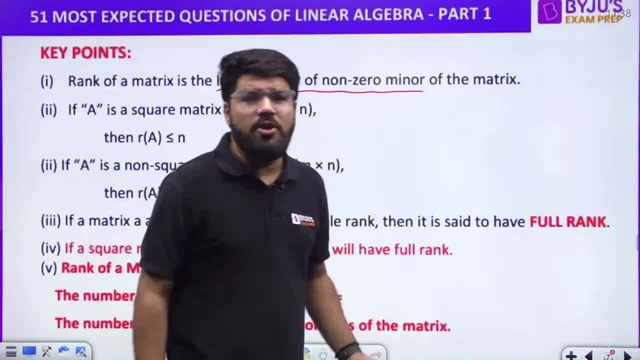 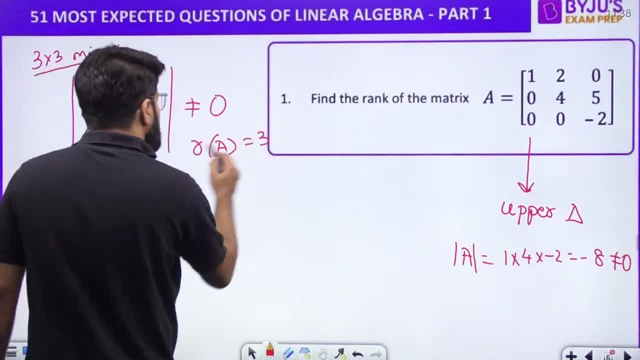 the rank of the matrix, which is the largest order of non-zero minor. So I have a 3 cross 3 minor. I have a 3 cross 3 minor, which is non-zero. So rank has to be 3.. Rank has to be 3.. Suppose if 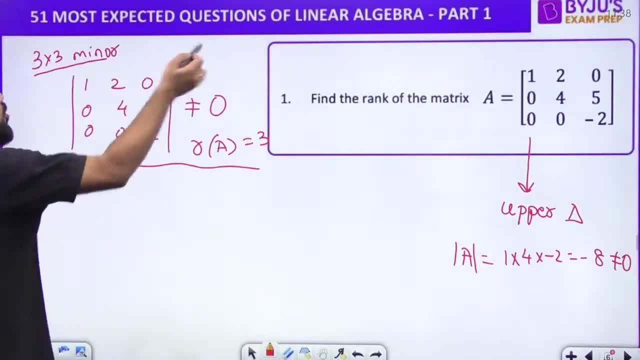 this was 0.. Suppose if this was 0.. Suppose, Imagine if this was 0.. This is not the final method, I am just making you understand something. Suppose if this was 0, then you will go and check some second order. matrix: 2 cross 2 minors. So these are 2 cross 2 minors. Okay, You can make. 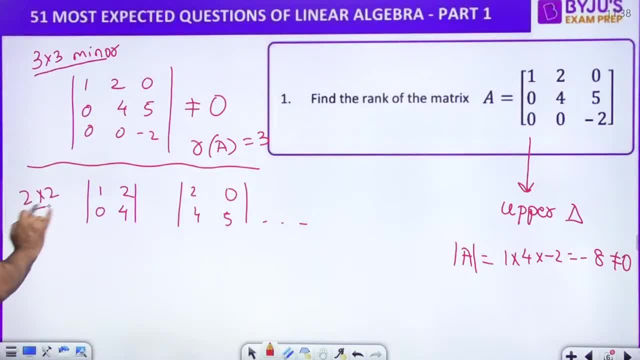 9, 2 cross 2 minors, etc. These are known as 2 cross 2 minors, But here you do not need to check. Any 2 cross 2 determinant which you can extract from the matrix is the 2 cross 2 minor. 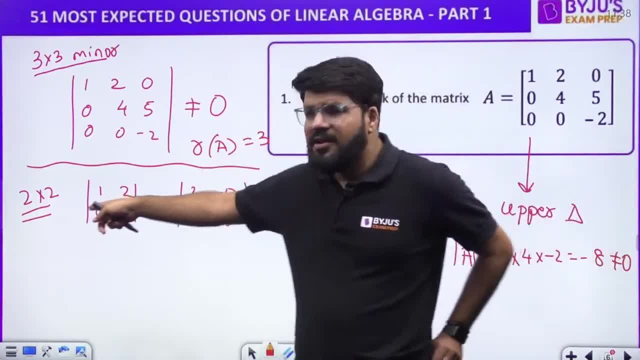 Right. So if suppose this was 0, then we will check whether the 2 cross 2 minor is non-zero, And if the 2 cross 2 minor is non-zero, then the rank would be 2.. Something of this sort, Okay. 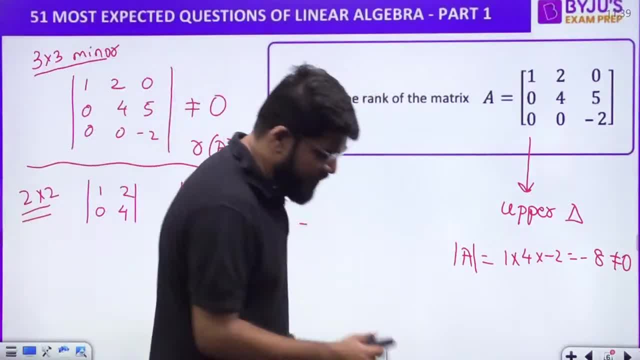 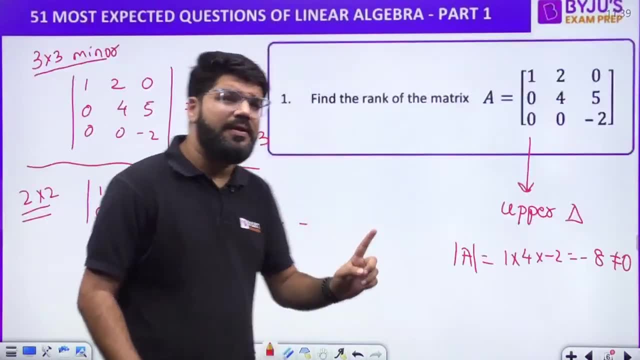 But here the 3 cross 3 minor itself is non-zero And, as per the first key point I am mentioning, rank is the largest order of non-zero minor of the matrix. So, which is the largest order of non-zero minor? This is non-zero. Okay, This is also non-zero. 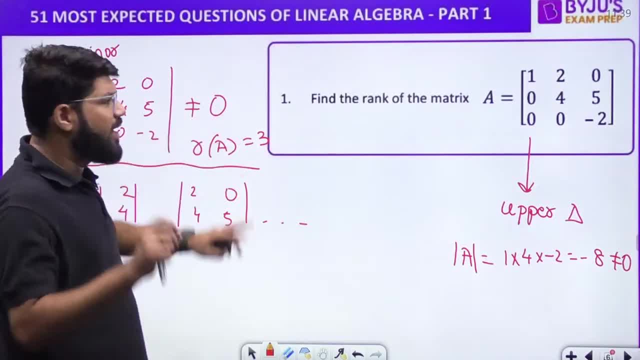 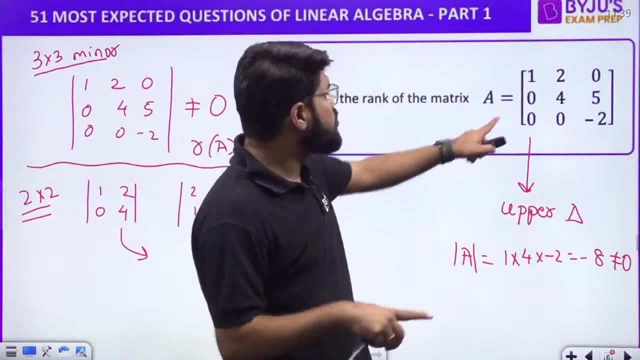 This is also non-zero, But this is not the largest order. The largest order is 3, and hence rank is known as the 3.. That simply means. that simply means, if there is a square matrix, if there is a square matrix like 3 cross 3, what can be the maximum possible rank? The maximum possible rank. 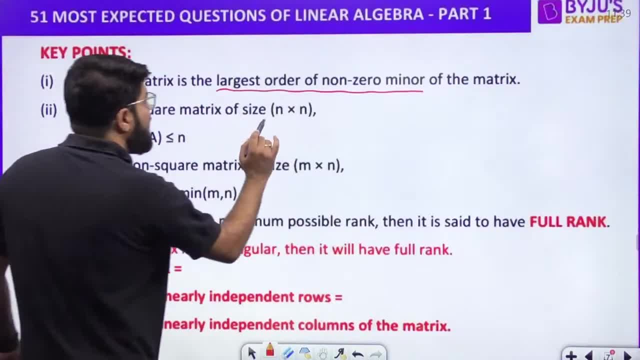 can be 3.. Here it is 3 only Right. In general, if there is a square matrix of size n, n, n, n, n cross n. if there is a square matrix of size n cross n, then the rank is always less than equal. 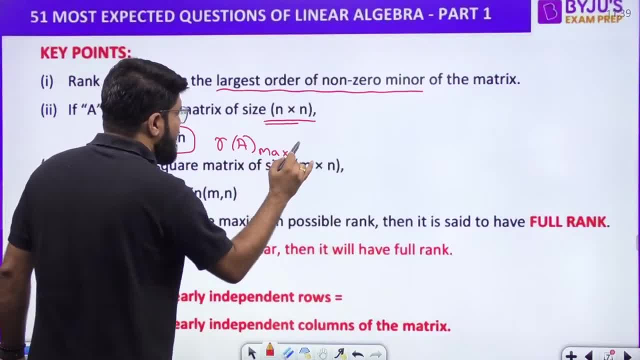 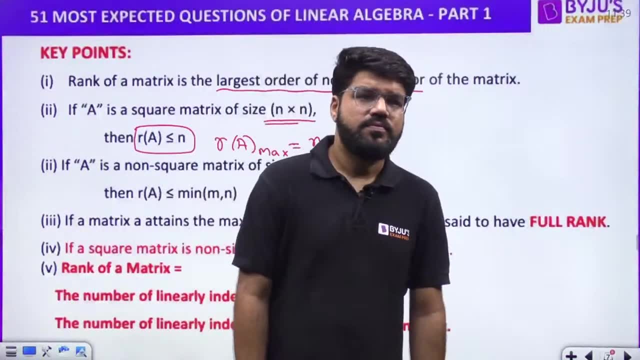 to n, Or I can say that the maximum value of the rank is equal to n. The maximum value of the rank is equal to n. Rank will be n or less than n. Okay, No, no, no. Largest order of non-zero Shiva. 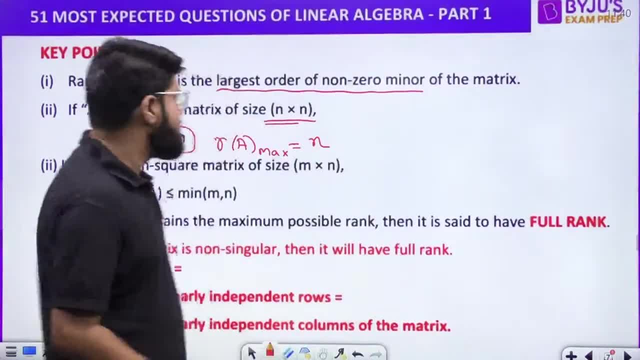 Right, No, rank will not be 2.. Rank is the largest order of non-zero minor. See, this is non-zero, So my rank is 3.. You don't need to actually check this. Okay, I have just written to show you 2 cross 2 minor. 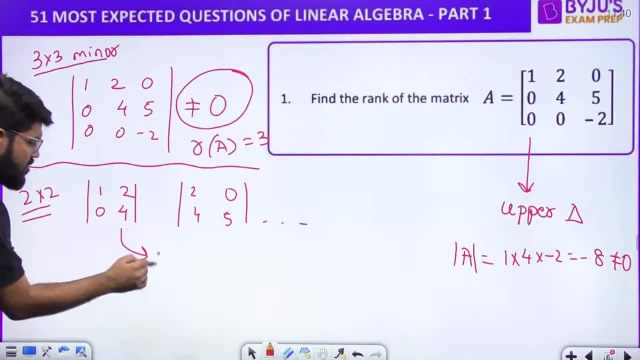 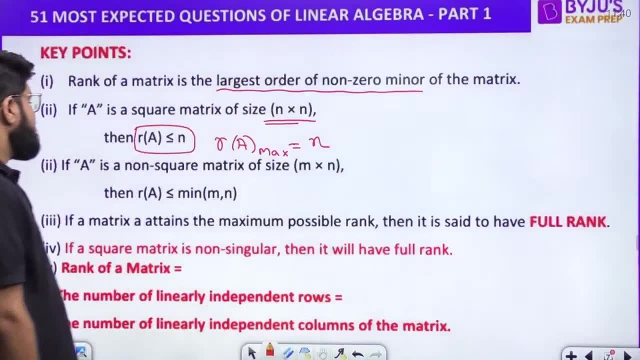 Suppose if this was 0. Then you go and check And if this is non-zero, then the answer will be 2.. Okay, Shiva, Understand the difference. Largest order, Okay. Similarly, if there is a non-square matrix of the size m cross n, then the rank. 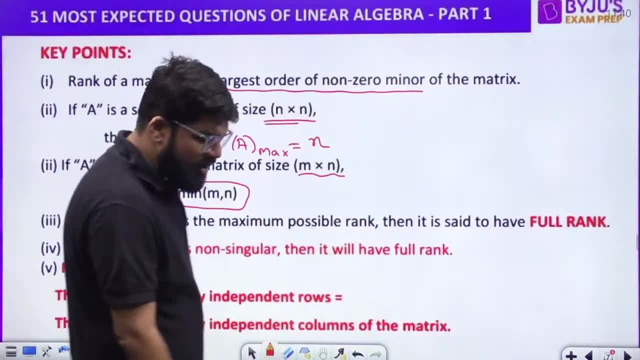 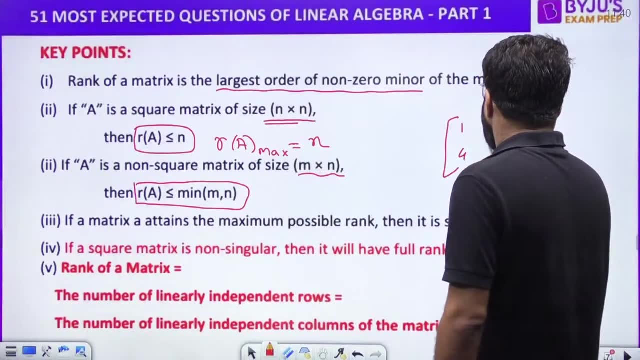 will be less than equal to minimum of m comma n, depending on whether m is len or n is len. Say, for example, I take a 3, I take a 2 cross 3 matrix. Suppose this is a 2 cross 3 matrix I. 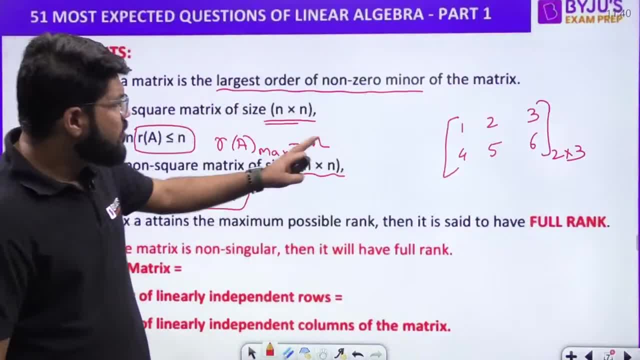 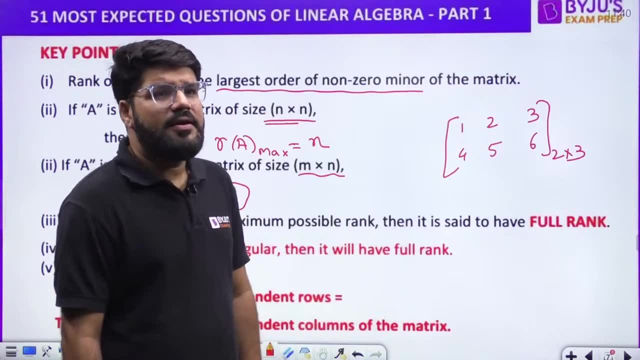 make a non-square matrix. I take a 2 cross 3 matrix. I take a 2 cross 3 matrix. I take a 2 cross 3 matrix, All there? Okay, If this is a 2 cross 3 matrix, then what is the rank? I'm not asking the. 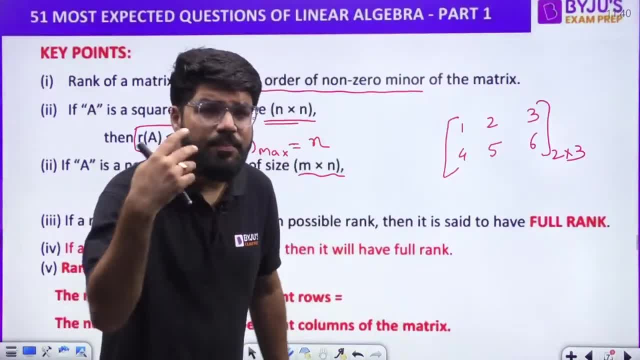 final value of rank, but what can be the maximum possible rank? So what is the maximum possible minor? Can you make a 3 cross 3 minor? For a 3 cross 3 minor, you need 3 rows and 3 columns. 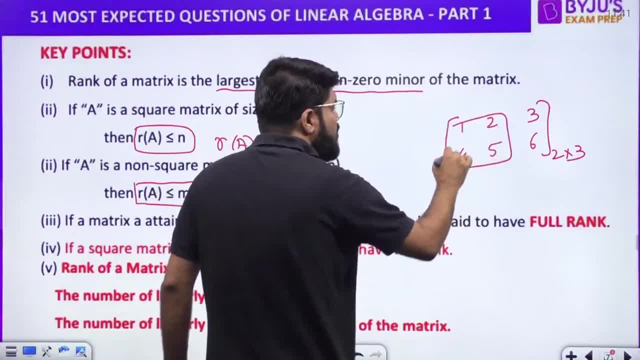 Right. Can you make a 3 cross 3 minor? No, Maximum you can take a 2 cross 2 minor. Maximum what you can take is a 2 cross 2 minor. So what is the maximum possible rank of this? 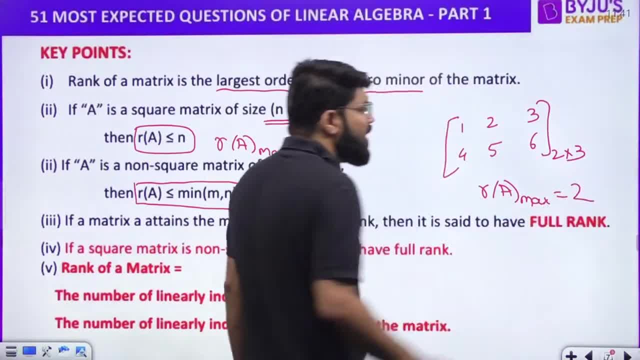 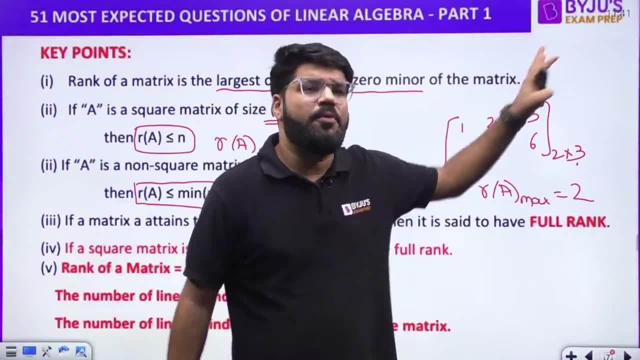 matrix. What is the maximum possible rank of this matrix is equal to 2.. Minimum of m? n. I'm not telling rank is 2.. I'm not calculating, I'm not bothering, I'm just telling you some important points. Baad mein, calculate karenge Right. But what I'm trying to say you, whenever there is a non-square, 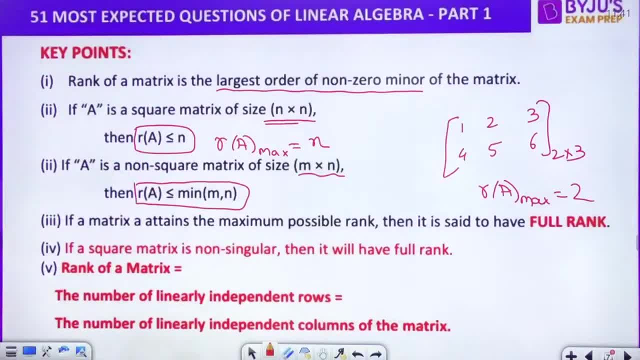 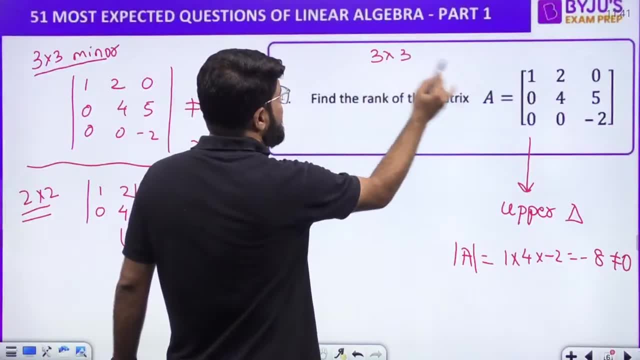 matrix, the rank is always less than equal to minimum of m n. Minimum of m n. Now, previous case: previous case: it is a 3 cross 3 matrix. A is a 3 cross 3 matrix, So what is the maximum? 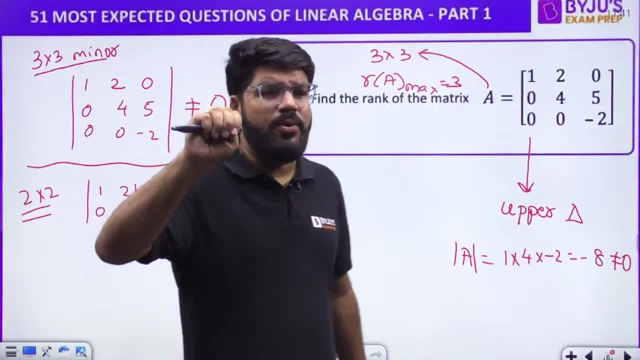 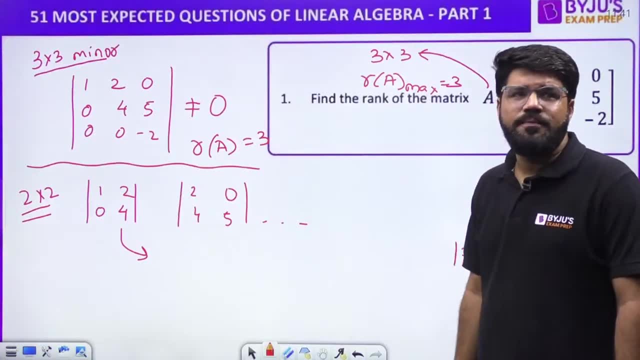 possible rank of a 3 cross 3 matrix. As I told you, rank is less than equal to 3.. Maximum possible rank is 3.. But actual rank is also 3.. In the previous question, actual rank is also 3.. Actual rank is also 3.. So 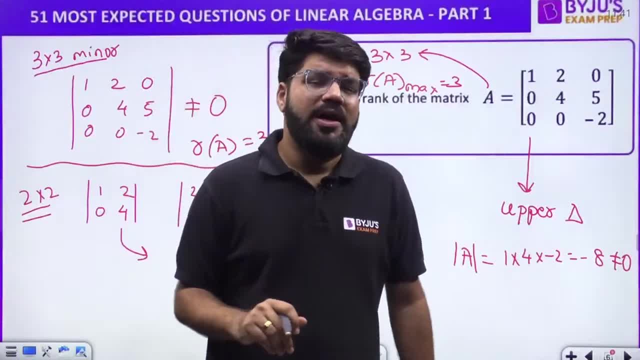 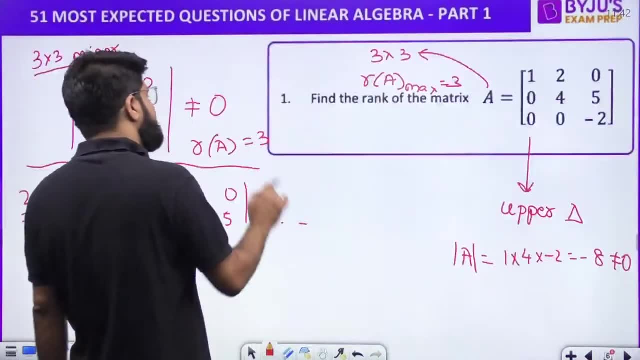 whenever a matrix attains the maximum possible value. whenever the rank of a matrix attains the maximum possible value, then it is said to have full rank, Then it is said to have full rank. So this is the condition of full rank: Whenever a matrix attains its maximum. 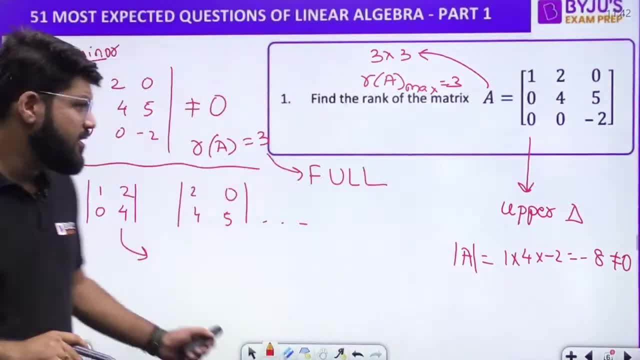 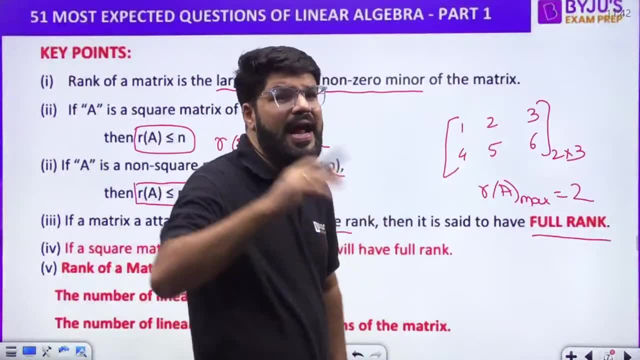 possible rank value, then it is said to have full rank. So this is the condition of full rank. So this is the condition of full rank. So, as I told you that with questions I am going to revise the concepts and the points also, Just stay tuned and stay updated and I don't 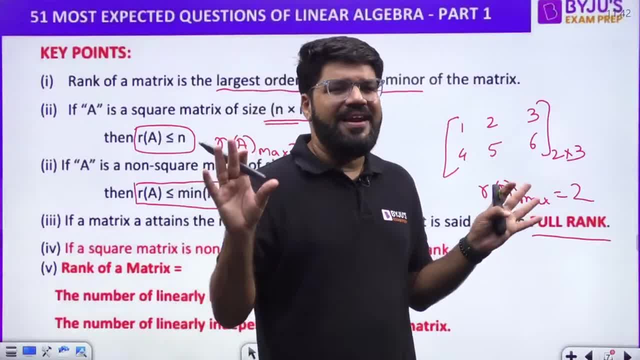 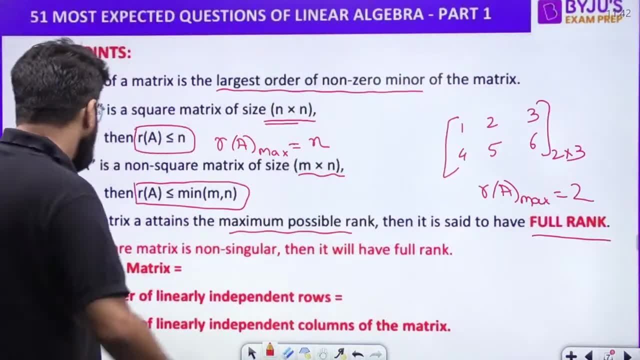 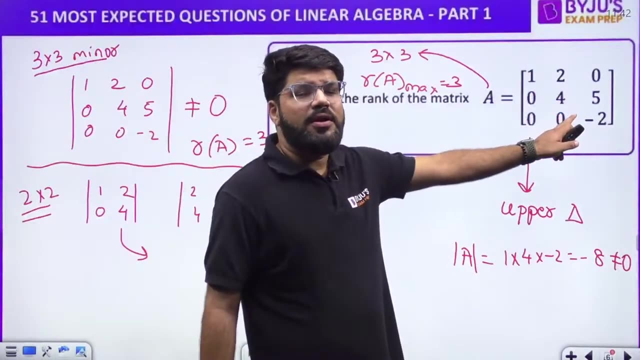 see that likes increasing Guys. dull morning, bright morning, motivated morning, What is that guys? What is that? Okay, we see little, very, very, very slow and sluggish type of response. Okay, right, So if a square matrix is non-singular, non-singular matrix is what? 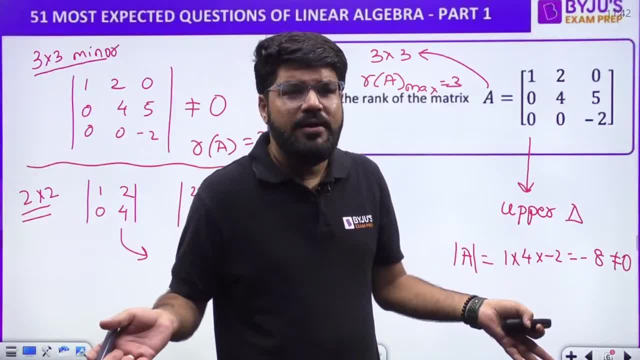 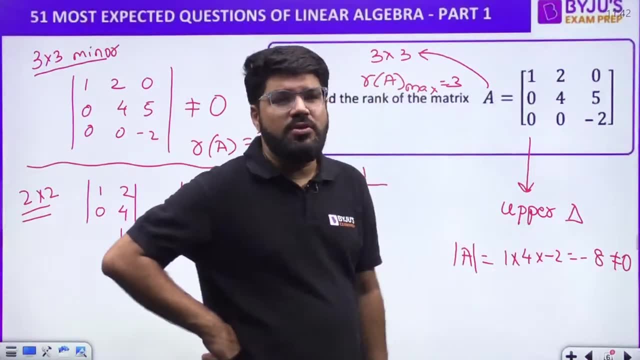 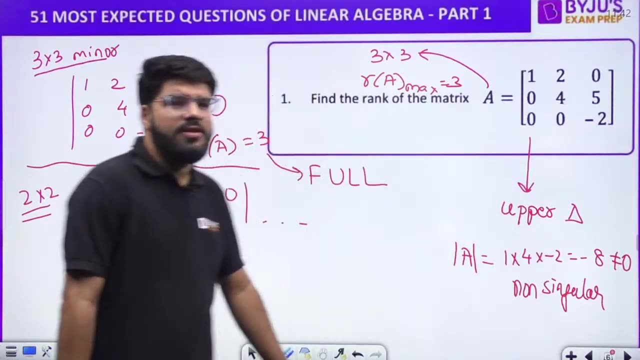 Non-singular matrix is one which has non-zero determinant, Which has non-zero determinant. A singular matrix is one which has zero determinant. So here the matrix has non-zero determinant. So I will call this matrix as I will call this matrix as non-singular. Okay, I will call this particular matrix as non-singular. 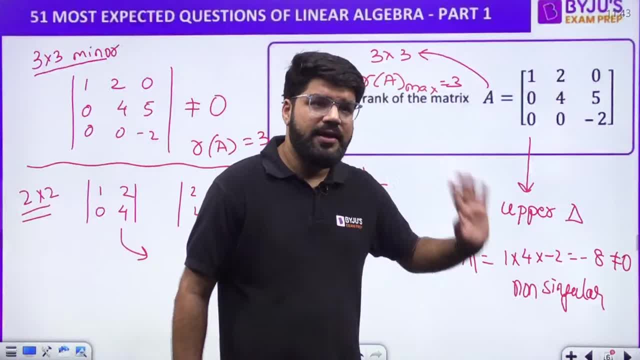 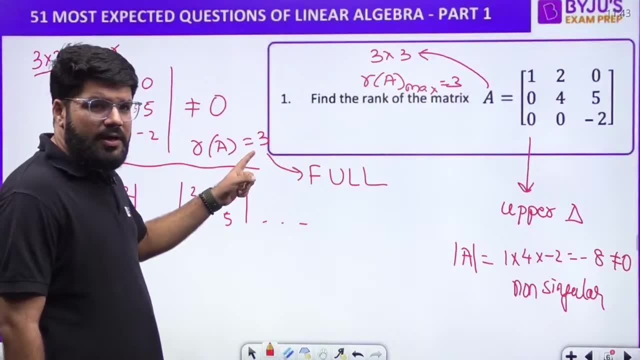 Is it okay? I will call this matrix as non-singular. Ye dhyan rakna. Okay. Now, if this is a non-singular matrix, that is why the rank was equal to full. Okay, Determinant non-zero rank is equal to 3.. So whenever a matrix is non-singular, then it will. 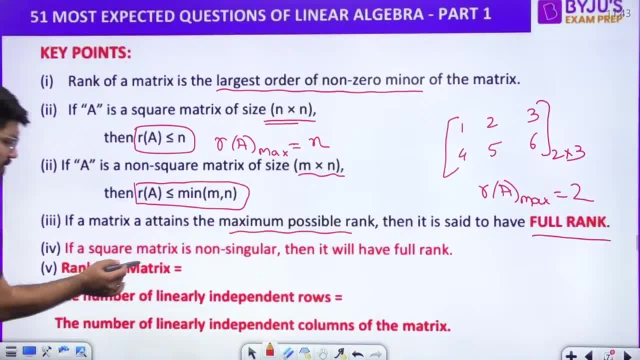 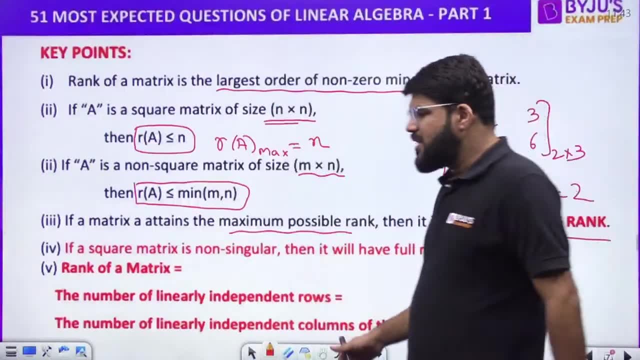 have full rank, Then it will have full rank. Okay, This is a very important point. last one, But leave it for a moment. I will discuss it after few more minutes. Okay, So whenever a matrix is non-singular, that is, having non-zero determinant, it will always have the full. 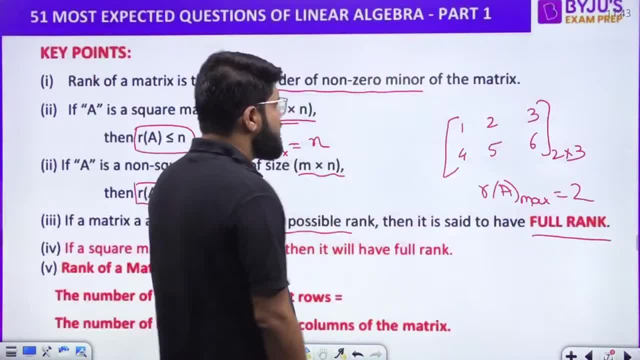 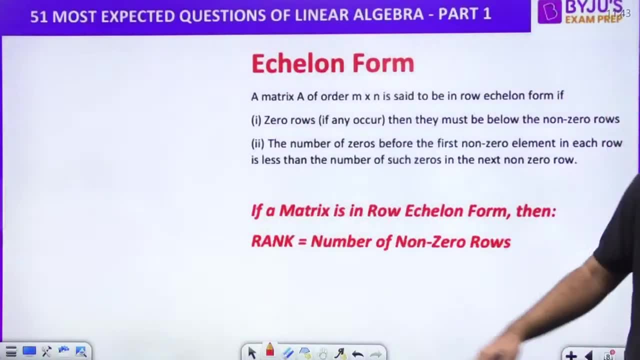 rank. It will always have the full rank. Okay, Ye condition, yaad rakna hai aapko. Now let us understand what echelon form is. In some of the questions, echelon method will be applied, and then I will come to the independency wala. This is the best one. This is the best one. 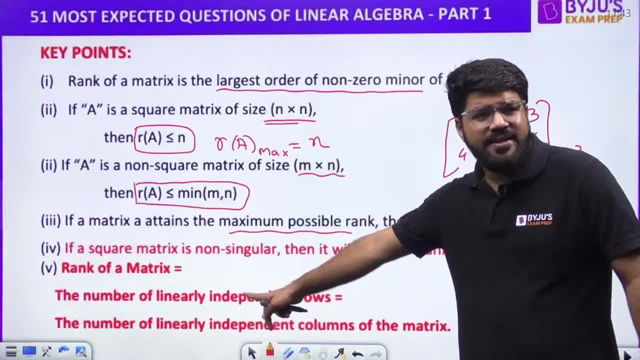 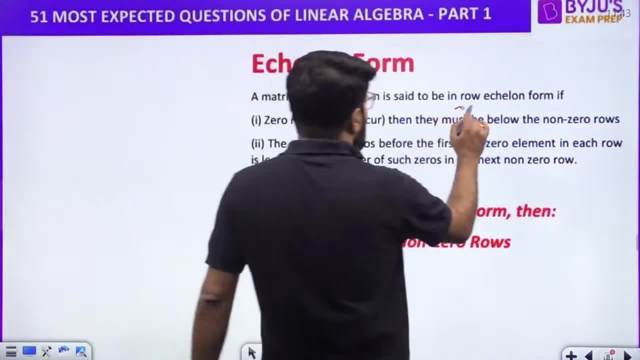 This is the shortcut. You can solve most of the questions within seconds because of the last property. So I will come back to that. But first let us understand what echelon form is Right, Specifically talking about row echelon form- Row echelon form Right A matrix. 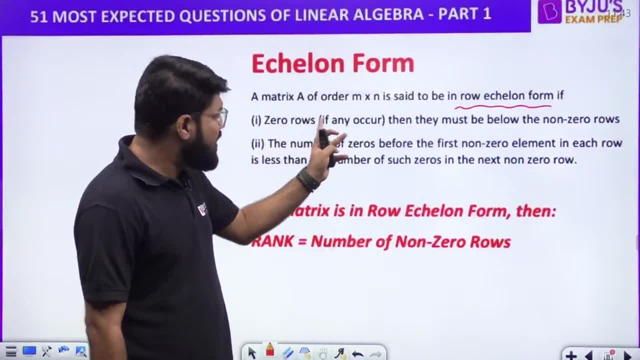 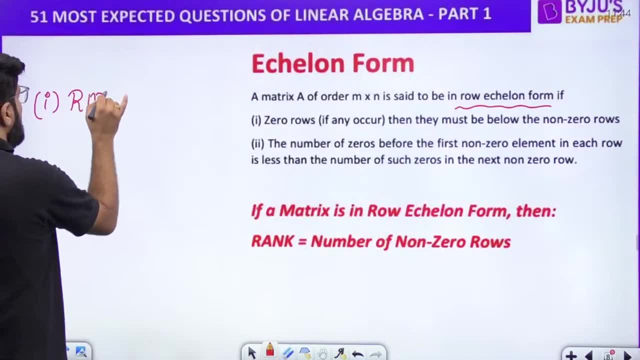 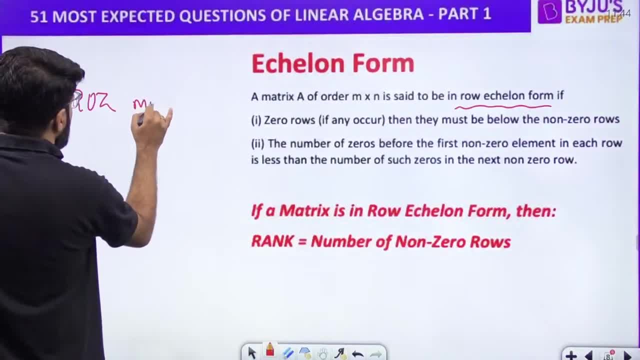 ROZ, ROZ, ROZ, ROZ, ROZ, ROZ ROZ. If any must be at last. If any Agar nahi hai, toh koi baat nahi. Number 2 condition: The number of zeros before the first non-zero element. 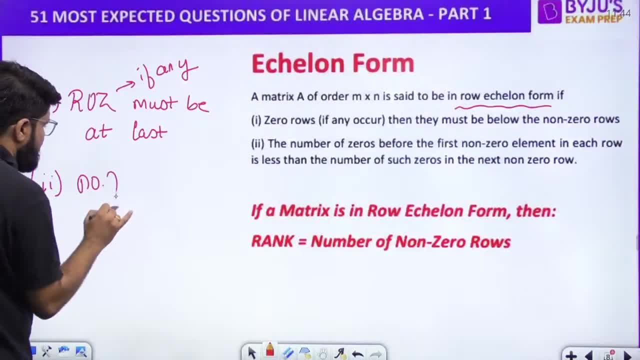 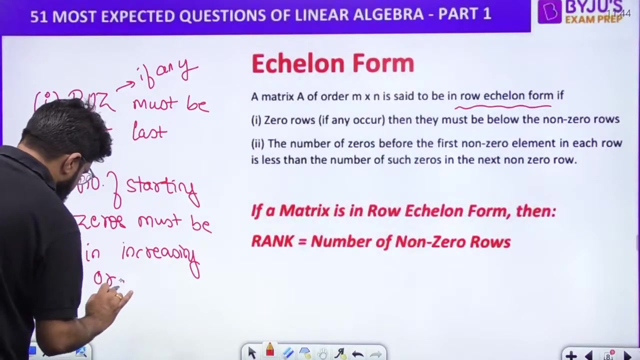 in every row. I will call it as. I will call it as number of starting zeros And I will explain you through the question: Number of starting zeros. Number of starting zeros must Must be in increasing order. Must be in increasing order. 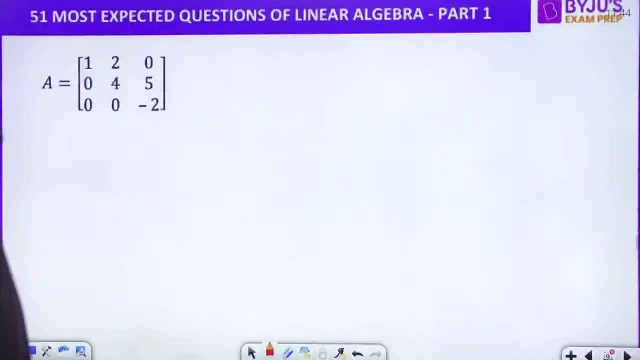 Let us understand very simply. If we understand this in a very simple way, have a look into this: 1, 2, 0, 0, 4, 5, 0, 0, minus 2.. 0, 0, minus 2.. 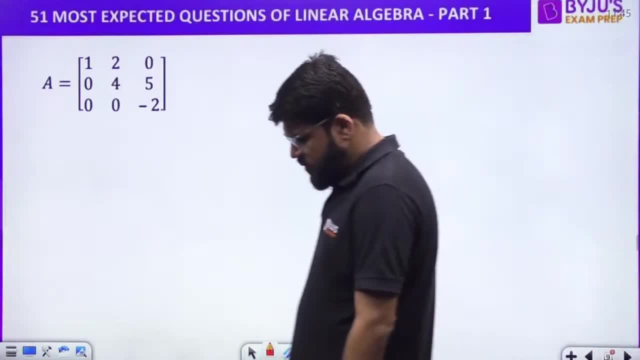 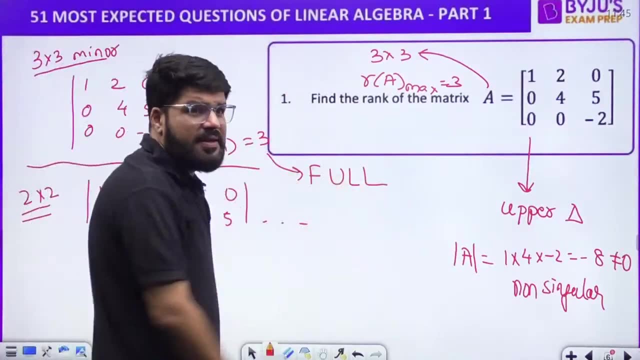 Okay, Let's go Now. same question, guys. It is the same question, The same question, which we have solved by the determinant. Now I am going to explain you the echelon form. Is there any row of 0?? Right now, I am not able to see any row of 0.. 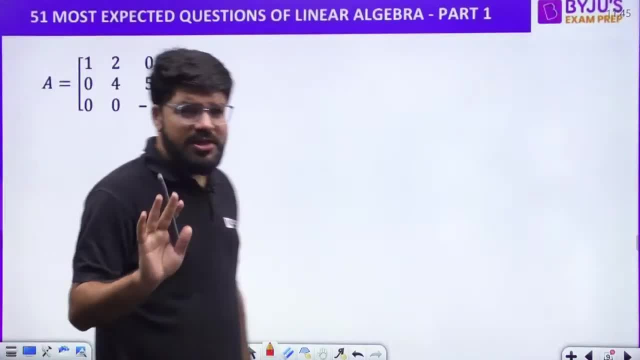 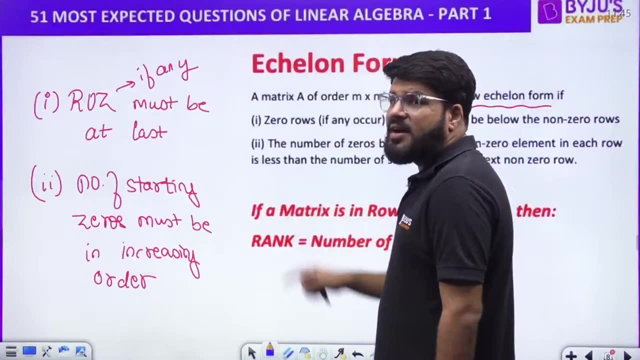 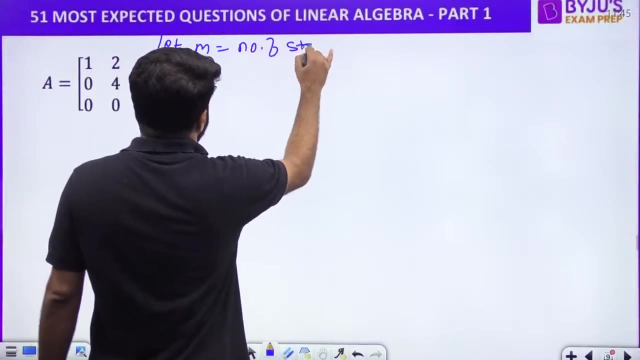 Let us count the number of starting 0s. I told you na What is the second point: Number of starting 0s. Okay, So understand here: Let M is equal to number of starting 0s. Let us say M is equal to the number of starting 0s. 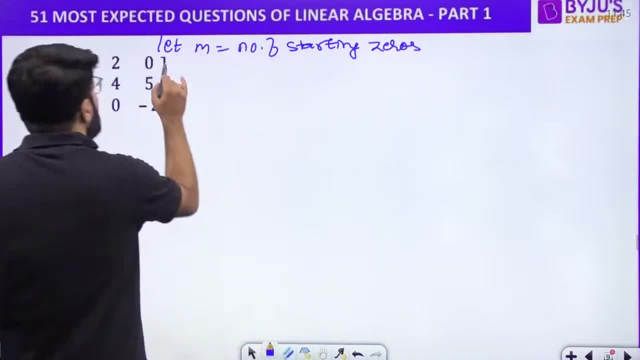 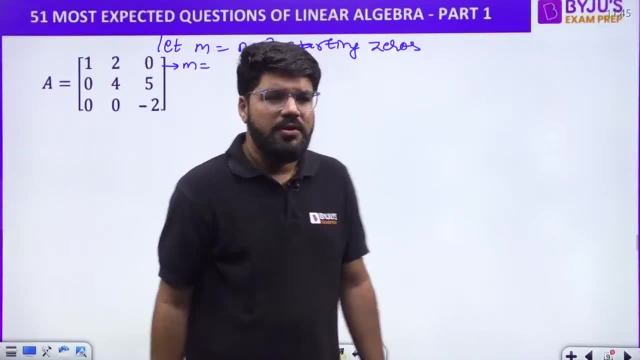 Okay, So M is equal to the number of starting zeros. So, guys, what is the value of m here? Starting zeros? Starting zeros means whatever the zeros you see in the beginning of any row, That is, m is equal to 0.. 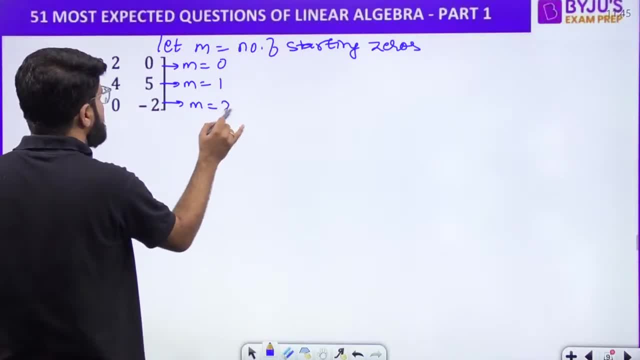 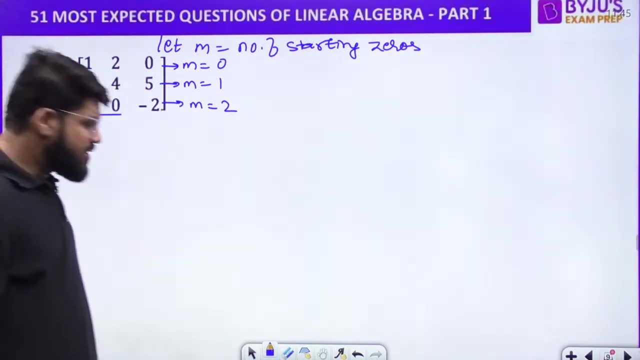 This is known as m is equal to 1, and this is known as m is equal to 2.. 0, then 1,, 0 and then 2 zeros. This is the starting zero. These are the starting zeros, right? Is it following increasing order? 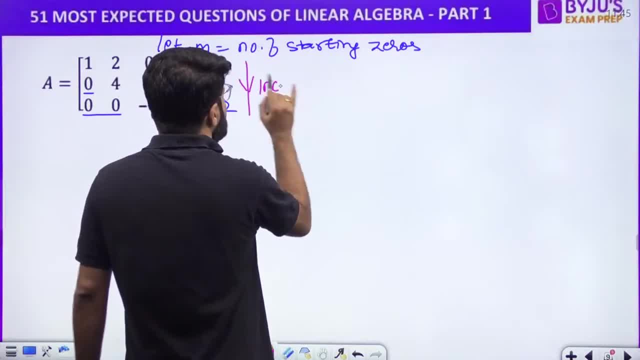 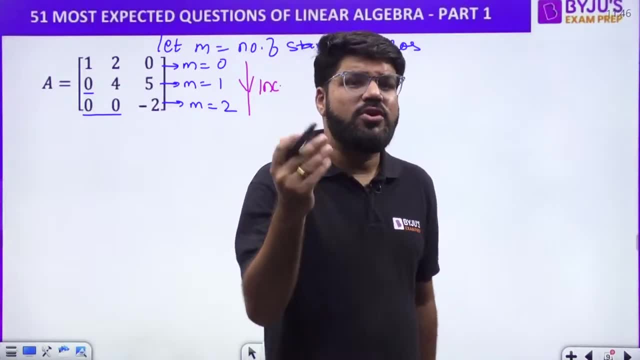 Yes, it is increasing, So number of starting zeros are increasing. There is no row of 0.. If there was a row of 0, it must be at the last, but there is no row of 0. That means it is in the. 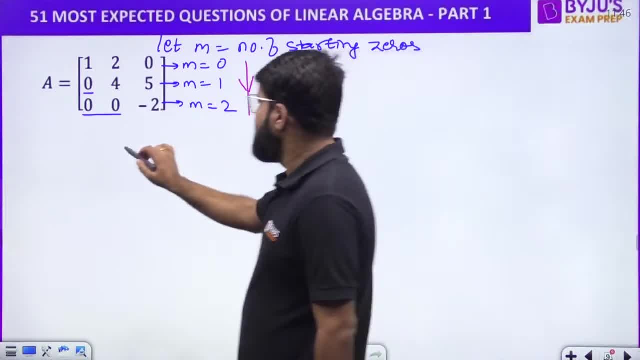 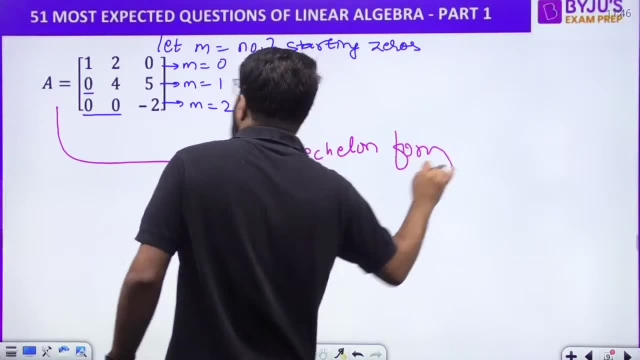 echelon form. It is known as the echelon form, So this matrix is in row echelon form automatically. I will tell you some questions. where the matrix is not in the echelon form, We will convert into echelon form. We are going to convert into echelon form. We are going to convert into echelon form. 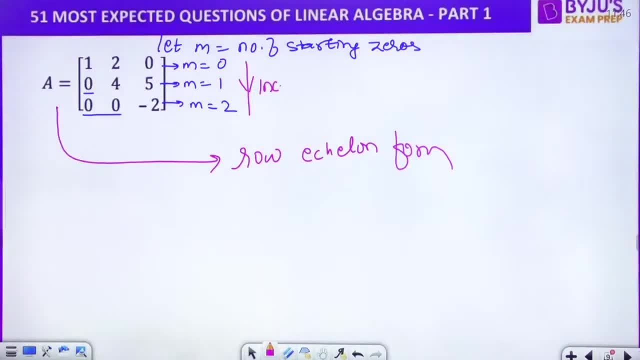 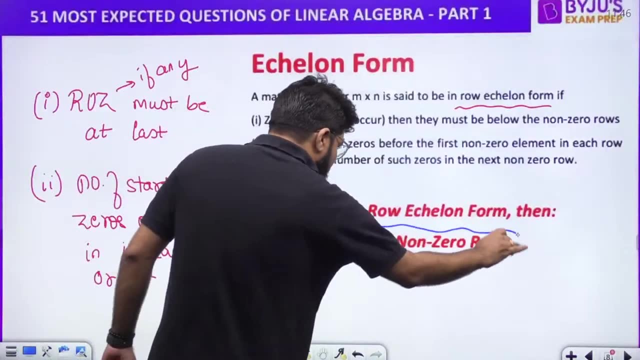 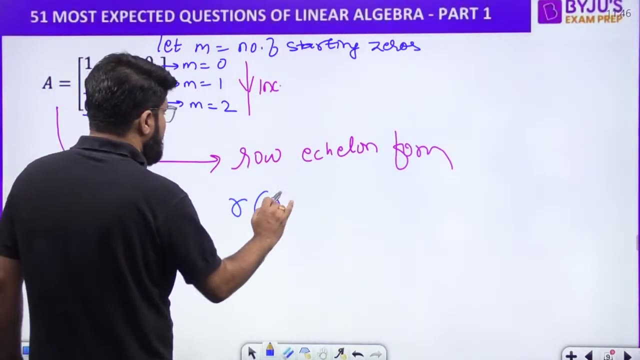 Don't worry, But this is already in the row echelon form. and then I told you, whenever a matrix is in the row echelon form, then then, dear, the rank is equal to number of non-zero rows. The rank is equal to number of non-zero rows. So what should be the rank here? How many? 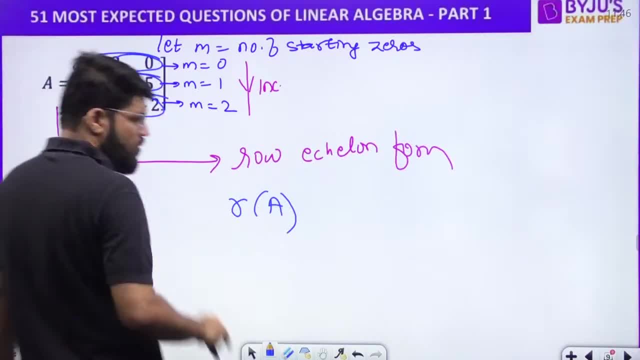 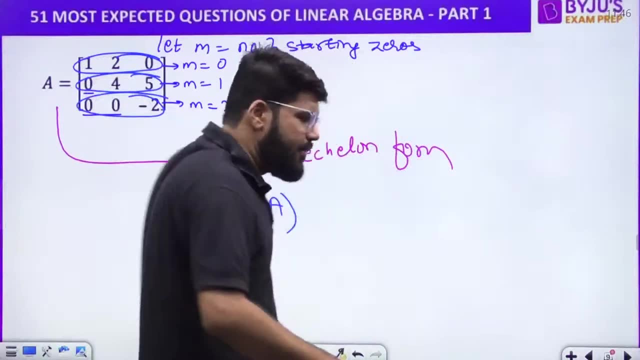 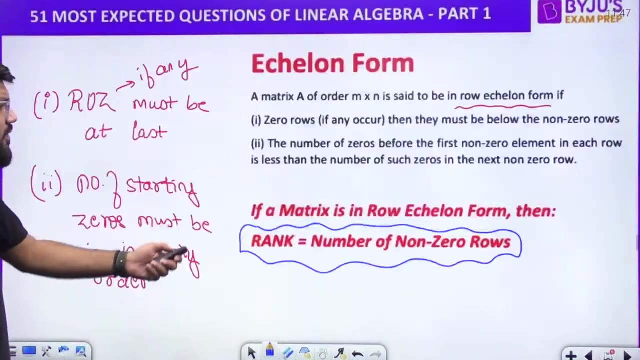 rows. This is non-zero. This is non-zero, This is non-zero. All the three rows are non-zero. Now, what do you mean by zero row? All elements must be zero. All elements must be zero, Right? So rank of A is equal to number of non-zero rows. That is equal to three. Already we have 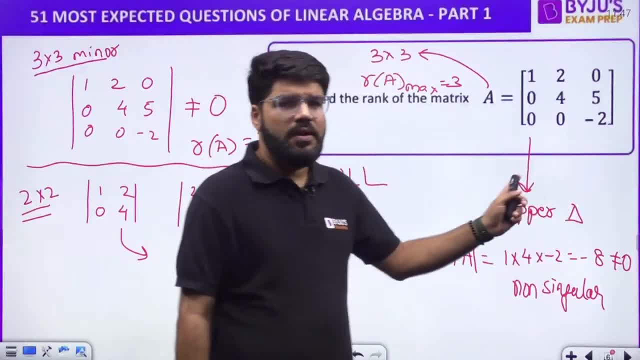 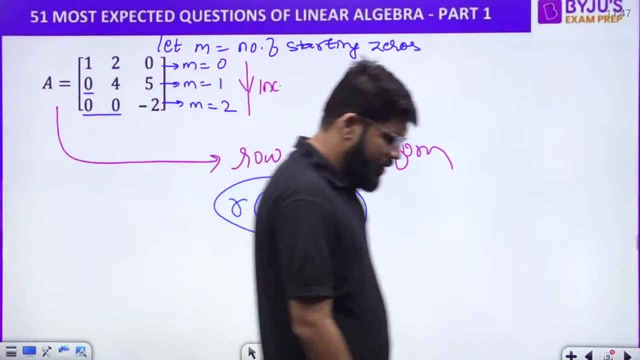 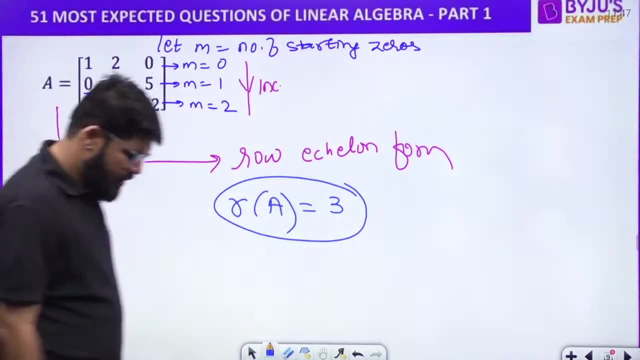 commented that the rank is going to be three. Already it was specified that the rank is going to be three. Here also we have found that the rank is going to be three. So the R of A is equal to the three Right dear. R of A is equal to be three. 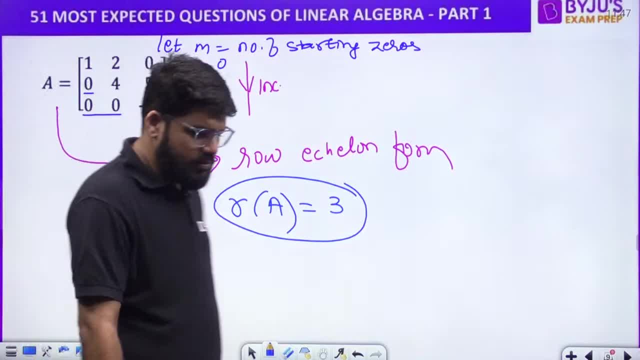 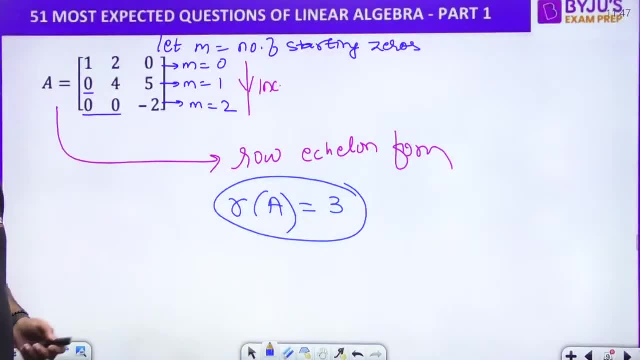 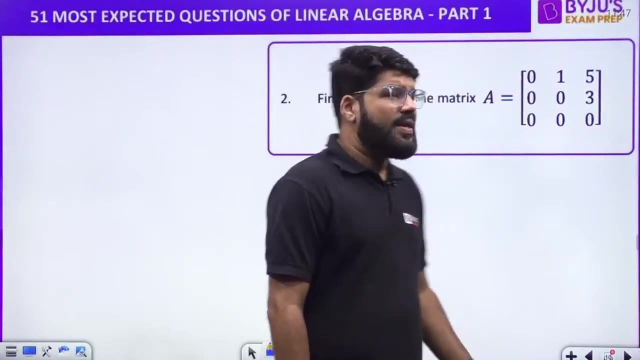 Chalo Cool R of A is equal to the three Chalo Great. Moving ahead to the next, then Moving ahead to the next. Okay, Find the rank of the matrix Now, see Find the rank of the matrix Once again. 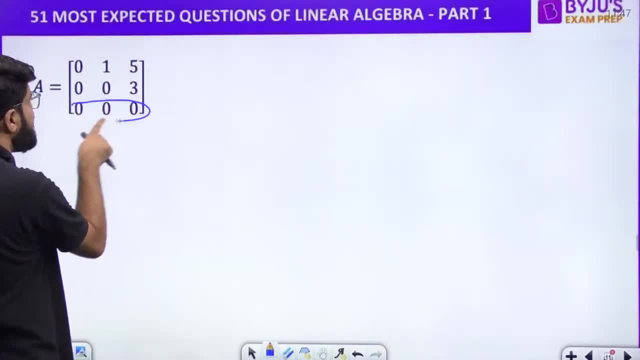 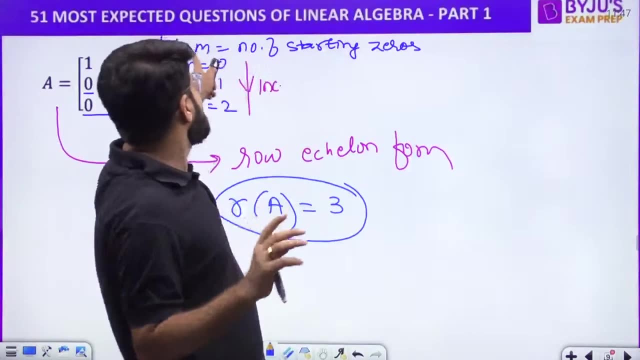 you see, I have taken this matrix separately. There is a row of zero here, but that is at the last. Okay, Let us count the M. M is what M is number of starting. zero, That I will fixed. Okay, That is fixed. Let us say M is the number of starting. 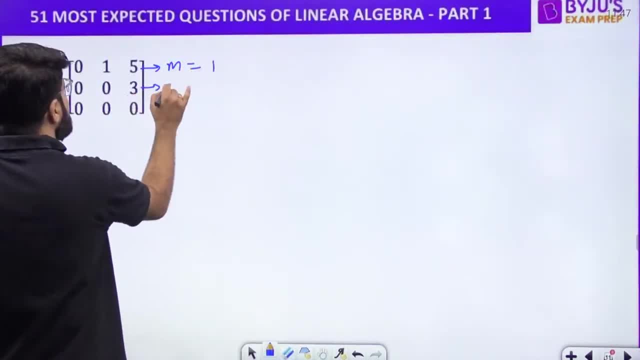 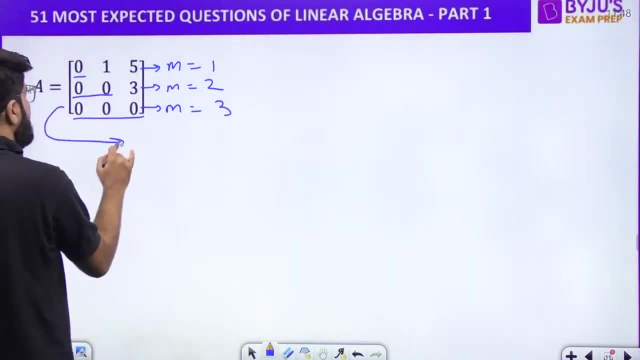 zero. So what is the M here? M is equal to one. What is the M here Two? One zero, two zeros and three zeros. What is the M here? Three? Okay, Automatically you are able to see. Yes, there is. 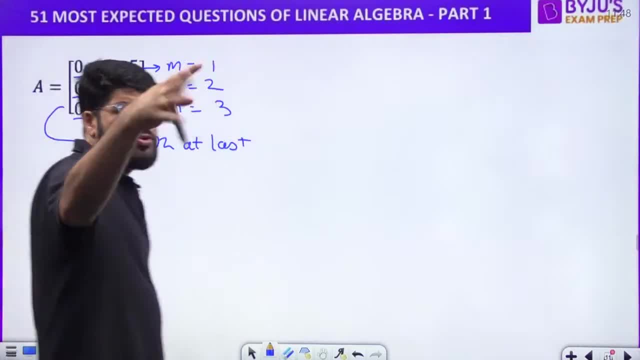 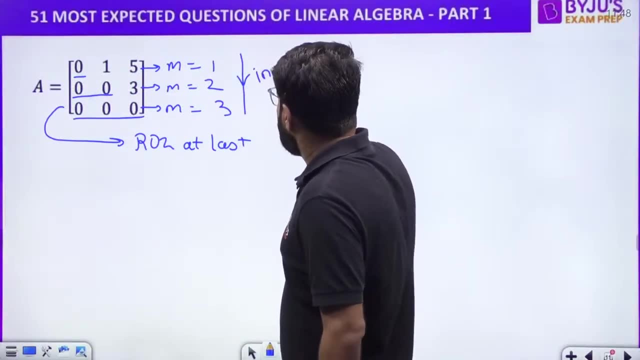 a row of zero, but that is at the last. If it is not at the last, you have to do some adjustment to come it into last. Okay, So row of zero is at the last. Number of zeros are in the increasing order. Okay, So this clearly says that the matrix is in echelon form. 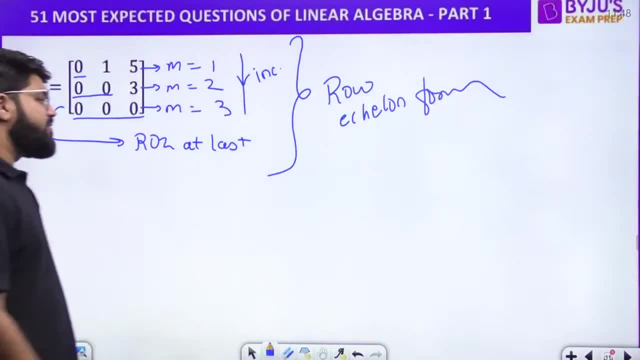 Matrix Is in echelon form. Matrix is in row echelon form. and if the matrix is in the row echelon form, what is going to be the rank? Rank is number of non-zero rows. Clearly, one is the row of zero. 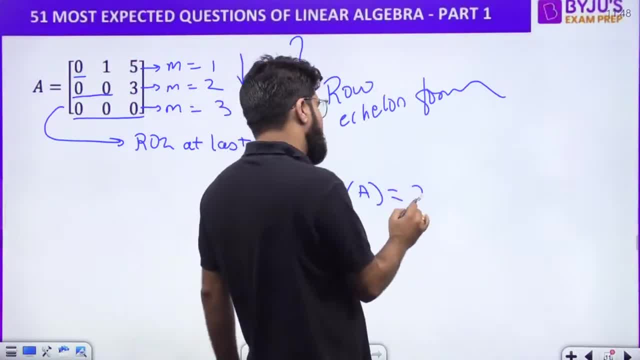 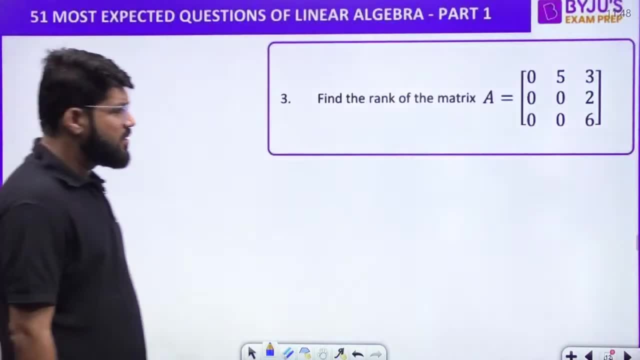 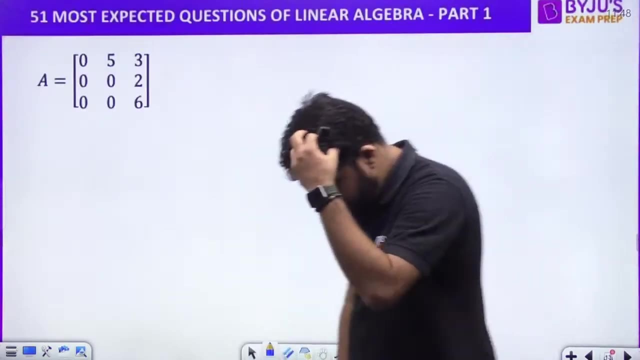 So how many non-zero rows, Sir? two non-zero rows and the rank of the matrix is equal to two. That is what is the meaning of echelon form. Next question, Number three: Have a look into this. Have a look into this matrix: 053, 002, 006.. Okay, And let us. I have copied this matrix once again. 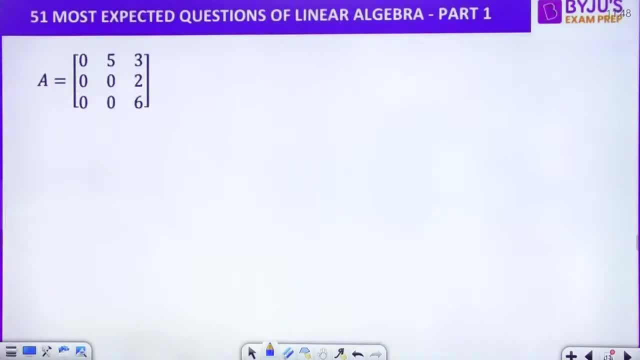 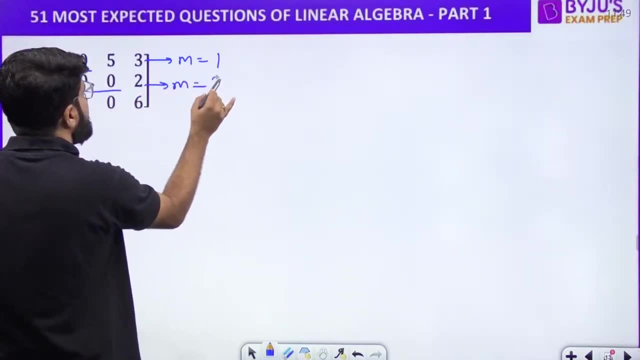 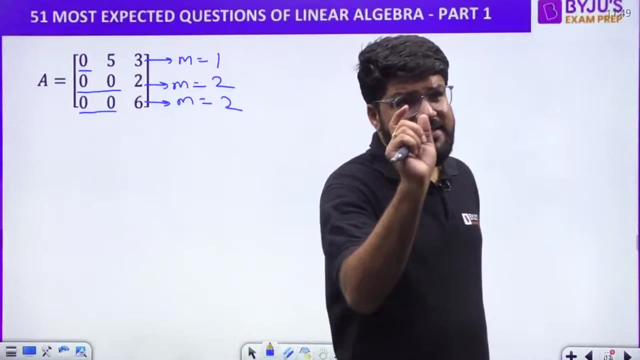 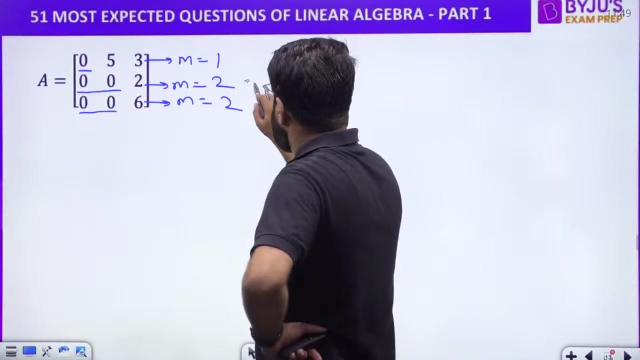 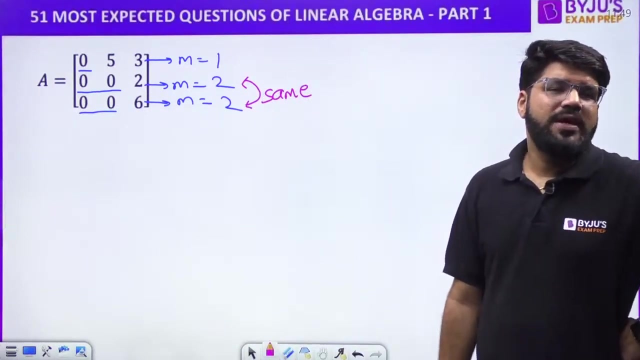 here, Okay: 053, 002, 006.. 006.. Okay, Now keep in mind. what is the value of m here? One, Right. Then next row: what is the value of m? It is two. Right now, there is no row of zero. Next row: number of zeros: starting zeros is two. Number of starting zeros: strictly Okay. Okay, Now tell me, does it follow increasing trend? Does it follow the increasing trend? Does it follow the increasing trend? 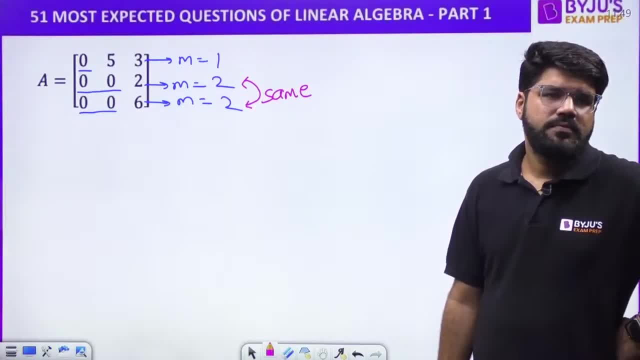 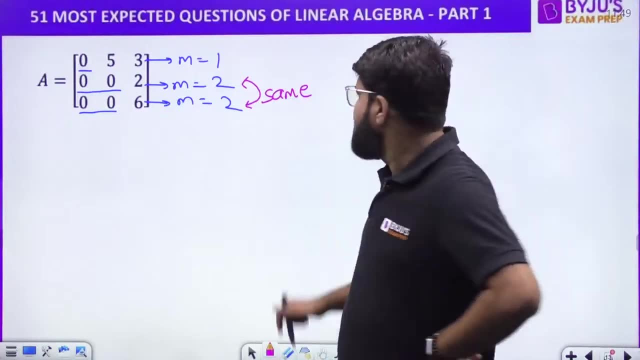 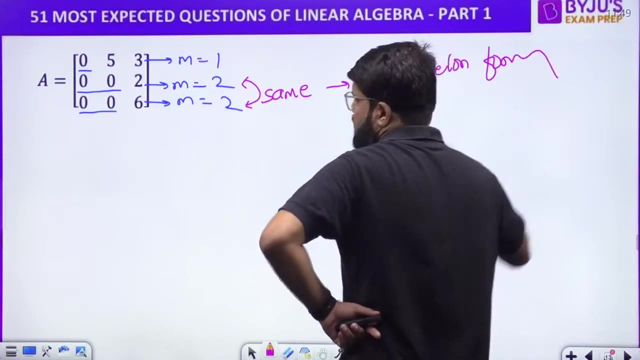 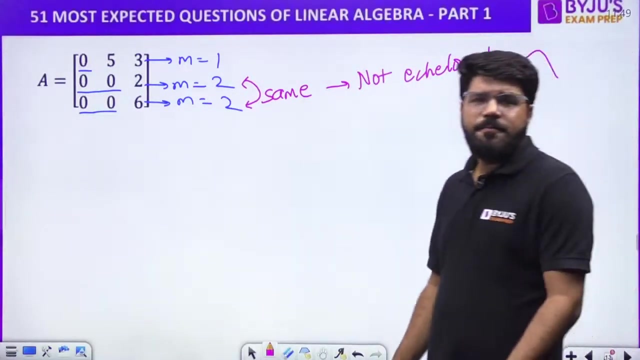 No, It should not be same. also Strictly increasing, Strictly increasing. It should not be same. also Right, So this is same. So this is not the echelon form. I will now say that this is not the echelon form. So what to do, dear? What to do then? How to convert into the echelon form Everybody with the big fire, Right, Right, Yes, yes, yes, The PDF you are going to receive for this session. 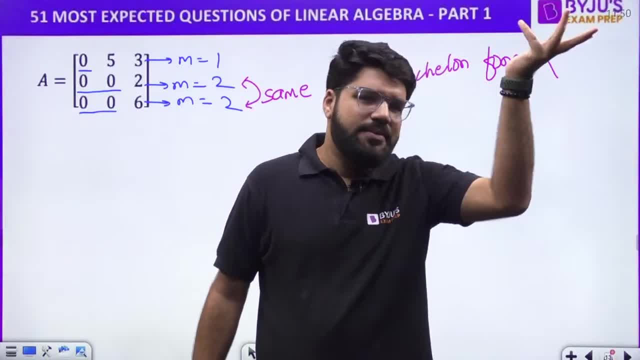 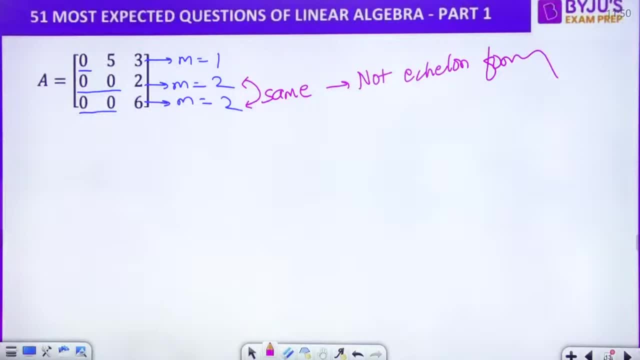 Password protected Password. I will tell you after some time, I don't know, But yeah, PDF, you will receive that- to password protected. So stay tuned to the session. Have a look into this. Okay, This is not the echelon form. So what to do, sir? Okay, What to do? So I will convert it into echelon form. So what I am going to do? have a look into this. Right To convert into echelon form, this should be increasing And for it to be increasing, 123.. Here should be 3.. 123. Here should be 3.. Is it okay? 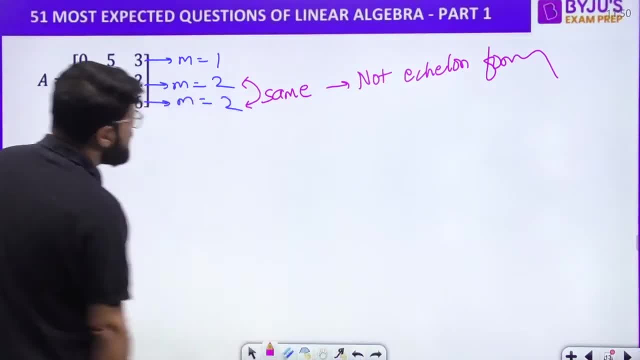 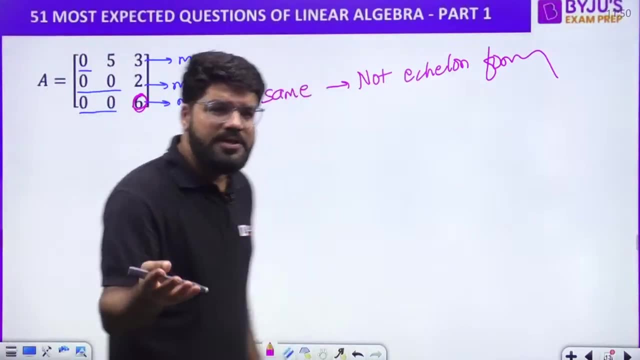 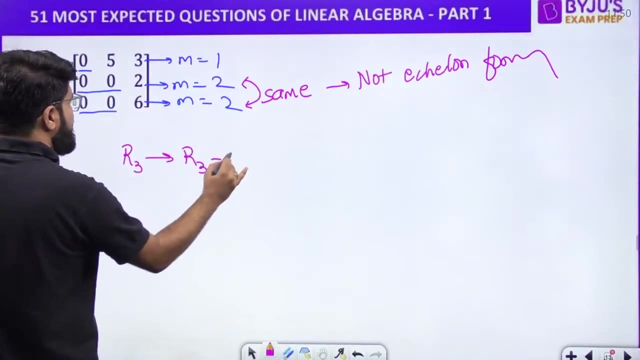 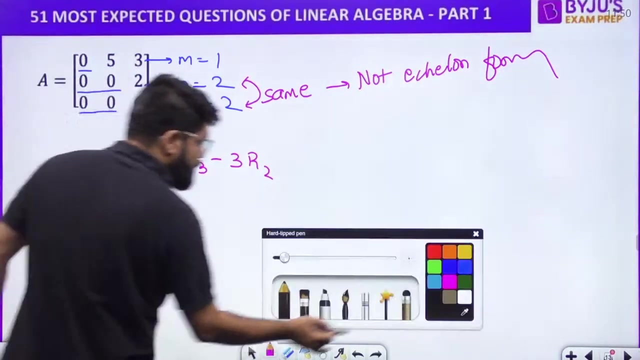 Here. this should be the 3.. Correct, This should be the 3.. So 3 zeros means I have to make it this 0.. So I have to apply the elementary row operations. I have to apply the elementary row operation. I have to convert this 6, which is in the third row, to 0.. R3 can be written as R3 minus 3R2.. Right, Multiplying this by 3.. 3, twos are 6.. 6 minus 6 will become 0.. Right. So doing this, performing this, I am going to get the matrix, which is 0,, 5,, 3.. 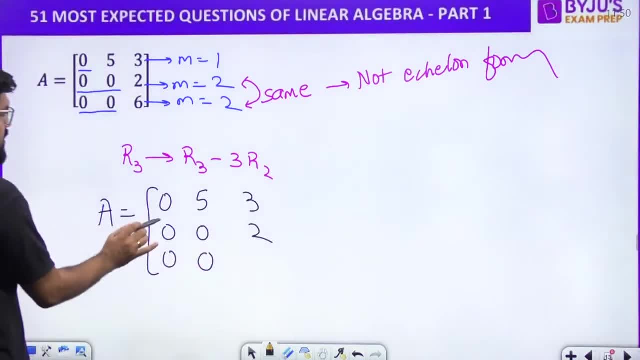 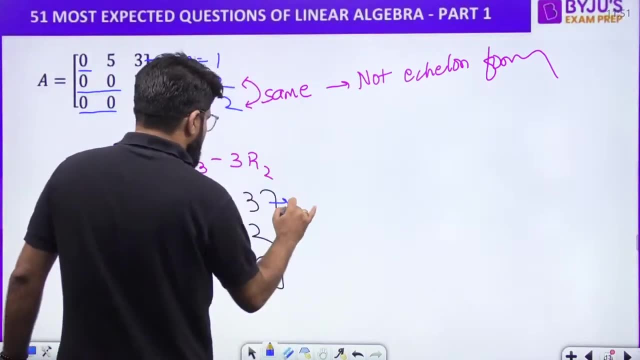 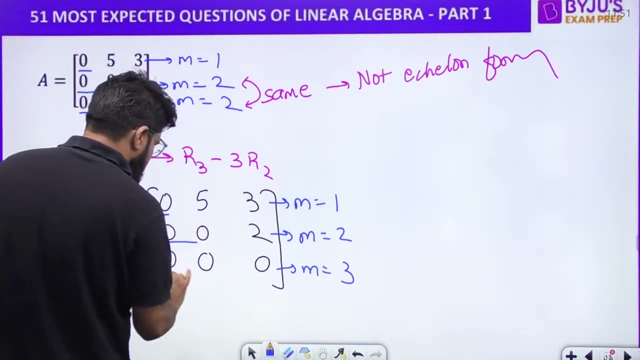 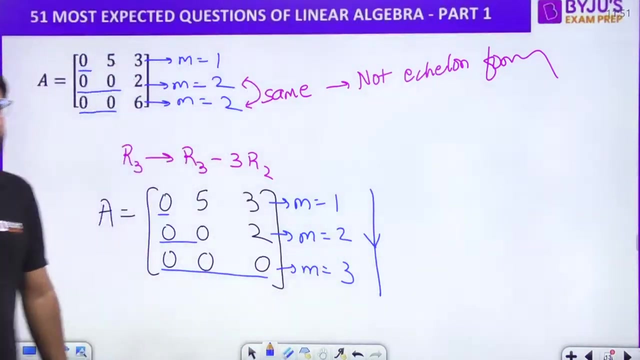 0, 0, 2.. 0, 0.. 0 minus 0, 0 minus 0.. 6 minus 3 into 2.. That is again 0.. That is again 0.. Now have a track of M. M is 1.. M is 2.. M is 3.. 1,, 2, 3.. M is 1.. M is 2.. M is 3.. Right, This is what is the increasing order. This is what is known as the increasing order. All, dear students, this is what is the increasing order. 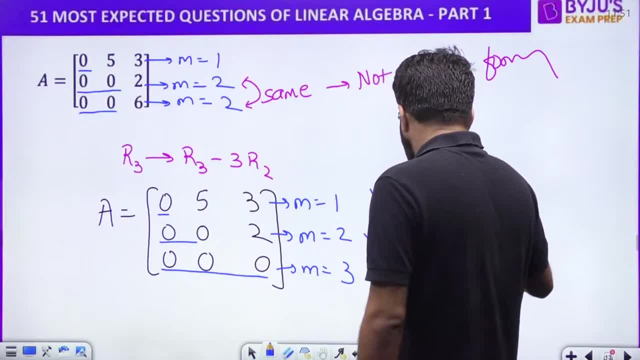 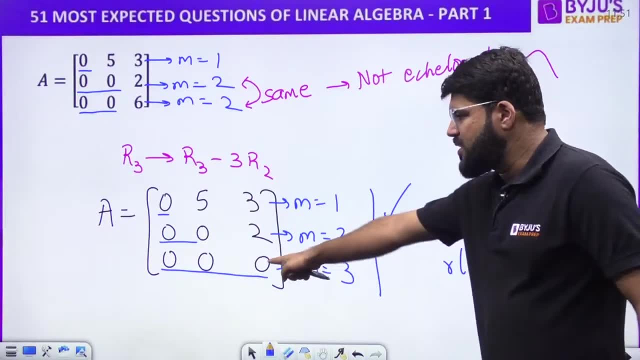 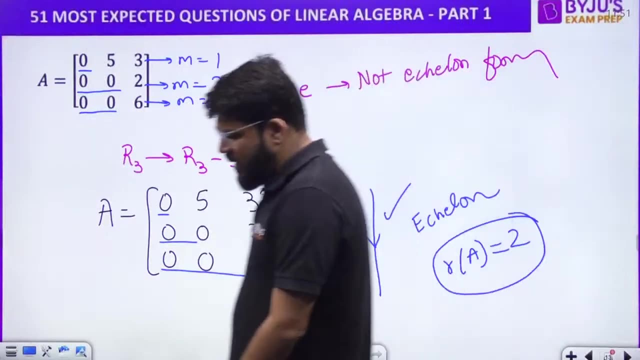 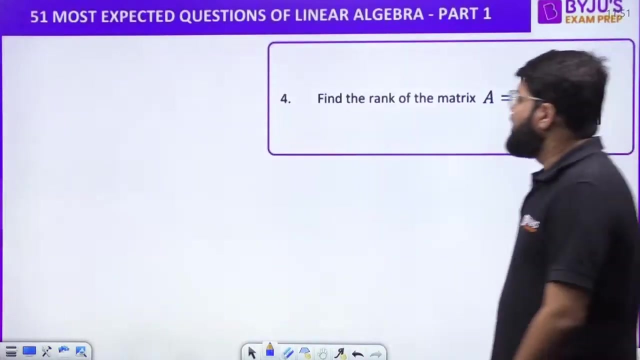 Okay, Now this is correct in the echelon form. Now, this is correctly in the echelon form. And if this is in the echelon form, rank is equal to number of non-zero rows. There is clearly a row of 0.. Row of 0 is, at the last, Very good. I wanted, at the last, only Number of non-zero rows, 2.. Who are? answer for the rank is equal to 2?? Answer for the rank is equal to 2.. Okay, Next one: Find the rank of the matrix. Find the rank of the matrix 1, 2,, 3,, 4,, 5,, 6,, 7, 8.. 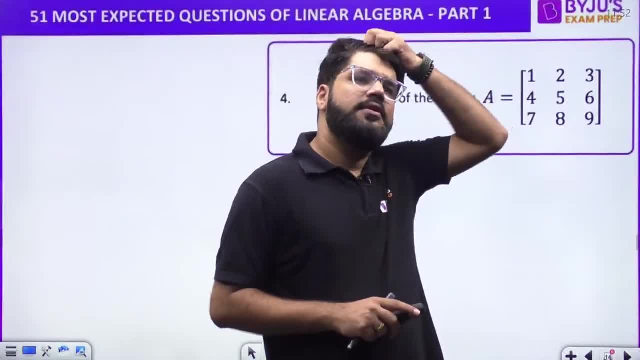 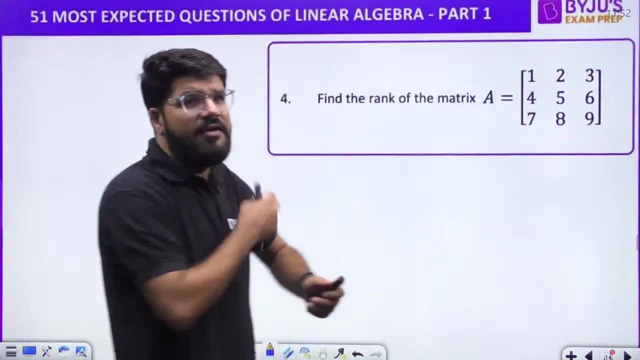 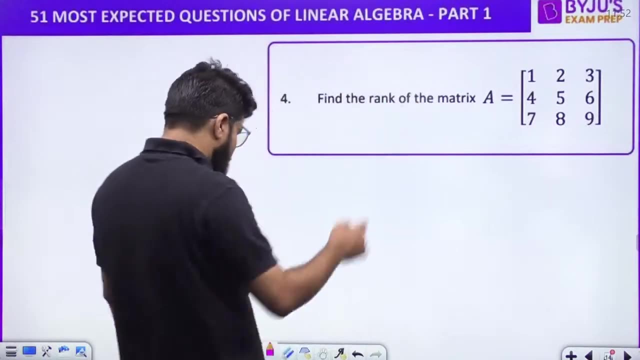 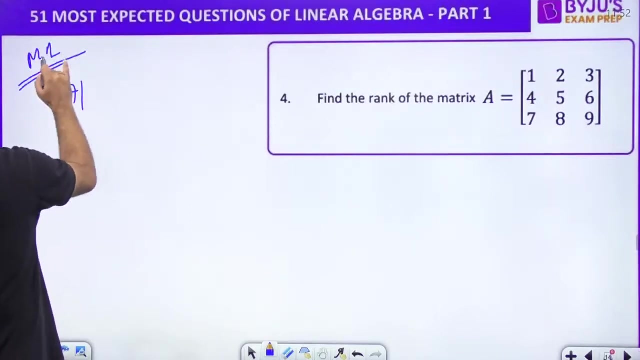 9.. I will tell you. I will tell you 2, 3 things here. I will tell you 2, 3 things here. Now, with this, let us summarize all of the points. Very important With this, let us summarize all of the points. Okay, With this, let us summarize all of the points. Number 1.. Okay, Number 1.. If I just calculate the determinant, Right Method number 1.. If you calculate the determinant of this matrix, this is going to be 0. 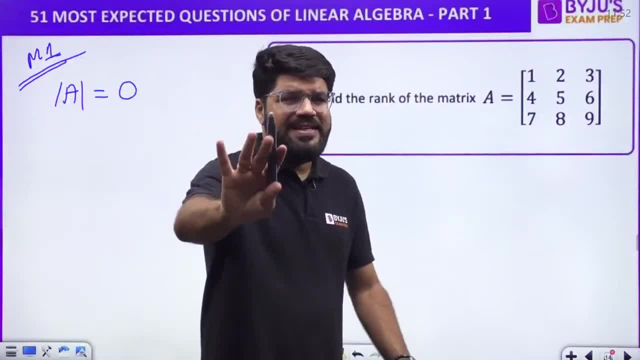 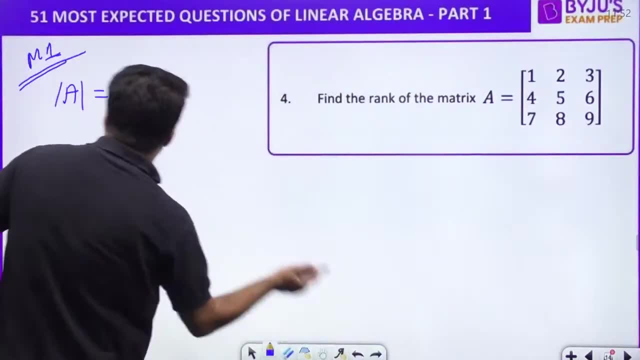 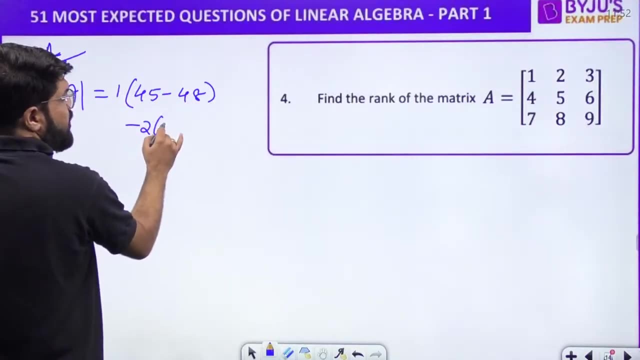 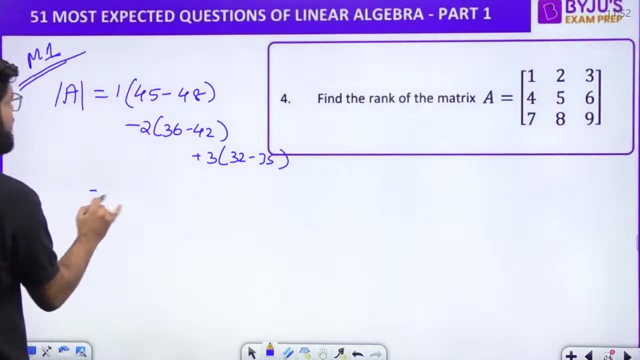 I hope you can complete the calculation. Please try and complete the calculation. Okay, When you calculate the determinant of this matrix, that is going to be 0.. That is going to be 0.. One single step. I will do it up: 1. 5, 9s are 45.. Minus 6, 8s are 48.. Minus 2.. Then you have 36 minus 42. And plus 3 times of 32 minus 35. Right So, minus 3.. Then plus 12. And this is minus 3 minus 9.. Answer is 0. 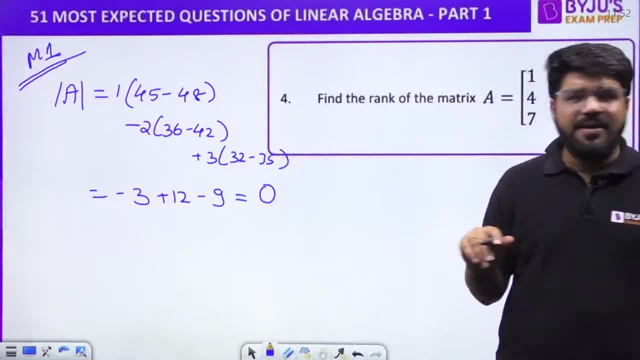 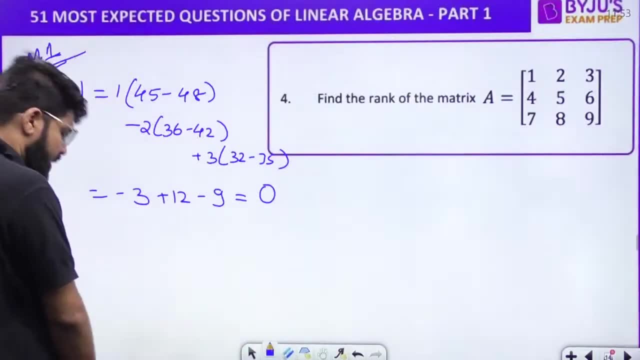 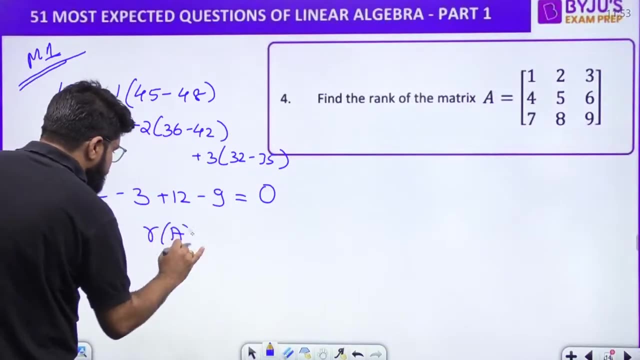 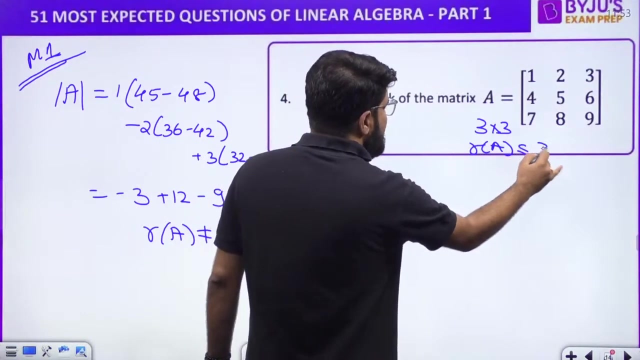 I told you it is going to come up as 0. We are summarizing all the things with this important and another trick to be introduced with this question, Okay, So just please concentrate Right And keep liking the session. So if determinant is 0, rank cannot be 3.. Rank cannot be full. It is a 3 cross 3 matrix. So what is the rank? It is less than equal to 3.. The maximum possible rank is 3.. But here it is not going to be 3.. 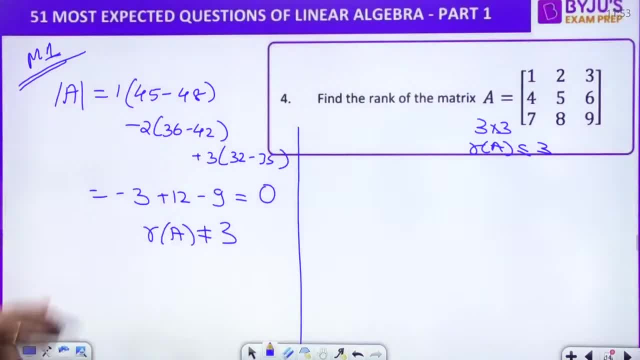 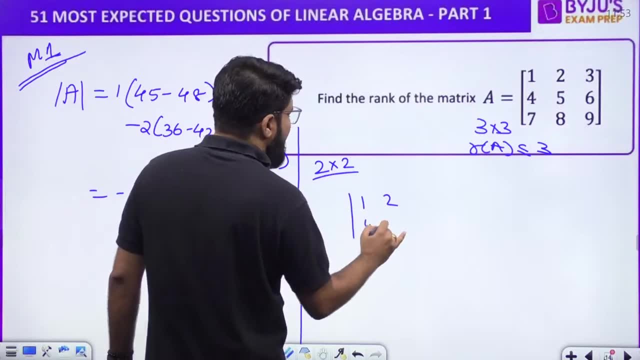 Here it is not going to be 3.. what is going to be the rank? I will check a 2 cross 2 minor. Let us take a 2 cross 2 minor. 1, 2, randomly, random, random. This is a random method. Then we will go to the Eklan method also. 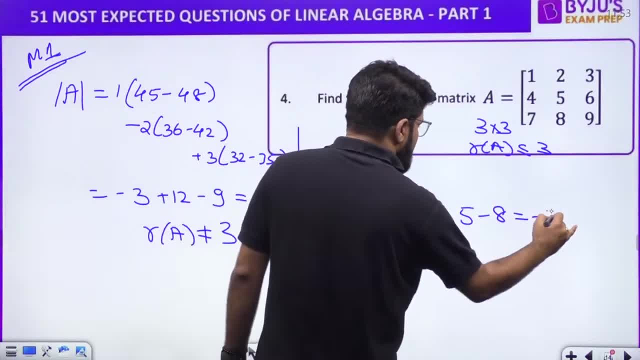 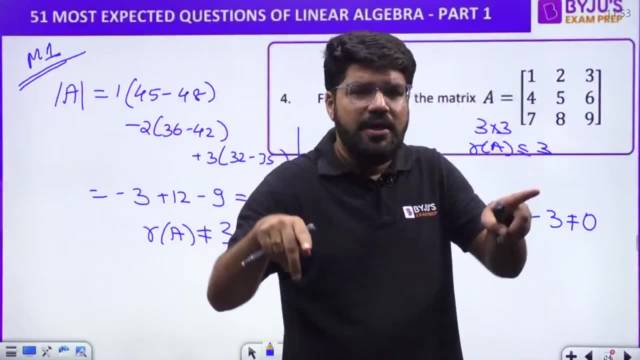 What is the value of this minor? 5, minus 8, minus 3, non-zero, Any 1 non-zero 2 cross 2 minor rank will be 2.. You don't have to check all minors, Even if you have 1 non-zero minor of order 2,. 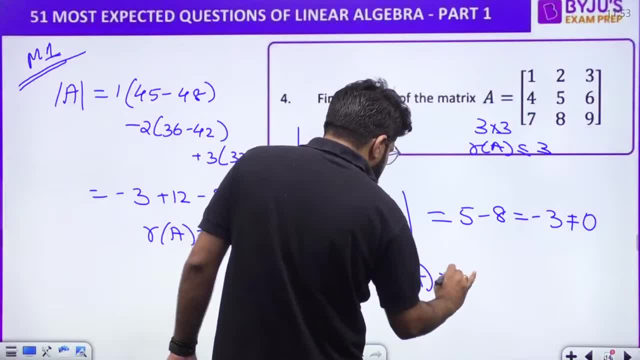 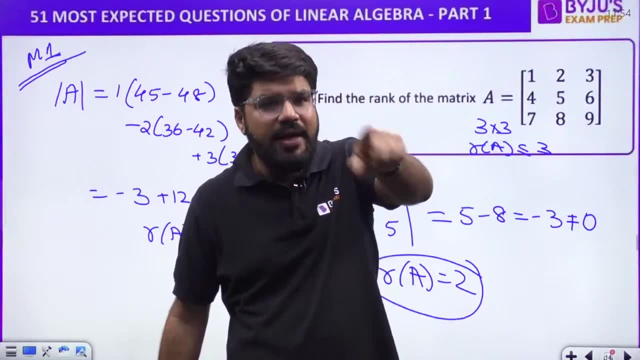 rank will be 2.. Good afternoon, Sehal. So rank is equal to 2.. I conclude: rank is equal to 2.. Even if you have 1 non-zero minor of order 2, rank will be 2.. Rank will be 2.. Rank will be 2.. Yes, 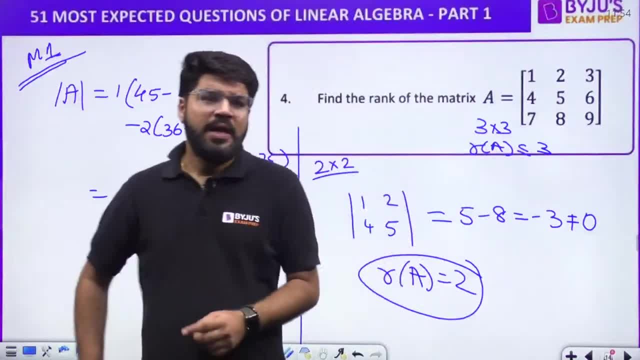 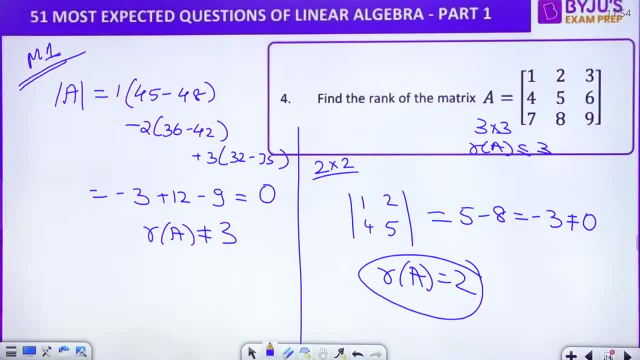 Sagnika, coming to that Indirectly, I am going to come to that. So rank is equal to 2.. Great Rank is equal to 2.. That is sorted to all of us. Next, Now, next method. Let us talk about: 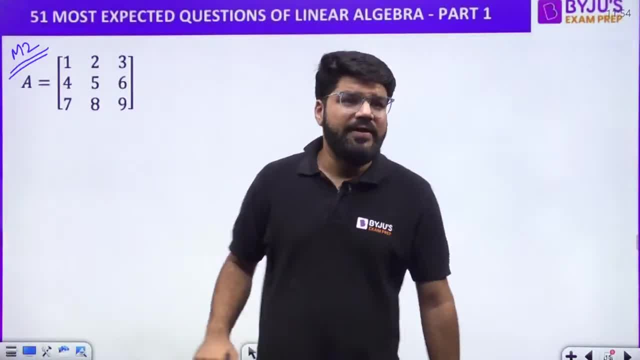 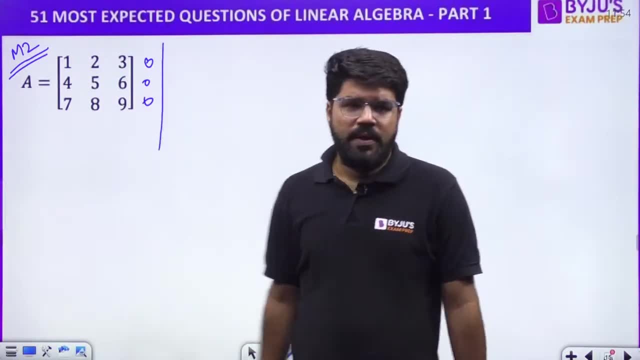 the method number 2, the same Eklan method. Same Eklan method. Very clearly: number of zeros: 0, 0, 0. Number of starting zeros: M. number of starting zero: it is same. So this is not in the Eklan form. I will quickly apply. 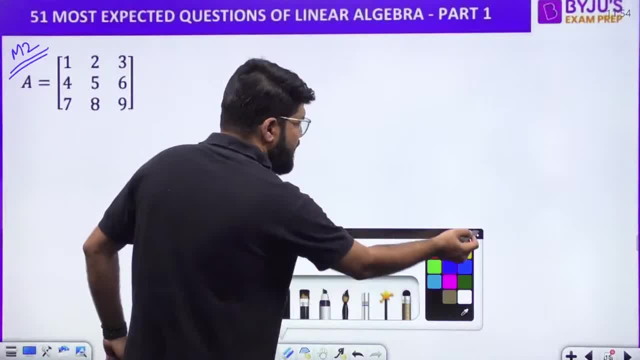 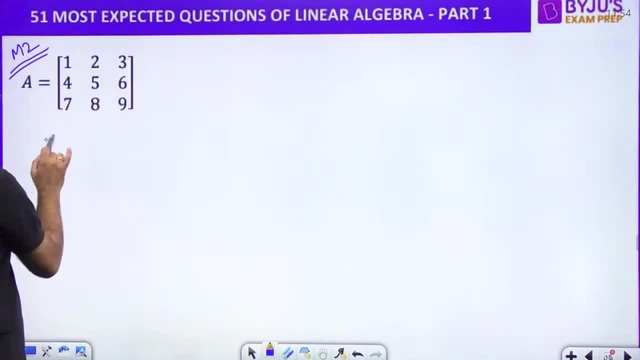 the elementary transformation. Okay, Then we will come to the shortcut. Story will be over by that shortcut. So what is going to be the result here? What is going to be the result here? I will apply the elementary transformation. R4 is equal to R4 minus 4R1.. First we will do this as 0. And then 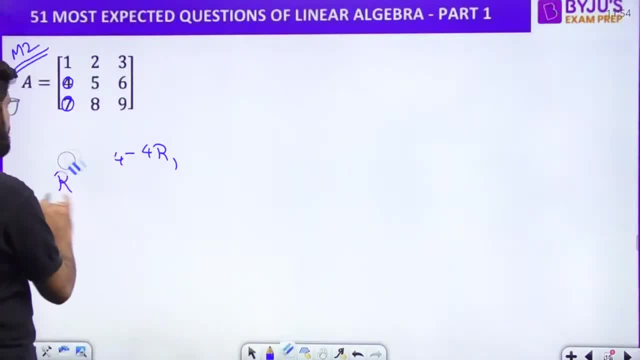 we will do this as 0.. Sorry, why R4?? Sorry, that is R2.. I am so sorry for that. That was R2.. Row number 2 is R2 minus 4R1.. And similarly, 7 has to be 0. So R3 has to be R3 minus 7R1.. Let us follow this much And after. 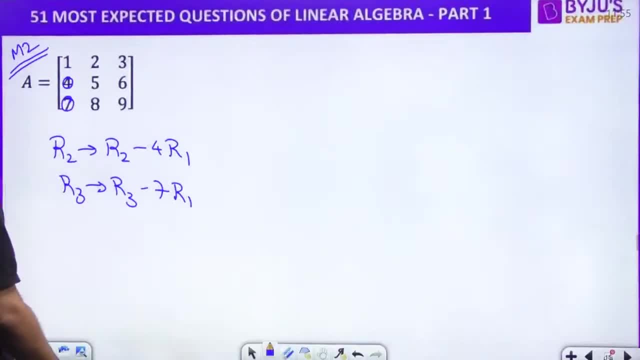 completing, after completing this much the matrix, the elementary operations 4 minus 4, 0.. 5 minus 2 into 8 minus 3.. This is minus 6.. Next, 7 times 7 minus 7, 0.. 8 minus 14, minus 6.. 9 minus 21, minus 12.. Okay. 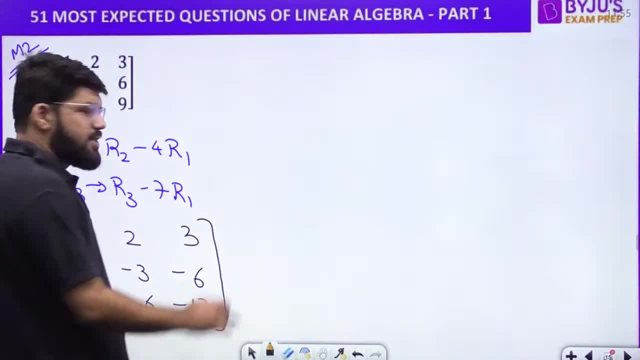 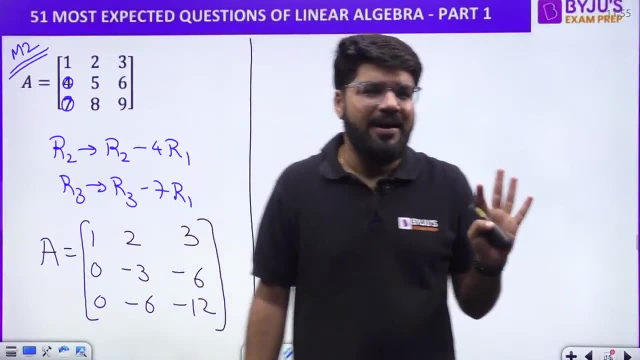 Now very clearly, the second and third row are identical. Okay, Second and third row will be identical. Yeah, For some of the questions, Eklan will be lengthy. That is why I am going to come up to the shortcut method. Just wait, We are going to come to the shortcut. Yes, I also agree For. 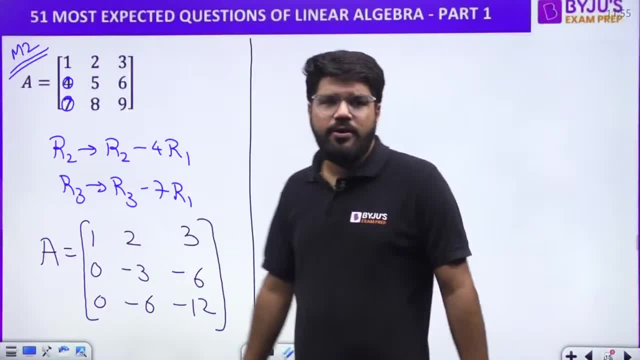 some of the questions like this, Eklan, can be lengthy. That is why we are going to come up to the shortcut method. We need to reduce it. Determinant method is simple. This is the very random method that you can apply. Finally, I come to the shortcut. Okay, Now, what you are. 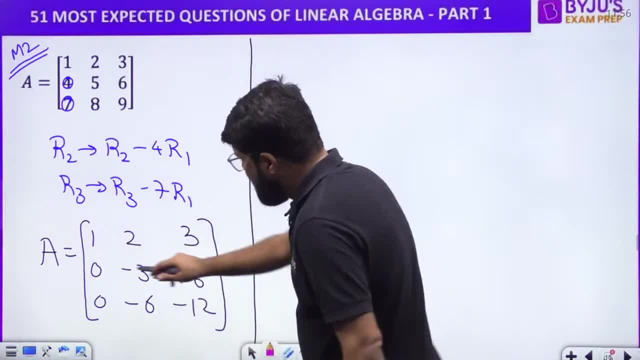 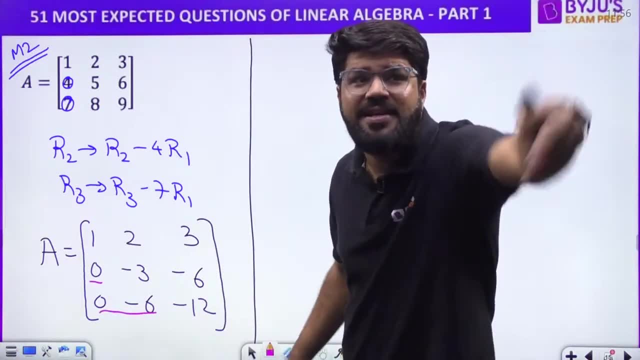 supposed to do here Now, the next step that you can do is: okay, this is already 0. So 0, then one single 0.. I want two 0s. I want the number of 0s in the increasing manner, No Increasing. 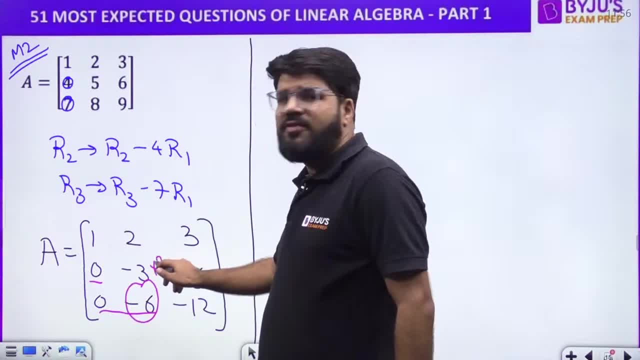 manner. So I have to make this as 0.. So what will we do? Multiply above number by 2. They become equal and then subtract. So what is the operation there? What is the operation there? R3 can be. 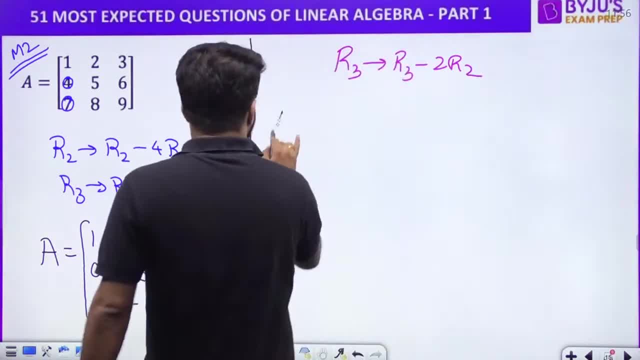 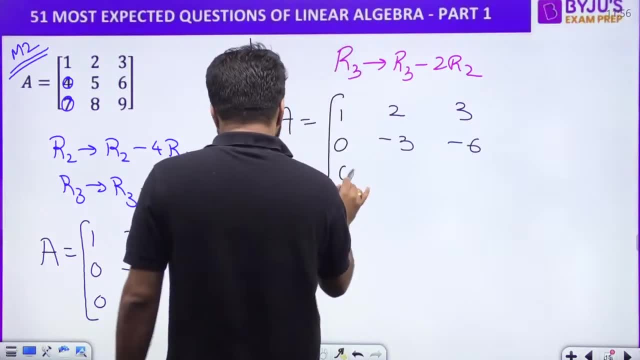 minus 2 or 2.. R3 minus 2 or 2.. So that my matrix becomes 1 and 2 and 3.. 0 and minus 3 and a minus 6.. 0 and then 0.. Minus 12, and this is also becoming minus 12 after multiplied by 2.. This is 0.. Now 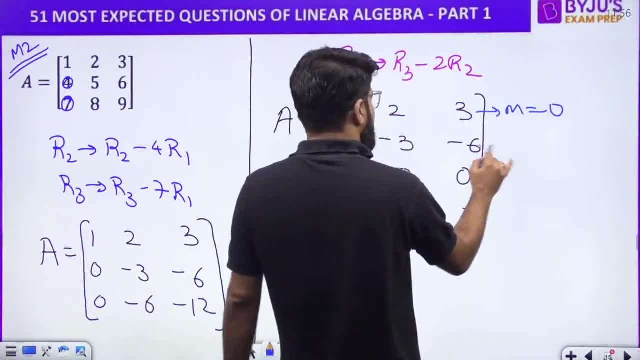 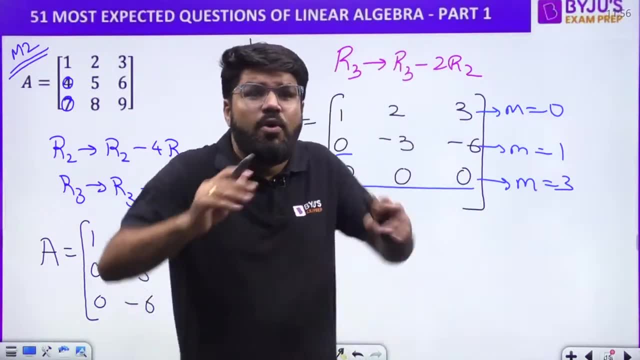 have a count of the number of 0s, Sir. number of 0s: nil. Number of 0s: 1. Number of 0s: 3. It directly becomes 3.. But it is increasing. I only want increasing. It is increasing. Yes, We all can. 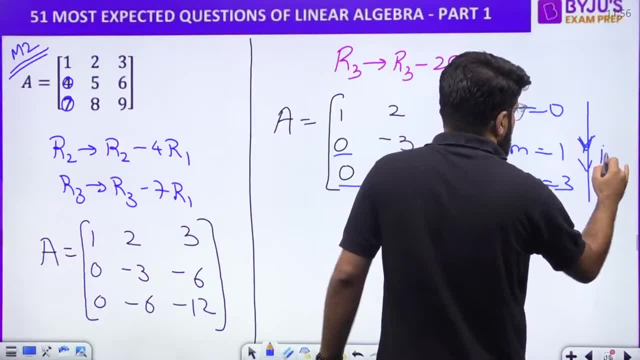 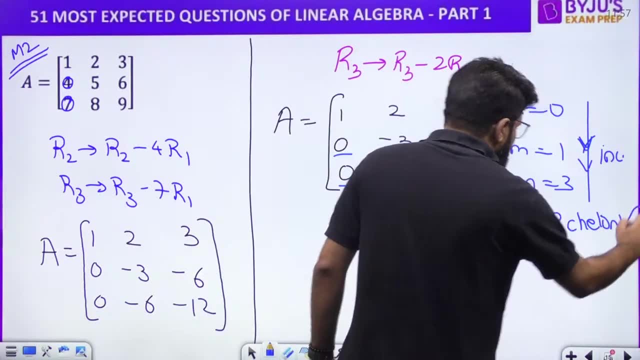 agree that it is increasing, So this is already the echelon form. There is a row of 0 also. That is at the last Row of 0, at the last. So it is the echelon form and whenever a matrix is in the 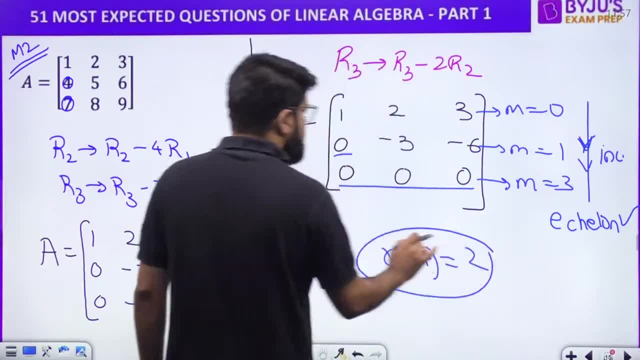 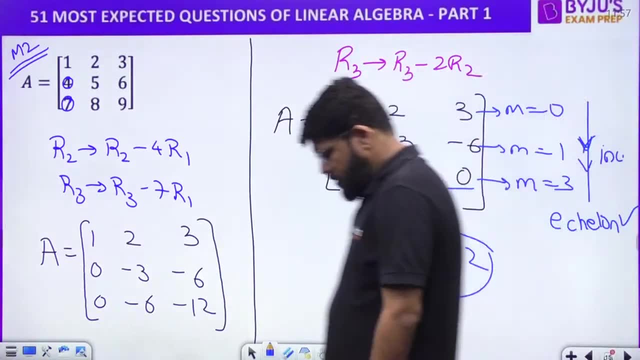 echelon form. rank of the matrix is number of non-0 rows. These are the two non-0 rows. Third one is 0.. These are the two non-0 rows. Third one is 0.. Third one is equal to 0.. 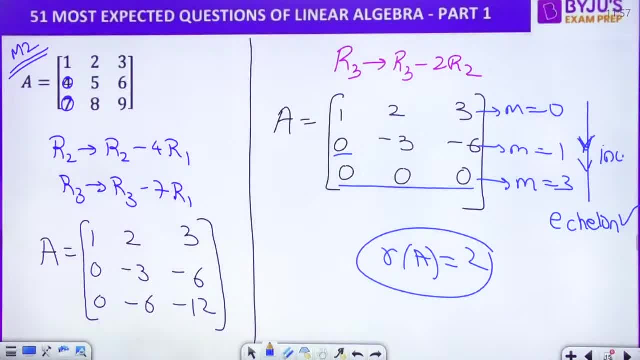 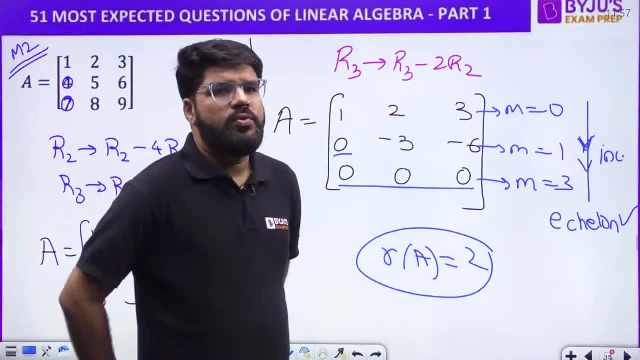 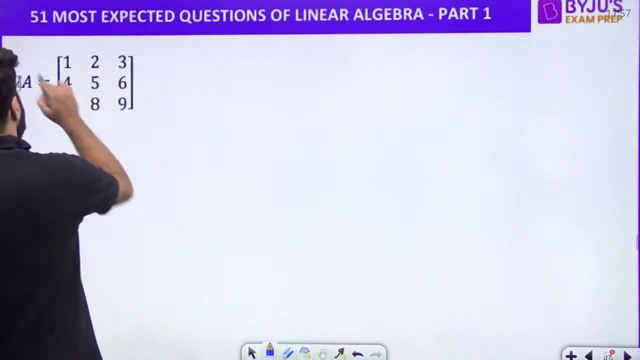 Third one is 0. Rank is equal to 2.. Same thing we got: Rank is equal to 2.. Now let us talk about the shortcut. Let us talk about the shortcut Method number 3.. Let us talk about the shortcut. 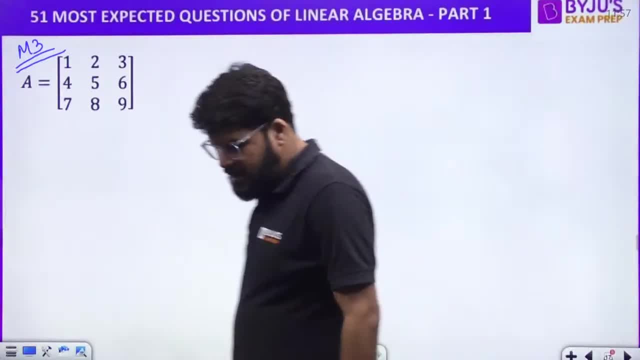 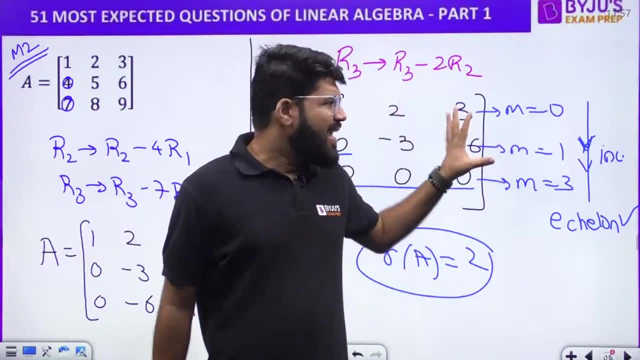 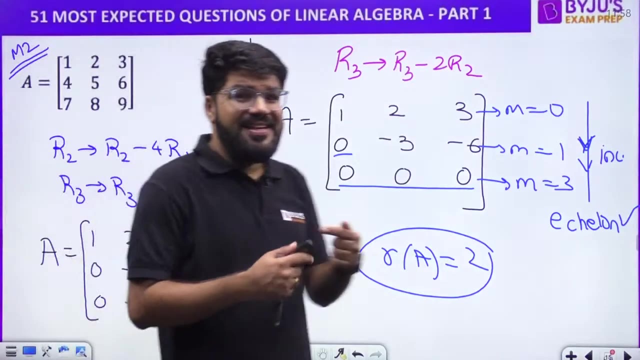 now guys, Please pay attention. now I understand that for some of the methods, for some of the questions, Yeah, Minor one was fast Echelon is good for some of the matrix, But in general this is lengthy, Take care. So what is the best thing? Okay, That needs little bit of logic, But if your logic is, 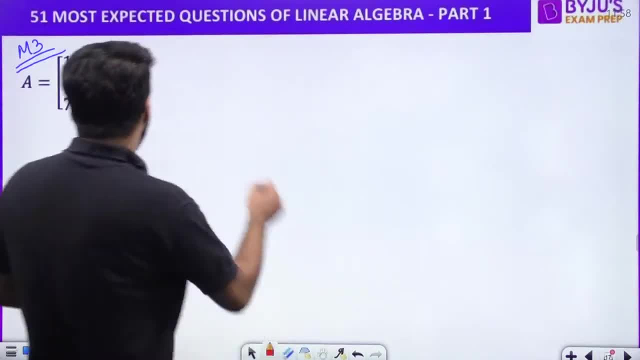 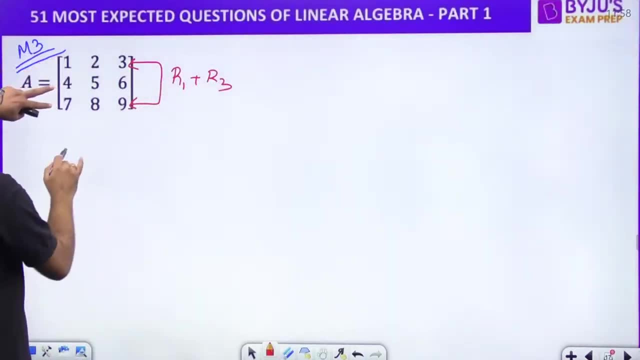 strong. the third method I am going to tell you, Going to solve the questions in seconds. Let us add. Let us add R1 and R3.. Okay, So what is 1 plus 7? 8.. 2 plus 8? 10.. 3 plus 9? 12.. 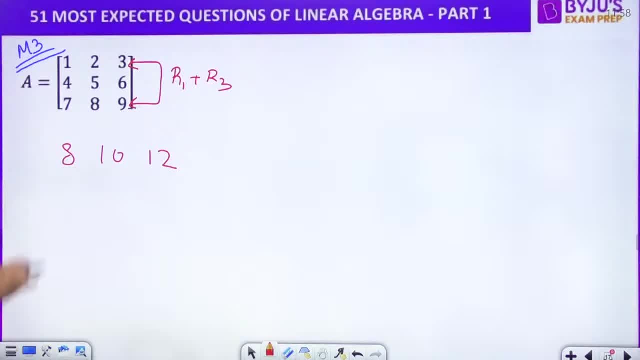 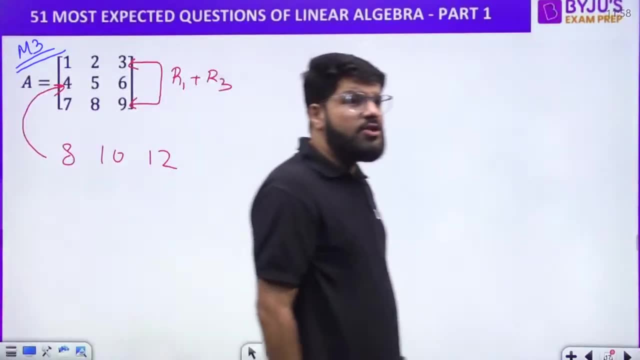 And look at the relation with the R2.. Look at the relation with the R2.. It is twice 4. twos are 5, twos are 6. twos are So dear. I can say that whenever I add R3 and R1,. 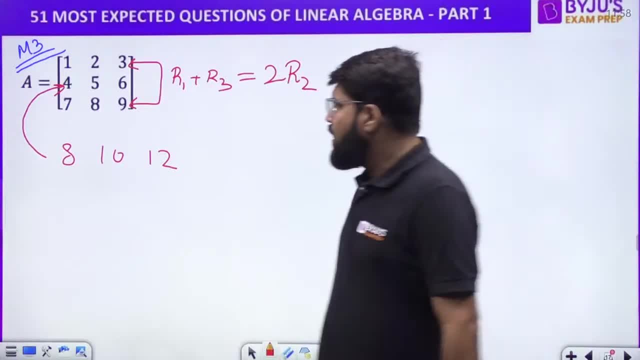 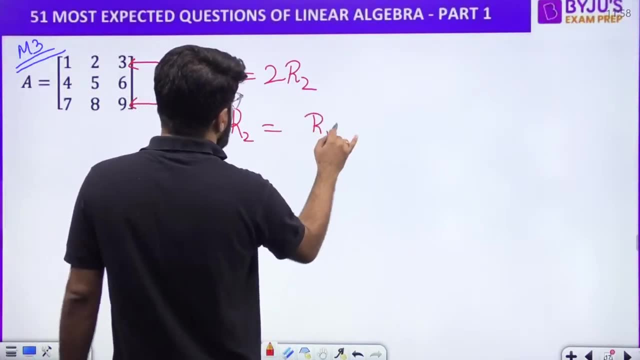 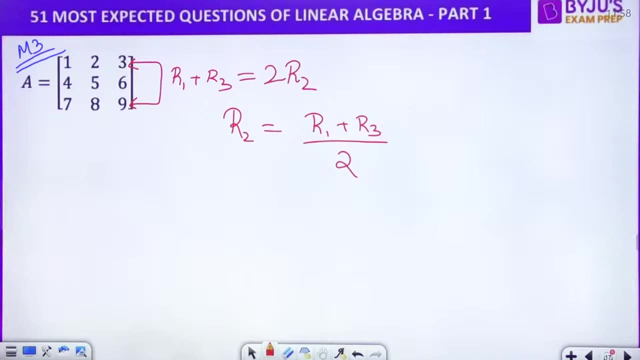 I get 2 R2.. Dependency: I get 2 R2.. I get 2 R2.. Or I can say that R2 is equal to R1 plus R3 is divided by 2.. R1 plus R3 is divided by the 2.. 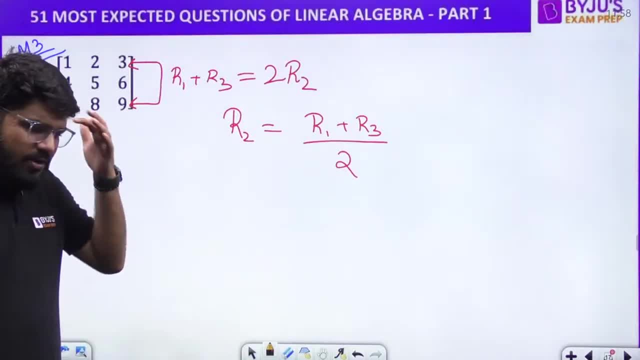 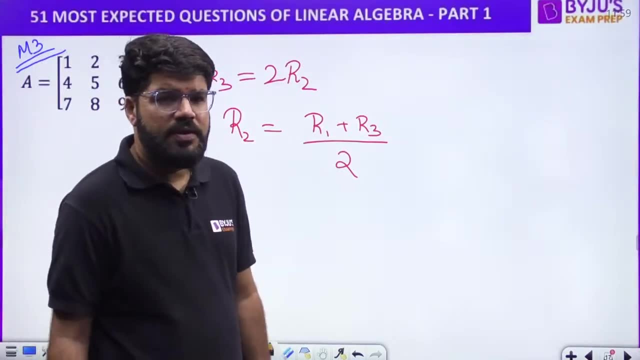 R1 plus R3 is divided by the 2. R2 is equal to the R1 plus R3 divided by 2.. Right everybody, Right everybody. If M is equal to 2 in last row, No, no, no, Then also it is. 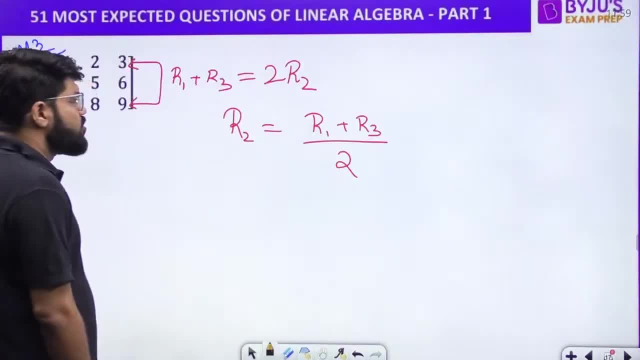 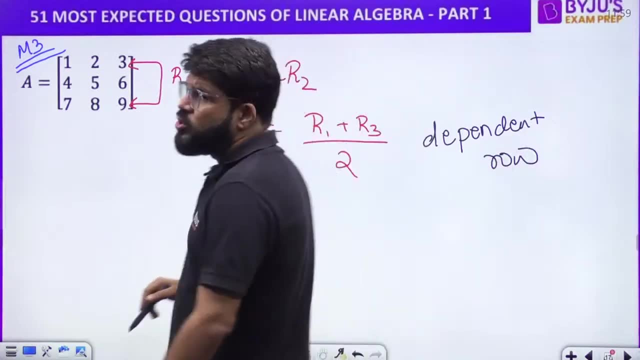 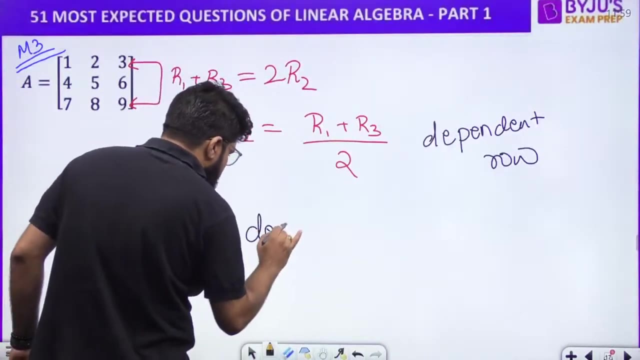 increasing. Okay, So there is a dependency. So out of the 3 rows of the matrix dear, 1 is dependent, Right? So you have 1 dependent row. So how many 2 independent rows? 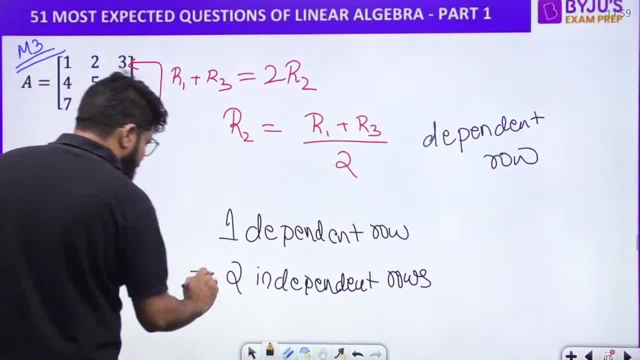 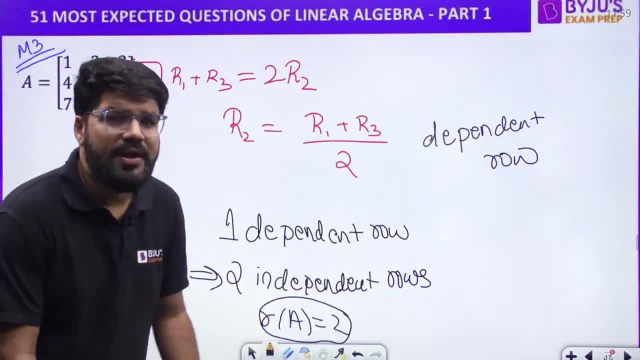 If you have 1 dependent rows, remaining 2 are independent rows and rank is equal to number of independent rows or independent columns. You can either check by rows or you can either check by column. That is one of the point I have mentioned in the beginning. Okay, I told you very, very. important point: You can either check by rows or you can either check by column. So you can either check by rows or you can either check by column. So you can either check by rows, or you can either check by rows or you can either check by column. Now let me highlight this: This is a very, very 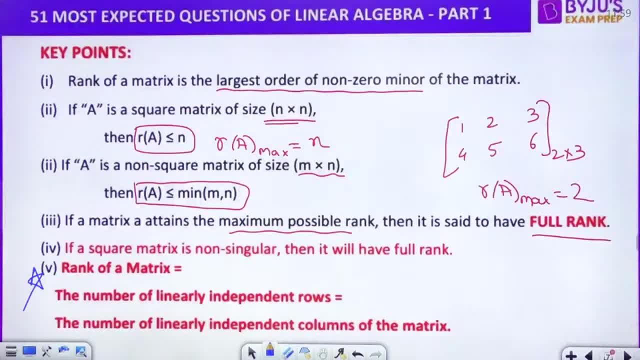 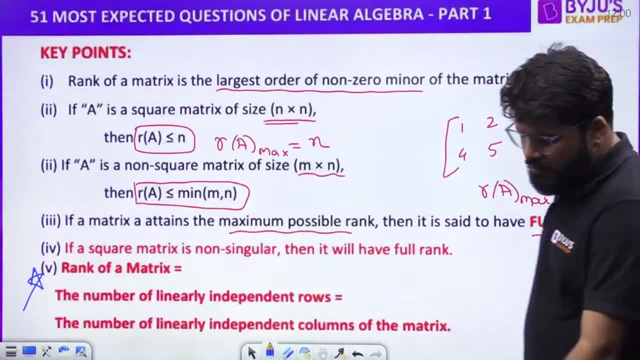 important point for many of the questions. Rank of a matrix is always equal to number of linearly independent rows or equal to number of linearly independent columns. Number of linearly independent rows or equal to the number of linearly independent columns. Right dear. 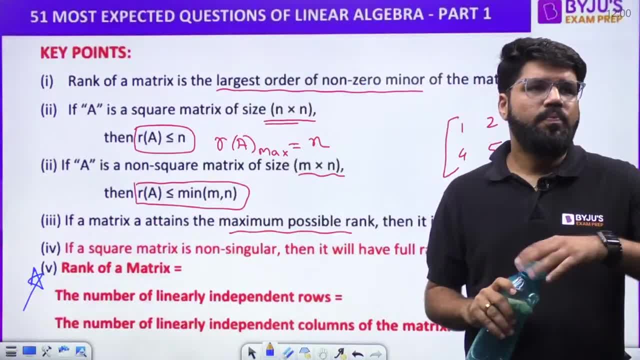 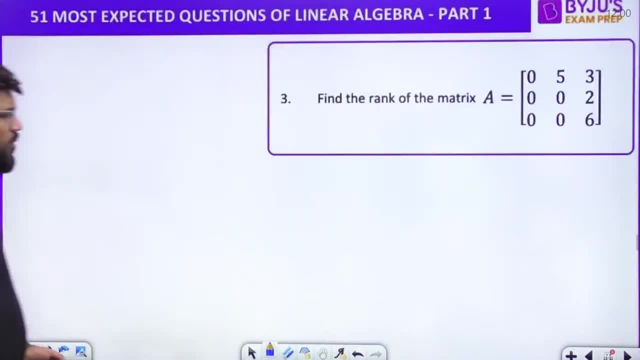 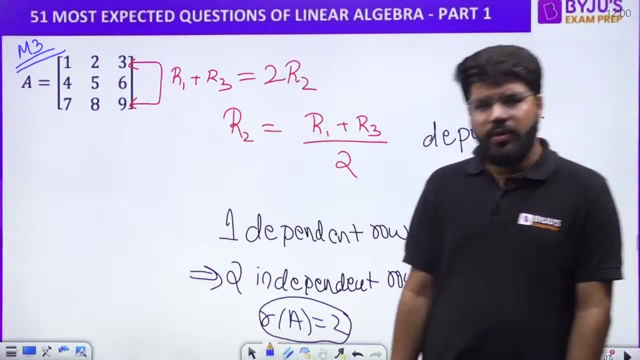 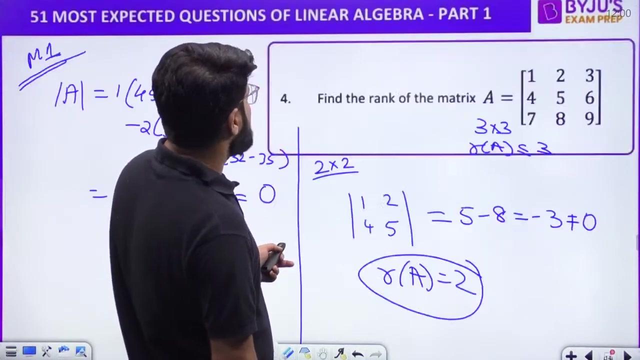 so that is what it is, and hence the rank is equal to 2 by the direct dependency we are able to see here. okay, good morning, chin may. okay, let's, let's figure out more questions. okay, what is the rank of this matrix? what is this? is fifth one only correct? what is the rank of this? 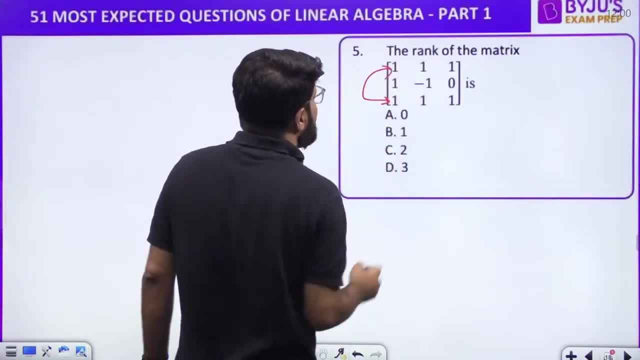 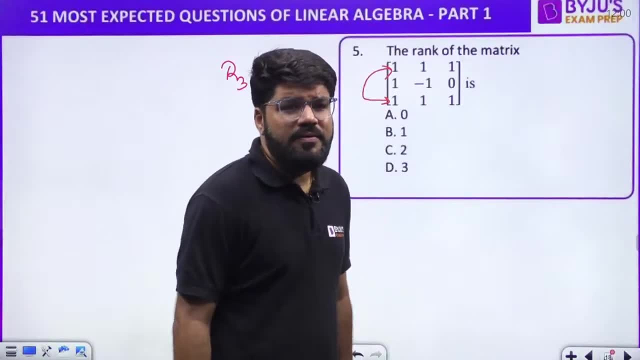 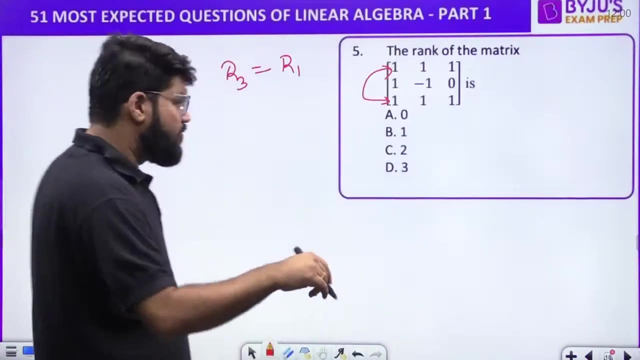 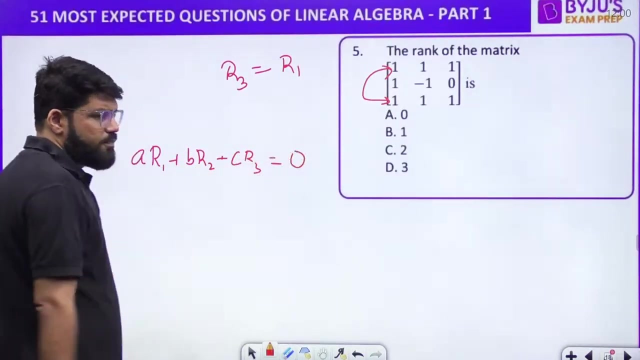 matrix, the two rows are given identical. r3 is same as r1, so r3 depends on r1, r3 depends on r1. no, no, no, no, no, no. only linear dependency. right, our linear dependency is of the form: manjeet: ar1 plus br2 plus cr3 equal to 0. okay, y equal to mx, y equal to mx plus cb. 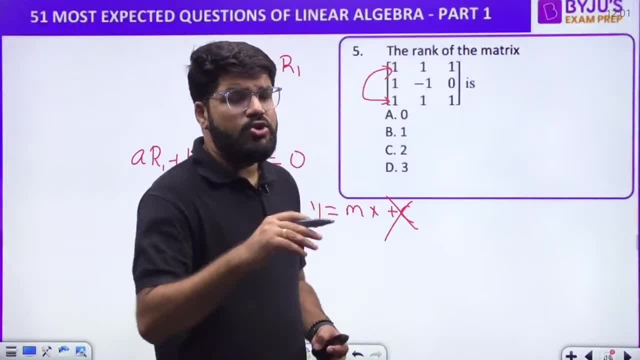 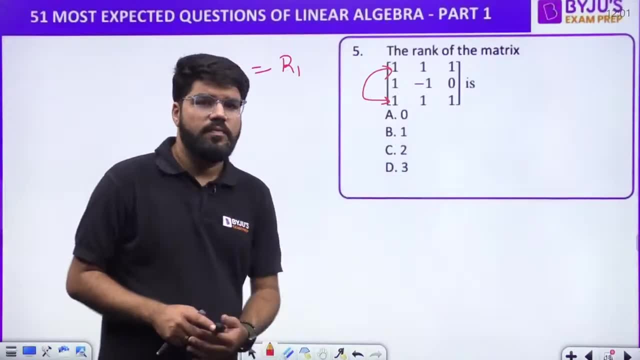 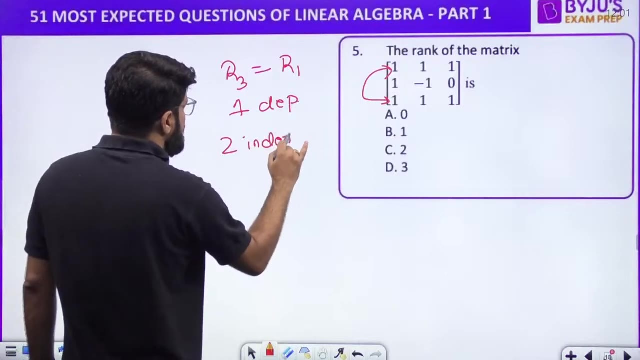 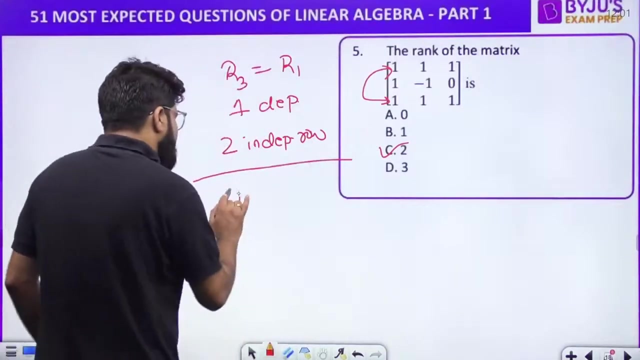 right. so there has there cannot be any constant. the rows should be dependent through their own numbers. okay, okay, chalo. so this is one dependency. so how many independent rows? two independent rows. you can either go by the determinant method, also right, or whatever clicks quickly, or determinant they go. two rows are same, determinant will be zero. 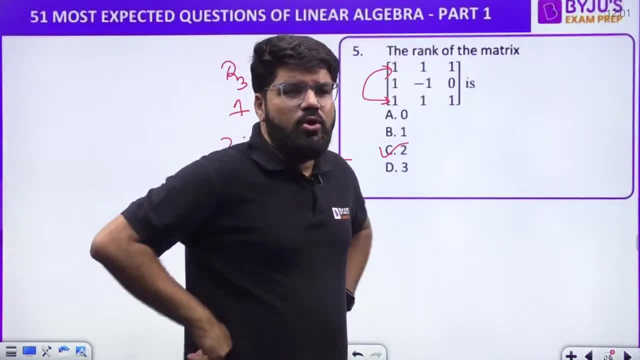 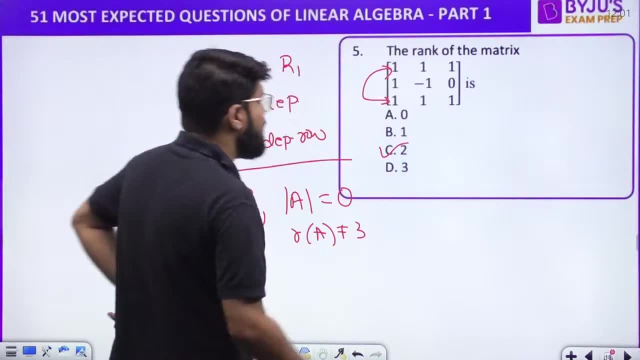 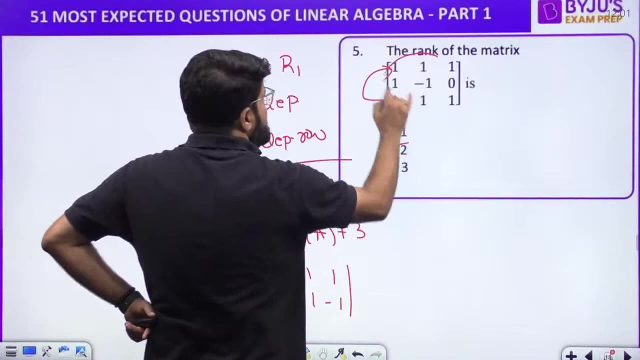 whenever two rows are same determinant property, two rows are same determinant zero. okay, determinant zero. the rank cannot be three. rank cannot be full. rank cannot be full. what about two cross two rank? what about a second rank? so one one, one minus one. i have randomly checked this: two cross two minor right and this: 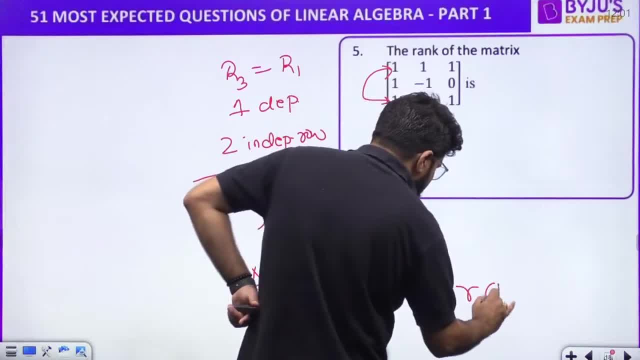 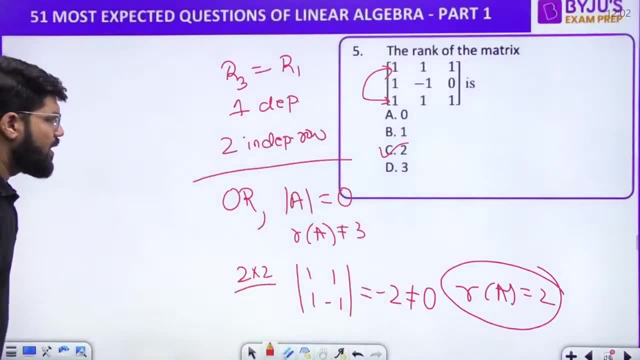 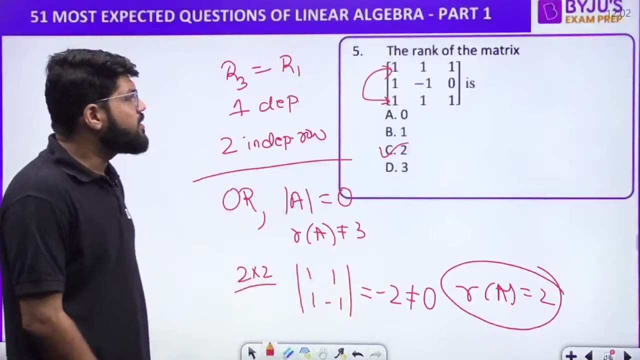 is minus one minus one, minus two, not equal to zero, right, not equal to zero. to rank: two cross two minor is non-zero. the rank has to be two. dear rank has to be two. answer is two. everybody answer is going to be two. all clear, chalo, very good. next question: find the rank of this. 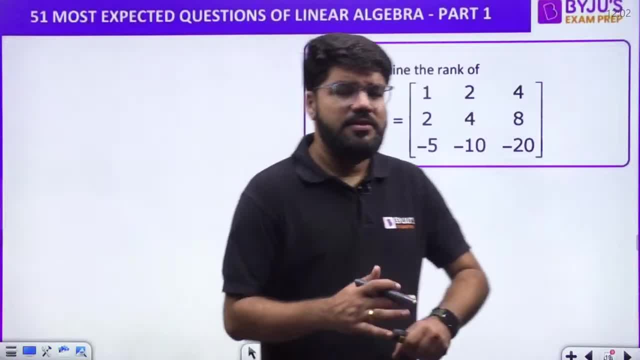 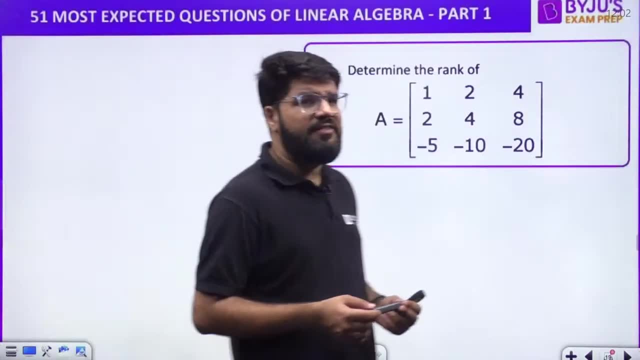 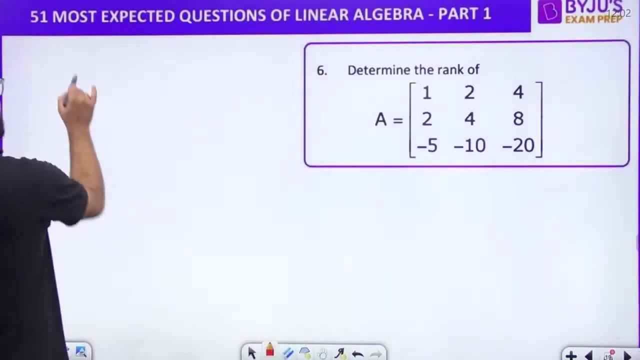 matrix. find the rank of the given matrix. question number six for you. find the rank of the given matrix: one, two, four, two, four, eight minus five minus ten minus twenty. right? one, two, four, two, four, eight minus five minus ten minus twenty. okay, chalo bahat badiya right. so what is going to be? 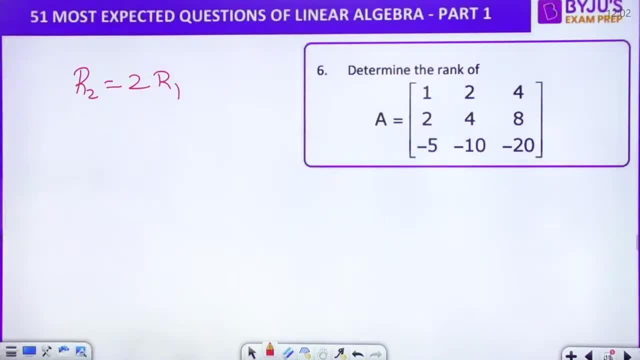 the r two. r two is going to be two r one. r two is going to be two r one, right, one into two, two into two, four into two. okay, what is going to be r three, r three? we taking in a one into minus five, two into minus five, four into minus five, right, so this is minus five r two. minus five r one, sorry. 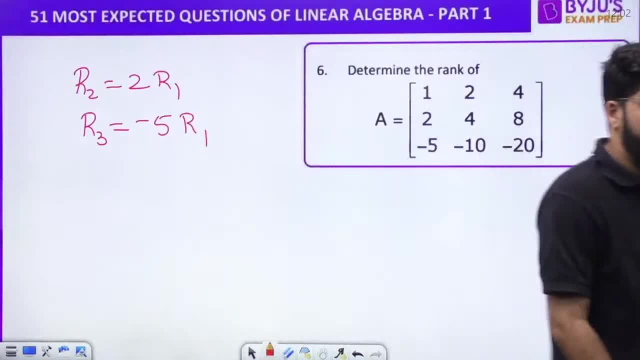 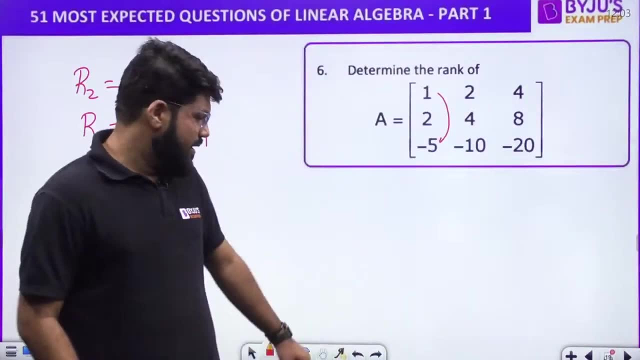 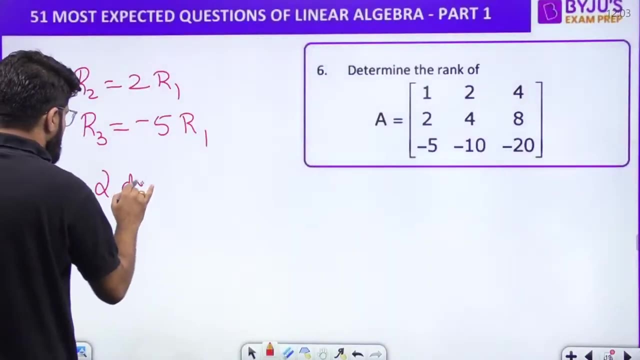 so what is the r three minus five, r one, isn't it? what is going to be r three minus five, r one minus five, minus five minus five. so so, how many rows are dependent, dear, two dependencies are there. two dependencies are there, right? so you have two dependent rows. there are two dependent rows, so there is only one. 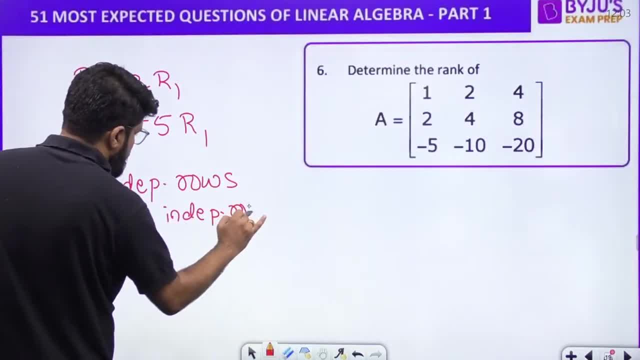 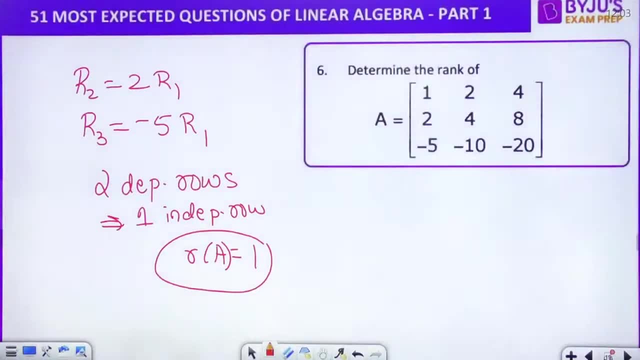 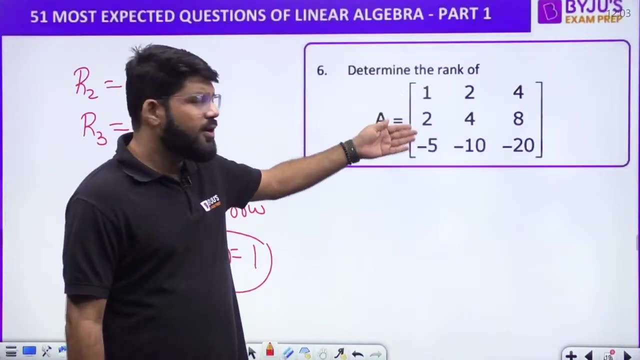 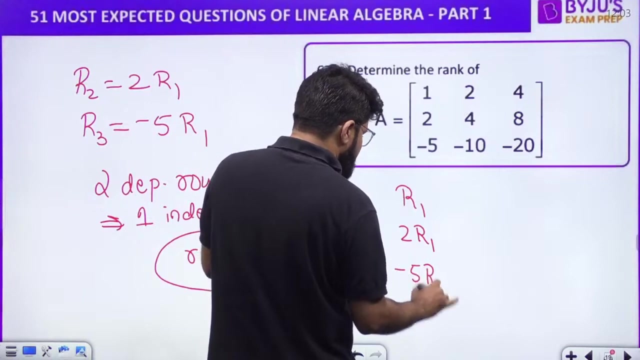 independent row. so rank of the matrix is equal to one. rank of the matrix is equal to one. so always note that now, in a sense, in a sense, all the rows are proportional to each other. this is a case when you have row one, then you have two r one, and then you have minus five r one. this is how the structure. 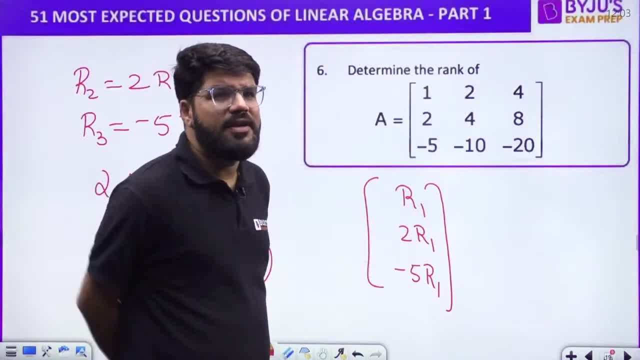 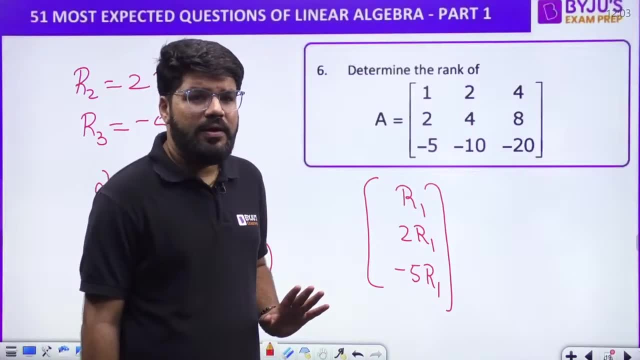 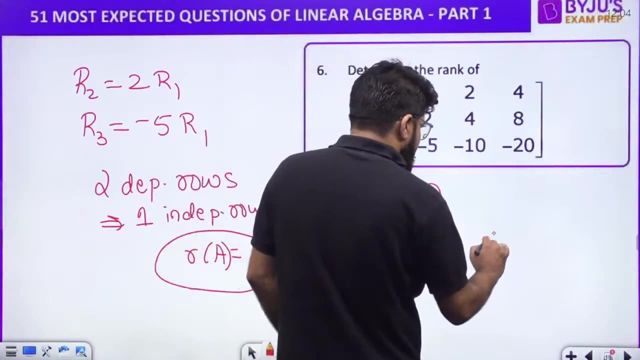 is actually, as a structure, one r one, two r one minus five r one right. that means: how many unique row is there? only one unique row, only one independent row. rank is equal to one. i can say that all the rows are proportional to r one, two r one minus five r one. all the rows are right, alpha. 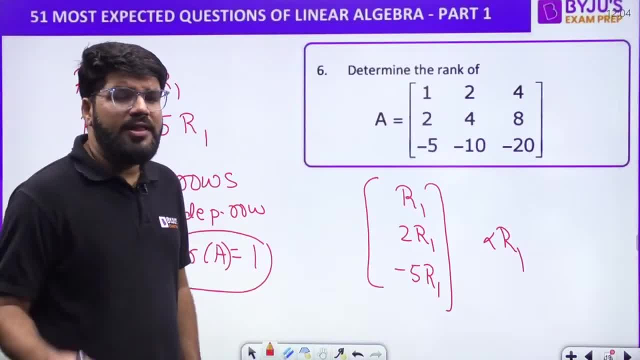 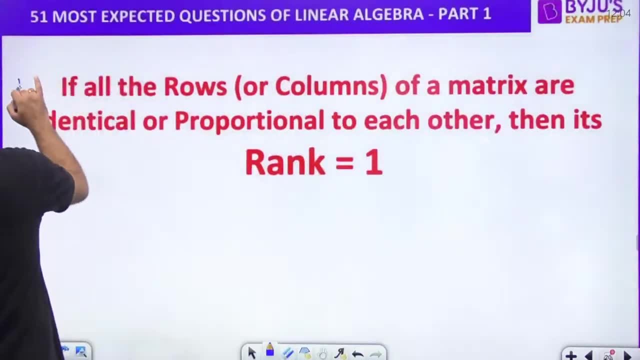 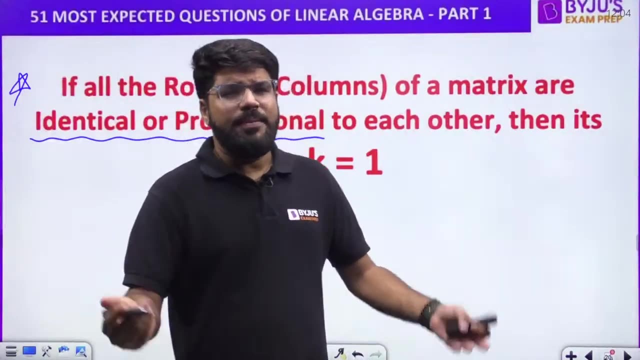 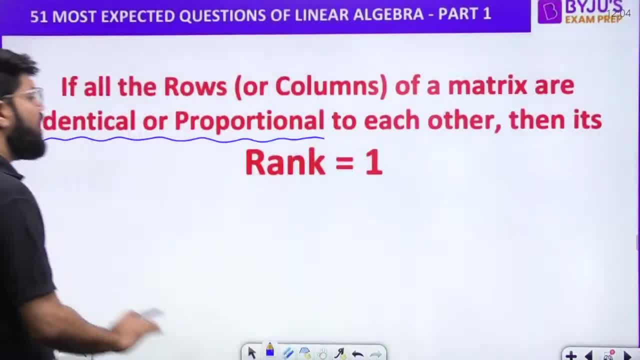 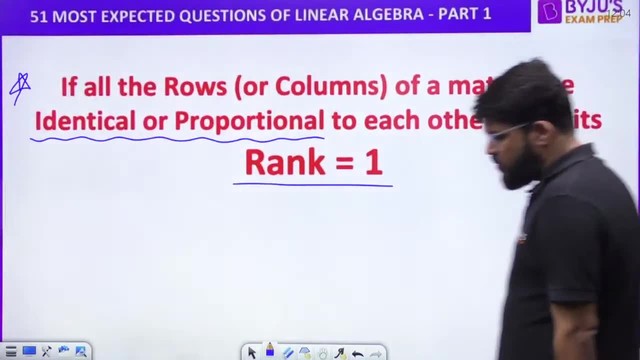 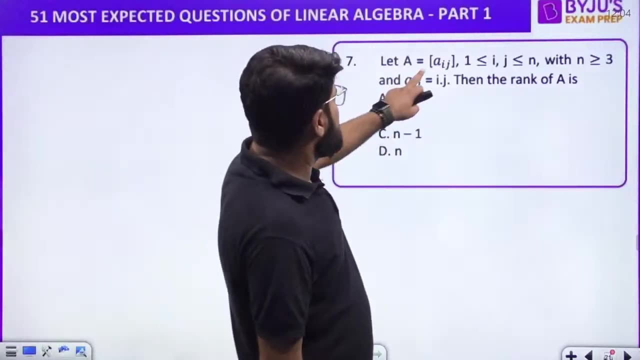 r one alpha can be one for all of the rows. okay, then, in all such case, rank of the matrix is equal to one. in all such case, rank of the matrix is equal to one. in all such case, rank of the matrix is equal to one. seventh question: let a is equal to a, i j. okay, so i and j are belonging to one, to n. 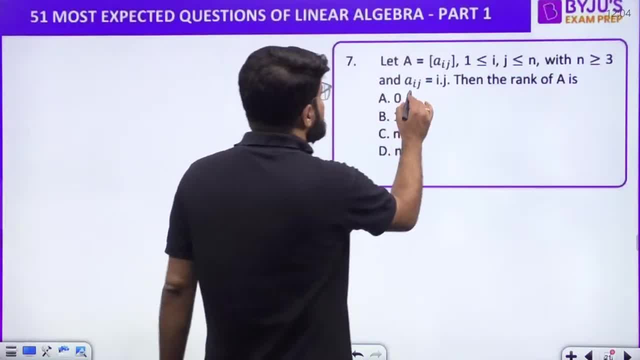 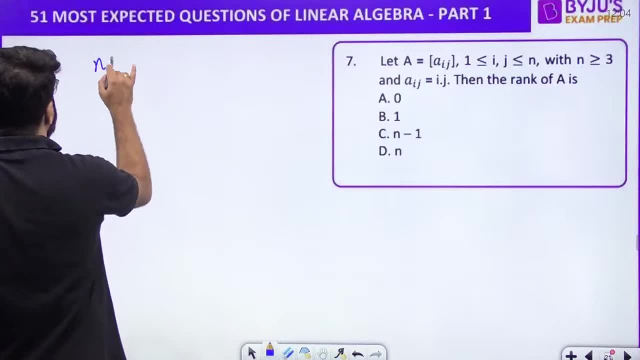 and n is greater than equal to three. a, i, j is i into j. that is the relation given. what is the rank of a? n can be any number greater than equal to three. now let us try with n equal to three. let us try this with the. n is equal to three. 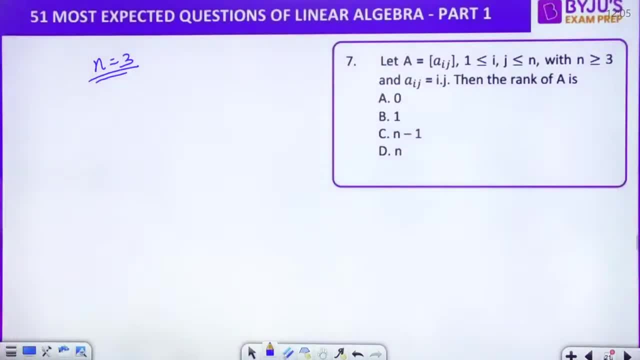 let us try this rapidly with the n equal to three. let us try this rapidly with the n equal to 3, and please pay attention here: n equal to 3, what should be the rank of the matrix? what should be the rank of the matrix? so for n. 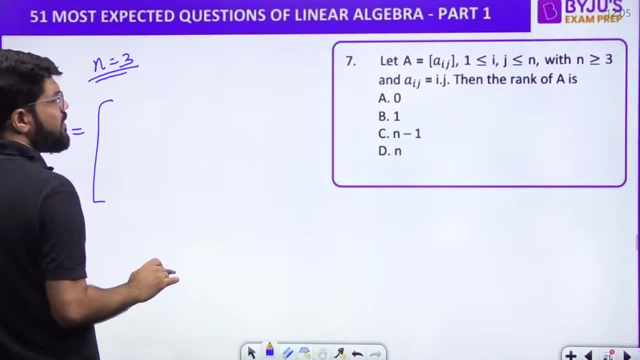 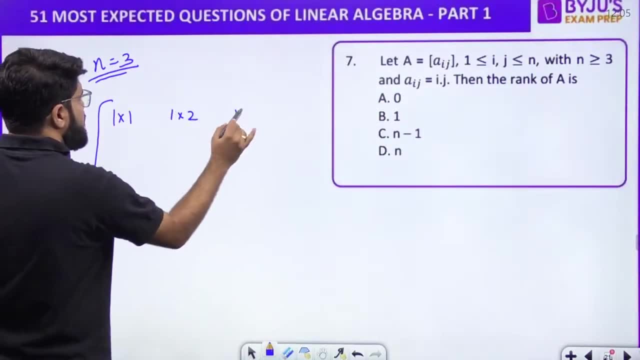 equal to 3. what is the matrix? it's a 3 cross 3 matrix. now all the elements: a, i, j is i into j. this is a 1, 1. this is 1 into 1, right, this is a 1, 2. this is a 1, 3. this is a 2. 1 a 2, 2 a 2, 3. then we: 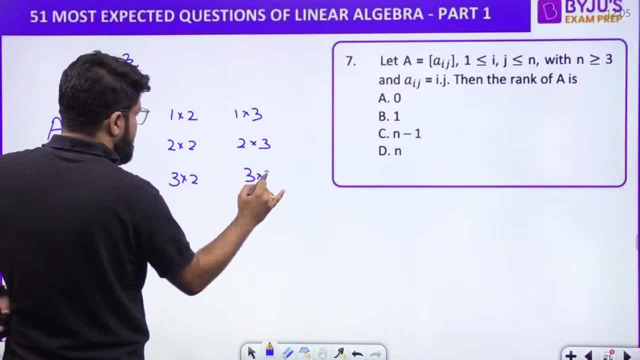 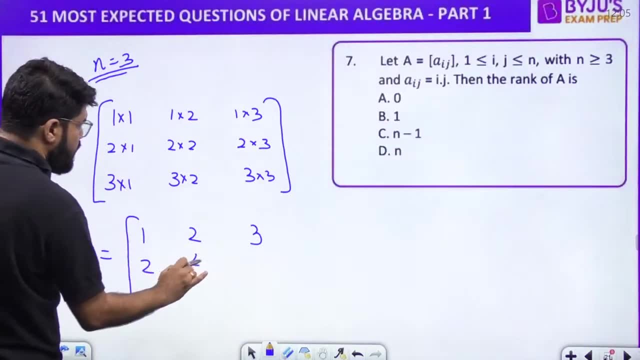 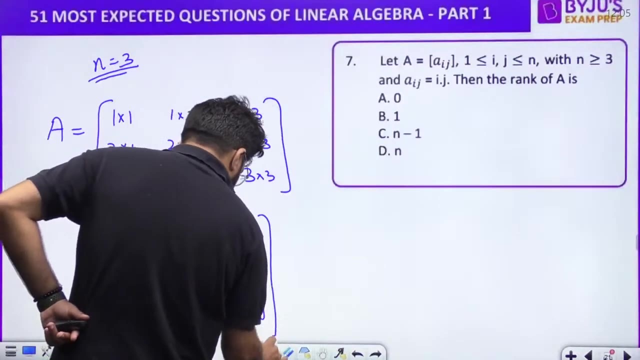 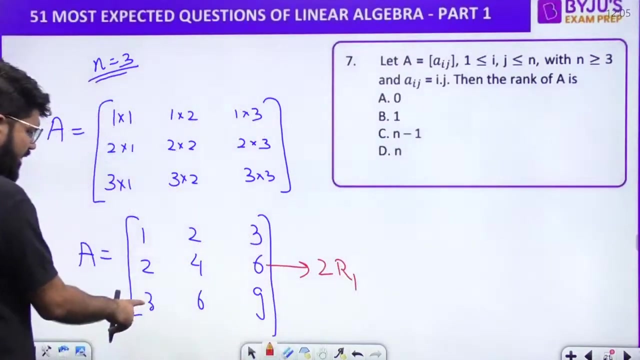 have a 3, 1 a, 3, 2 a, 3, 3, right? if I simplify this, the matrix a actually becomes 1, 2, 3, 2, 4, 6, 3, 6, 9, 3, 6, 9, right? so how much this is into 2, right, this is 2 r 1. how much is the last one, 3 times 1, into? 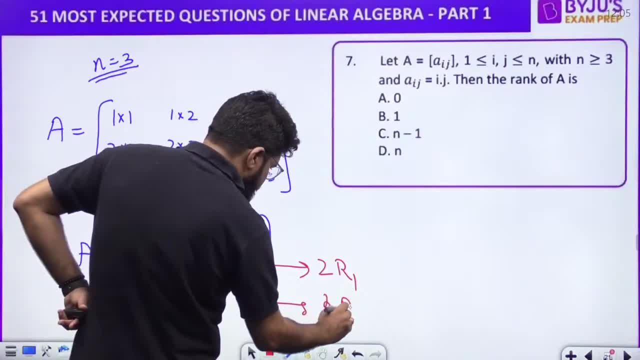 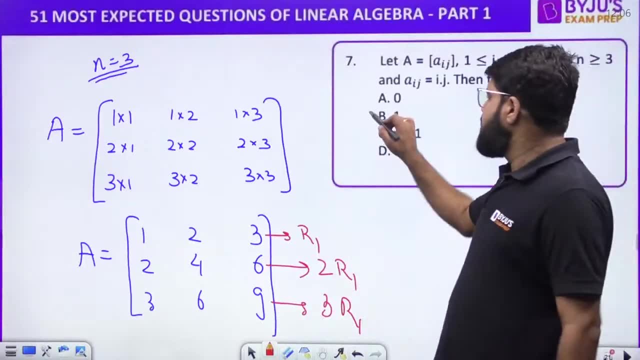 3. 2 into 3, 3 into 3. this is 3 r, 1 right. all the rows are proportional to each other. all the rows are proportional to each other, so rank is equal to 1. only one independent row. all rows are proportional. 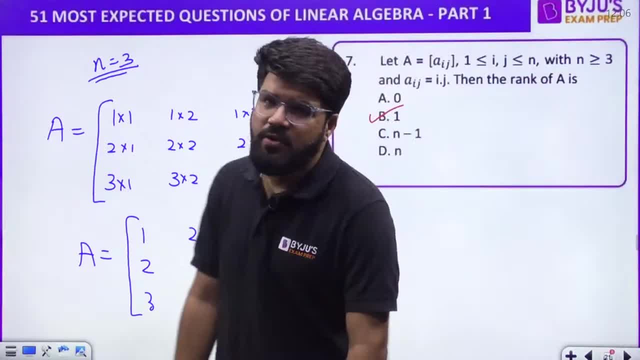 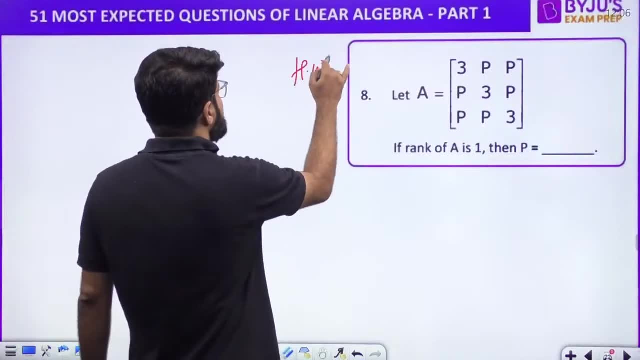 r 1, 2 r 1, 3, r 1. all the rows are in the form of alpha r 1 and all such cases rank will be 1. all such cases, rank will be 1. an entity type question has a homework because it is on the. 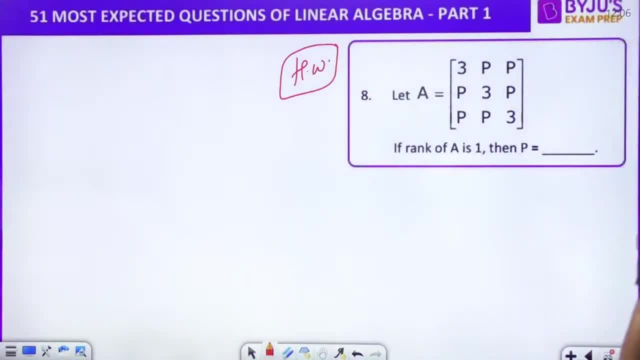 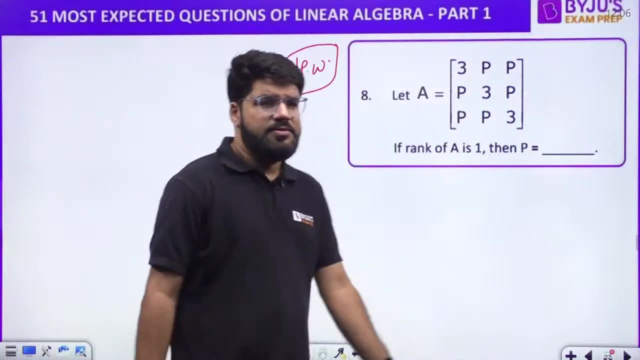 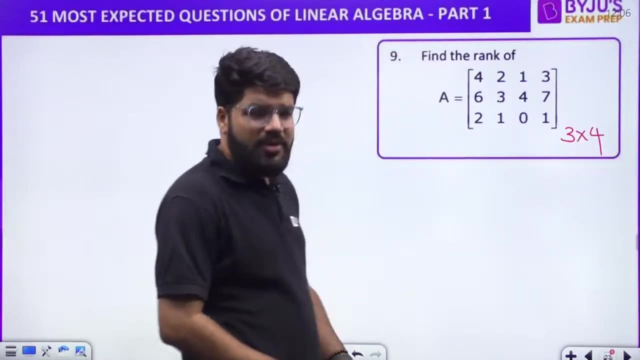 similar concept. one or two homeworks also. I'll keep adding: okay, this one is a homework for you, right? this one is a homework for you. next question, let's move ahead to the next question here. find a rank of the matrix. it's a 3 cross, 4 matrix, non square matrix. think about. 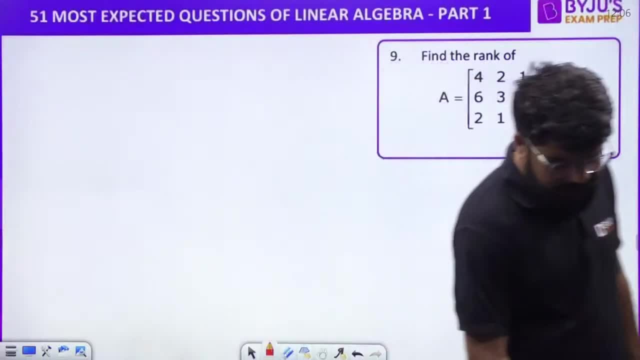 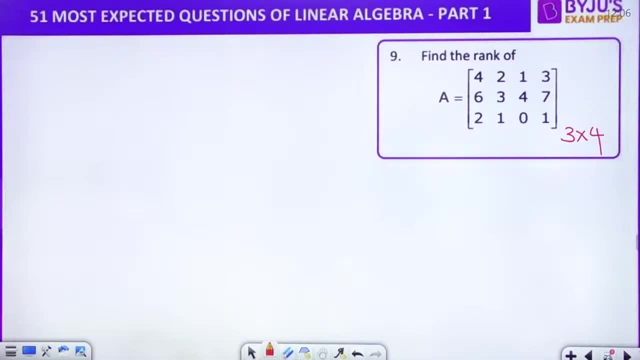 this and get me the rank. and by the time, let me just take the charger as well, just a minute and see if it fits the question. okay, let's ask the same question here on the right. we are gonna take r 1 of r and all these r 1's and the r 1's are in a row. so how many rows? 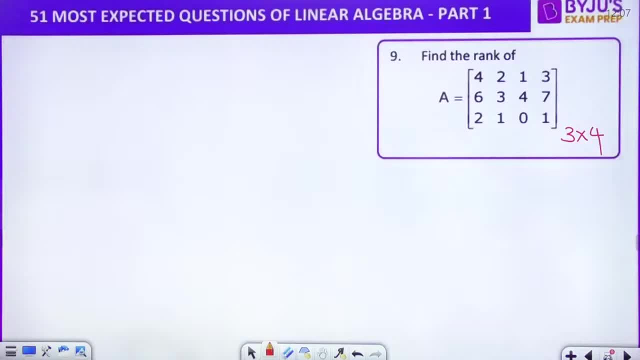 does it fit to the random matrix? all right, so for r 1 and r 2, all rows are proportional to each other in 2 rows, and that's the argument for the rank. you have a row, r 1, r 2, r 1 and. 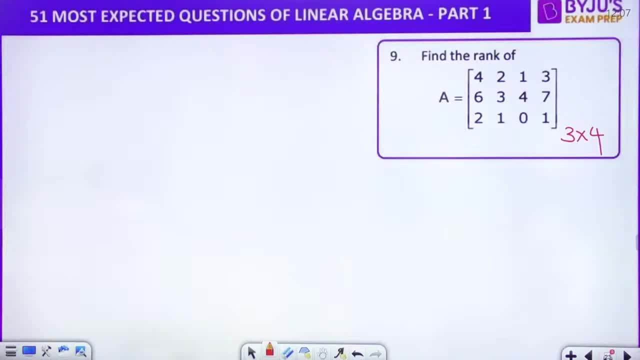 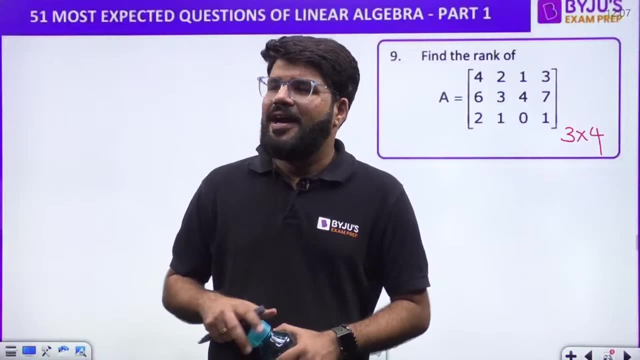 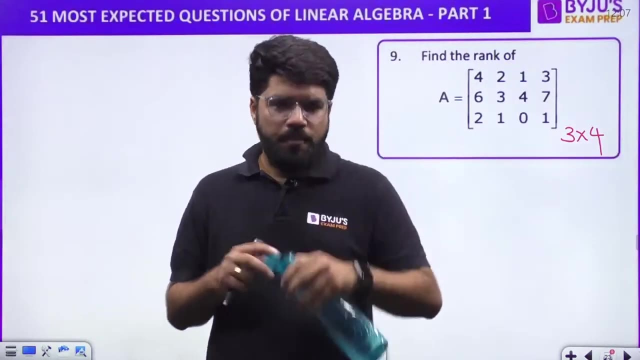 a row 2 r 1 and a row 2 r one, and that's the answer to the question. do you think that today's Yes, guys chalo? Now I told you the dependency method which I am talking is applicable on rows as well as columns. Dekho, I will show you that. yes, Manjeet, very good Sometimes. 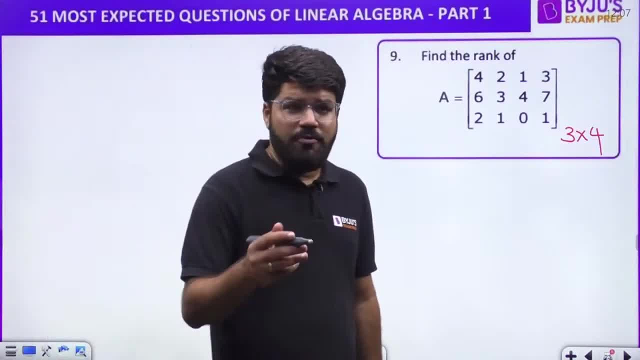 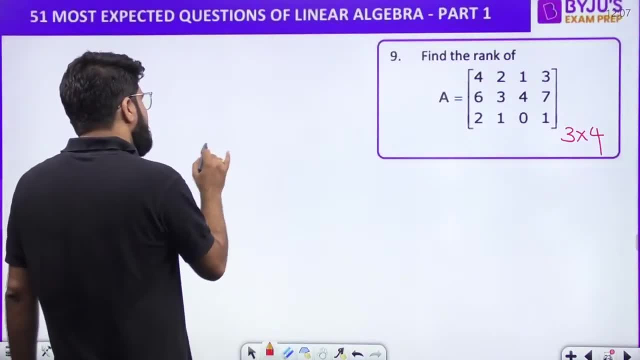 you may not be able to find the dependency between the rows. You may not be able to find, There will be dependency, but you are not able to find because dependency is any dependency, Kabhi, kabhi, asa bhi ho sakta hai. Suppose there may be a dependency of the form 5r1. 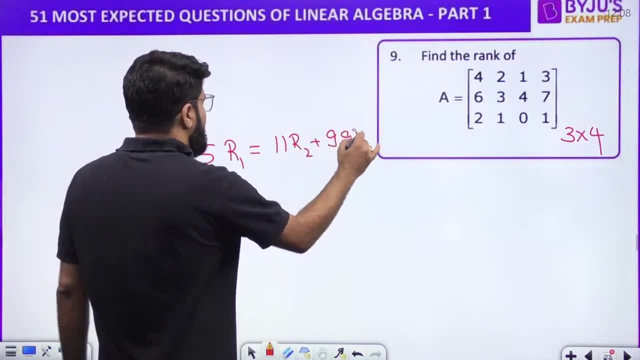 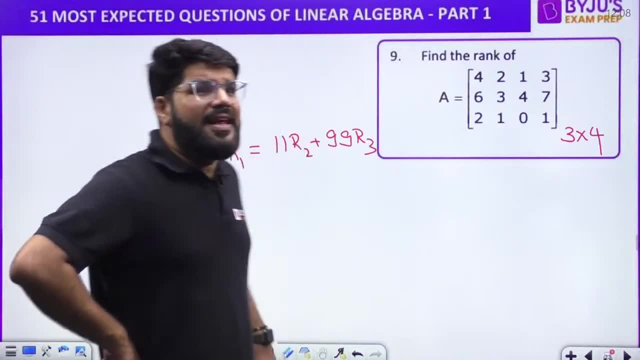 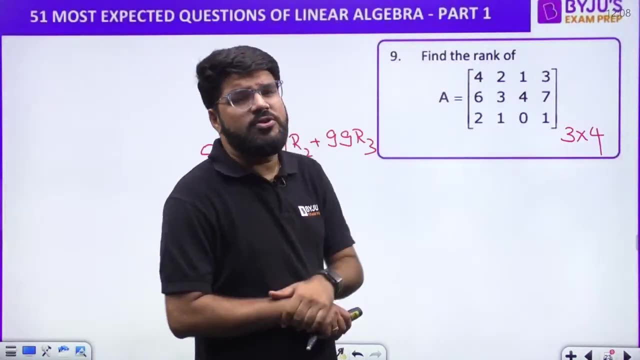 is equal to 11r2 plus 99r3.. What will you do then? Maybe this is also a dependency, na, This is also a dependency, So there can be sometimes, you know, complicated dependency Dekho, so here you are not able to figure out. a dependency does not mean that there. 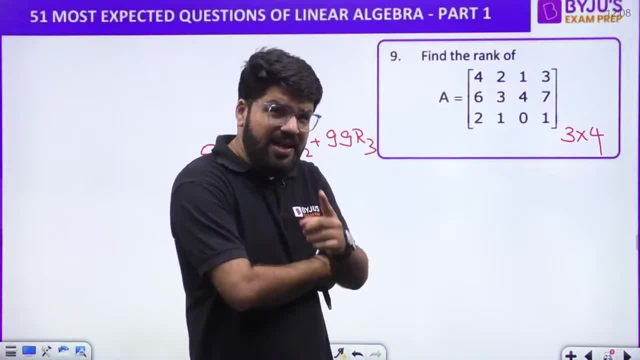 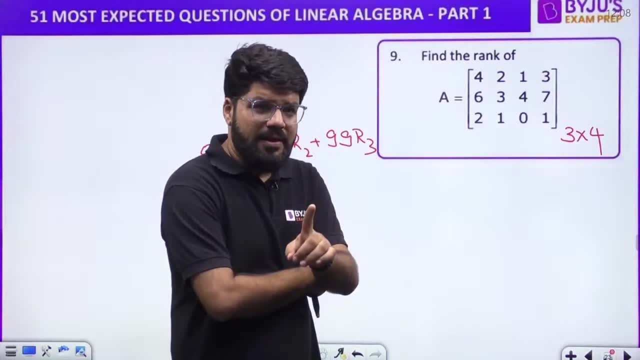 is no dependency. So don't comment that. the answer is 3. Either confirm by equivalent form If you are not able to find the dependency, either confirm by equivalent form. If you are not able to find the dependency, either do the echelon method. Either go for the echelon method, If not, go for the columns. 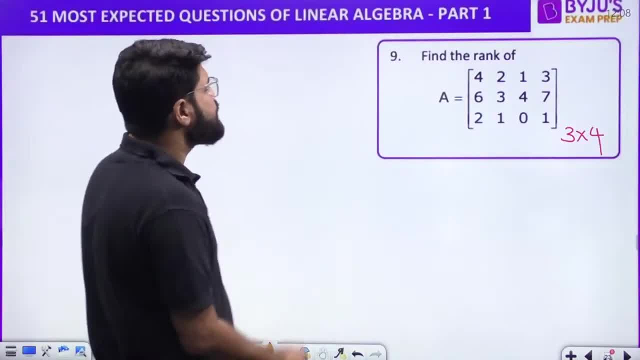 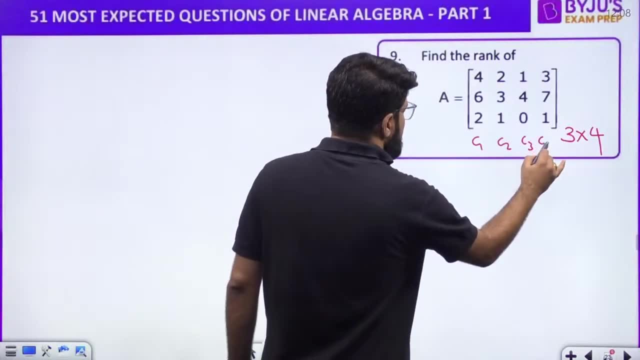 also Columns bhi to hain, Columns bhi to hain Right. So if I take this as the columns C1, C2, C3, C4, clearly these are related as double 2 into 4, 3 into 2, 2 into 2, 3. 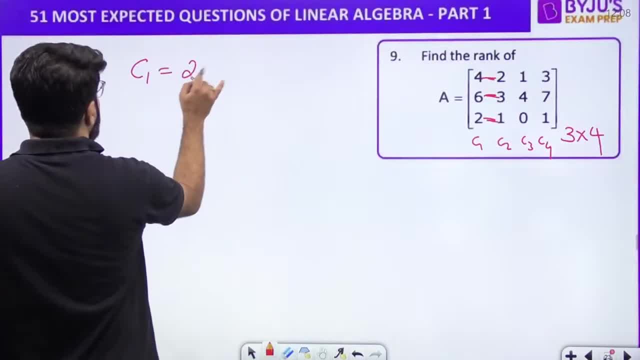 into 2, 1 into 2.. So they are related as double Column. number 1 is twice of column number 2.. It is twice of column number 2.. So it is twice of column number 2.. So it 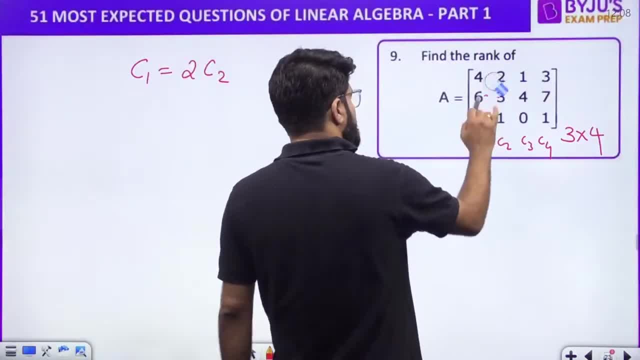 is times 2 of column number 2.. So it is times 2 of column number 2.. So let us look. So here we have 2. 저는 c1, c2.. C1, c2.. So you can use that Enter 1 is right there. 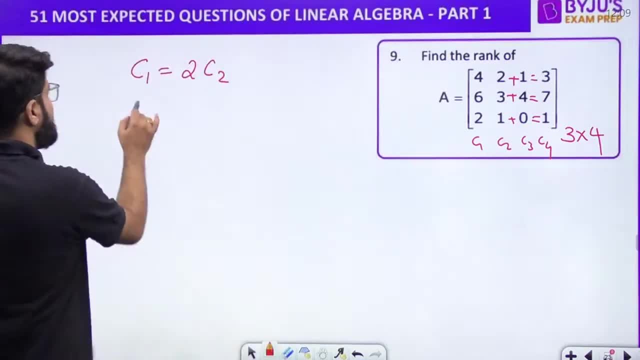 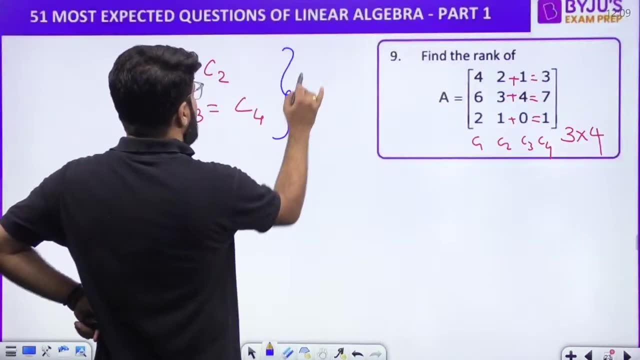 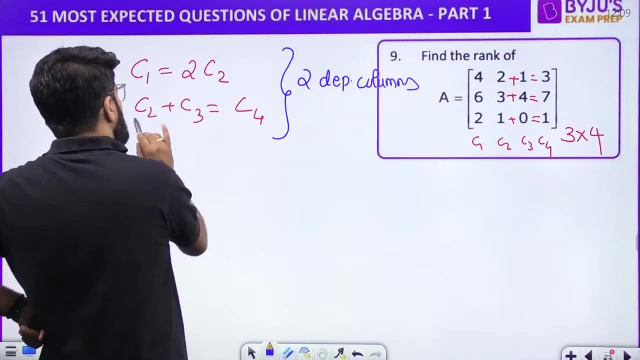 Here, all right, so c2, c3, c3 number I asked, and then I asked c2 anymore. You do the same number as before. c2 will be equal to c2. Then I can do only one cleaning. We are simply following c1, c2.. 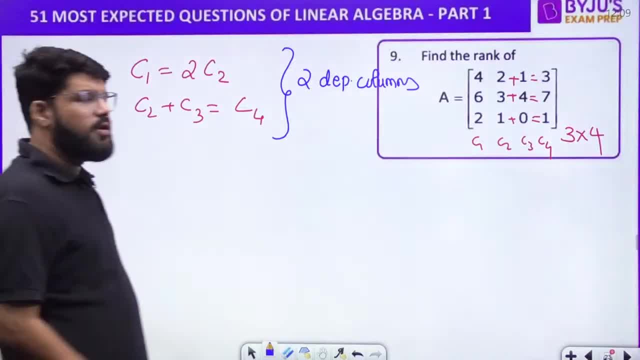 2 is the right answer. 2 is left: nec pe 2.. nec pe bli bhi a SI c3, c3, c4, c3, c4, c1, c2, которая has the corresponding number. here We have two dependent columns. 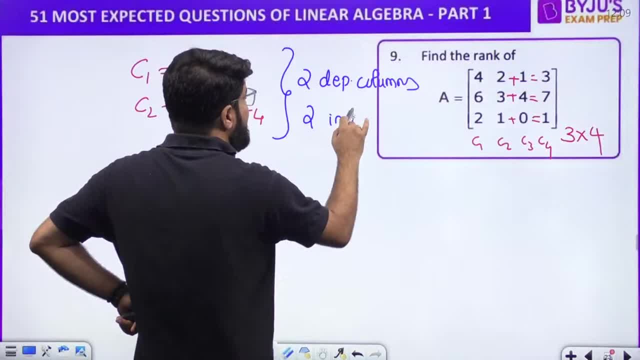 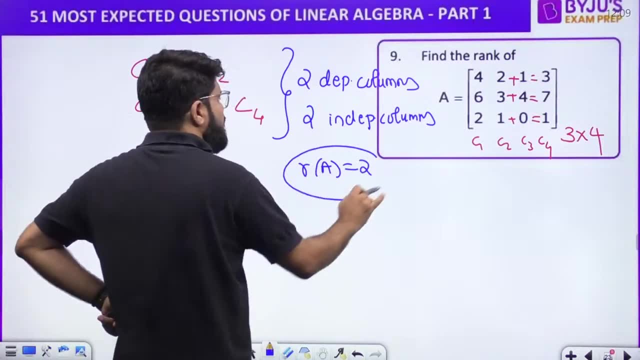 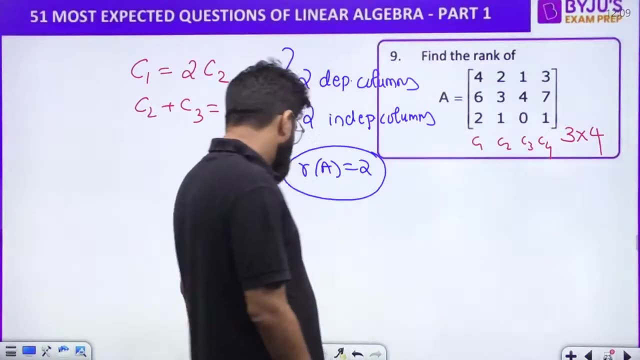 So we have total four columns, So two independent columns. So rank is equal to two. Rank is equal to number of independent rows or independent columns of the matrix. applicable to both rows and columns. You have to keep this in mind. Applicable to both rows and columns. 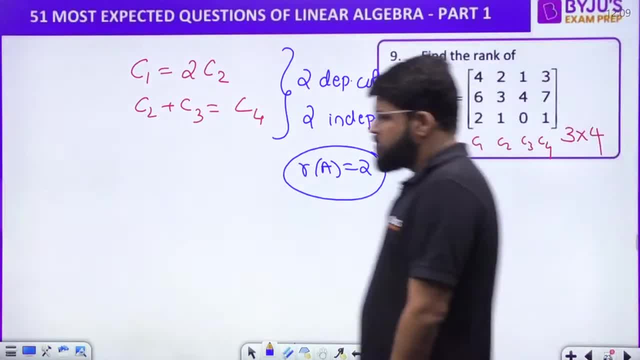 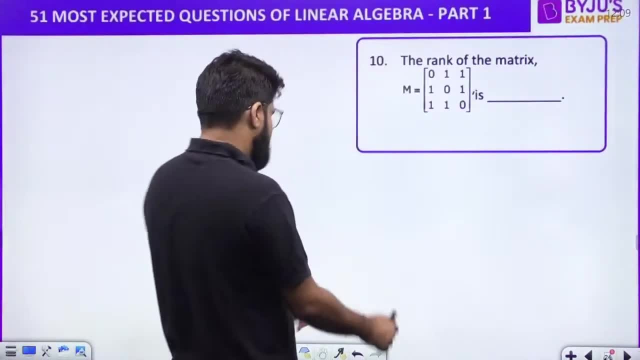 Applicable to both the rows and columns. So rank of the matrix will be equal to two. Rank of the matrix will be equal to two. Find the rank of this given matrix. This one put it as a simple question You can even solve by the basic determinant method. 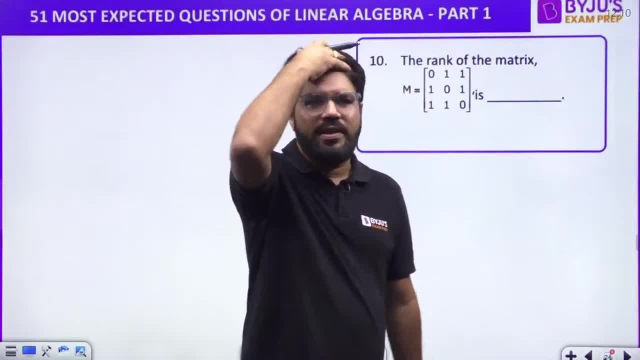 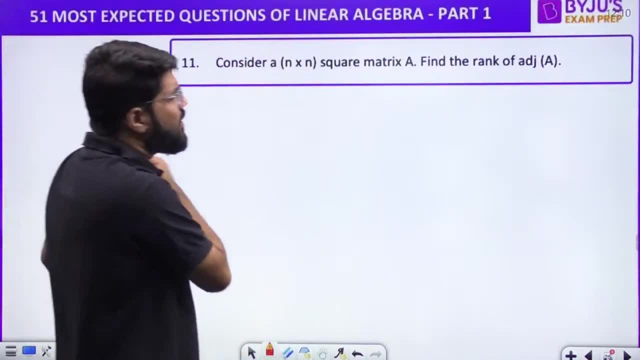 This is a homework. Similar type of questions homework. Let us understand all variety of questions of rank and linear system of equations today. Consider a, n, cross, n square matrix. Find the rank of adjoint. This is a last moment of time. 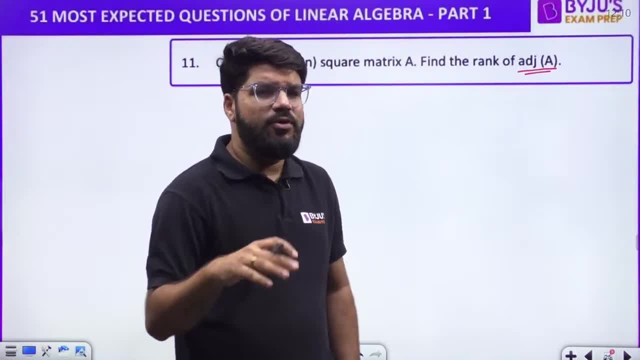 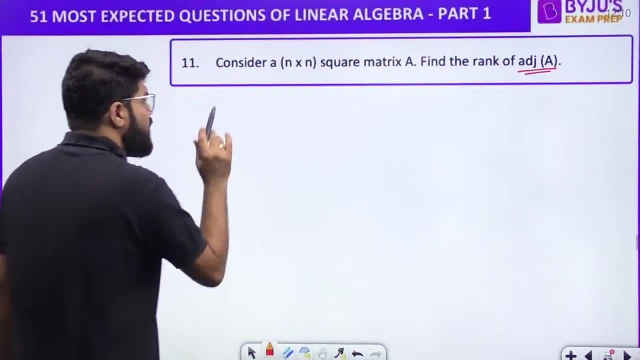 There is no need of derivation. There are some standard results which I will give Derivations you want, you can try at home. Rest concept and logic and calculations, everything. I am explaining you. What is the rank of adjoint a? 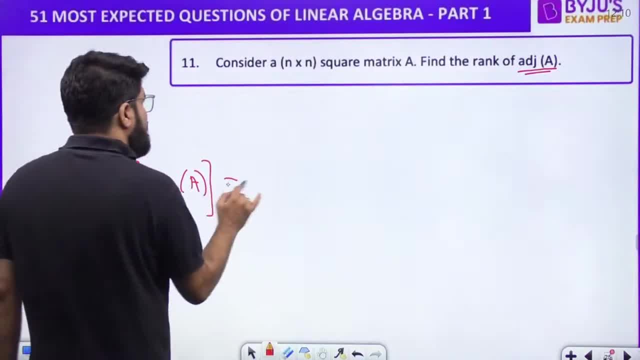 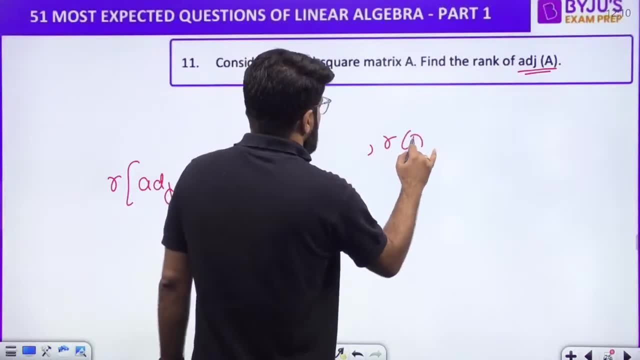 What is the rank of adjoint a? What is the rank of adjoint a If the rank of n is equal to if the rank of a rank of a must be given to you. If the rank of n is equal to if the rank of a must be given to you. 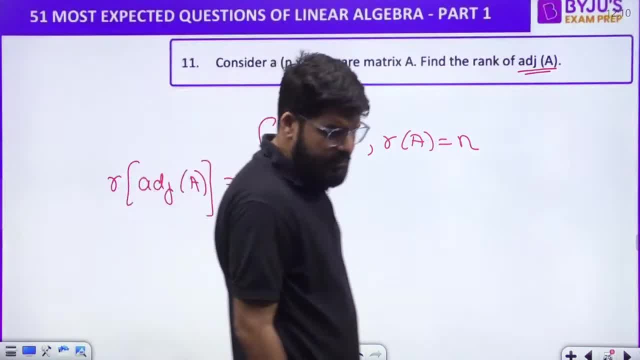 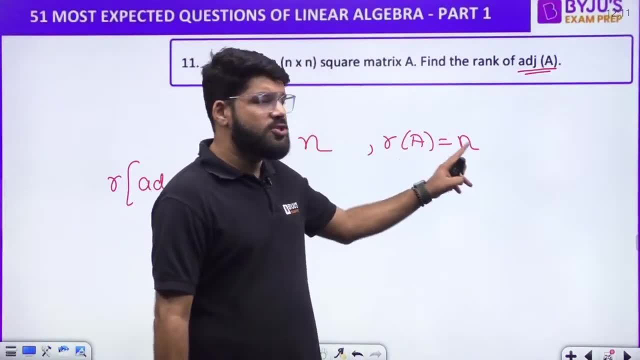 If the rank of a is equal to n, then the rank of adjoint a will also be n, Because if rank of a is equal to n, then it is the full rank case. Then the determinant of the matrix is non-zero And determinant of adjoint a also will be non-zero. 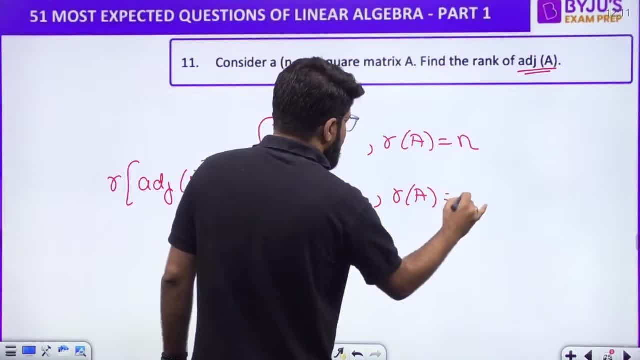 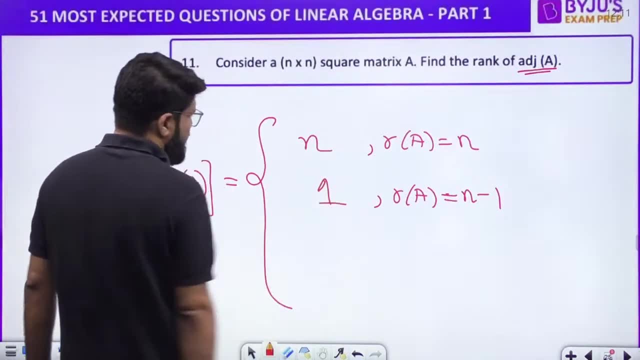 Next, if the rank of a is equal to n minus 1.. If the rank of a is equal to n minus 1, then the rank of adjoint a is 1.. Directly, it is 1.. Directly, it is 1.. 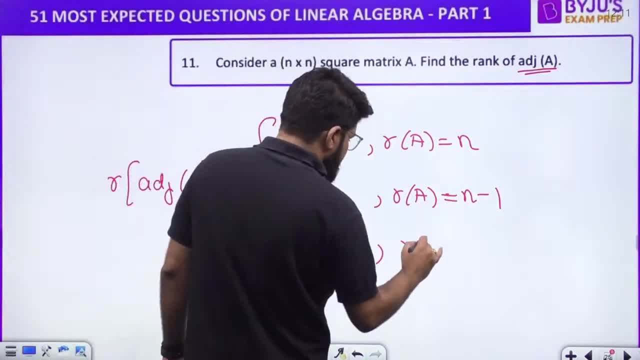 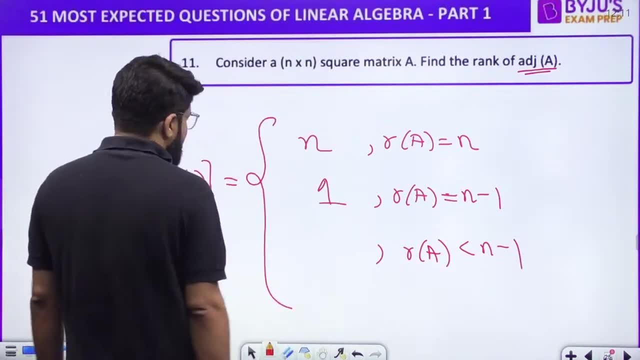 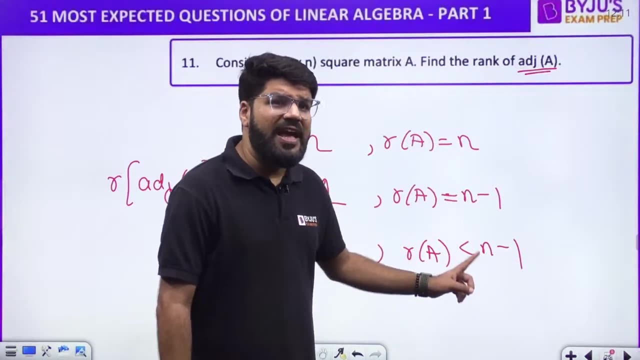 And if the rank of a is less than n minus 1.. Any value less than n minus 1.. You can simply understand logically. if the rank is less than n minus 1, means all minors of n minus 1 size. Think: all the minors of n minus 1 size- are 0. 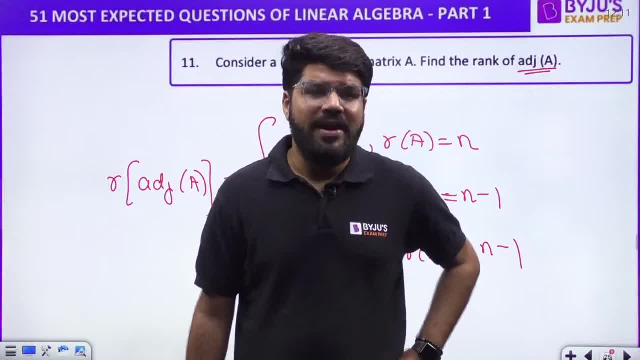 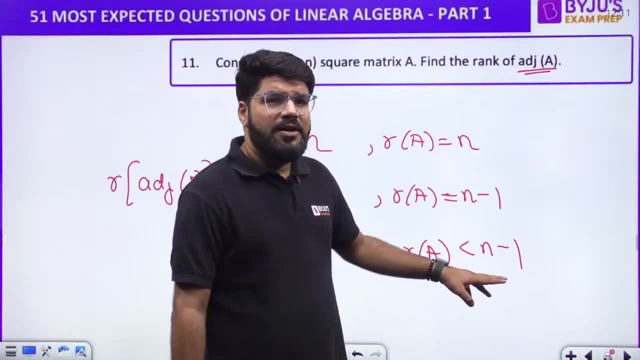 How do you build an adjoint? Adjoint is built by cofactors. Cofactors depends on minors. Cofactors depends on minors If the rank is less than n minus 1, so all minors of n minus 1 would be 0. 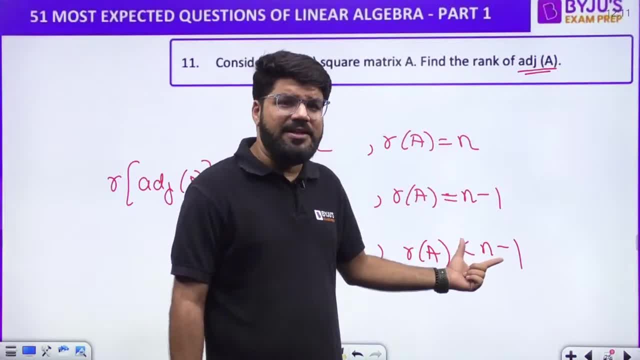 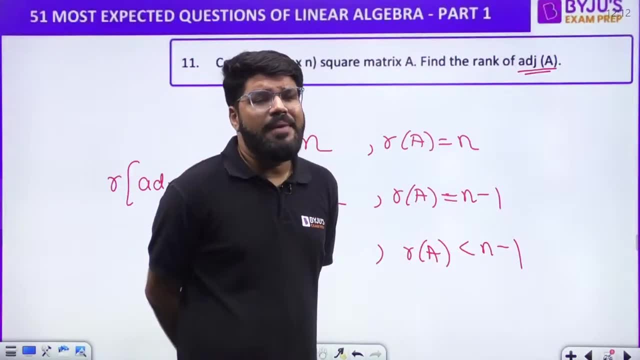 If there was a n minus 1 minor non-zero, then the rank will be n minus 1.. I say that, I say that. just remember my logic, honey. If the rank is less than n minus 1, all minors of the size n minus 1 will be 0. 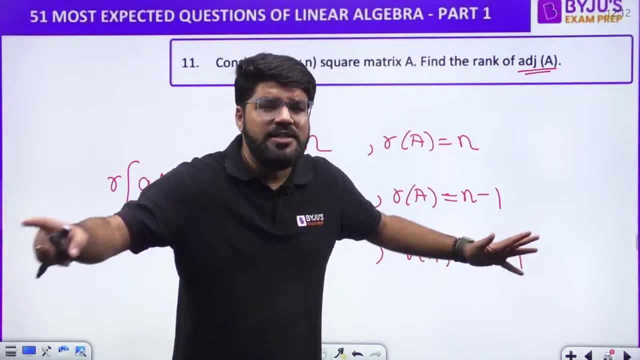 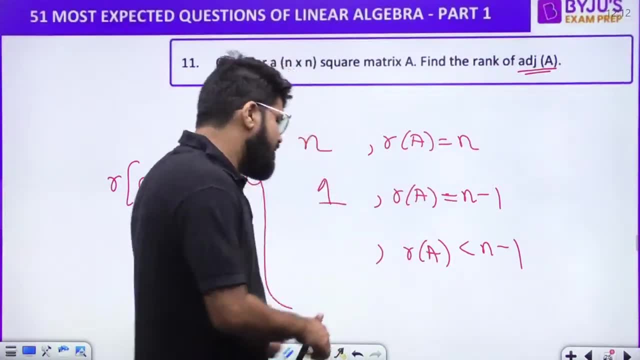 That means all cofactors will be 0.. All cofactors will be 0.. So what do you get in the adjoint? Nothing. All the elements of the adjoint matrix are 0. It is a null matrix. It is a null matrix. 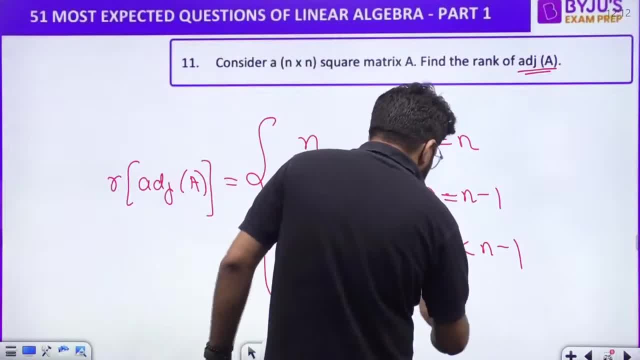 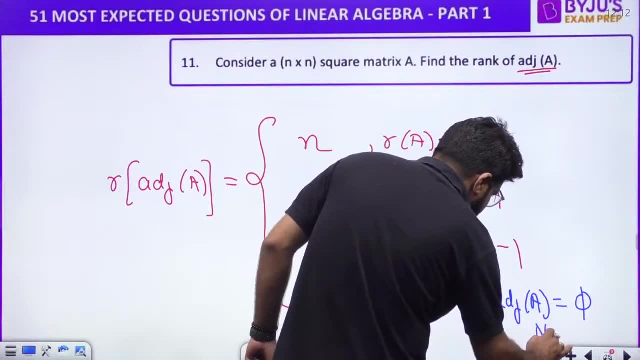 And hence rank will be 0.. And hence the rank will be 0.. So whenever the rank of a is less than n minus 1, adjoint of a will be a null matrix. That is why the rank will be 0.. 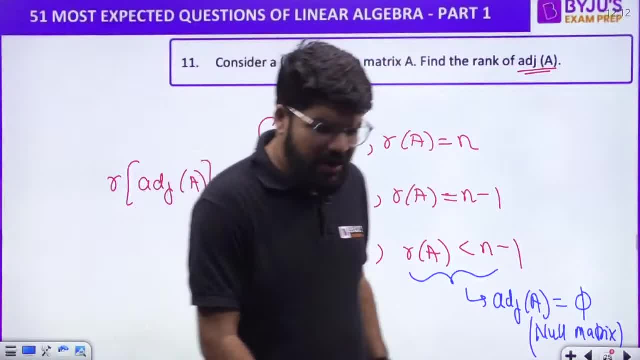 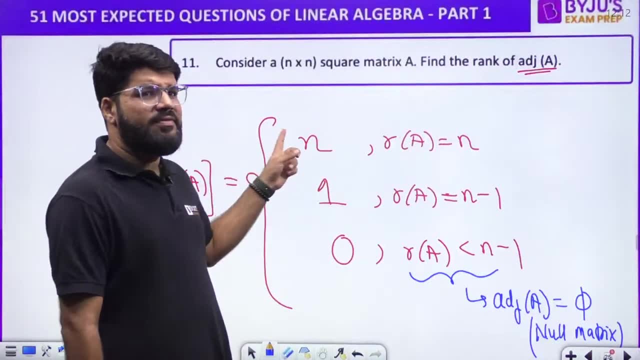 Rank equal to 0 only for a null matrix. What is a null matrix? All elements are 0.. So these are the three conditions. If rank of a equal to n, adjoint a also will have the rank n. If rank of a less than n minus 1, adjoint a is a null matrix. 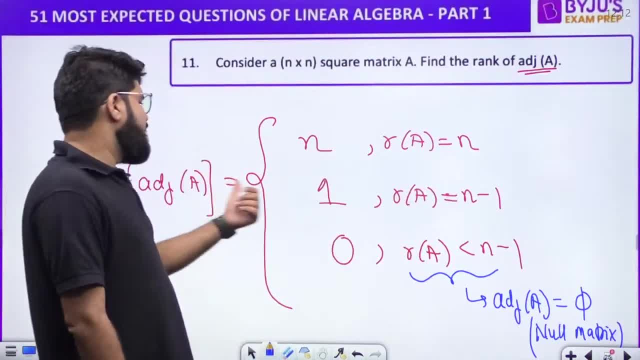 So rank will be 0.. If rank of a equal to n, rank of a is less than n minus 1, rank of adjoint a turns out to be 1.. This is a simple. This has a simple. These two are clear by the logic. 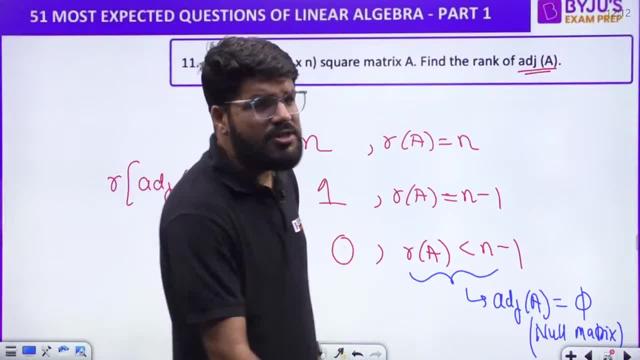 This is a simple mathematical derivation. But no need of derivation right now. Let's focus on the questions. Okay, guys. So just remember. it is a standard result. Now they can give you any value. Here I have generalized n, cross, n. 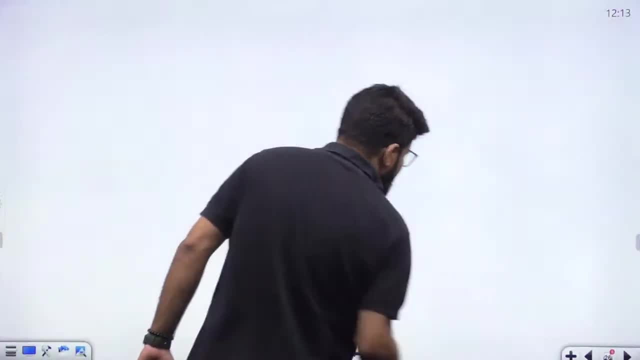 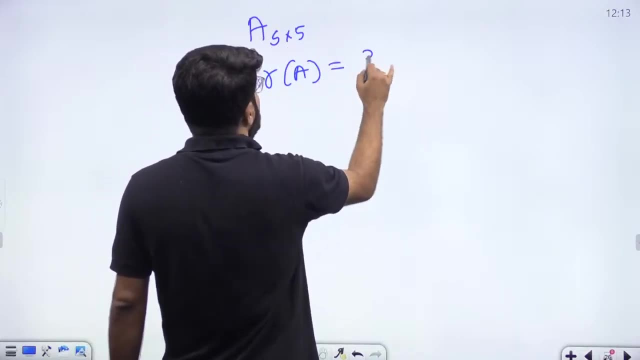 They can give you any value and ask you the question. Okay, They can give you any value, Suppose they can give you. They can give you a question like this: A is a 5 cross 5 matrix And rank of a is given to be 3.. 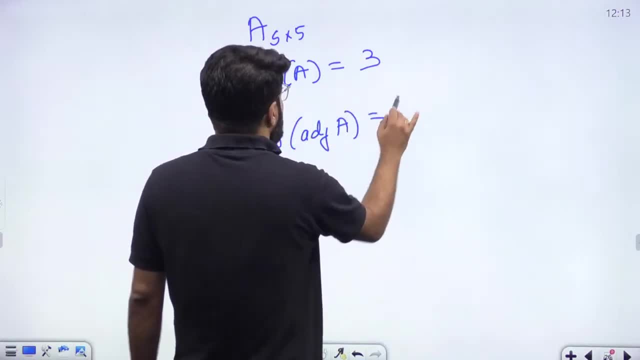 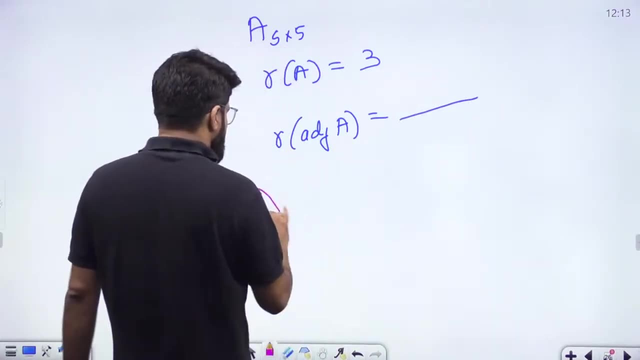 What is the rank of adjoint a? They can give you questions in the numeric form: What is the rank of adjoint a N-80 type question. So tell me what should be the answer. Right, So rank of a which is given. 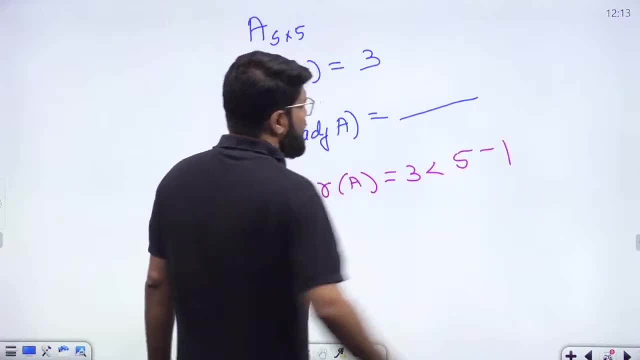 that is equal to 3, but that is less than 5 minus 1.. That is less than n minus 1.. That is less than n minus 1.. Right, So what is going to be the rank of adjoint a in that case? 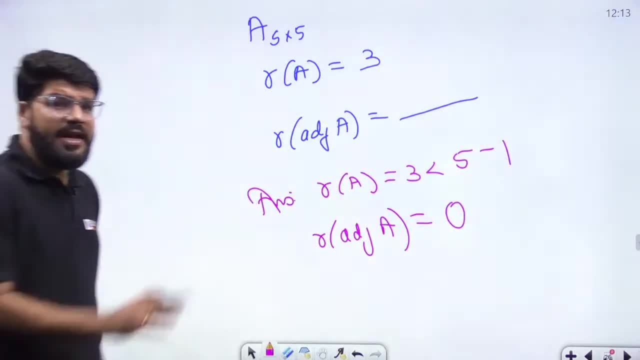 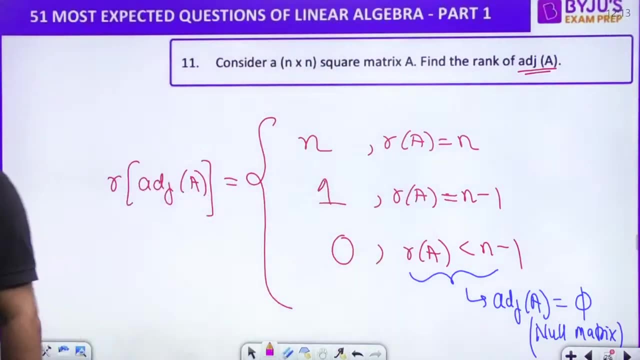 Rank of adjoint a will be 0.. Adjoint a will be a null matrix. They can put it into numbers. They can frame the question into numbers. I have given you the general results. I have given you the general results, Right. 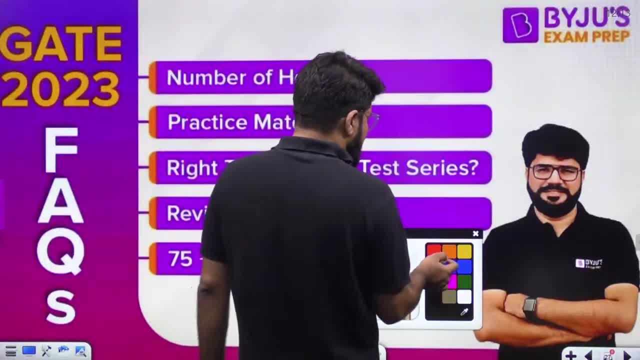 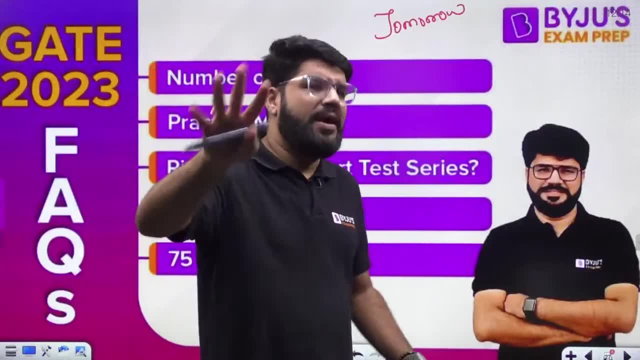 Okay, Before we move to the next question, a quick reminder that this session is going to come for you tomorrow. Right, Last 3 months, more than 3 months around, 100 days- you can say Last 100 days around- are left for the GATE examination. 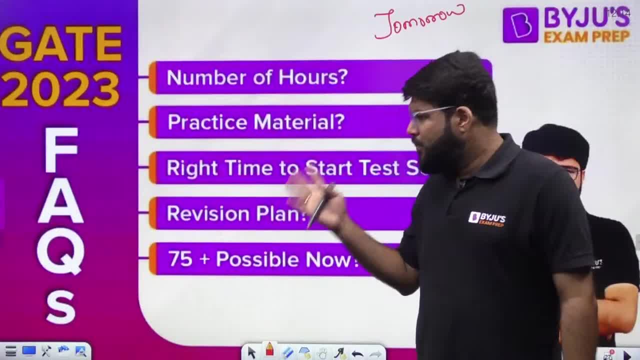 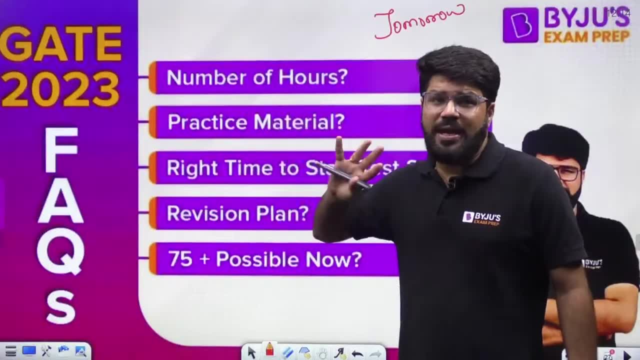 Okay, If you have any of the doubts regarding to the preparation, regarding to your practice, what should be the revision plan now? how many hours to study now? Now it is the crucial time Now. no compromise, No. What is the right time to start test series, especially the mock test, and is 75 plus possible now? 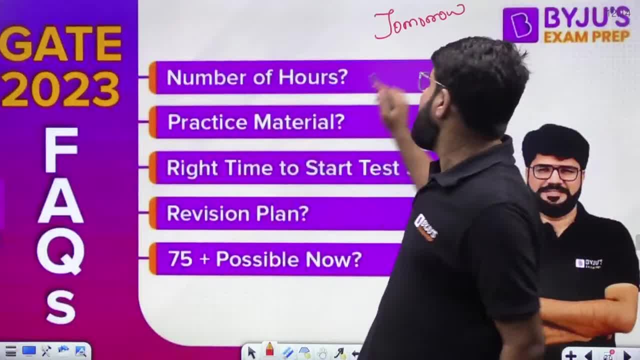 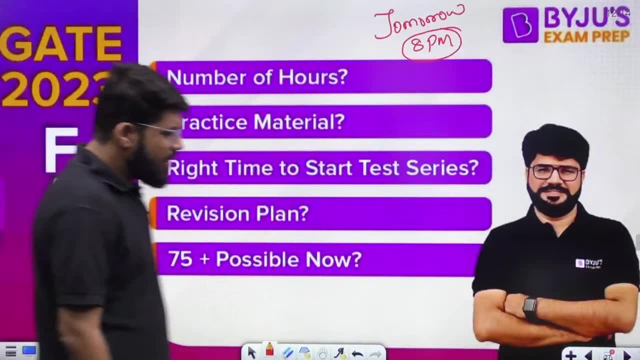 Get answer to all your. if you have any of these doubts, do join me live tomorrow, 8 pm. This is tomorrow night at 8 pm. Join me, live and we'll rectify all your doubts. Okay, Let's move ahead to the next question. 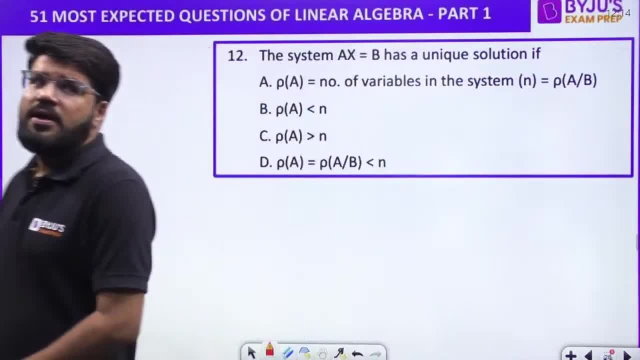 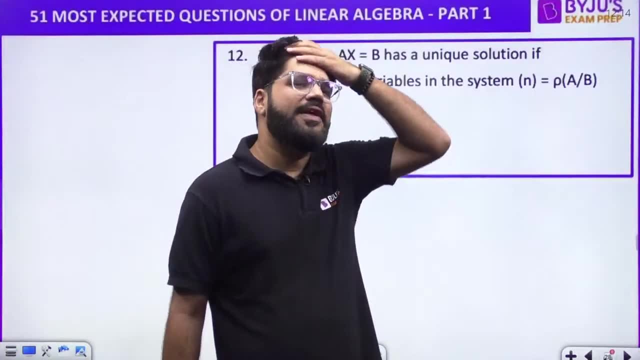 Number 12.. Next question, Number 12.. The system AX equal to B has a unique solution. If now let me test how many of you remember I'm going to, you know, review all of that, the results You need to remember now, whatever we have done in the rank till now. 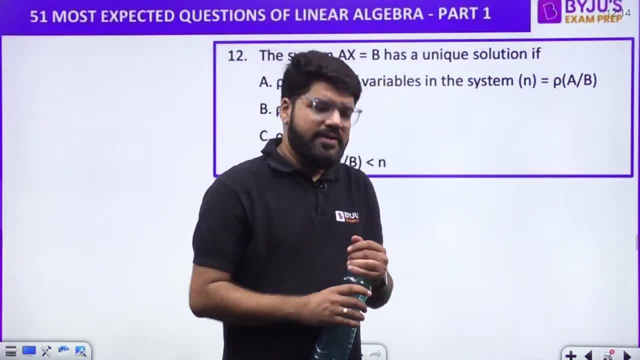 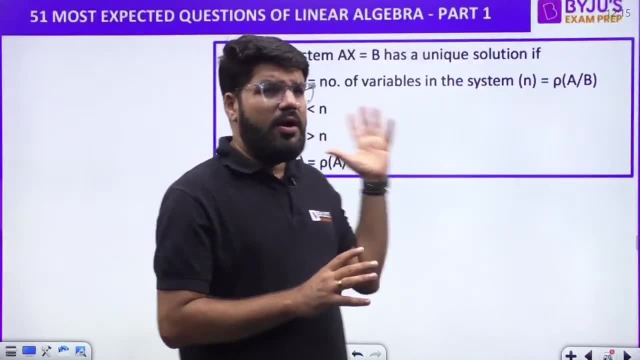 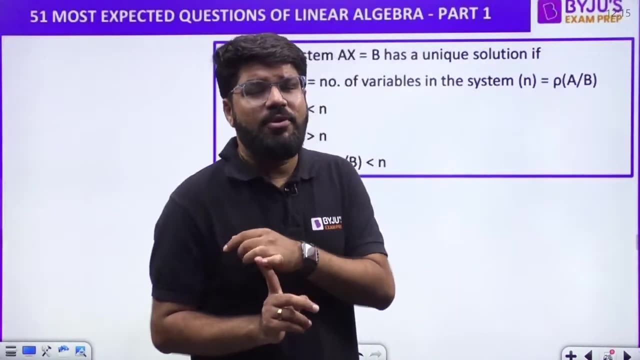 Okay, Yeah, sure, honey, I will try. I'll try. If this is helping you, I'll try. Do not forget to like the session. Keep liking the session, guys. Okay, so you know, whatever 11 questions we have discussed for the rank, rank will be used here also. rank will be used even in the system of equations. 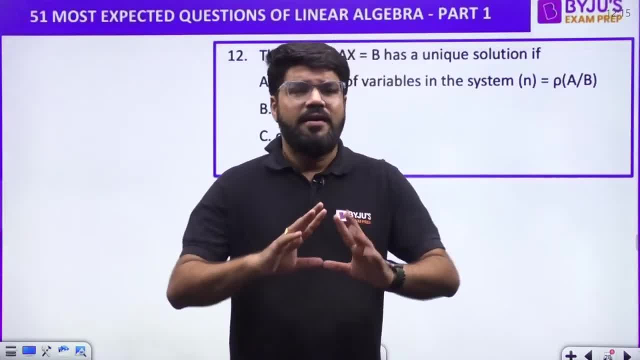 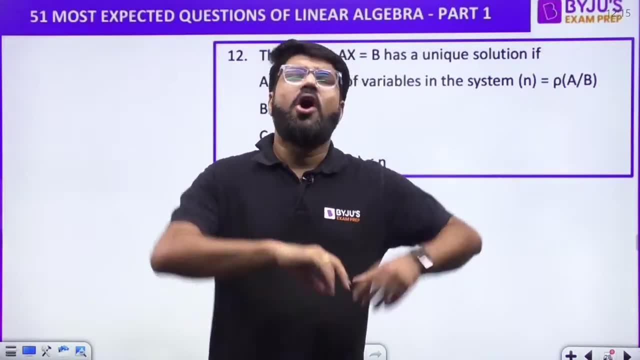 But? but whatever questions we have done with rank, whether it is determinant method, it is the echelon method, echelon form method, Or it is the dependency, independency method, all questions of rank will be simplified And, don't worry, you have covered everything with respect to rank. 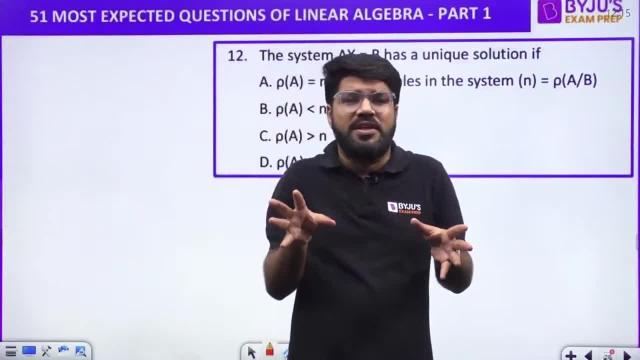 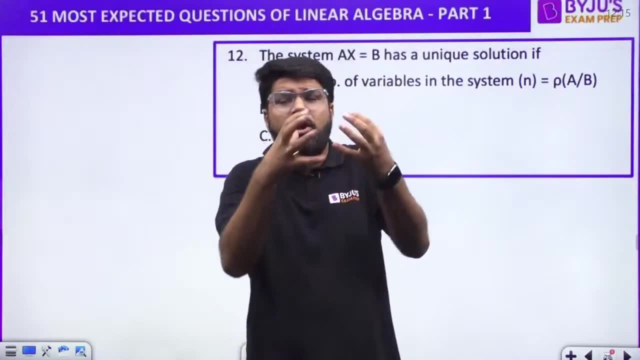 Okay, And that is why I'm bringing you and bringing you a question- express type of series question. We cover current and I'm explaining you the methods and concepts as well. Right, You are able to see that we are not going into, you know, theoretical type of thing. 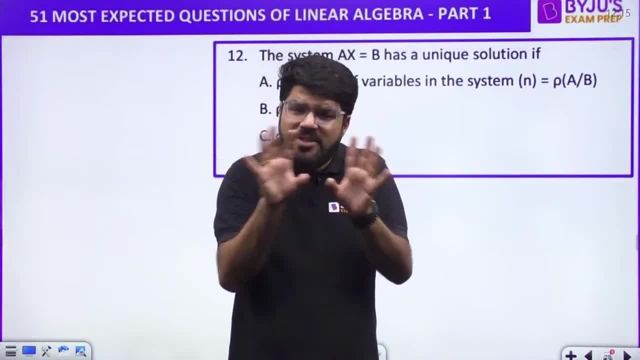 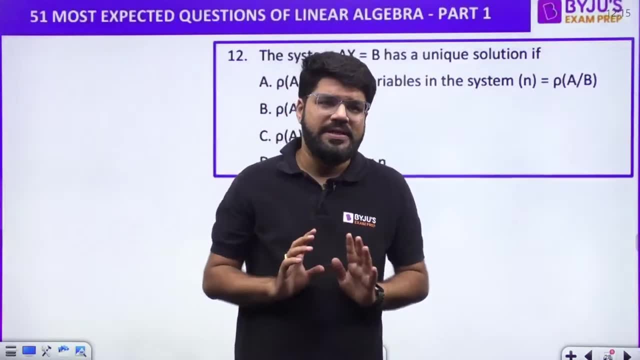 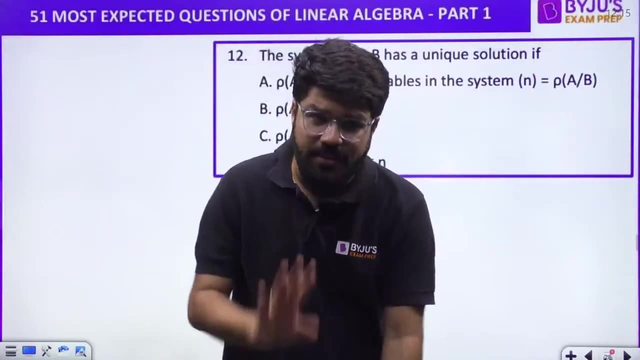 We are not defining, We are not stating the theorem. that is not actually required here. If required, I will tell you that also. But what is required? question, The approach of the question. Question and some important points. even if you have not studied algebra, I hope this session can still get you marks in the gate. examination for the questions of algebra. 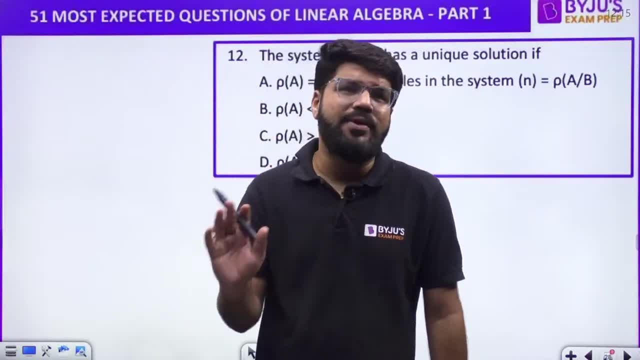 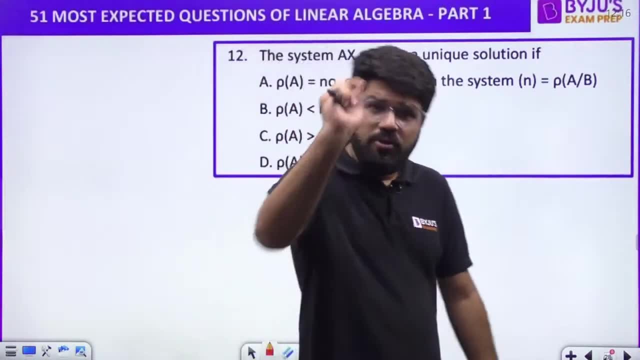 Okay, don't worry, this session and tomorrow. Tomorrow we will have eigenvalue, eigenvector, 11 am- 11 am. Today was again 11 am, But today it was little bit, you know, postponed for 30 minutes. tomorrow 11 am. 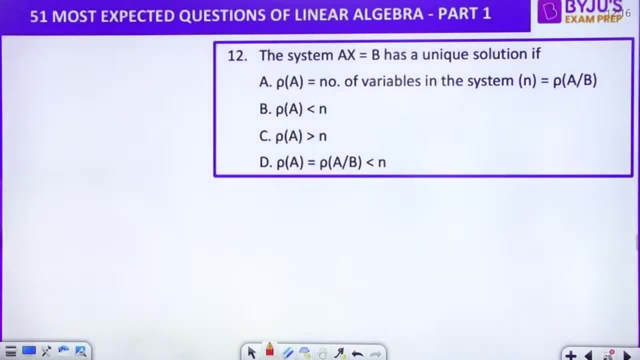 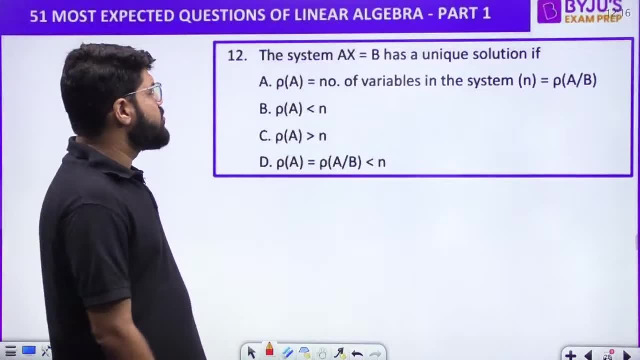 We will meet. Okay, The system AX equal to B has unique solution. If, what? if? what is the condition? true? rank of A is equal to number of variables in the system is equal to. rank Of A is to B. rank of A less than N. rank of A greater than N. rank of A equal to rank of A is to B is equal, is less than N. 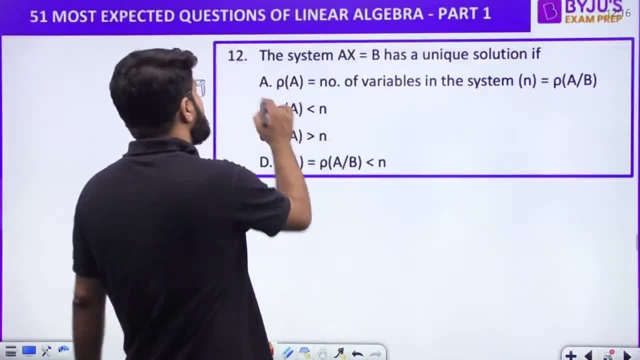 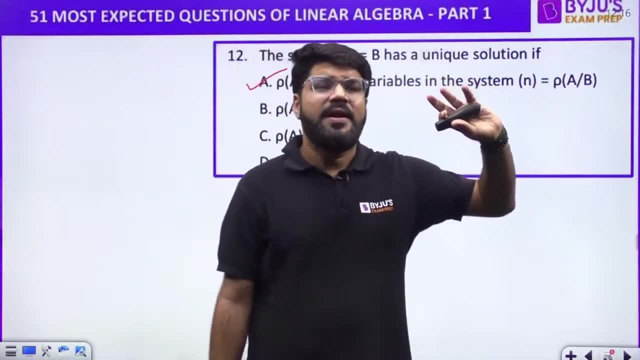 Tell me anybody remembering this point, The? the correct answer is option number A, rank of A. and rank of A is to B. That is, the augmented matrix should be equal to number of variables in the system. If you are not remembering, see, I'm not getting much answers. 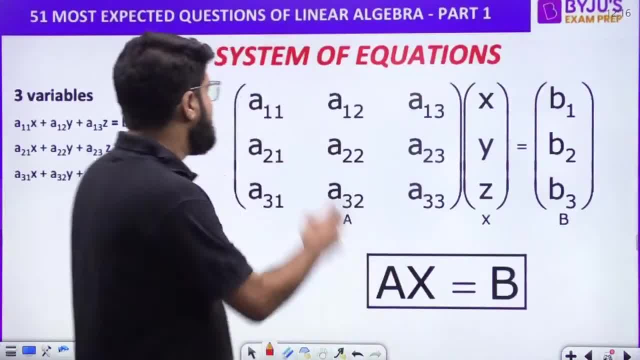 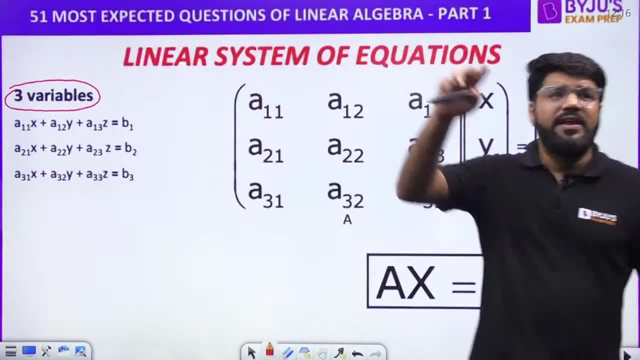 Let us review this, Then go to the proper questions. It's called review, Cutting a linear system of equation Right And commonly the questions can be in three variables, although there can be questions with three variable, four Equals Equations, three variable, two equations under determined, over determined. 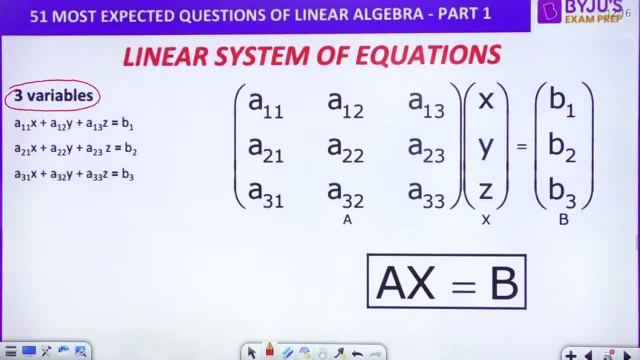 So of course, cover cutting it, Okay, But first let us focus here: Right, Three variables. Right, X, Y, Z. So we have three equations, normally for three variable: even one, X plus even two, Y plus even three Z equal to B one and et cetera, et cetera, et cetera. 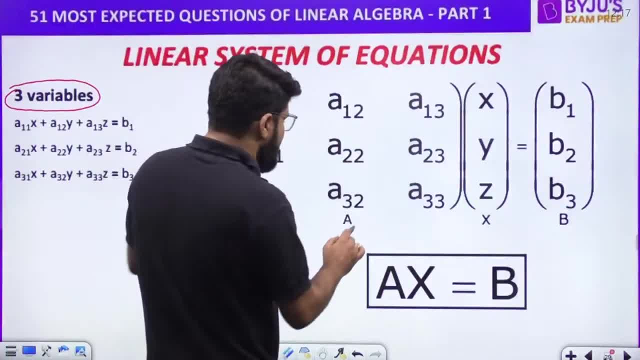 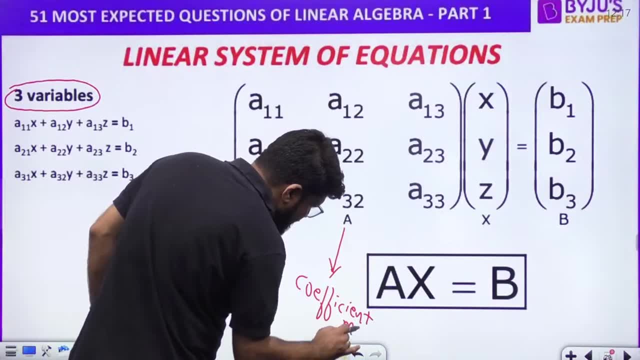 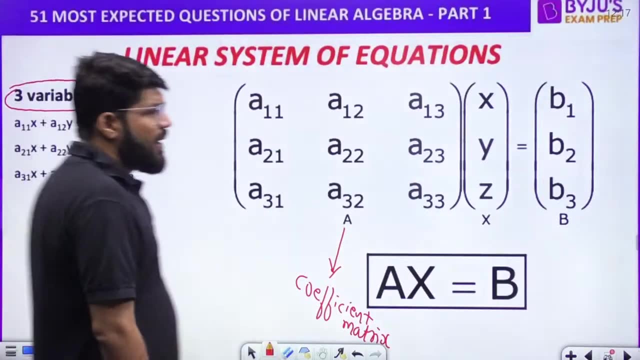 First of all we write down into the matrix form, where this is the matrix A. matrix A is known as Matrix A is here known as the coefficient matrix. The matrix A is known as the coefficient matrix. The matrix A is known as the coefficient matrix. 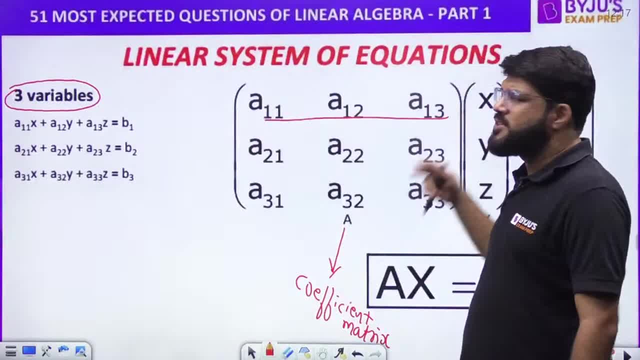 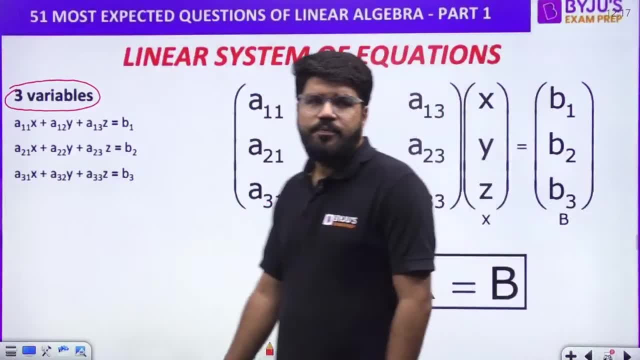 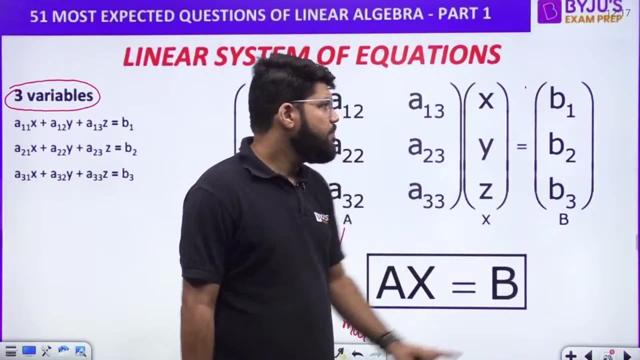 Right, It contains all the coefficients. First equation: coefficients in the first row. Second equation: coefficients in the second row. Third equation: coefficients in the third row. Okay, Multiplied by the unknown vector X that contains X, Y, Z variable is equal to the constant vector B, B1,, B2, B3.. 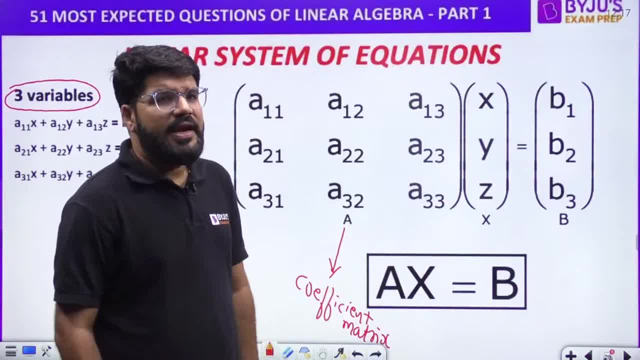 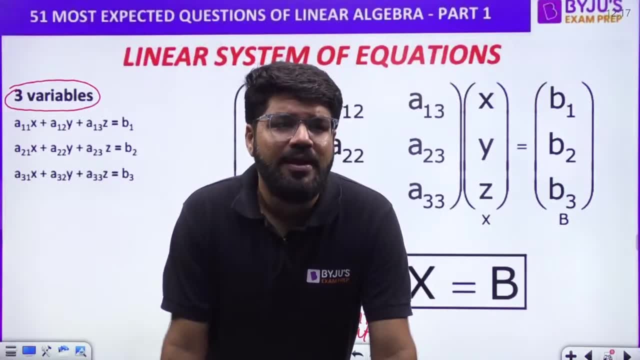 Right, And we write this as AX equal to B. We write this as AX equal to B. Right Now, most ninety nine point nine percent chance, the question in gate will not be finding X, Y, Z. They don't bother. 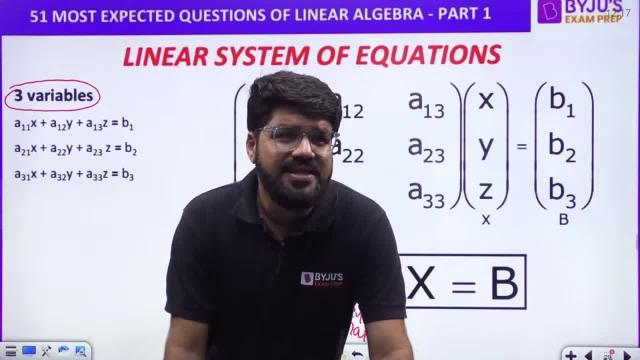 What is X, Y, Z? They only try to test whether you know whether the system has unique solution, infinite solution, no solution. I will tell you method, I will tell you trick, like for rank. Also, we discuss some tricks. 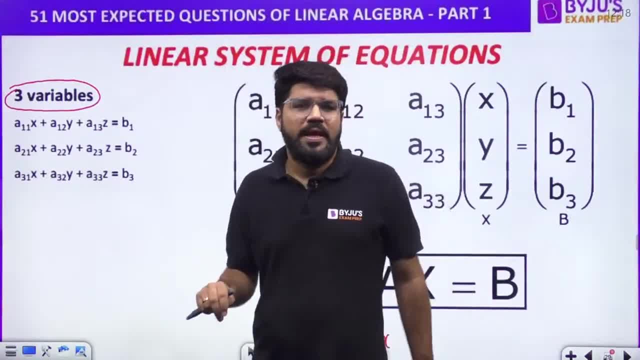 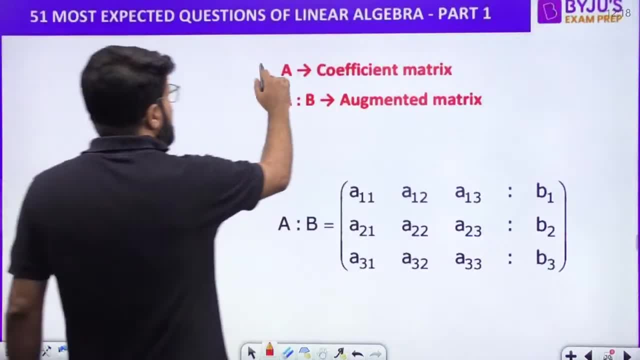 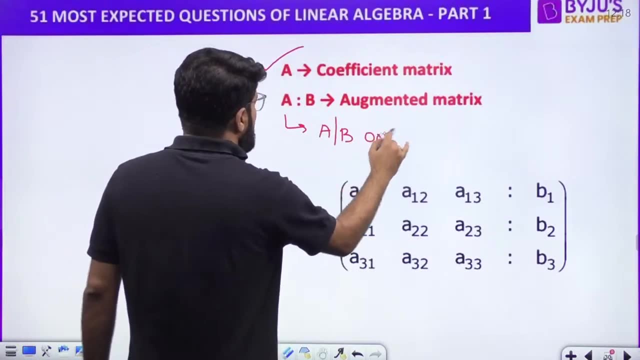 The tricks were related on dependency and independency. Similarly, here I'll also add some tricks based on dependency, independency. But first the method. Okay, First the method. So already I told you, A is the coefficient matrix. We form another matrix. A is to B, or this is also written as A slash B, or this is also written as something like this: 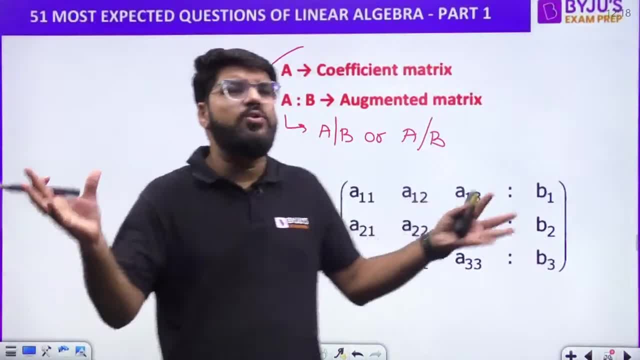 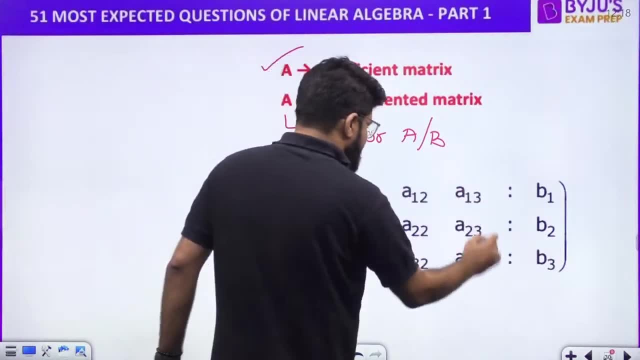 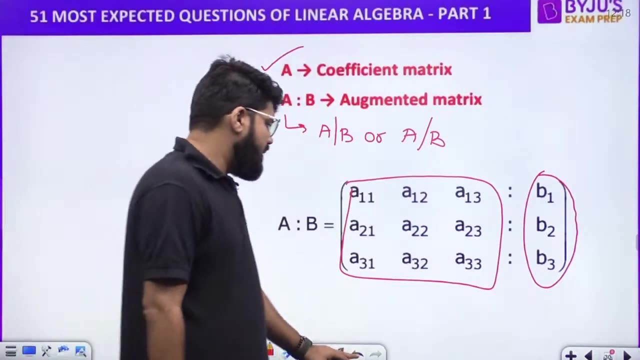 All of this means augmented matrix. Augmented matrix means when two different matrices are combined together to form a larger matrix. Okay, So this part is the matrix A. I'm augmenting, I'm adding the column of B here. This is known as the A is to B matrix and this is of the size three cross four. 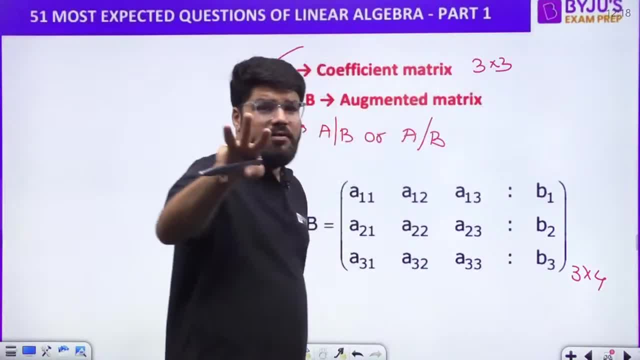 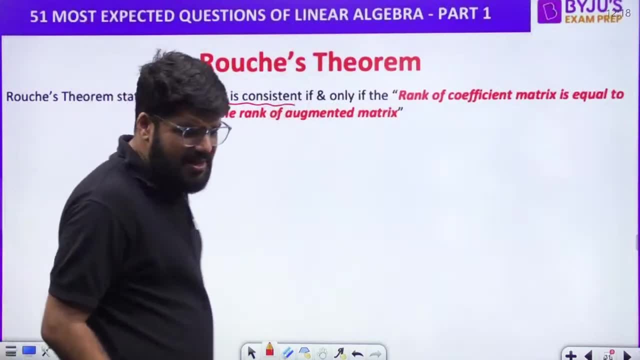 A matrix was of the size three. Z cross three For three. variable system. Rauch's theorem says that a system is consistent. What is the meaning of consistency? What is the meaning of consistency? That means the system will provide some solution. 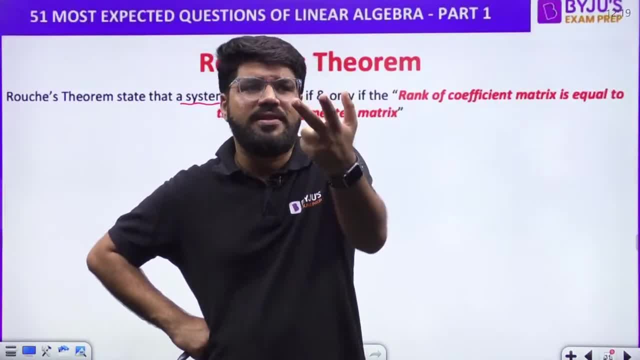 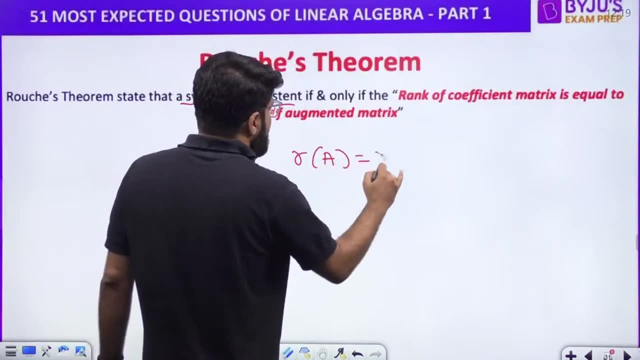 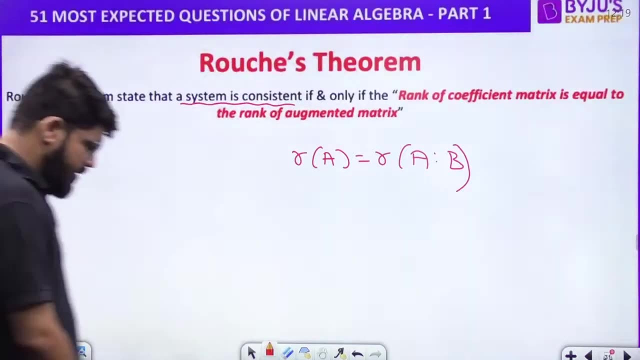 System will provide some solution. It may be one solution and more than one solution, but it will provide some solution. but system is consistent. if rank of coefficient matrix is equal to rank of augmented matrix, Rank of coefficient matrix is equal to the augmented matrix. rank of coefficient matrix is equal to the rank of augmented matrix. okay, dear. 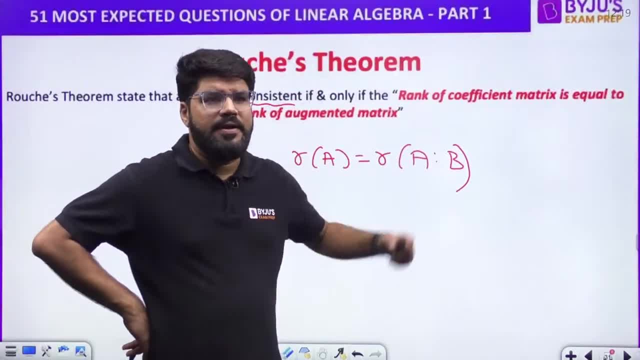 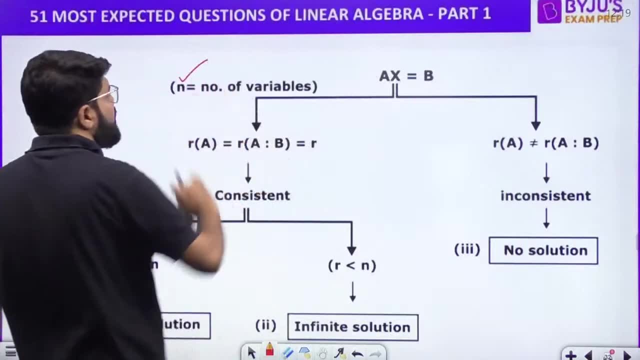 rank of coefficient matrix is equal to rank of augmented matrix. let us, i told you the theorem case. let us understand by the flow chart. it is easy to remember. so you have ax equal to b, where n is the number of variables. if rank of a is equal to rank of a is to b, suppose it is equal to r. 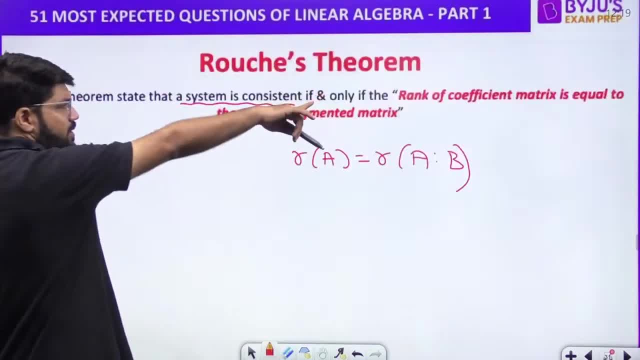 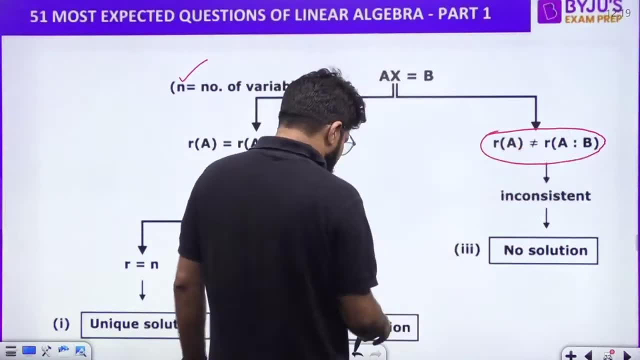 if both these ranks are equal, then the system is consistent. system is consistent. if rank of a equal to rank of a is to b. so if the two ranks are not equal, rank of it does not equal to rank of a is to b, then the system is said to be inconsistent. then the system is said to be. 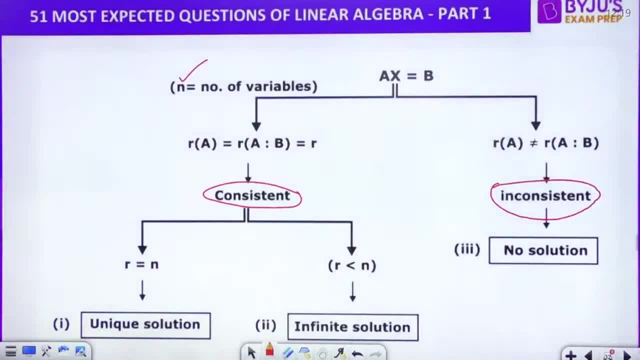 inconsistent and the system will have no solution. the system is said to be inconsistent. inconsistent means the system cannot give you any solution. that is the case of no solution. but if the system is consistent, it will give you some solution. it may be unique, right it may be. 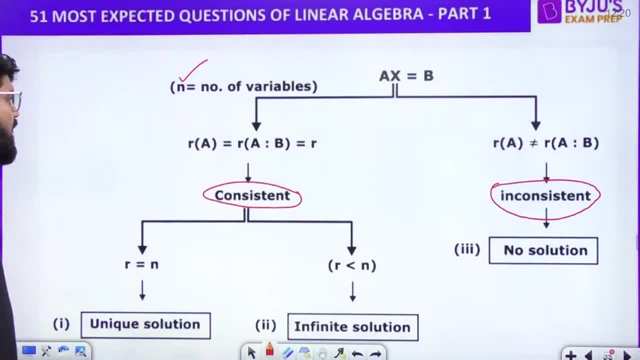 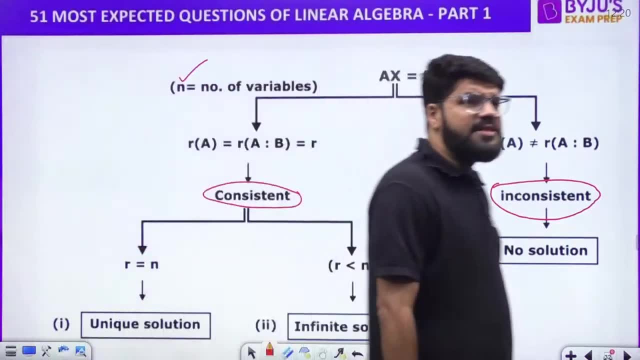 unique or it may be multiple solutions, many solutions. whenever rank of a, equal to rank of a, is to be equal to the number of variables, equal to number of variables, then the system has unique solution. but if both the ranks are equal, both are equal but less than. 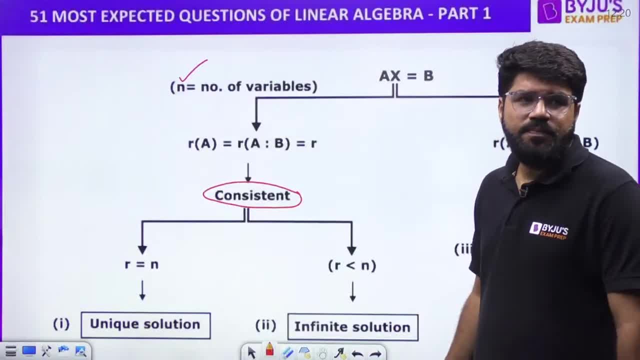 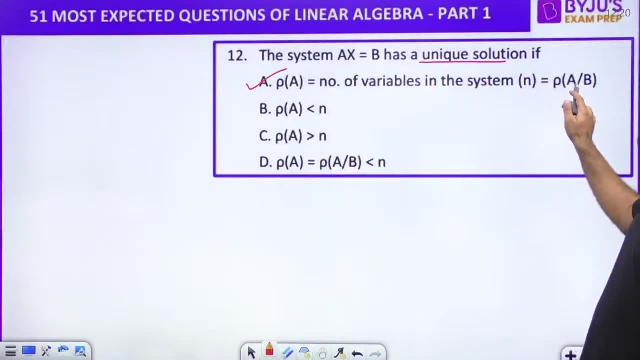 the number of variables, then the system has infinite solutions. right? that is what the first of the question was asking you. system has unique solution if rank of a, equal to rank of a, is to be equal to n, equal to number of variables in the system, equal to number of variables in the system. 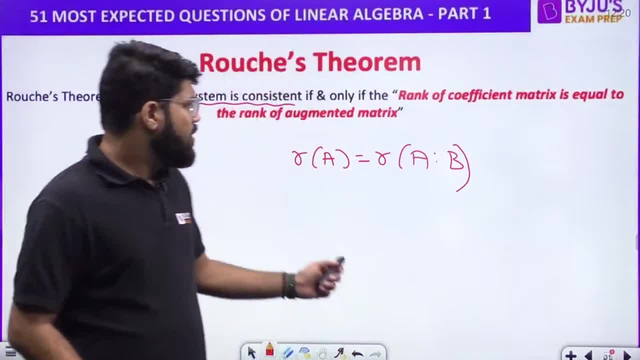 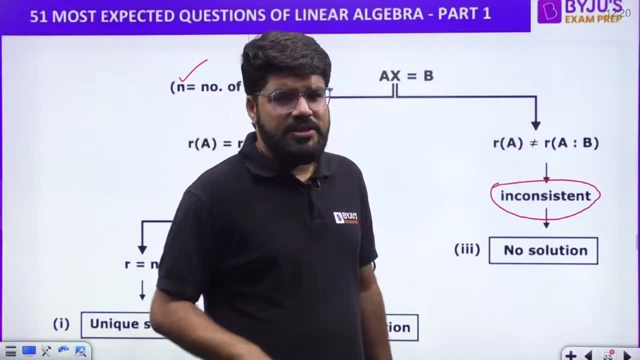 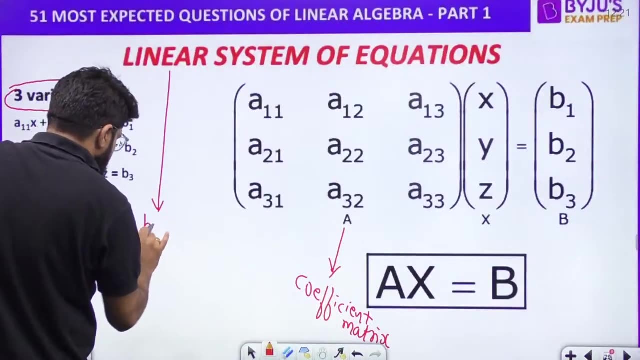 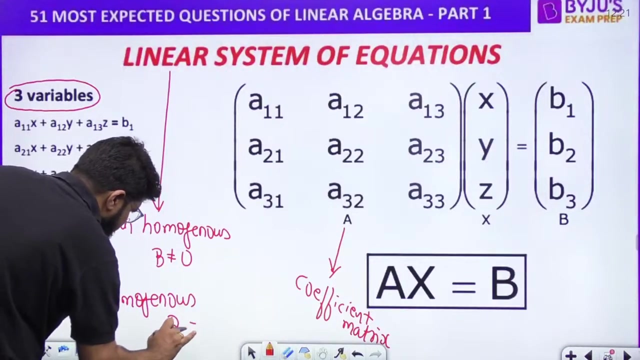 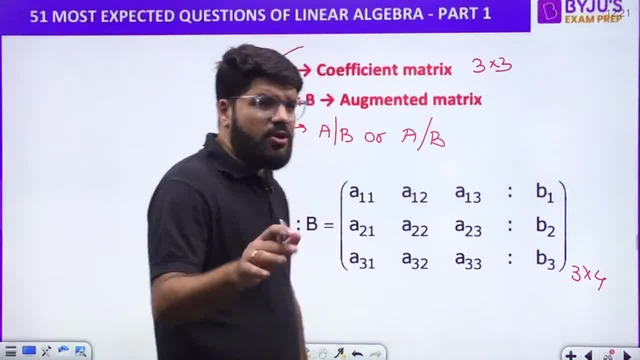 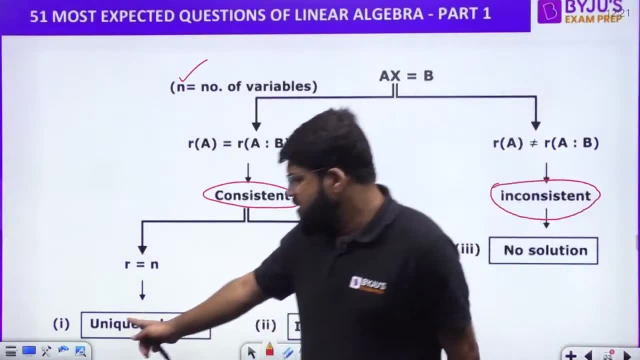 homogeneous with. when b equal to one, 0Right homogeneous value when we Uber equal with one to 0, ax equal to 0. both will be covered. that is also important. both are important. okay, right, this is the flow chart to be remember. now let us separate out the unique solution. this is important. 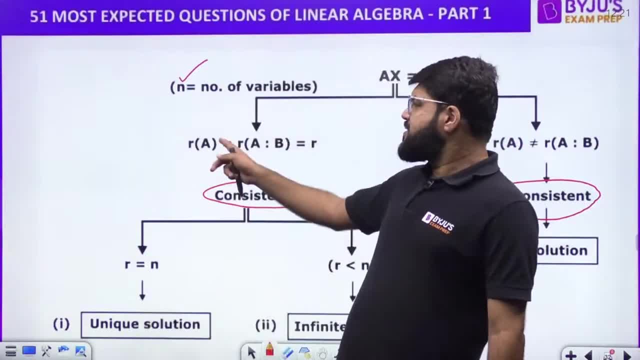 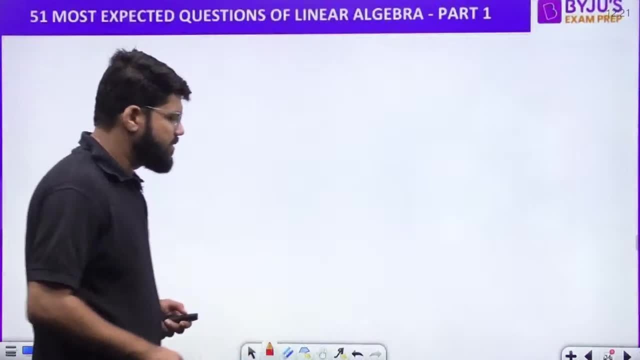 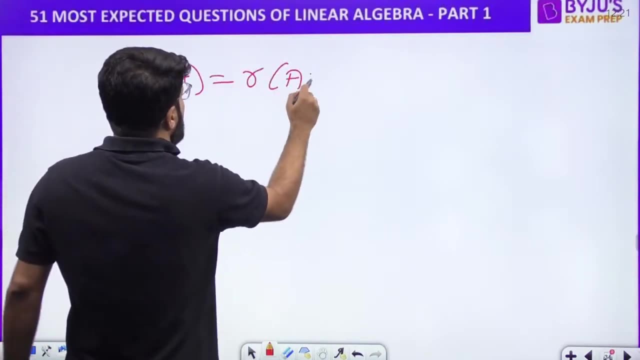 for question- and this is a direct trick for unique solution. the method says rank, but i will never use the rank for unique solution. i am going to make it simple for unique solution. i am going to make it simple: forget whatever is written, forget okay. for unique solution. rank of a equal to rank of a. 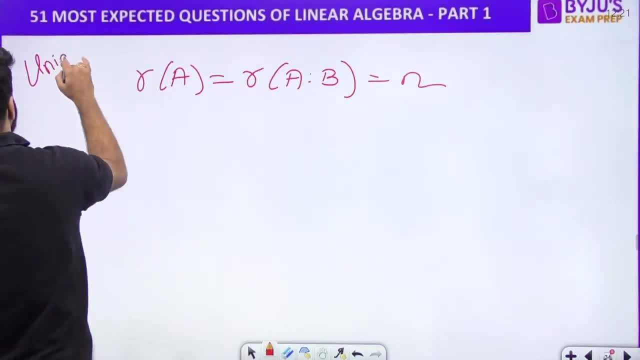 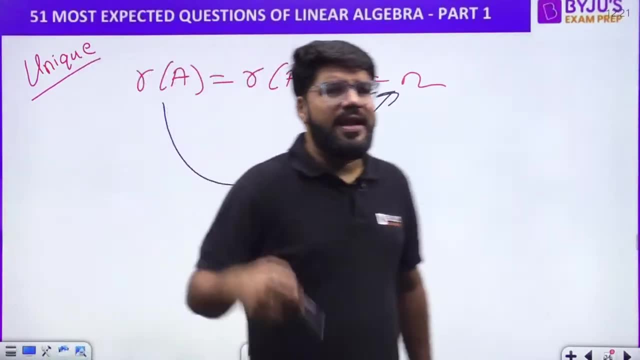 is to be equal to n. that is what is the condition for unique solution. if this is the condition dear for the unique solution, all the three are equal. so, eventually, rank of a is equal to n. eventually, rank of a is equal to n. a is a, n cross n matrix. 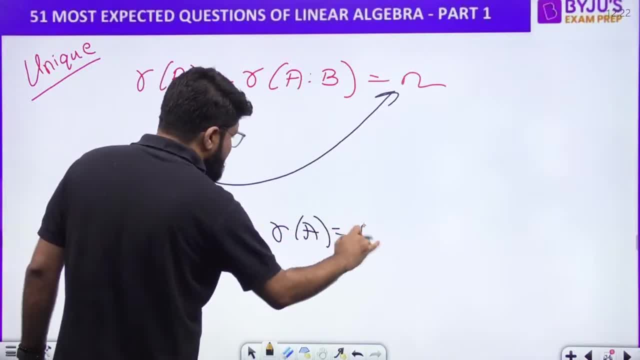 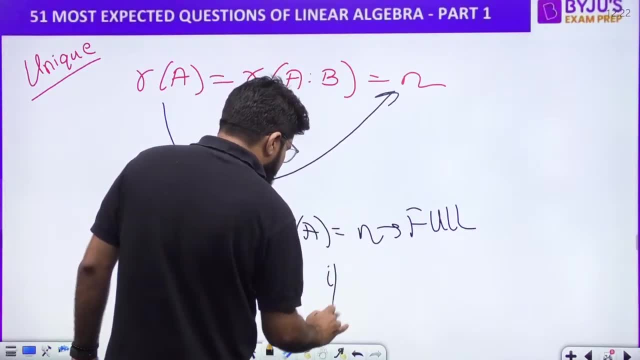 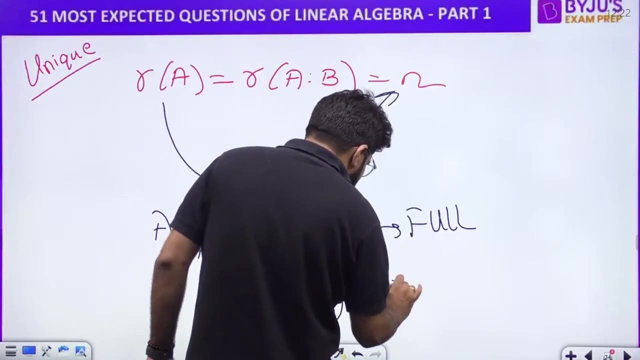 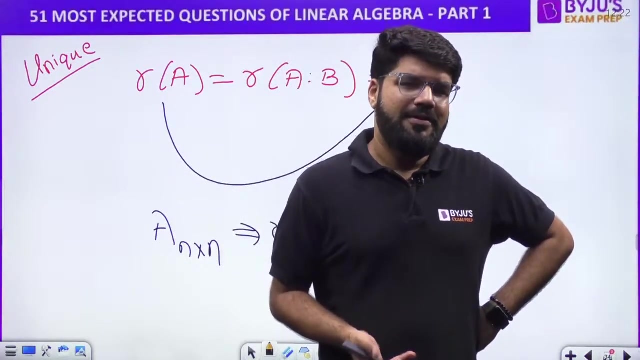 rank of a is equal to full. n matlab full right rank equal to full. if, if the matrix is non-sense singular- the very first thing we have studied today- only if the matrix is non-singular right. so for unique solution you only have to check: determinant baba: no rank. this comes to a. 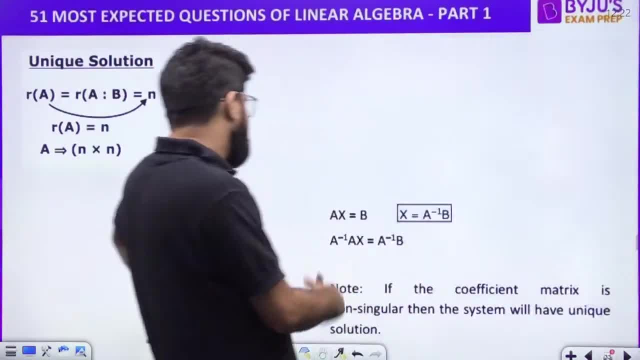 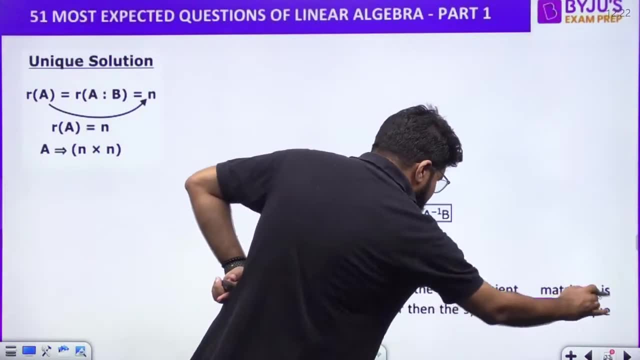 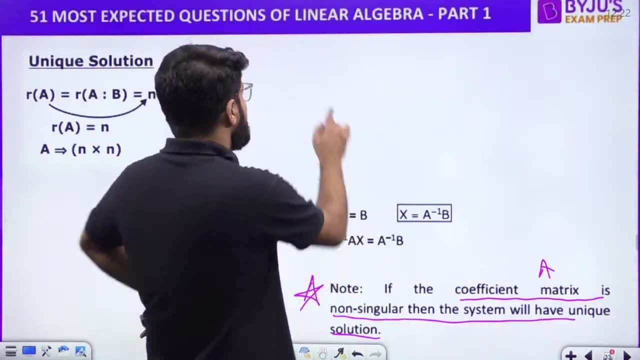 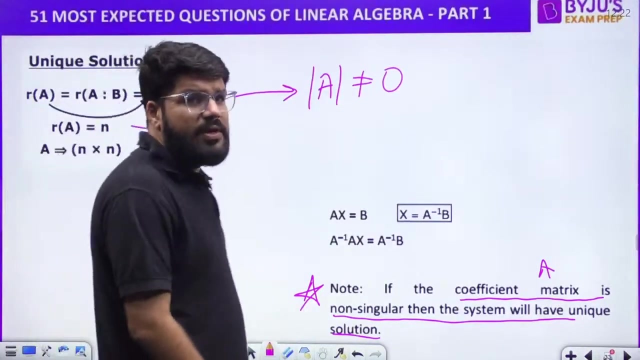 determinant question. this comes to a determinant question. same thing i have written here, right. same thing i have written here. okay, if the coefficient matrix, which is a, if the coefficient matrix is non-singular, then the system will have unique solution. if the determinant of a does not equal to 0, now right. if the determinant of a does not equal to 0, then the inverse will. 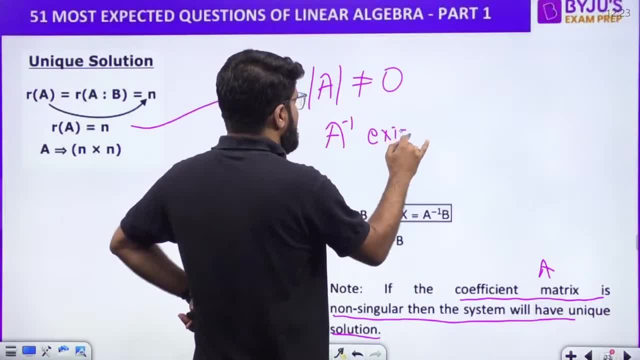 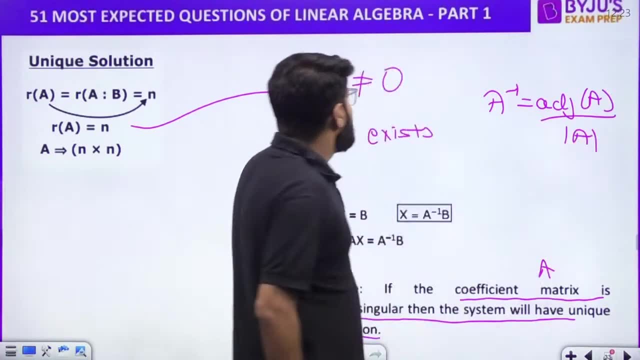 exist, then the inverse of the matrix will exist, because a inverse is given by the formula adjoint a divided by modulus of a. so if the determinant of the matrix is non-zero, then you can also calculate the inverse of the matrix. and if you can calculate the inverse, 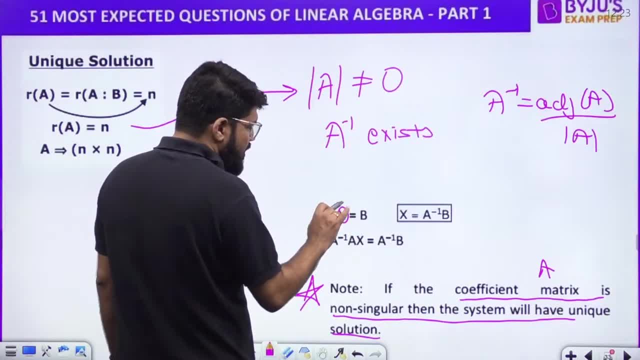 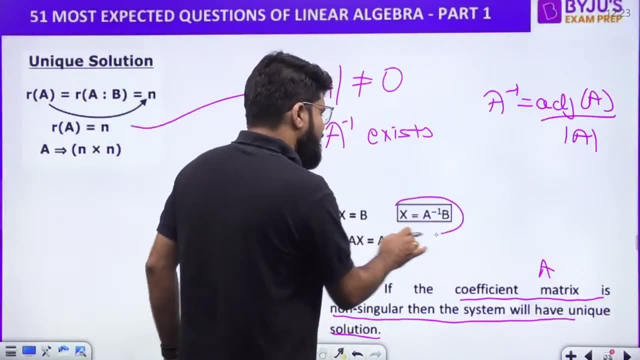 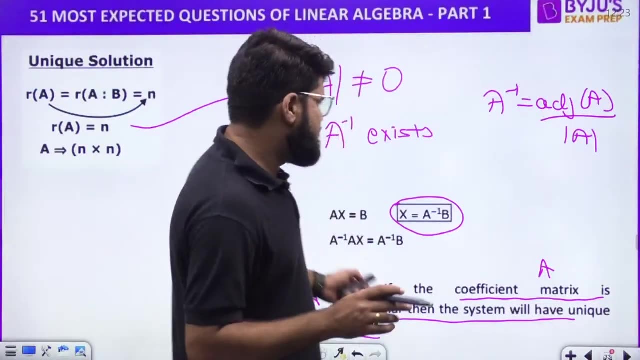 of the matrix. you can also determine x, ax equal to b. so x will be a inverse and x will into B. X will be A inverse into B. But I told you 99.9% chance. they are not going to ask what is X, what is the XYZ variable. They only try to test whether you know to. 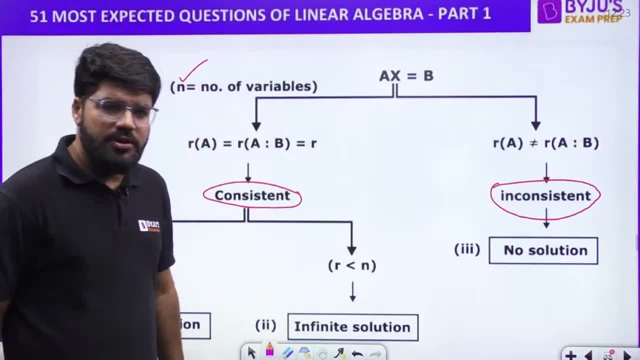 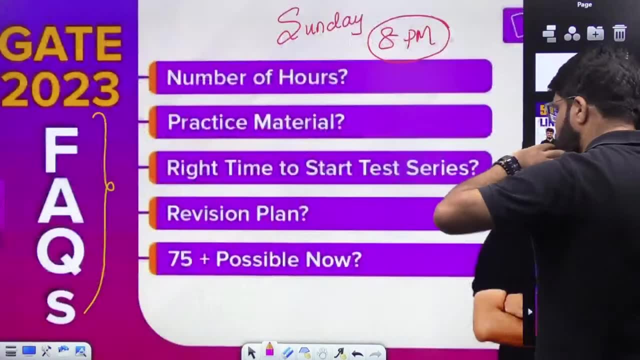 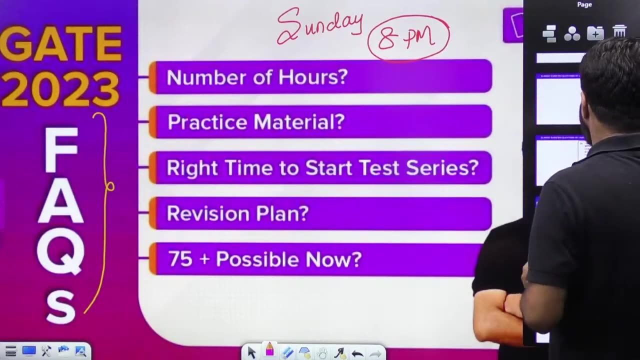 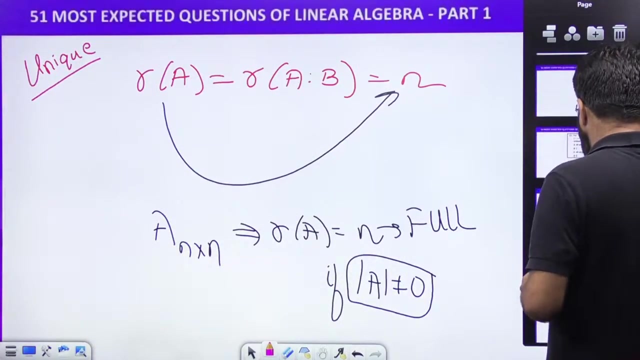 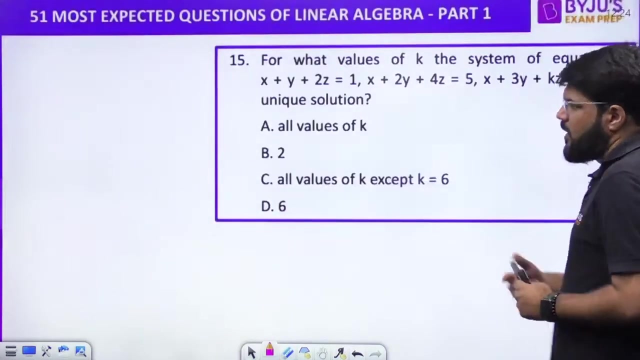 determine: unique solution, no solution, infinite solution. Now let us turn back to a question. Okay, let's do a little mixing of questions here. Just wait for a moment. Oh, slightly mixed the questions here for better understanding. yeah, 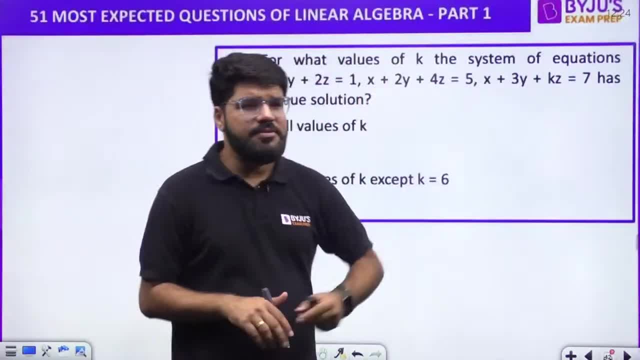 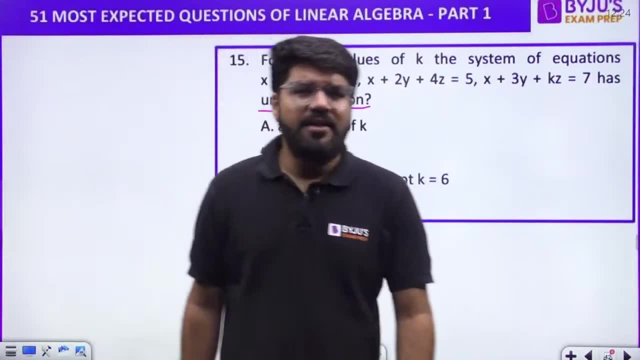 So kindly take this question. I will just mix. don't worry about the names, that would be okay. Only one numbering all 51. we complete karenge, but i'm just mixing the questions here. for what value of k, the system of equations has unique solution. so starting with the simple one, starting with the simple one. 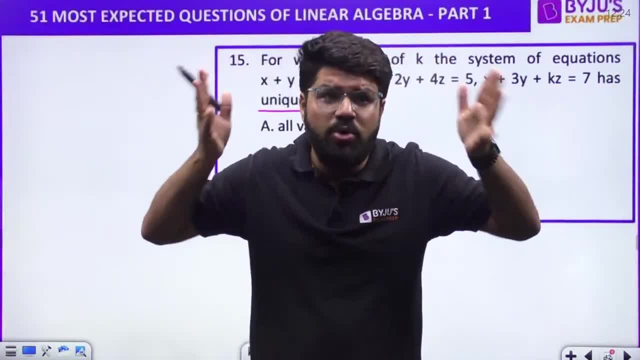 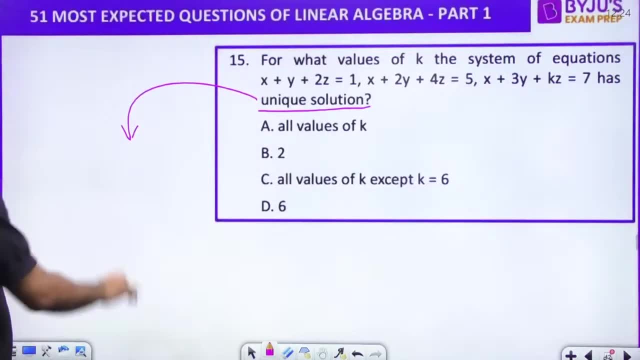 unique solution ke liye. condition batao to unique solution is very simple, the most simple, the most simplest, the most simplest: determinant of a does not equal to zero right. so determinant bole to 1, 1, 2. determinant of what coefficient matrix? so only write down the coefficients of x, y, z, so 1, 1, 2, then you have. 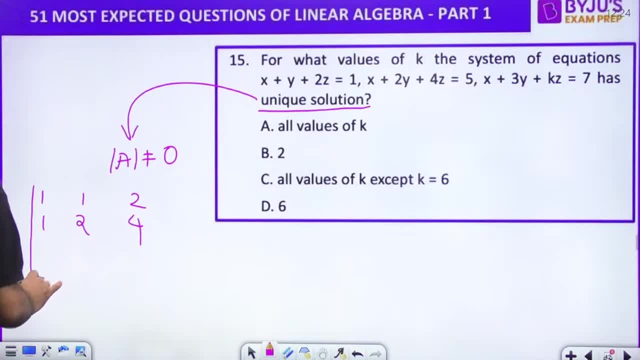 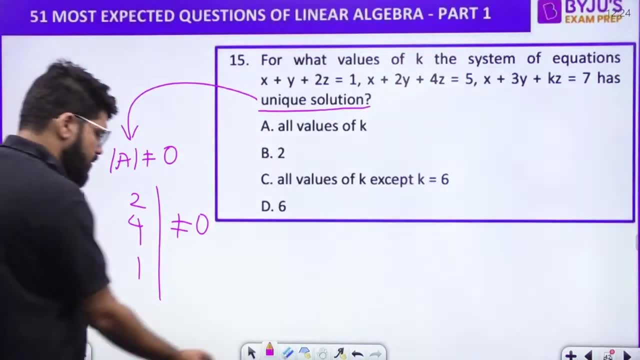 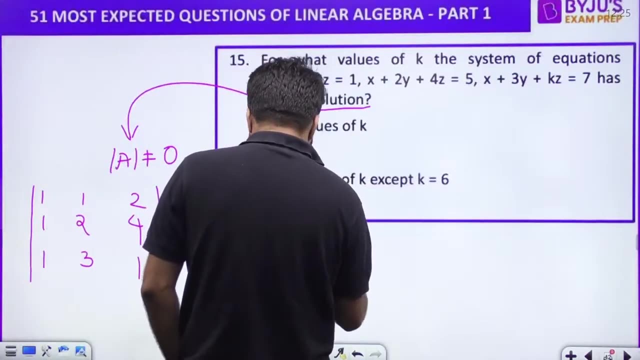 1, 2, 4. you have the 1, 2, 4. you have then 1, 3, 1, the 1 and 3 and 1. this should be not equal to 0. this should be not equal to 0. okay, so kitna hua, 1 into 2, minus 12, minus 1, right into. 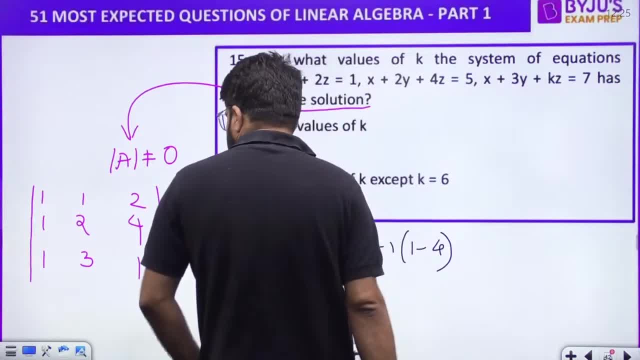 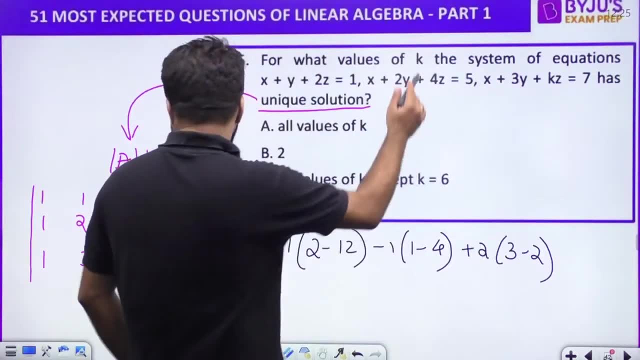 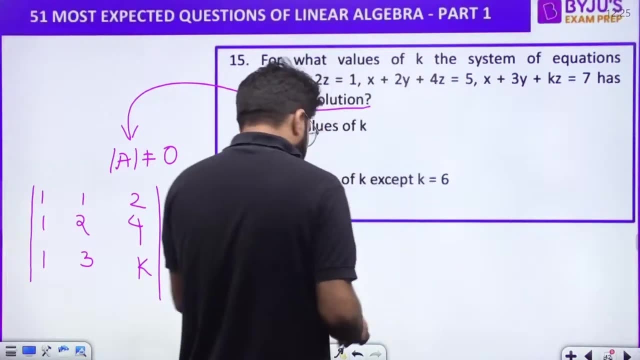 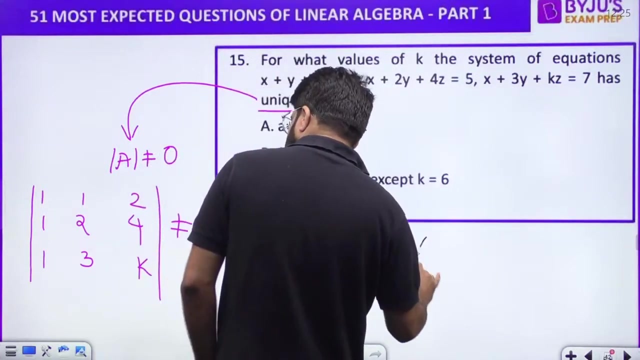 1 minus 4 plus 2 into 3 minus 2. this should not. where is the k? i'm sorry k sorry, sorry ye k miss hua this k i have missed out. okay, just a moment, that is how i felt. calculation me chala gaya. okay, so i'll just redo the calculation: 1 into 2k minus 12 minus 1. 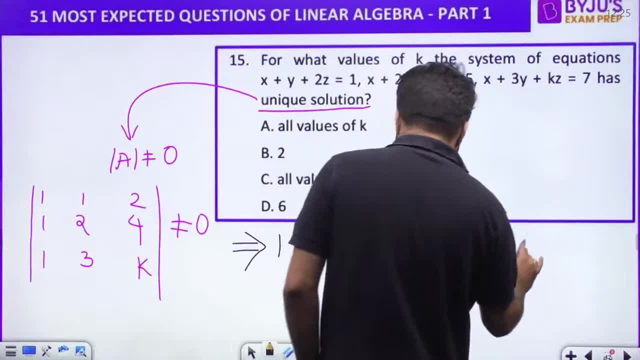 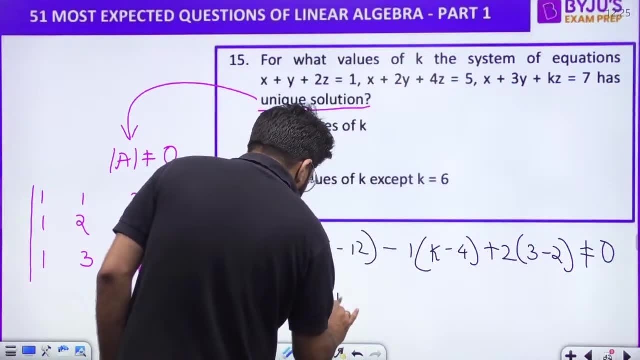 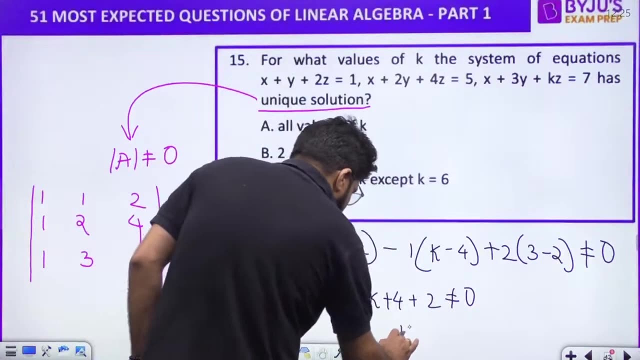 into k minus 4 plus of 2 plus of 2 into 3 minus 2. this is not equal to 0. so this means 2k minus 12 minus k plus 4 plus 2 does not equal to 0. so this is going to let 2k minus. 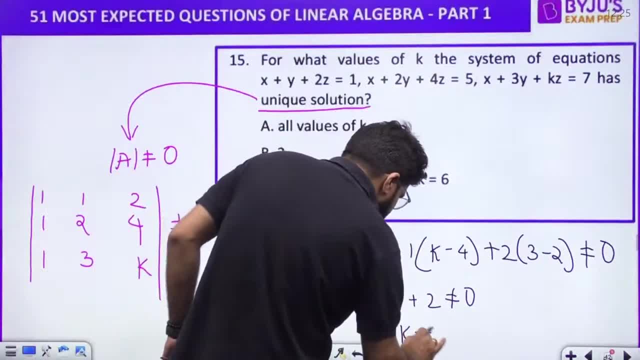 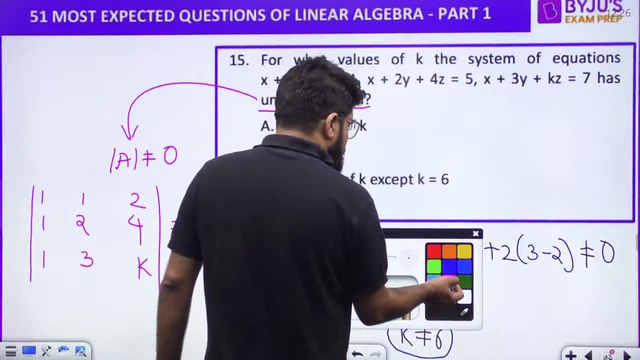 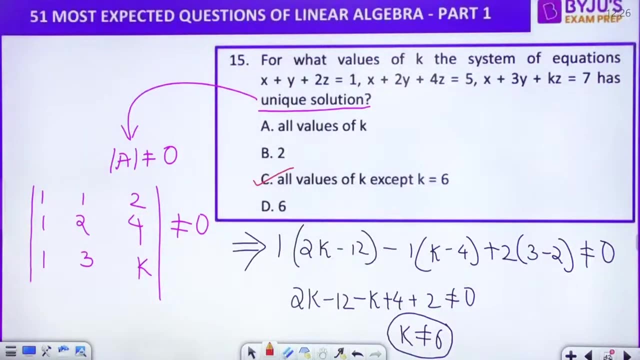 k is k and this is not equal to 6. k minus 6 bacha to k does not equal to 6. what is the correct answer then? all values k can take any value, but it should not be 6. so all values of k except 6. this is the simplest question and this is a type of expected question for 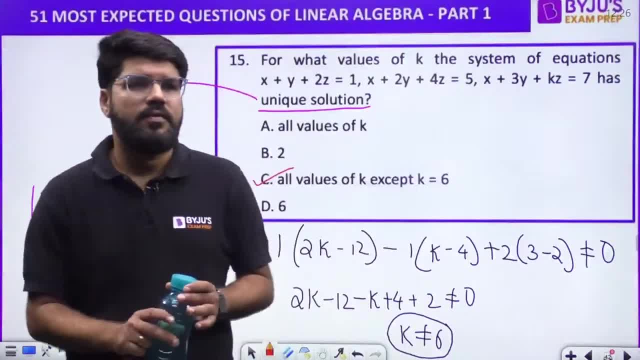 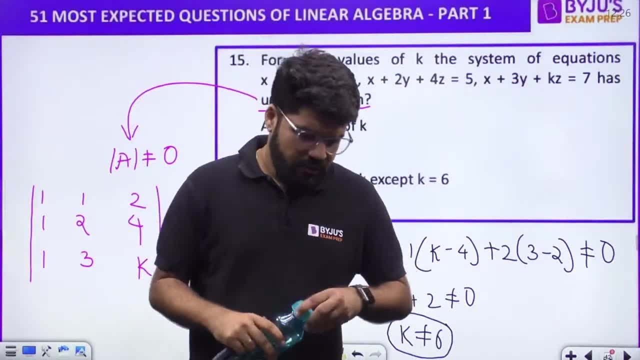 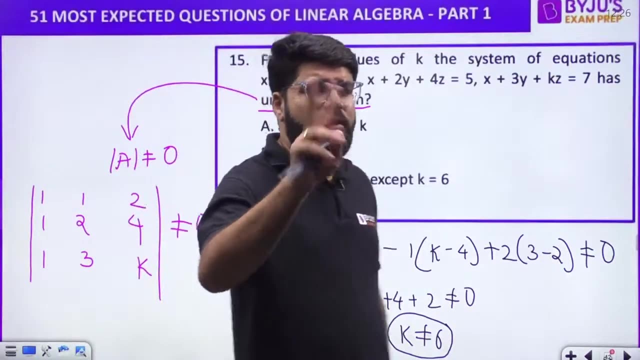 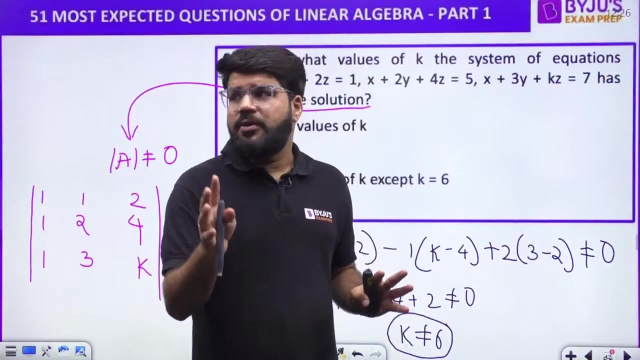 what value of k the system has unique solution. moving ahead to the next right? no, no, today 51 total 51 questions into two parts. hania: total 51 questions of linear algebra, where today i will cover rank and system of equations. system of equations means non homogenous, also homogeneous. also tomorrow i will cover very 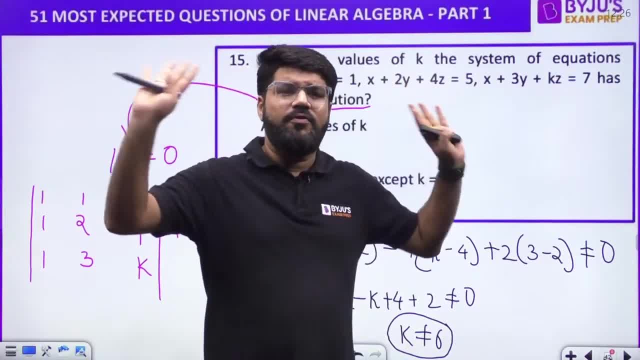 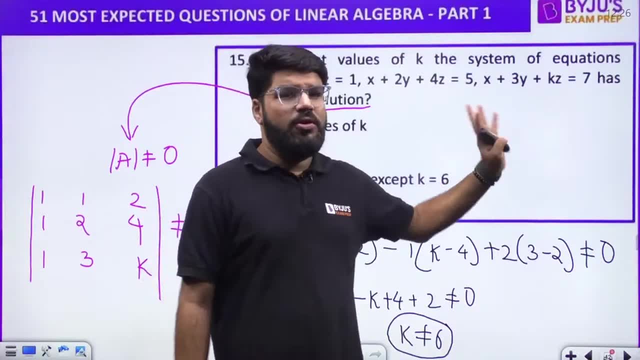 very important: eigen value, eigen vector. combining today and tomorrow: 51 questions, only 5 questions questions right. So today around 25, I don't know exact. I made the PPD morning only but I don't know what is the exact number, but somewhere around 25, 27 questions will be today. next will: 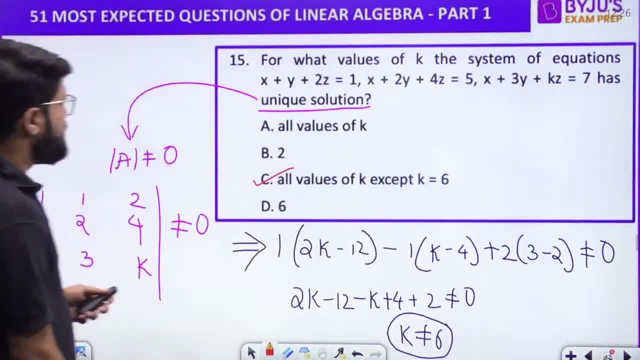 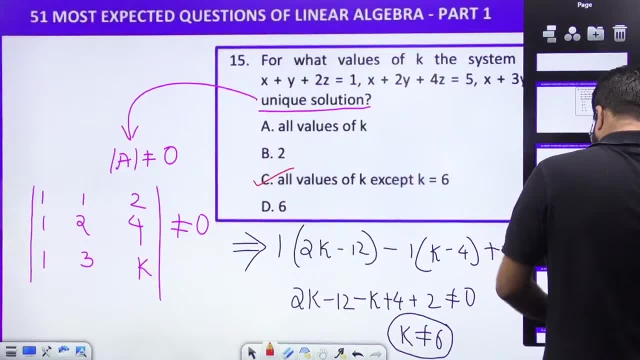 be tomorrow. okay, So total 51 of algebra: okay, So k is not equal to 6, this is one simple question. okay, dear, This is one simple question. now let me shuffle up. yeah, let me come to this. 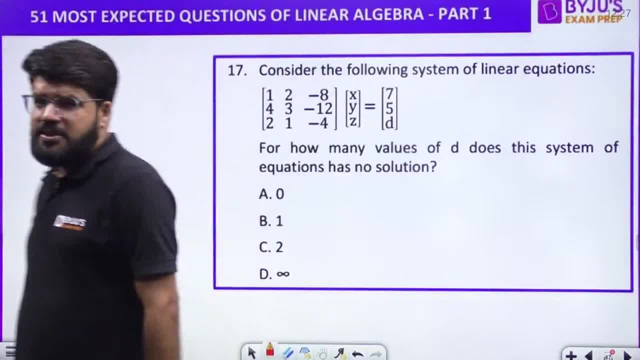 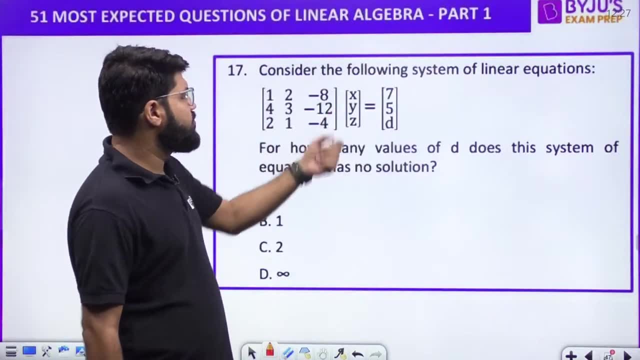 question now. Consider the following system of linear equations. consider the following system of linear equations: 1,, 2, minus 8,, 4,, 3, minus 12,, 2,, 1, minus 4, x, y, z is 7,, 5, d. How many? 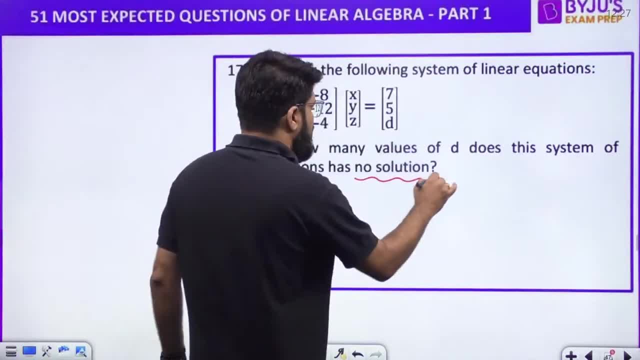 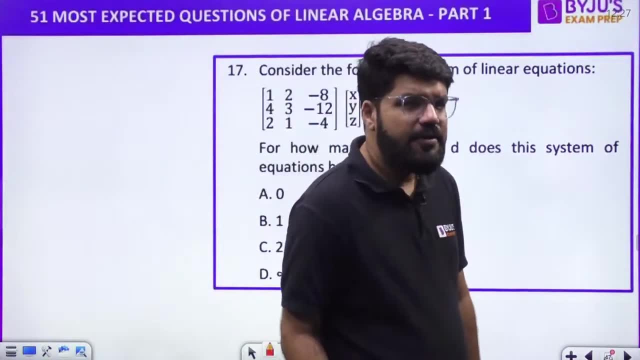 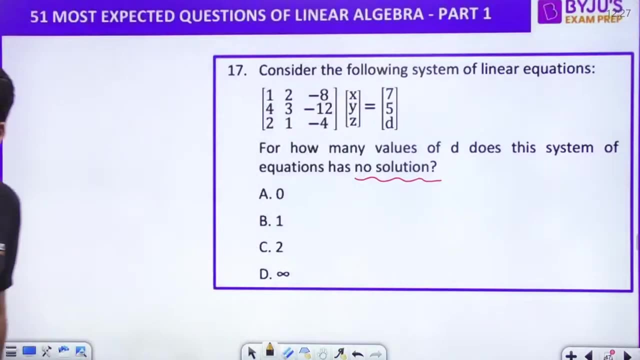 values of d does? the system has no solution. For how many values of d does? the system has no solution. For how many values of d does the system has no solution. right System has no solution, no solution. First of all, I will add on shortcuts also. let me just apply the proper method first. okay, First. 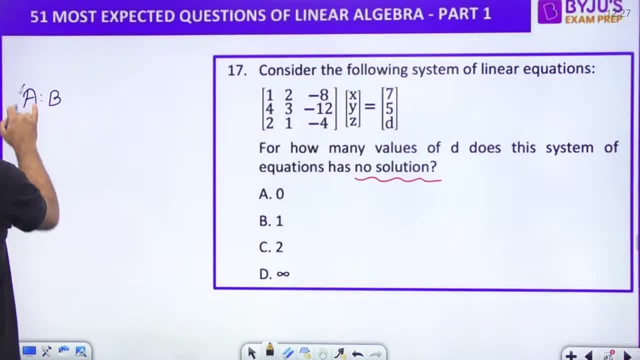 of all, let us take the matrix A is to B, and that is going to be the matrix: 1, 2, minus 8, 7, then 4, 3, minus 12, 5, and 2, 1, minus 4 is to D. that is what it is. okay, Okay, right. 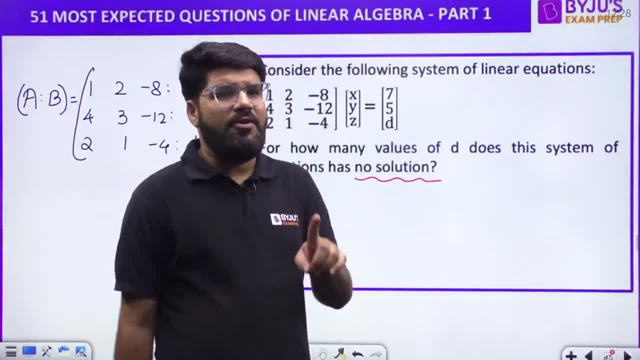 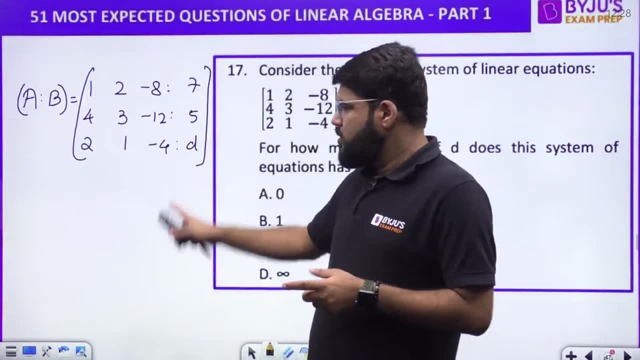 Now the system has no solution. if rank of A does not equal to rank of A is to B. I have written both the matrix together, because for rank here one of the value is unknown. So for rank I will go to Ecclain method. For Ecclain method we need to apply elementary transformations, elementary 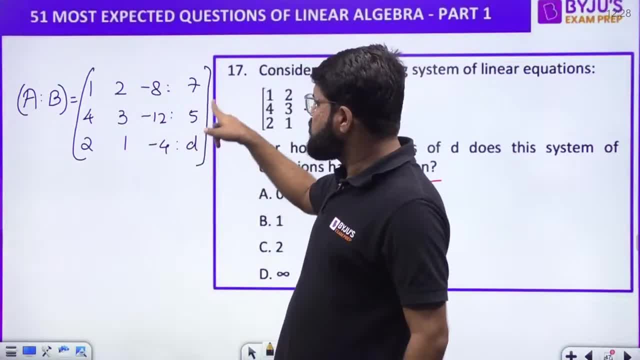 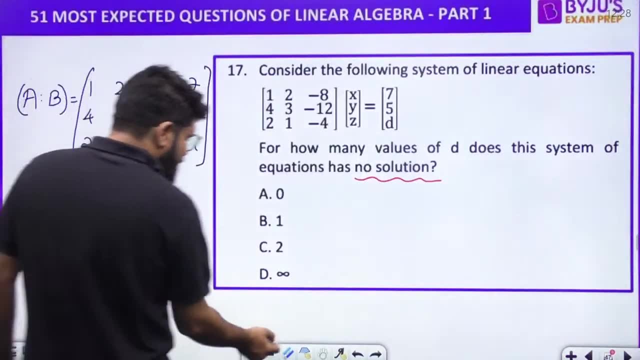 row operations, and if I apply elementary row operations on A is to B, automatically it is applied on A also. okay, So we will take it as only one activity. okay, Now, what do we have to do? First of all, I want to increase the number of zeros, so this has to. 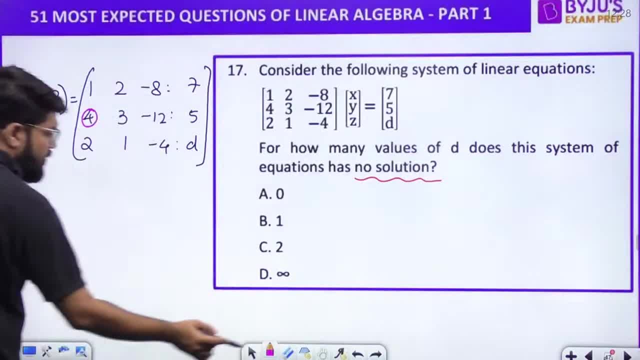 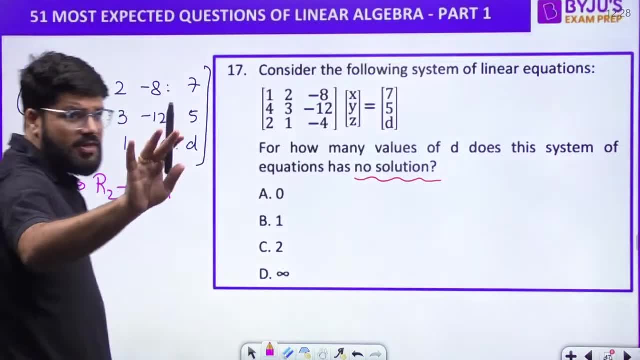 be 0,. this has to be 0, right? The first step that you are going to write is R2, is R2 minus 4R1,. after this, I will add the trick. okay, Just wait after this, I will add the trick. okay, And. 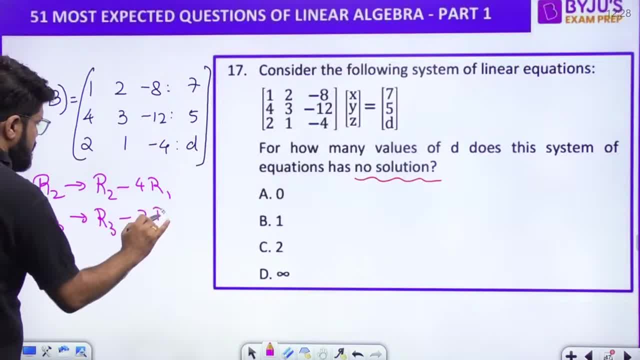 similarly, R3 will be R3 minus 2R1, R3 minus 2R1.. So how much is the A is to B? How much is the A is to B? 1, 2, minus 8, 7.. 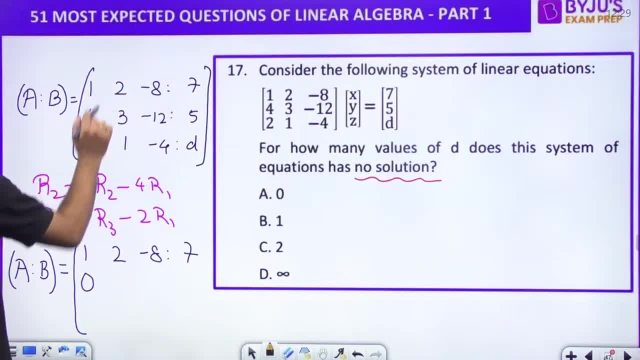 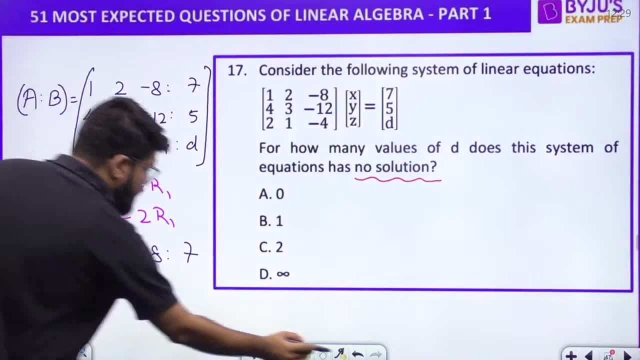 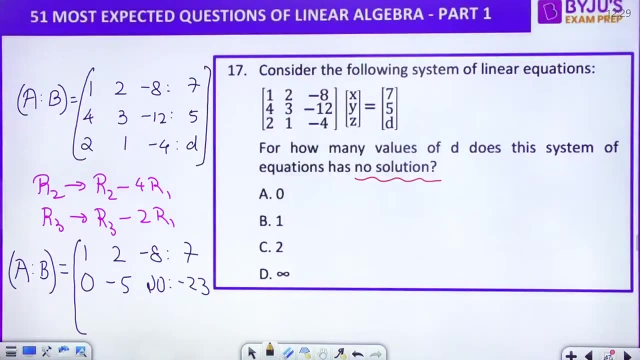 Right, 4 minus 4, 0.. 3 minus 2 into 4, minus 5, 3 minus 8.. This is also multiplied by 4, so minus 32, and this becomes total: 20 is to 5 minus 28 minus 23.. Some random numbers are coming. 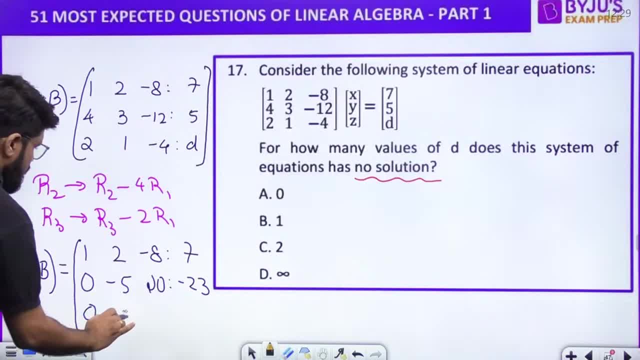 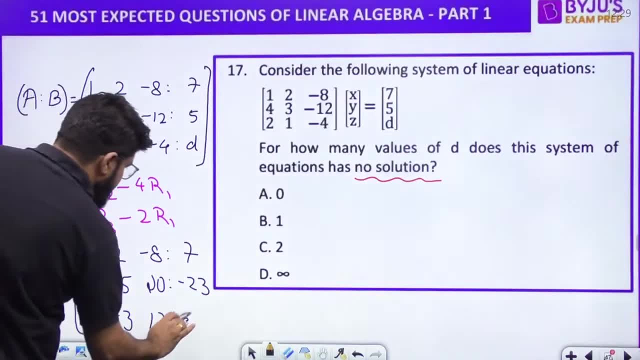 but no problem, we will deal with this. This is 2 minus 2, 0.. 1 minus 4, minus 3.. This is 2, so minus 16, and this is total left as 12, and then this is D minus 14.. 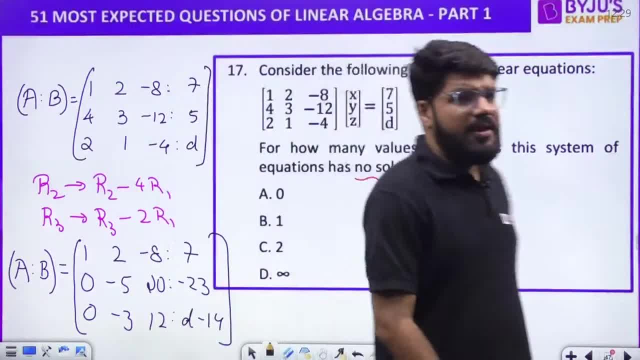 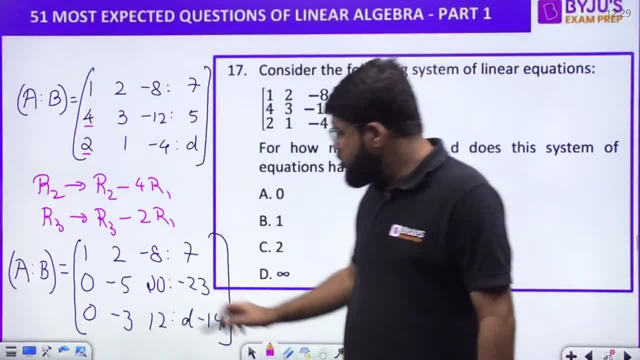 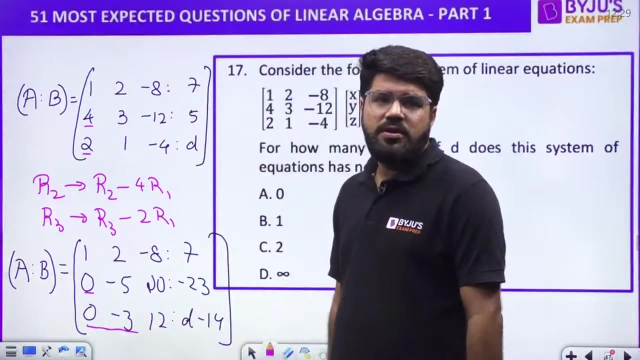 Okay, Now again to convert into the echelon form, dear, again to convert into the echelon form. now I want to increase the number of zeros. It should be increasing order. Here there is no zero, single zero. Then here I want two zeros, Here I want two zeros, right? So what is the? 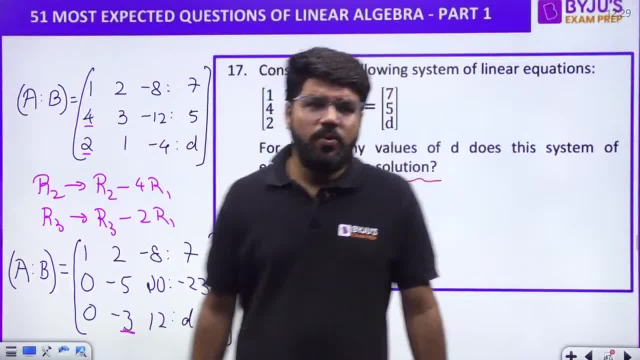 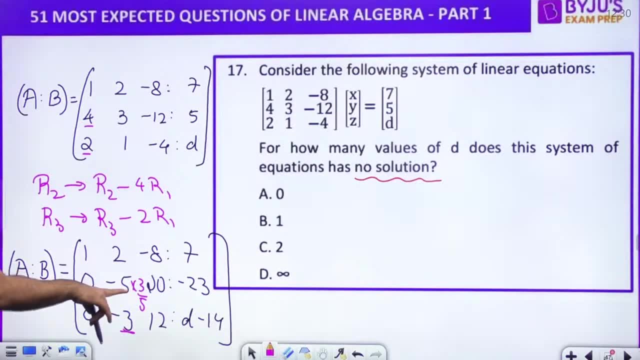 next number to be converted to zero. This is to be converted to zero, So what I will do, What I will do, This: I have to multiply by 3 by 5.. R2 has to be multiplied by 3 by 5,. 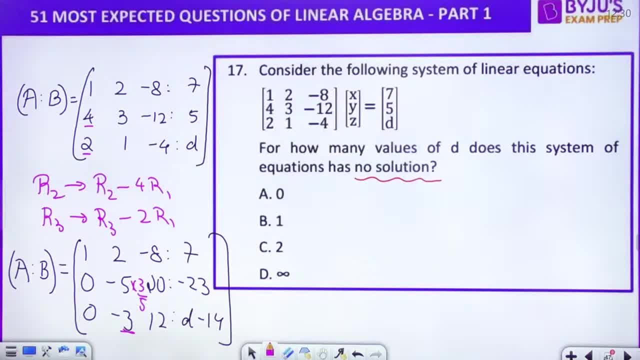 5 by 5.. Cancel, then minus 3, minus 3, same. Then you can subtract and you can make it as zero. Then you subtract and you make it as zero. So what is the thing that I am now going to do? 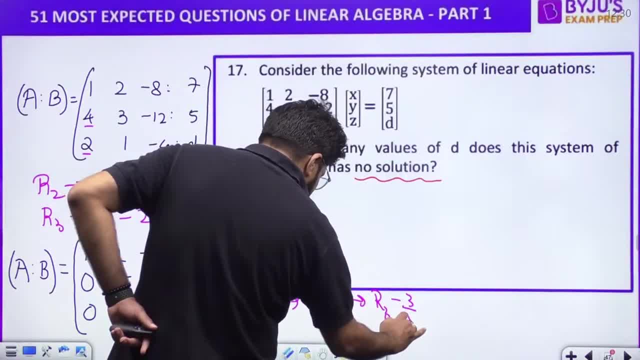 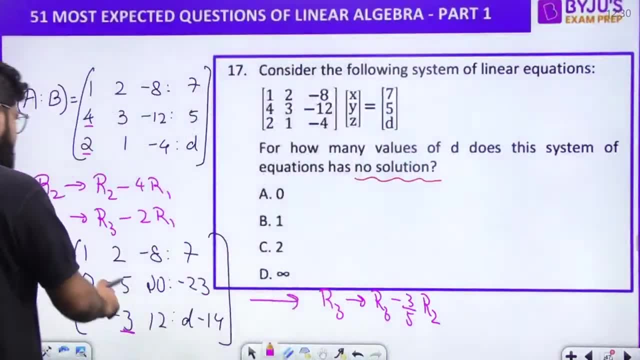 R3 will be R3 minus 3 by 5 R2.. Thoda sa teda calculation hai. but yeah, we have to be ready for, you know, sometimes unusual calculation also: R3 is R3 minus 3 by 5 R2.. So, doing this, how what I get? 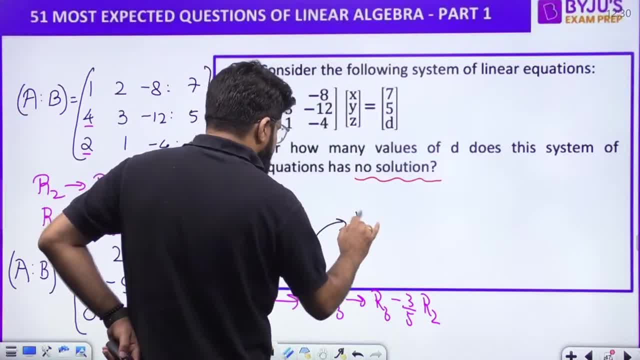 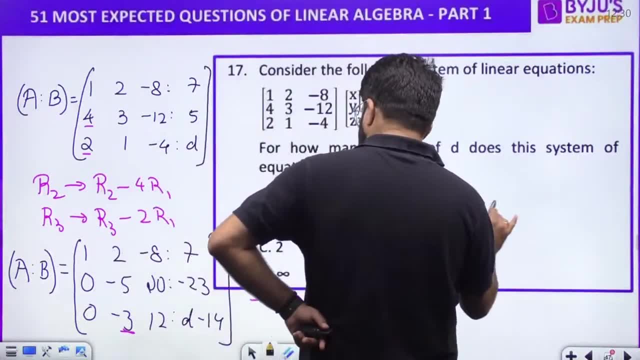 Doing this, how much I get After this? what is the matrix I am going to get? Let me write down here only. Let me write down the here only: 1, 2, minus 8, 7.. Then you have 0 minus 5, 20.. Just. 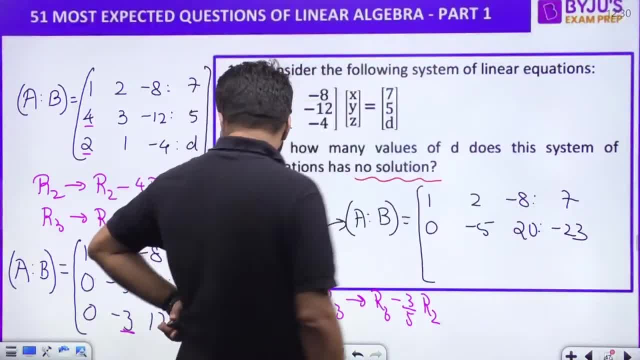 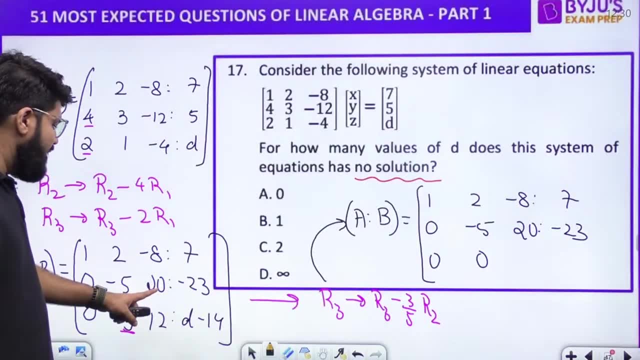 keep checking the calculation. okay, If there is any calculation correction you can also suggest me. Then this is zero. This becomes zero. Ab isko 3 by 5 se. multiply karenge. Multiplying by 3, fifth, it becomes 12.. It becomes 12.. So 12 minus 12.. This is also zero. Very good, Multiply this. 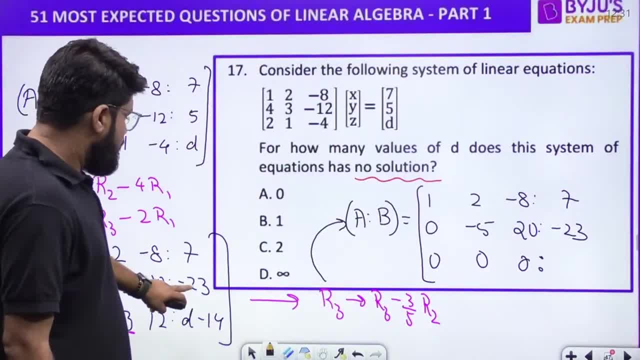 by 3 by 5.. Ye hai, Ye sahi to hai na Yeah, Multiplying this by 3 by 5.. See what you are going to get: D minus 14.. Minus 3 by 5 of minus. 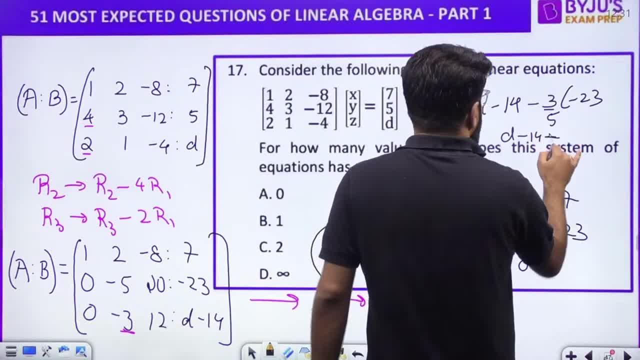 23. Minus, minus, plus, what. So D minus 14, and plus how much? Plus 69 by 5.. Okay, So you are eventually getting D minus. you have got 70 plus 69 by 5.. So D minus 1 by 5 actually. 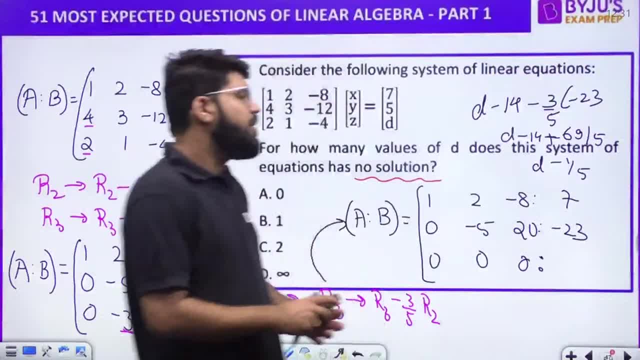 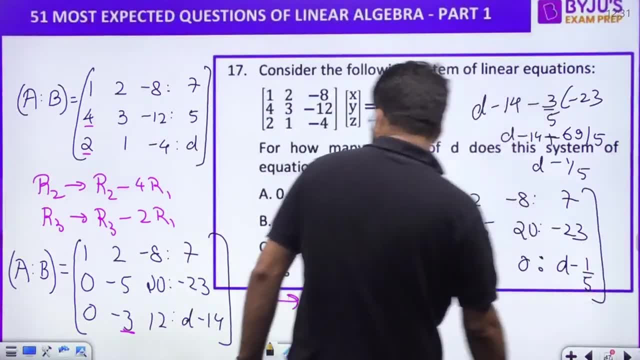 So you are going to get D minus 1 by 5 total, right? That portion is D minus 1 by 5.. So here, what I am getting is D minus 1 by 5.. What I am getting is D minus 1 by 5.. Clear everybody. 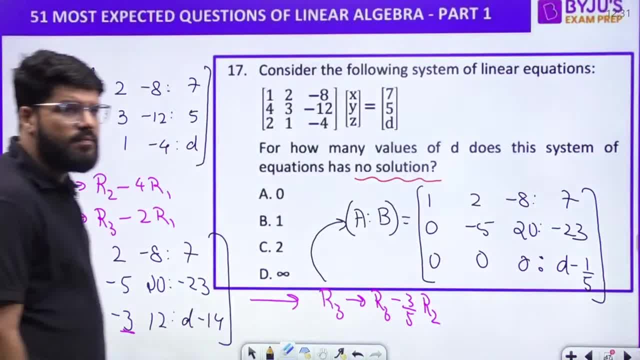 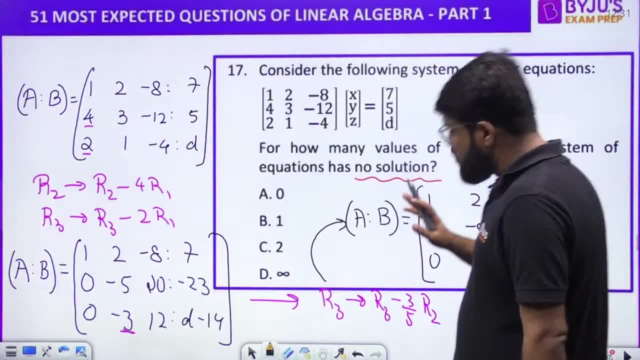 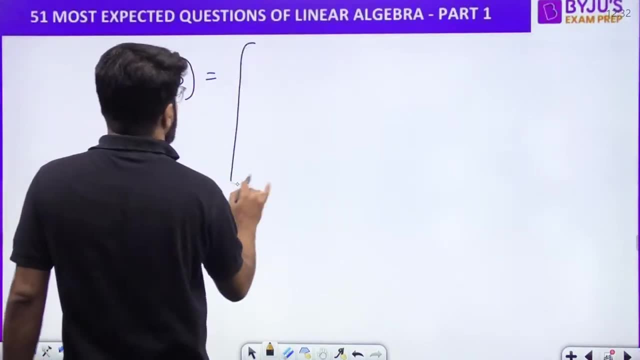 What I am getting here is D minus 1 by 5.. Okay, Now, how many values of D does the system has No solution. No solution. Now let me write down this matrix actually once again, So that I can. 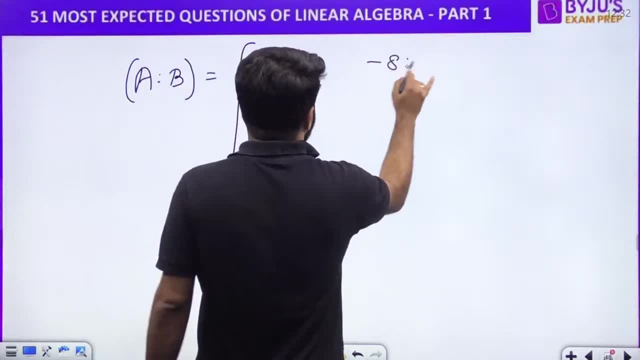 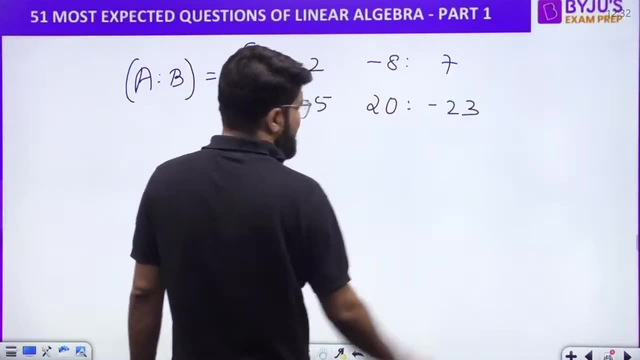 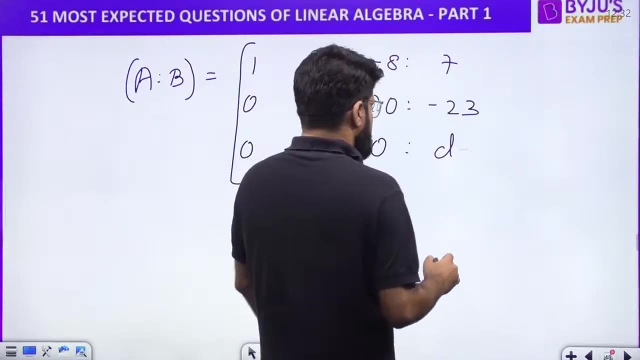 Explain you: 1, 2, minus 8, 7.. Check the calculations once. Okay, 1, 2, minus 8, 7.. Then you have 0, minus 5, 20.. Minus 23. Then you have 0, 0, 0, 0, 0, 0, D minus 1 by 5.. Everybody Now. 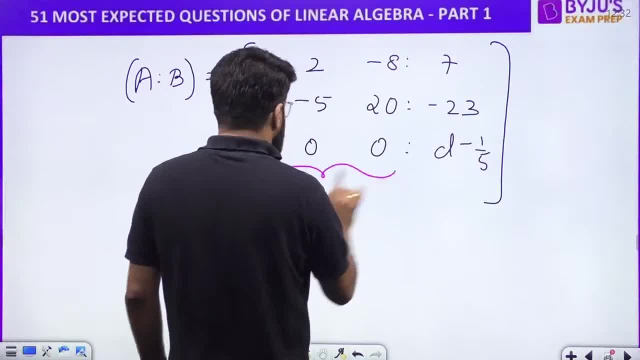 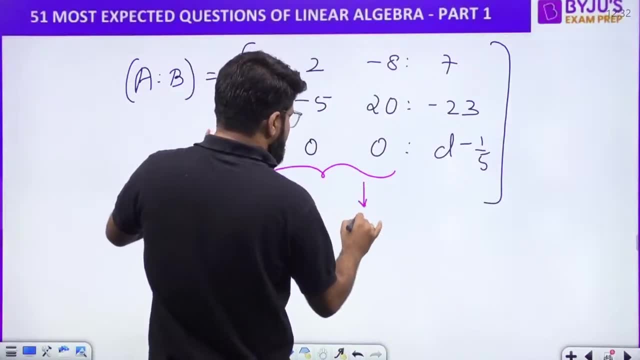 everybody. please track this matrix. This is the A matrix. This much portion is A matrix and this is the A is to B matrix. In the A matrix, in the A matrix, if I talk about number of 0s, it is nil, then 1,, then 2.. 0, 1, 2, right. 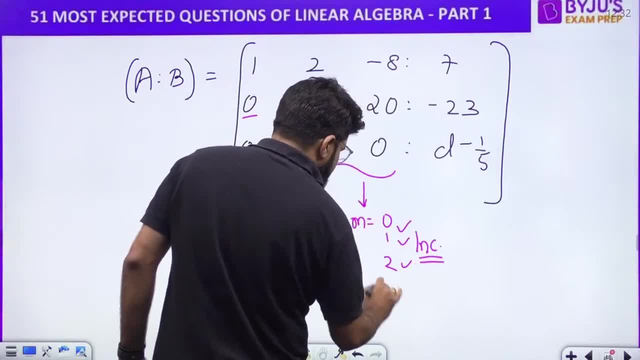 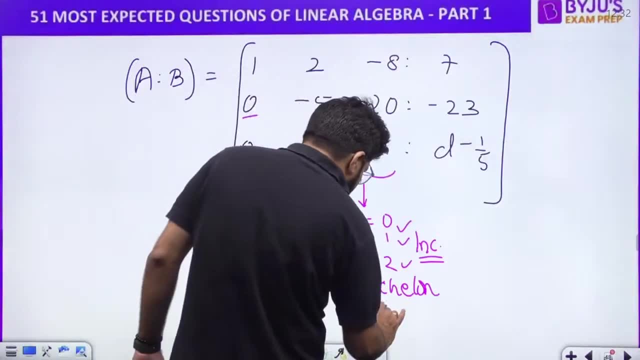 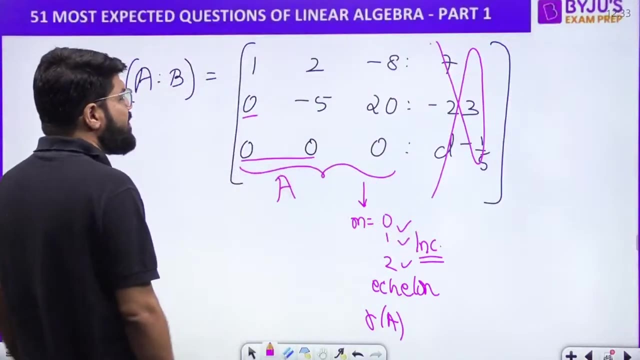 This is increasing. This is increasing. This is echelon form, This is the increasing form, echelon form. And if the matrix is in echelon form, rank of A is equal. to forget this For a moment, don't see this, Okay. So what is the rank of matrix? Number of non-zero row: This is 0.. 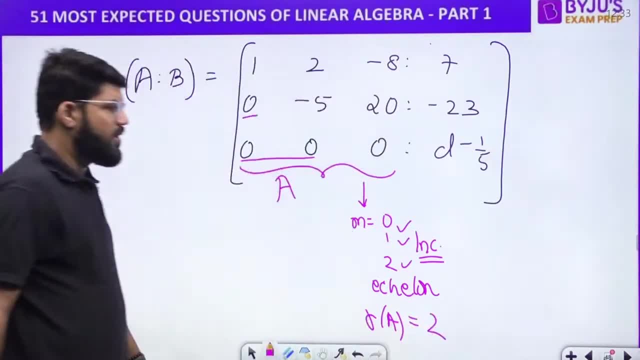 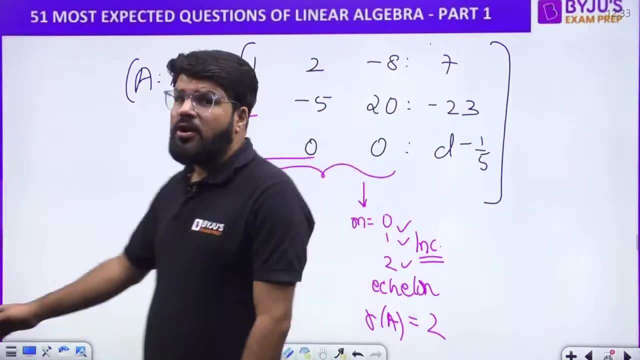 2 rows are non-zero. 2 rows are non-zero. Rank of A is equal to 2.. But what is the condition dear? What is the condition dear for no solution? The question is asking no solution. What is the? 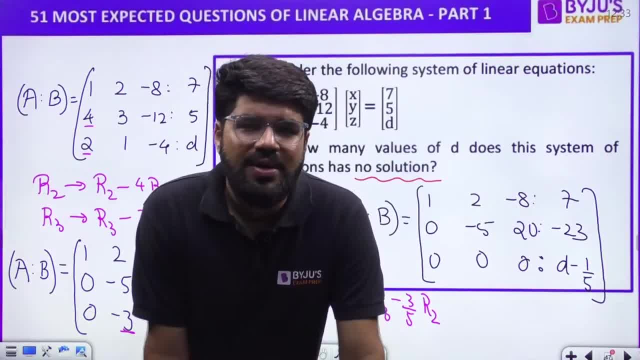 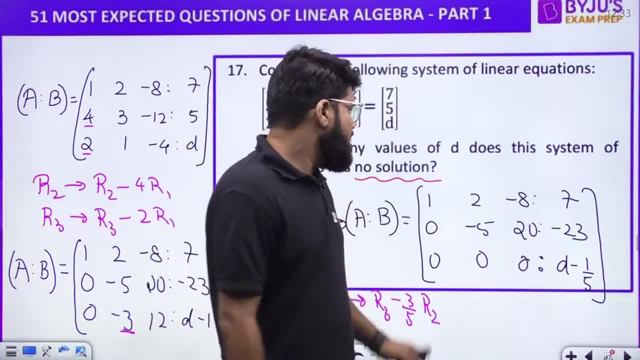 condition for no, no, no, no, no solution. What is the condition for no, no, no, no, no solution. Think about this. What should be the condition for no solution? The condition is: rank of A should not be equal to rank of A is to B. Okay, If rank of A equal to 2,. 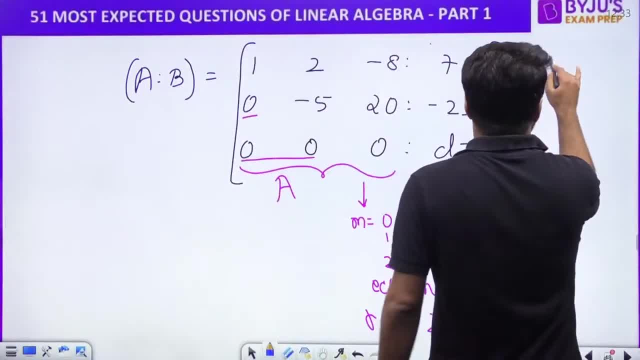 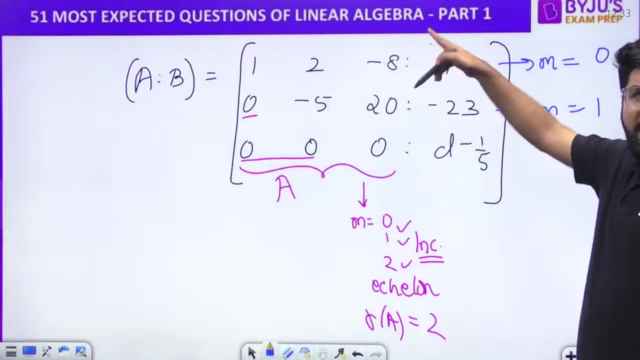 have a look into the M here. Have a look into the M here: 0.. Have a look into the M here: 1.. Overall M. Overall number of zeros in the entire A is to B matrix. What is the number of non-zero? 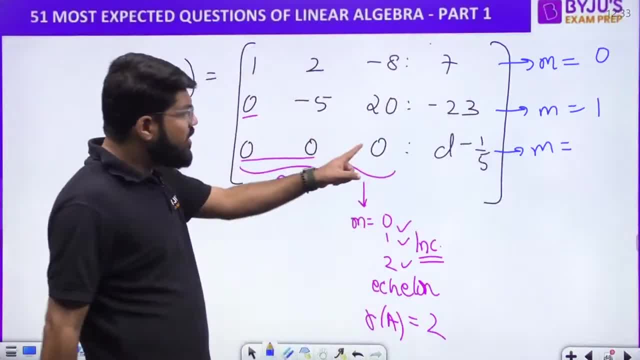 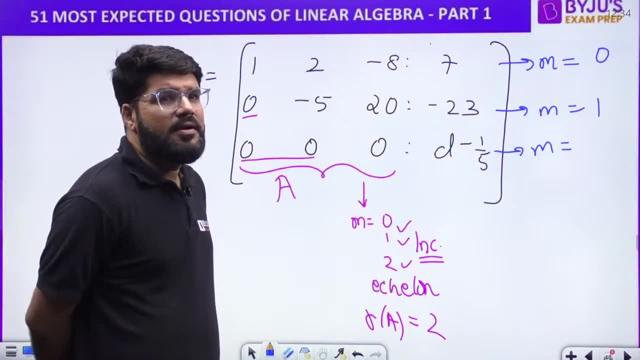 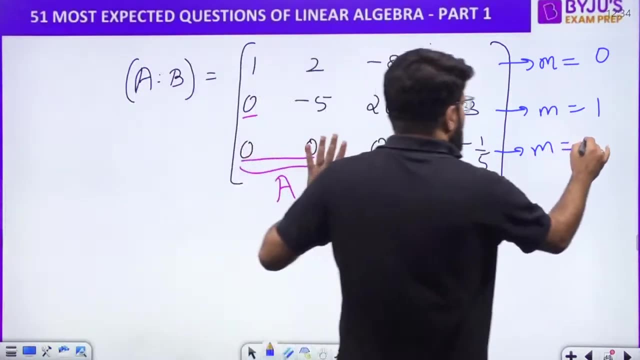 elements, Starting zeros here. What is the number of starting zeros? 3 to hai, 3 to hai, Right, 3 to hai, 3 to hai. But it can be fourth one as well. It can be fourth one. So minimum, 3. Right, Minimum, 3. Right Or 4.. Right now I am able. 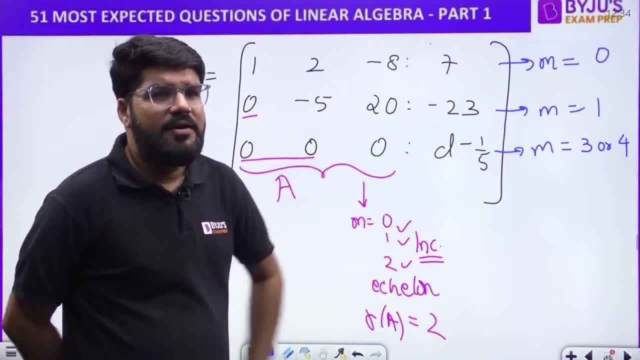 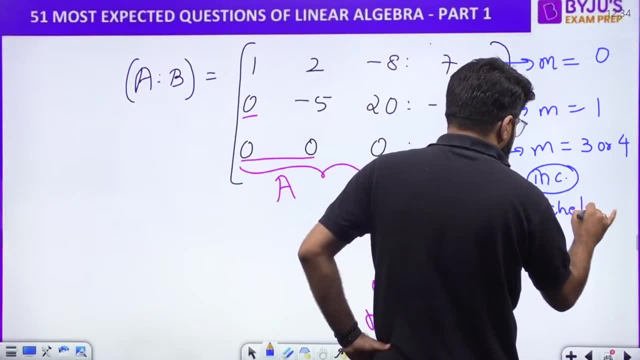 to see 3 or 4, depending on D minus 1 by 5.. Right, So echelon form to hai. This is clearly echelon form, Increasing trend hai. So this is echelon form, Right? So what is the rank? 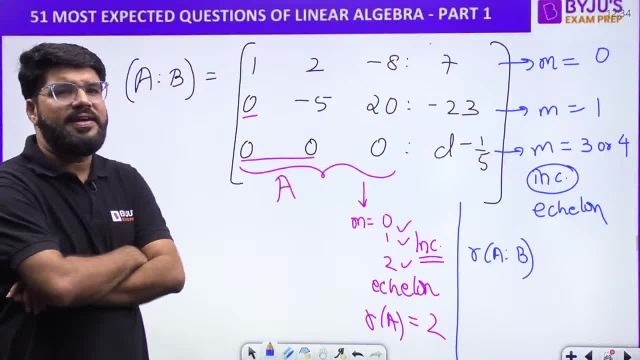 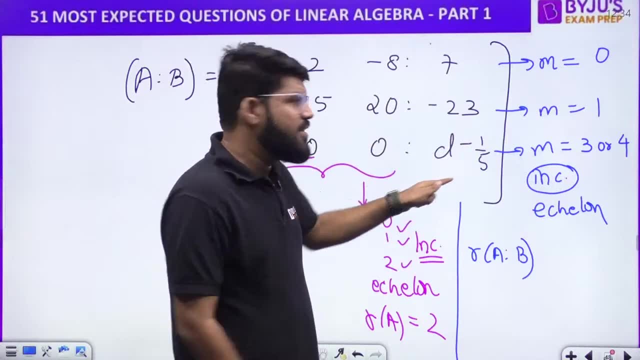 of A is to B. What is the rank? of A is to B. Number of non-zero rows. This is non-zero. This is non-zero. D minus 1 by 5.. Isko maine 0 kar diya. Then what do you get? Dekho Toh yaha pe dihan. 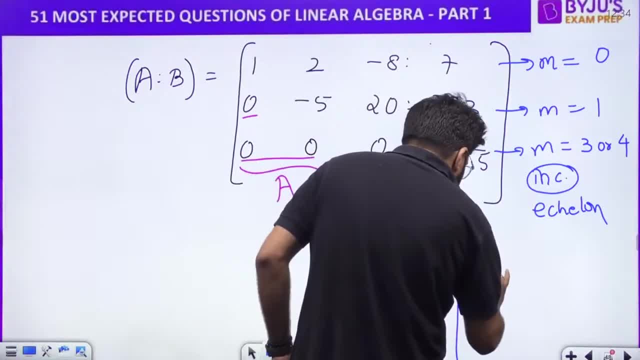 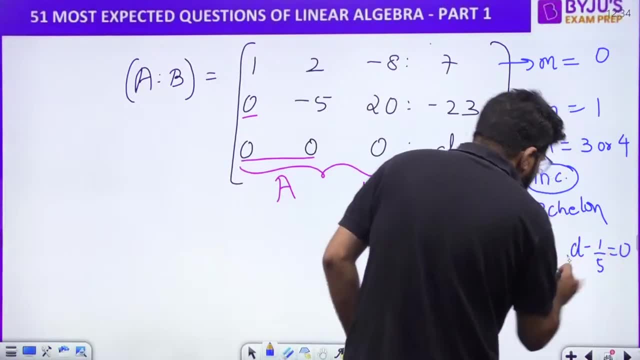 dena, I will write down clearly: Right Rank of A is to B Dear. If D minus 1 by 5 equal to 0. Then what is the rank Everybody understand? If D minus 1 by 5 is 0. This is row of 0.. 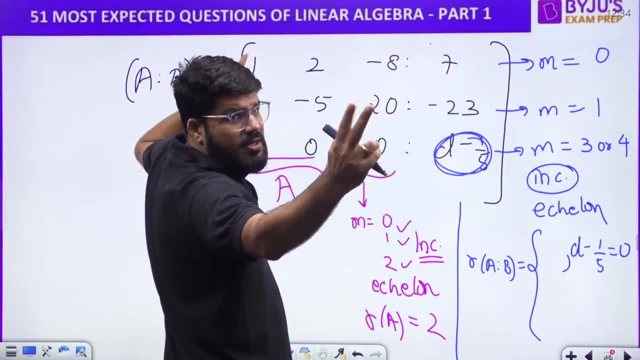 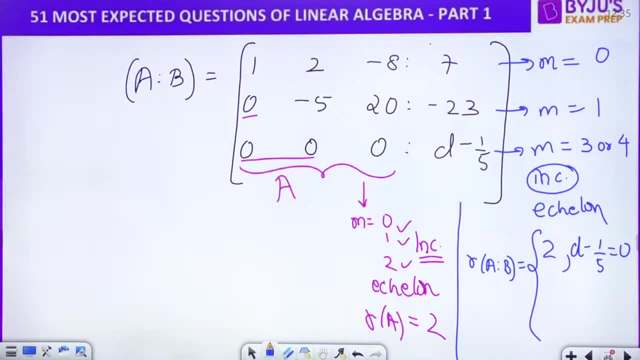 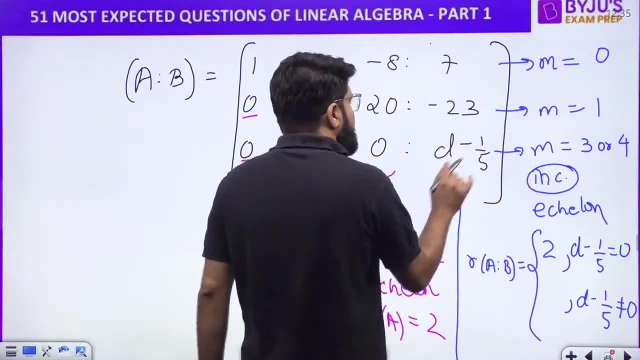 So how many non-zero rows? How many non-zero rows? There are 2 non-zero rows. There are the 2 non-zero rows, Everybody. But if D minus 1 by 5 does not equal to 0. Right, Suppose this is not equal to 0.. Suppose: 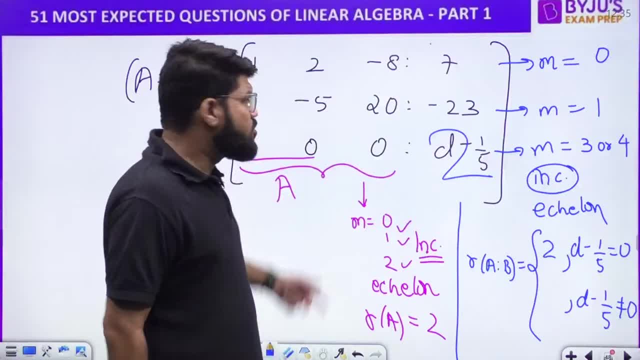 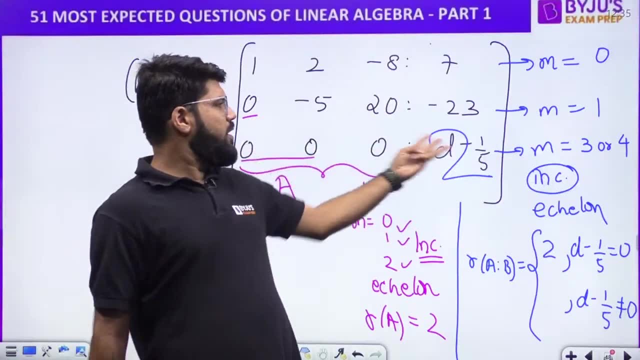 this is 2.. Suppose this is 2.. Toh, how many non-zero row? How many non-zero rows 1,, 2, 3.. Then all are non-zero. naa, Yeh bhi non zero ho gaya, Yeh bhi non-zero ho gaya, Correct? 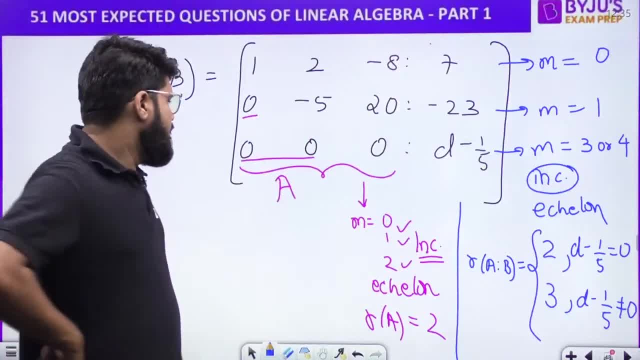 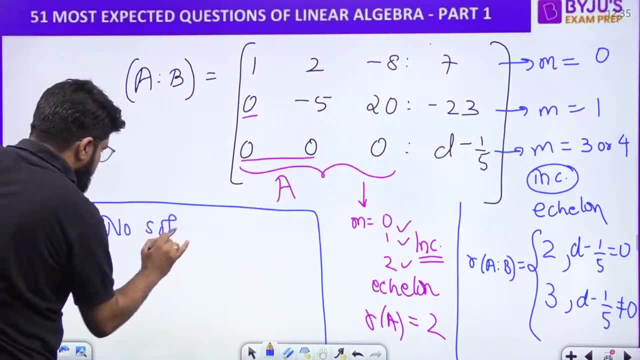 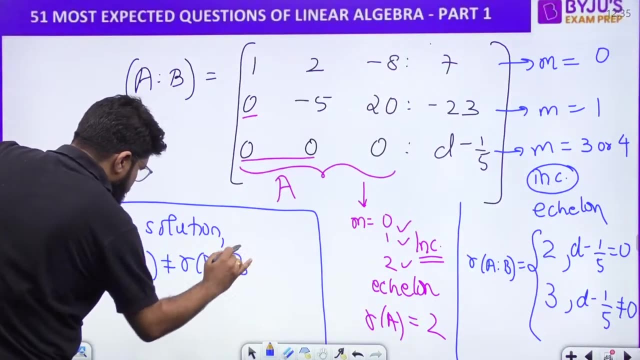 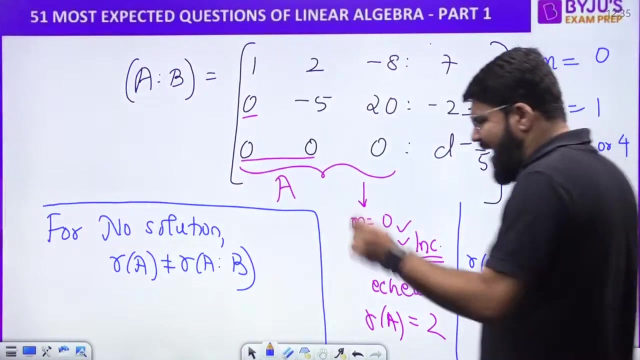 All are non-zero rows. Right Now the question is asking you no solution. You gotta get all solution For no solution for inconsistency of the system. rank of A should not be equal to the rank of A is to B. Rank of A should not be equal to the rank of A is to B Rank. 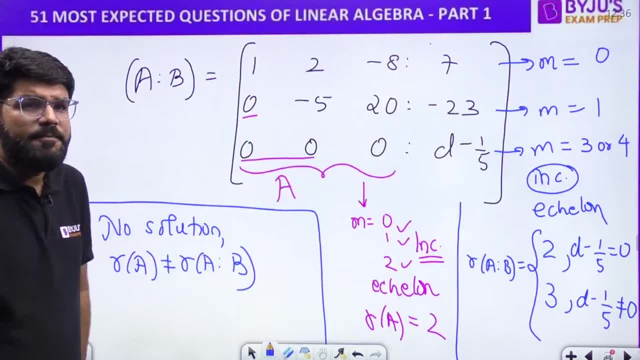 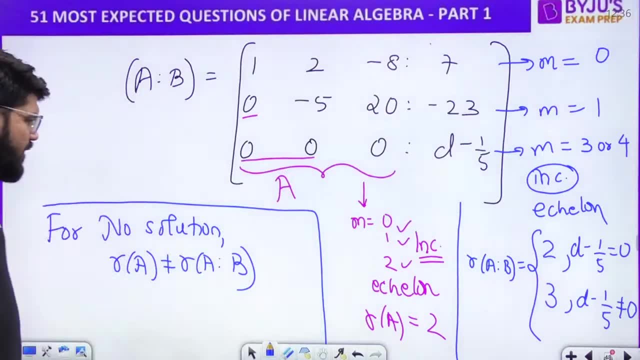 of A should not be equal to. rank of A is to B, Then what it should be. Rank of A should not be equal to rank of A is to B, then what it should be. Kya hona chahiye, Then what it is. 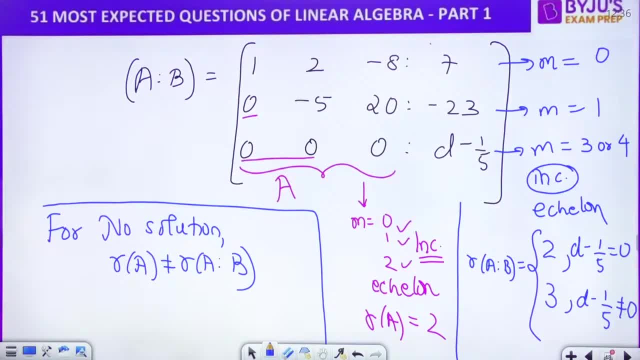 going to be. Have a look into this What it is going to be. Rank of A should not be equal to. rank of A is to B, so what it should be. Okay. Rank of A is 2, so rank of A is to B for non-equal. 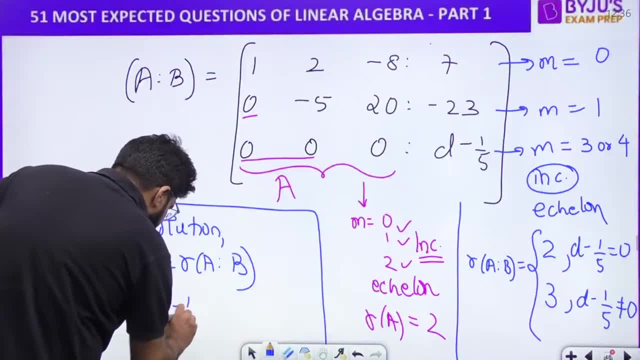 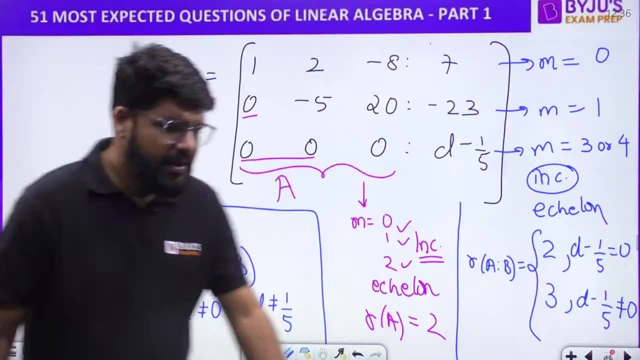 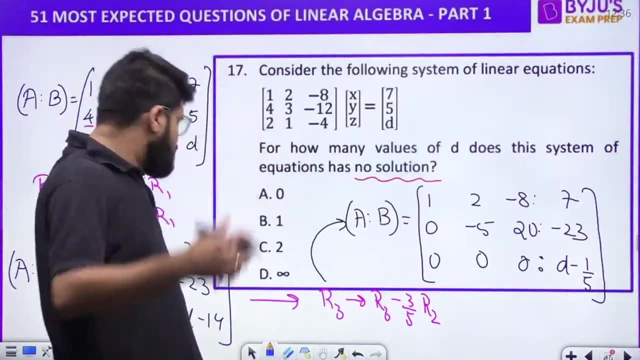 it should be 3.. That means that means D minus 1 by 5, not equal to 0.. So D does not equal to 1 by 5.. Correct: D does not equal to 1 by 5.. Right, So for question mein, kya bolo hai, How many values. 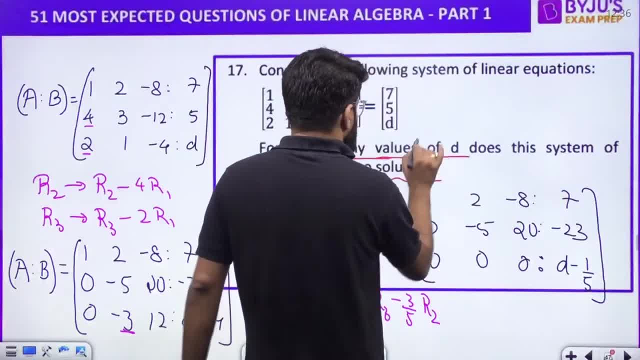 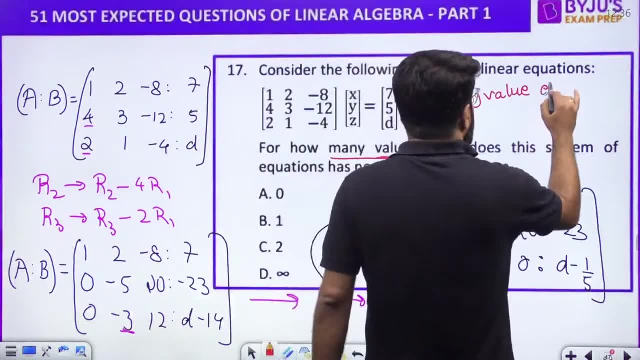 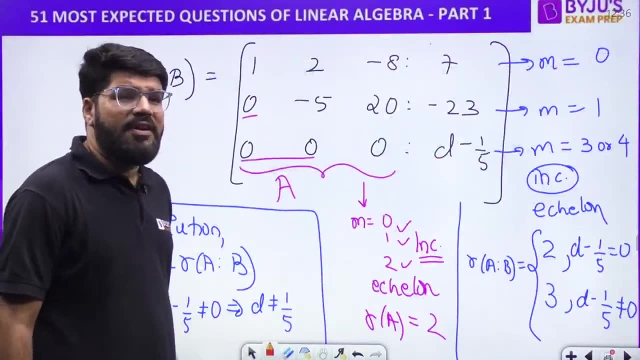 of D. Bhai answer kya, nikla, How many values So D can take any value. D can take any value except 1 by 5.. D can take any value except 1 by 5.. To except 1 by 5, how many numbers are there? 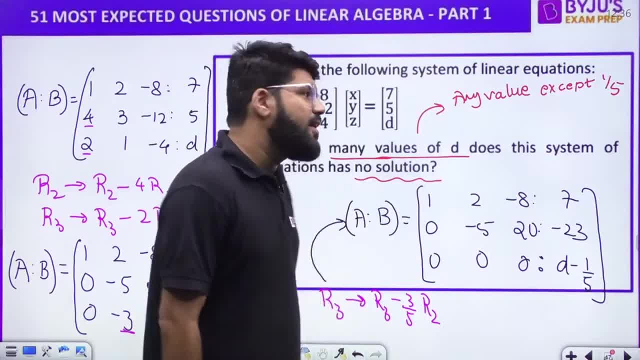 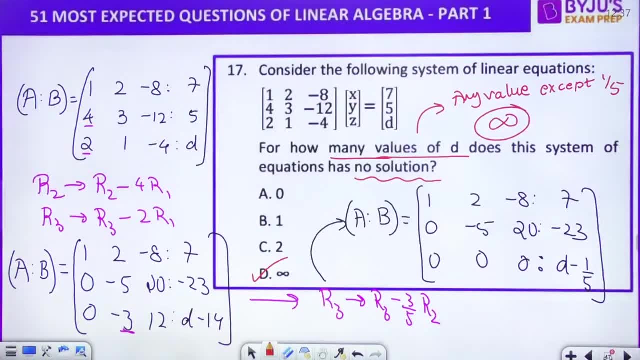 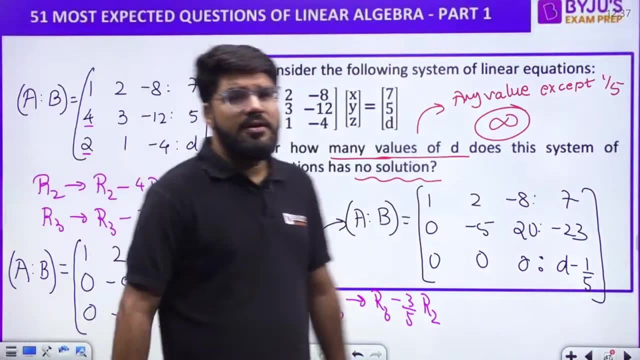 in the world. How many real numbers are there in the world. How many real numbers are there in the world? Infinite number of values are there in the world. Right, All okay, dear, All okay. This is what. This is what. This is how you should understand the problem. Okay, Let me add on one. 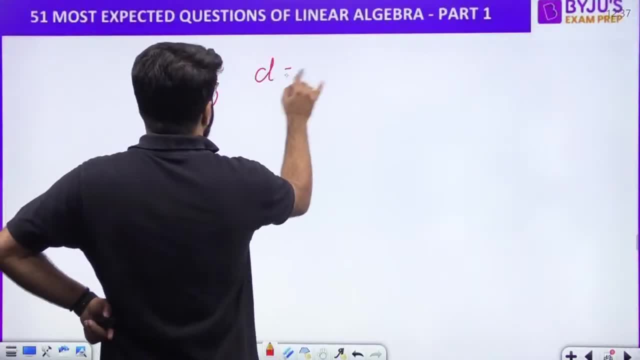 more thing here. Right, Suppose if D is equal to 1 by 5. If D minus 1 by 5 is 0 to D will be 1 by 5. Then the rank of A is equal to 1 by 5.. Right, So if D is equal to 1 by 5, then the rank of A is: 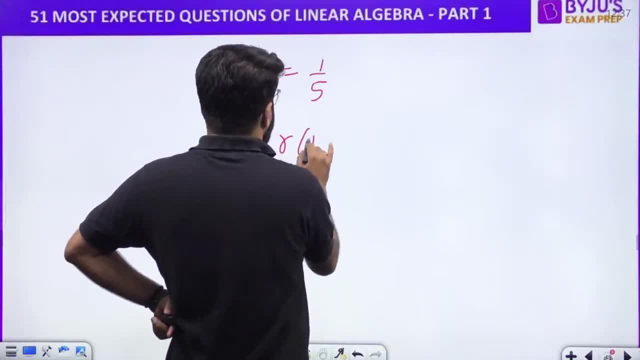 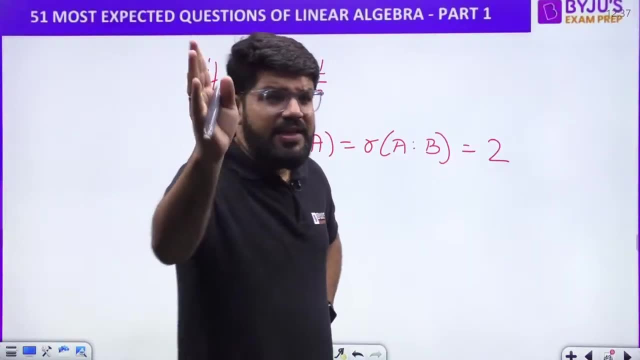 to be that is 2.. Okay, Then I will say: rank of A equal to rank of A is to be that is 2.. Then what is the type of solution? Then, what is the type of solution, everybody? Then what is the type of? 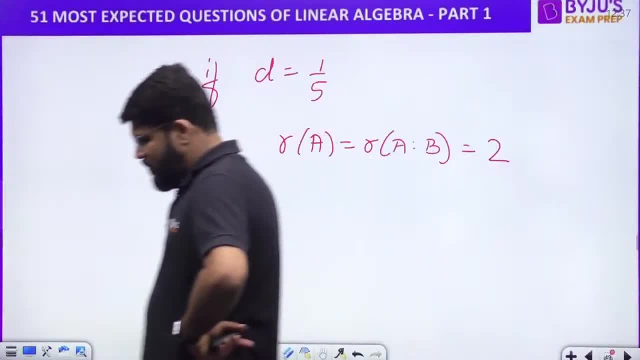 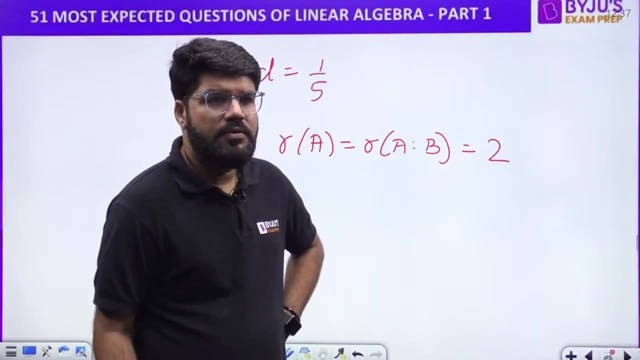 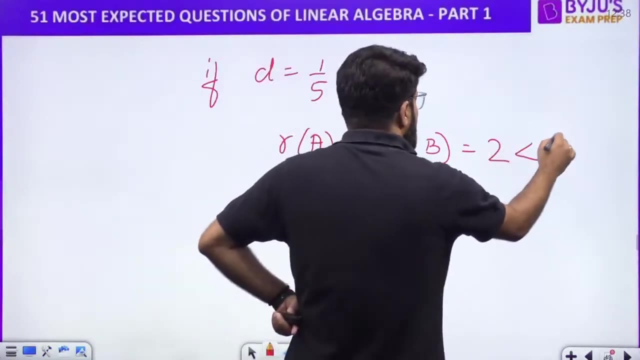 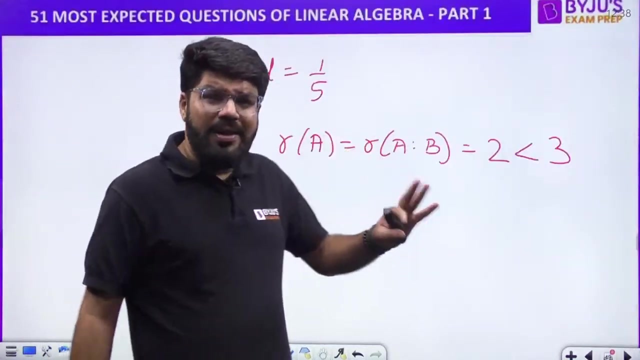 solution All dear. what is the type of solution then? Then, what is the type of solution? Infinite right, Yes, Rank of A, equal to rank of A is to be, but less than the number of variables. i Number of variables: 3 here here: N, k, value 3, hai. Both the ranks are equal, but less than. 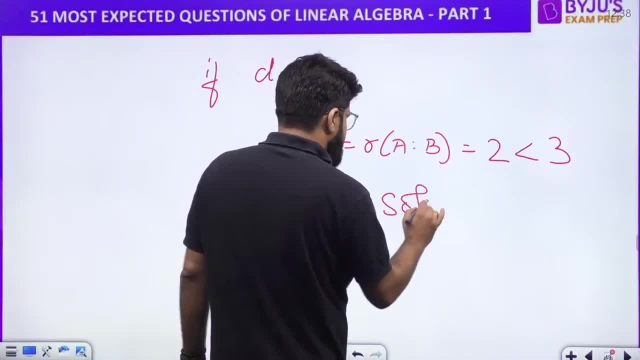 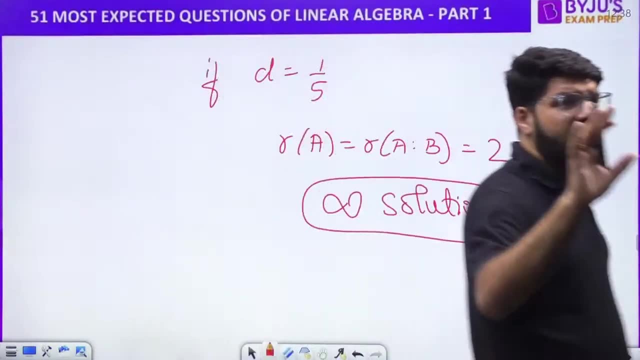 number of variables, Then the system has infinite solutions. For only a single value of D, the system will have infinite solutions. Okaytr, Custom class. fine. Now if you go and check this determinate If you total 0 and 1 anymore, So 0 and 1 in the come down cell Right. Listen closely as I am midst of on all time. R x. 1 plus 0 to 2 minus 1 is less than the distance between uh, since one and 1 is 1 minus 1.. But given 8 to 6 by negative n times, k times, sir. The distance between 1 means you do5 four times k times 2.. For difference between 5 to 10, x, n, 0 under the value of d, equal, but under 6 and 2, the difference between the numbers of 2 and n is 6: 0 and. 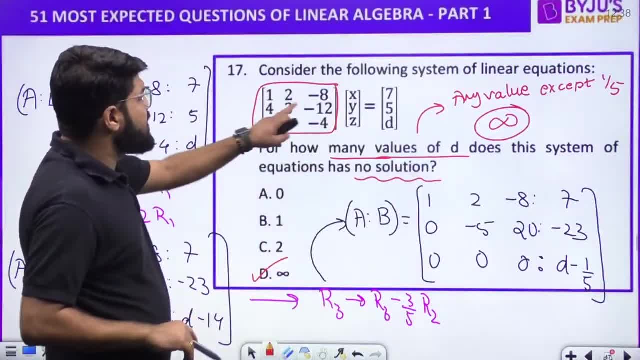 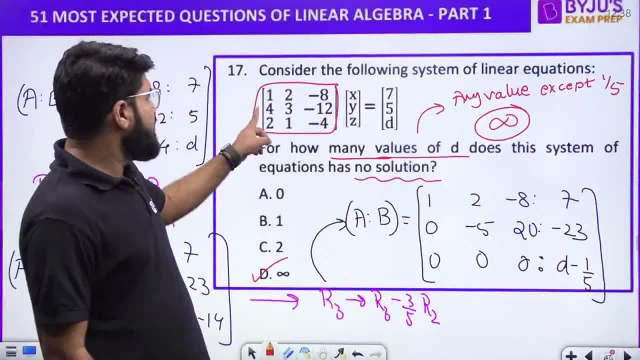 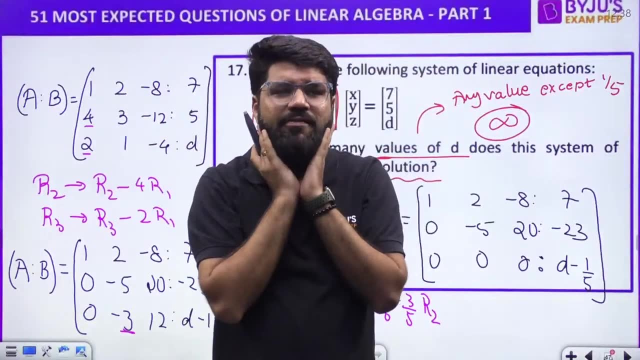 check this determinant. if you go and check this determinant, this determinant will be zero. that is why- unique solution- it will never have the unique solution case. this determinant will be zero. it will never have the unique solution case. it will never have the unique solution case. it will only have either infinite or no, either infinite or no right. so if d does not equal to, 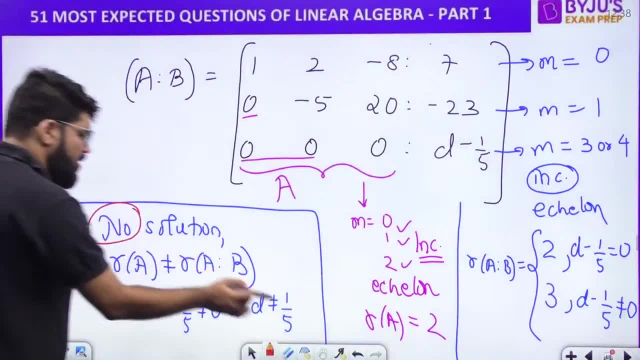 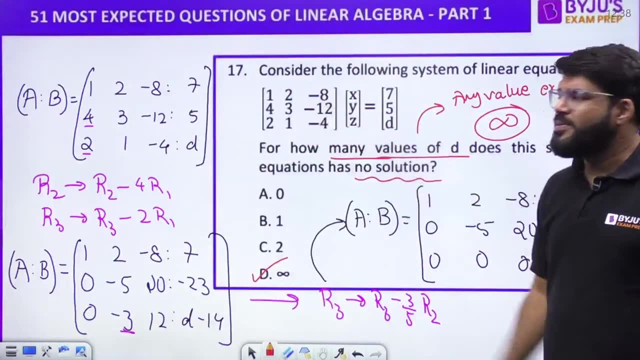 1 by 5. no solution. this one, no solution. if d equal to 1 by 5, then you have infinite solution. unique solution not possible here because determinant of a. please check it out. it is going to be zero. quickly, you can check. it's going to be zero. okay, right, so no solution. 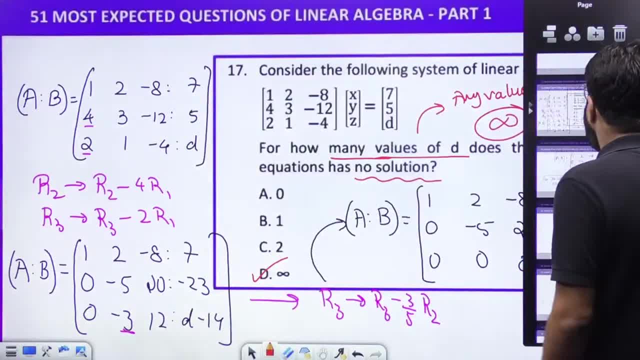 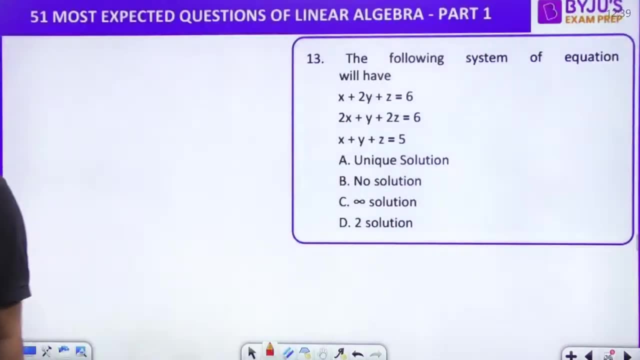 question now. now, everybody, let's keep rolling, everybody, let's keep rolling and have a look into this question. the following system of equations will have the following system of equations will have: the following system of equations will have: what type of solution following system: this question. i will introduce the trick, but let me solve it regularly first. 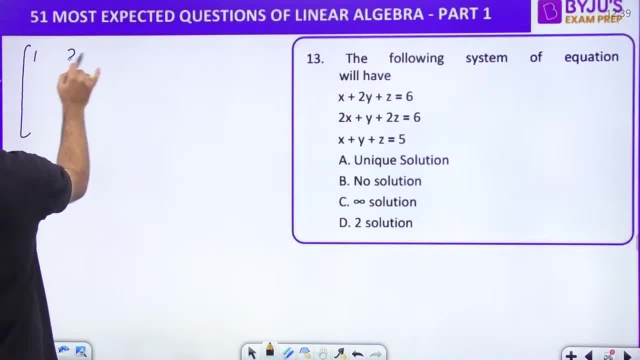 okay, regularly. what is the? a is to b matrix: 1, 2, 1, 6, 2, 1, 2, 6, 1, 1. 1. is to 5: 1, 2, 1, 6, 2, 1, 2, 6, 1, 1, 1, 5. okay, what will the system of equations have? 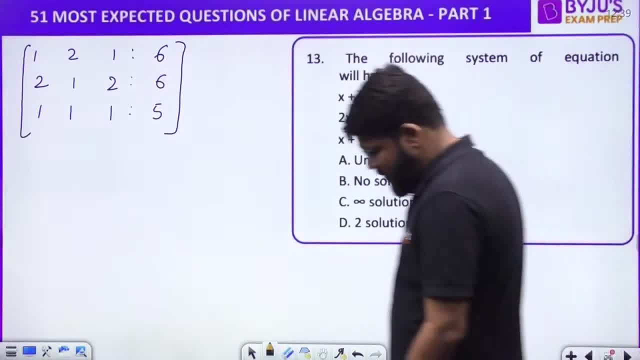 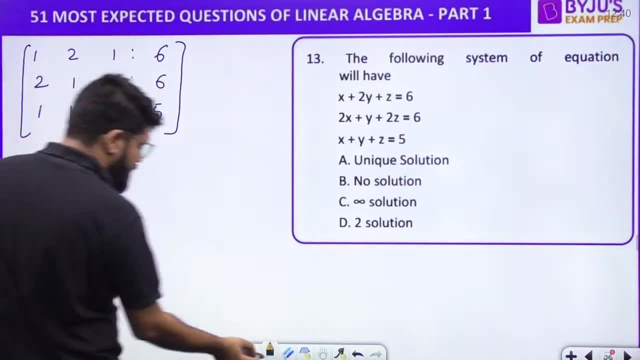 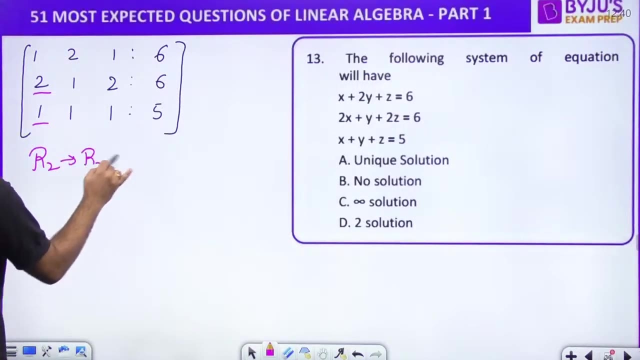 what will the system of equations have? okay, very simply, let me start with the echelon method once again. okay, i need to convert first this into 0. i will apply clearly: r2 is equal to r2 minus 2, r1 and r3 is directly r3 minus r1. 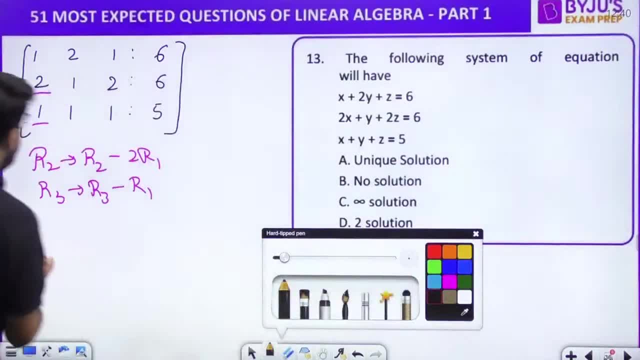 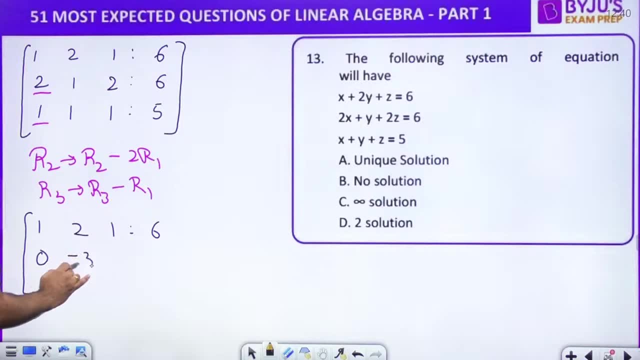 both are same, 1 and 1. okay, subtract here. so what is the matrix now? 1, 2, 1, 6 i, 2 minus 2, 0, 1 minus 4 minus 3, 2 minus 2. again 0, 6 minus 2 into 6 minus 6, one minus one zero. 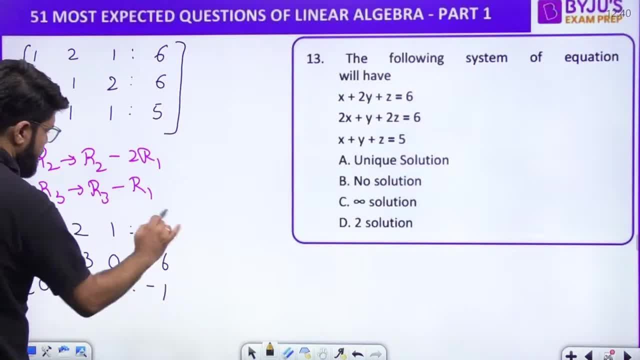 1 minus 2 minus one, 1 minus 1, 0, 5 minus 6 minus 1. okay, now again for ec volcanic form. i need to increase the number of zeros, nil, then one, and then this also has to be 0 for increasing number of the starting zeros, increasing number. 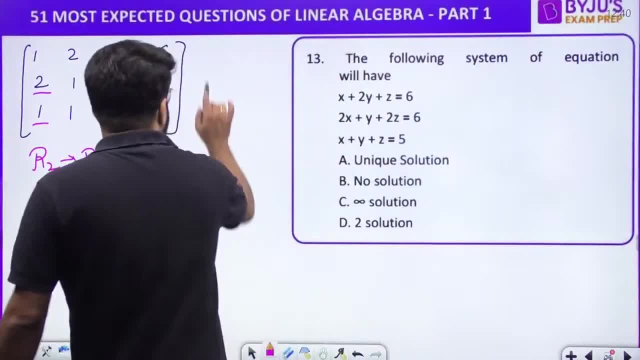 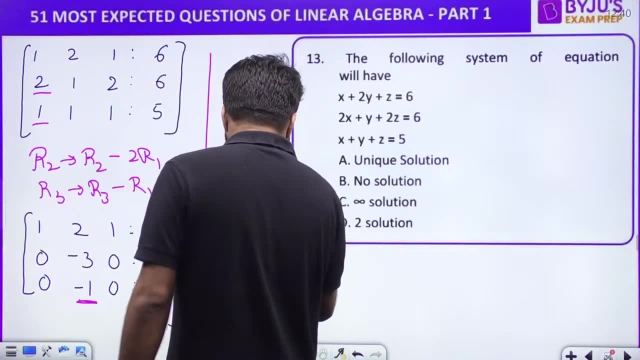 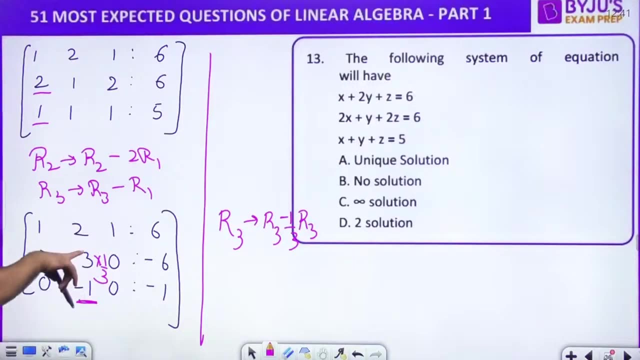 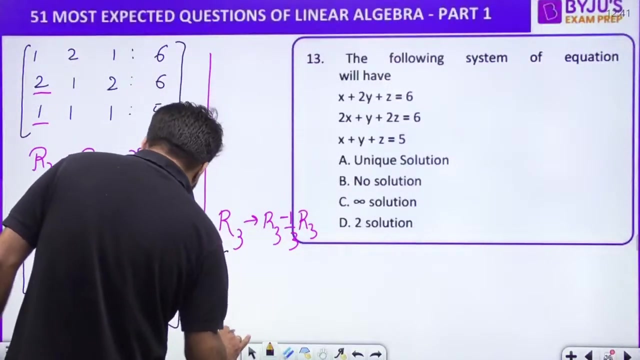 starting zeros, right, okay, so what is the next step i will do now? next step that i will do now is: multiply r2 by one third, multiply r2 by one third, multiply, and then this becomes minus one. then i can subtract. okay, after doing this, see the matrix that now comes: one, two, one. 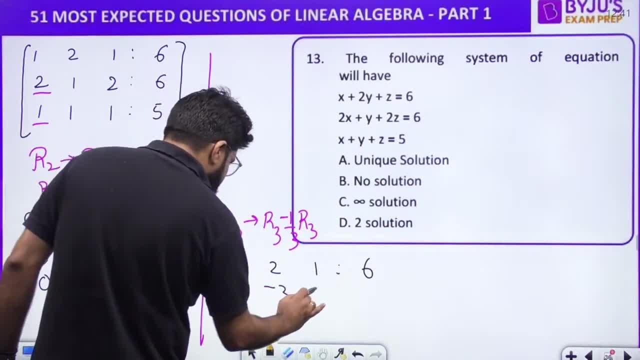 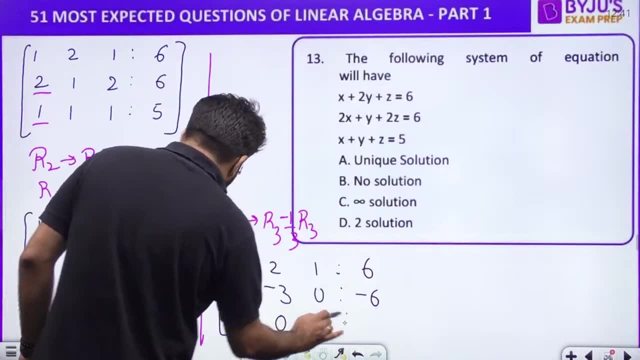 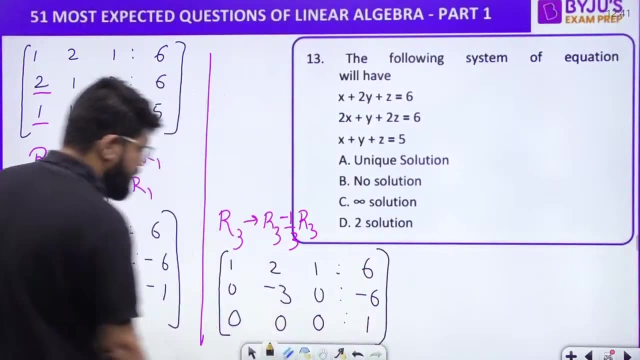 six right zero minus three zero minus six right zero, one third. say: subtract here zero, zero. here also you subtract, you multiply one third. this becomes minus two minus one. minus of minus two will be plus one, will be plus one. okay now number of starting zeros are in the increasing order: no. 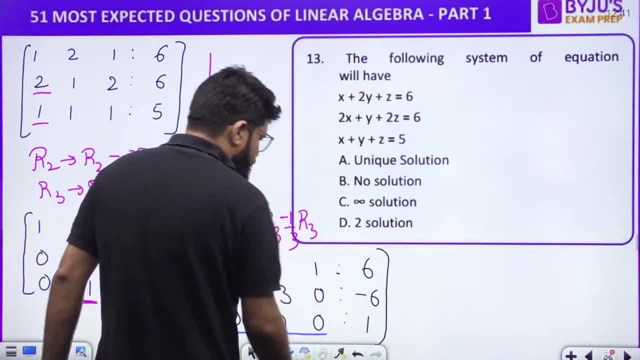 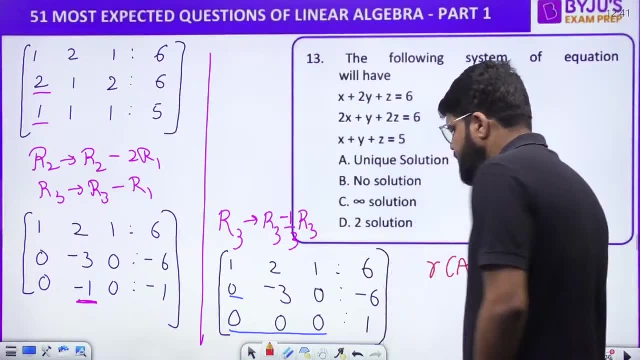 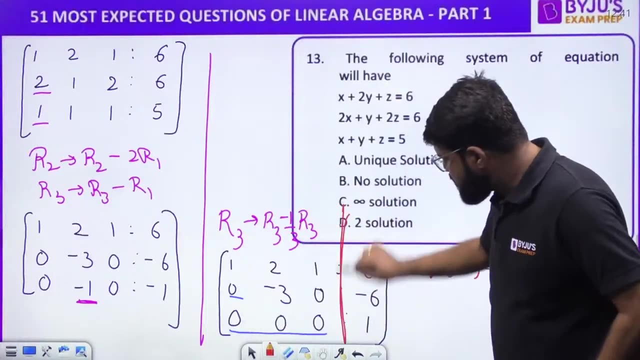 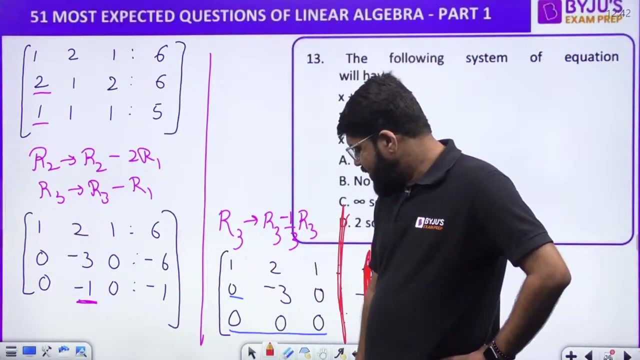 problem. number of starting zeros are in the increasing problem. what is the rank of the? a matrix, a? what is the rank of a matrix? how many zero rows? how many non-zero rows? sorry for the a matrix. look into this much part, look into this much of part and see the answer right. rank of the matrix is number of non-zero. 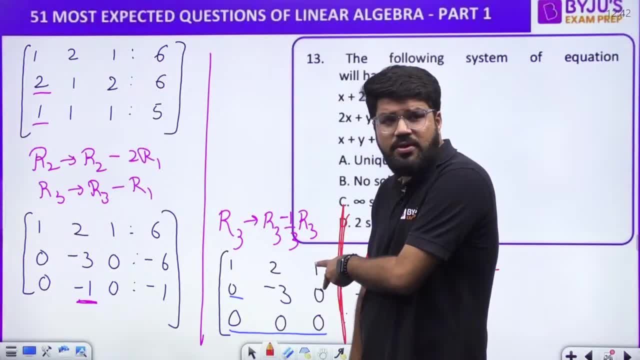 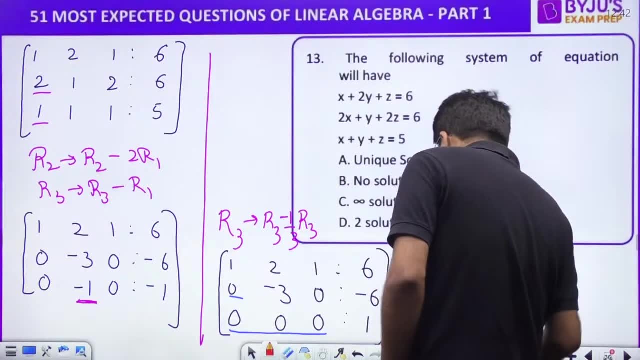 rows. only two non-zero rows. three: only two non-zero rows. right? only two non-zero rows. the rank of a is equal to two. rank of a is to b is to b, even the bigger matrix. both are in the achelon form. starting zero is one, so starting zero. 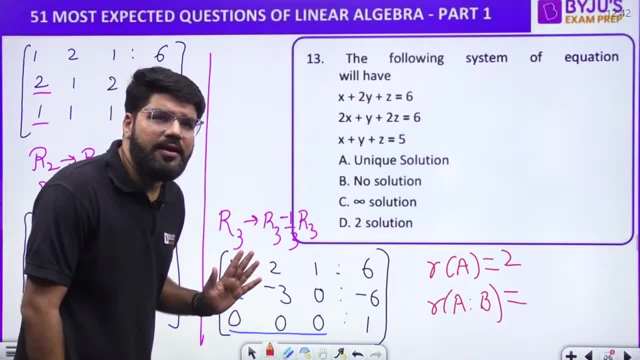 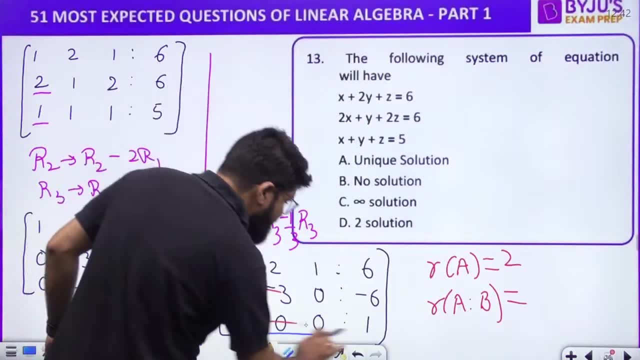 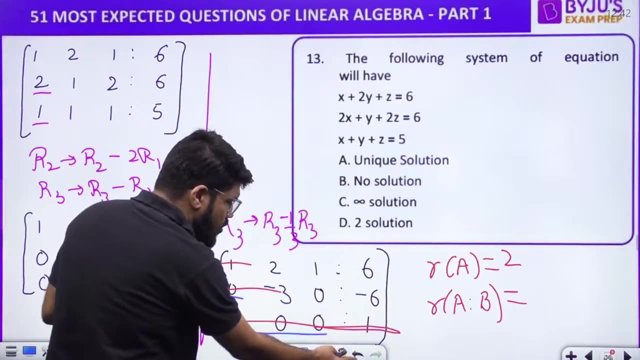 sorry, starting zeros is zero. one and three. increasing order: increasing order, strictly increasing order. okay, how many non-zero rows? non-zero, this is non zero. this is also total non-zero. na, you cannot call it as row of zero. a is to b of a means you have to see the entire row up to this point and this is a nonzero row. 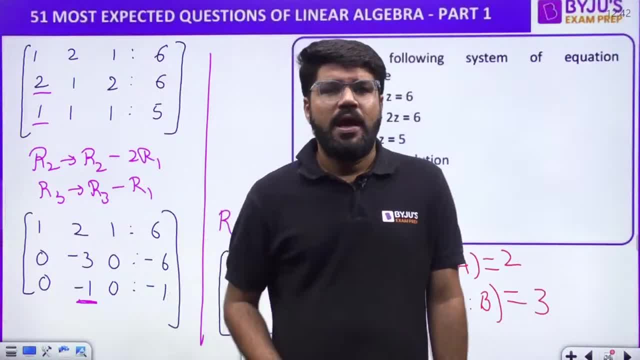 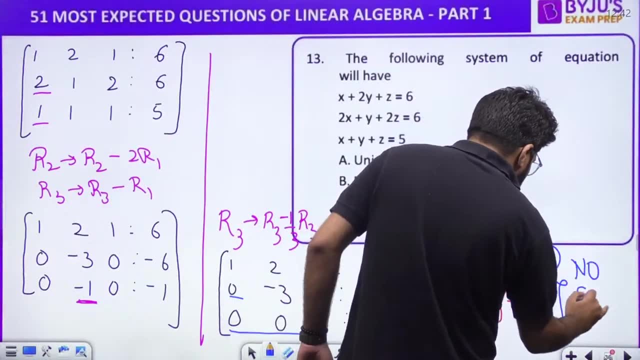 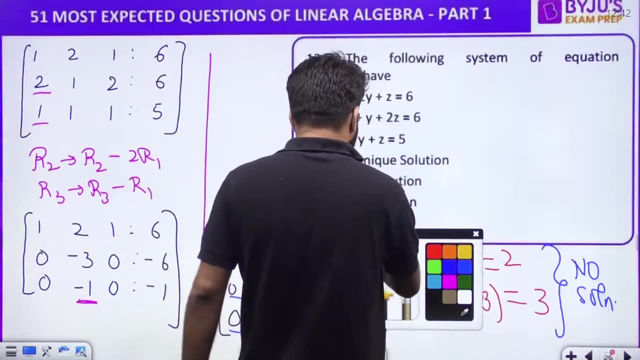 this is a nonzero row. so how many non-zero rows in a is to b? how many non-zero rows in a is to be 3? it is 3, right? so system has both the ranks mismatch, just like the previous question. both the ranks mismatch. the system has no solution. the system has no solution. 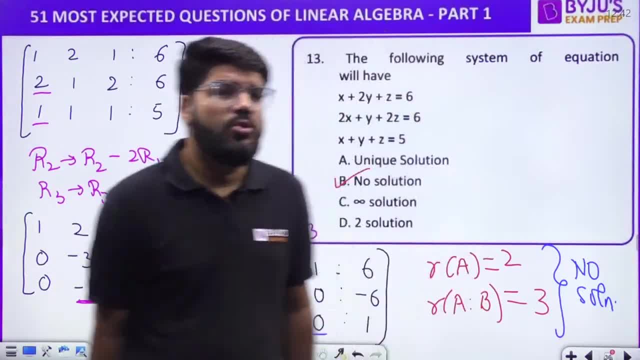 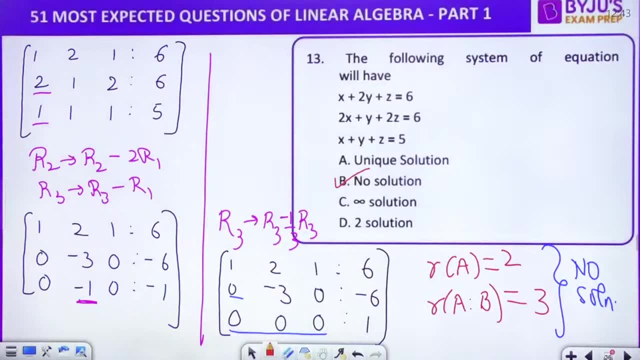 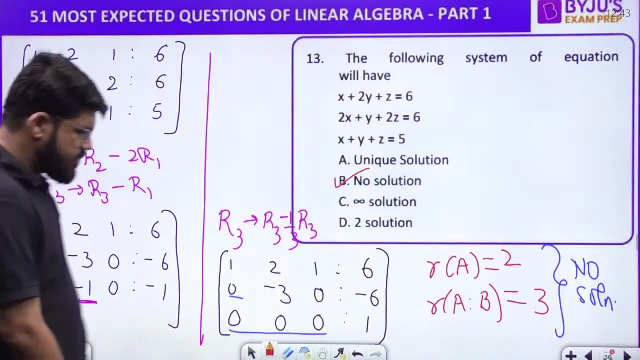 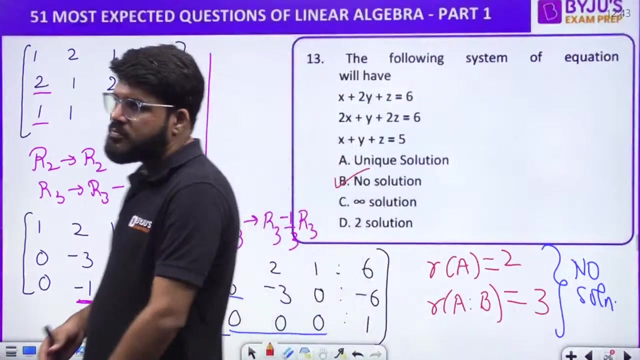 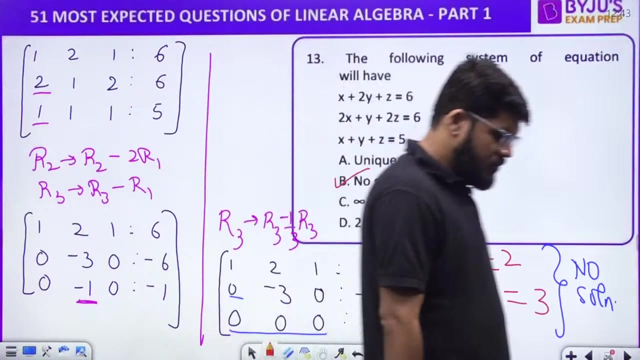 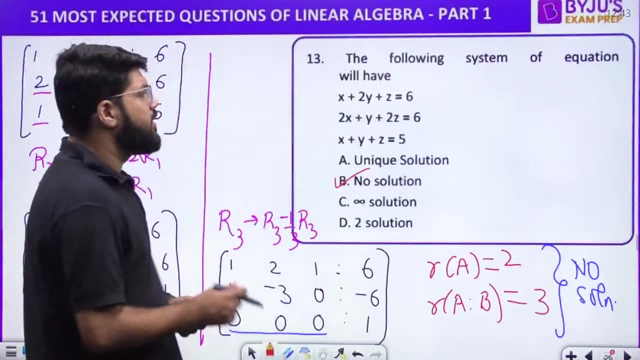 option number B is the correct answer here. the system has no solution, right. the system has no solution here. everybody chalo cool. the system has no solution, very good, okay, up the core is shortcut. kya hoga? have a look into the shortcut directly. have a look into the shortcut. 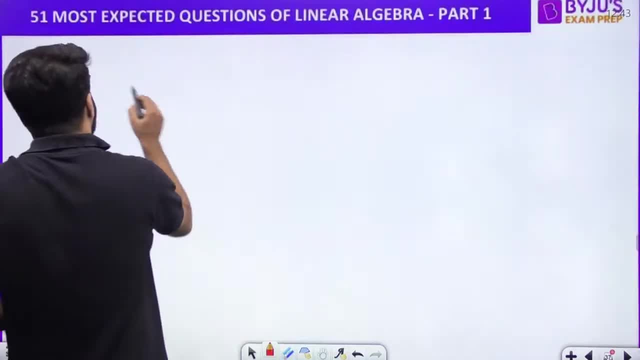 the following system of equations will have what? okay shortcut making a method number 2. let me rewrite that the equations okay, x plus 2, y plus z is equal to 6, 2 x plus y plus 2, z is equal to 6 x plus. 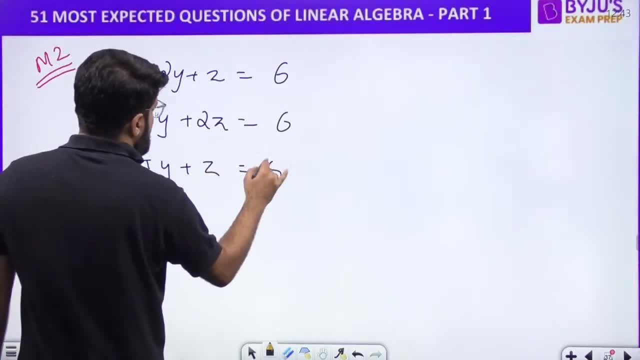 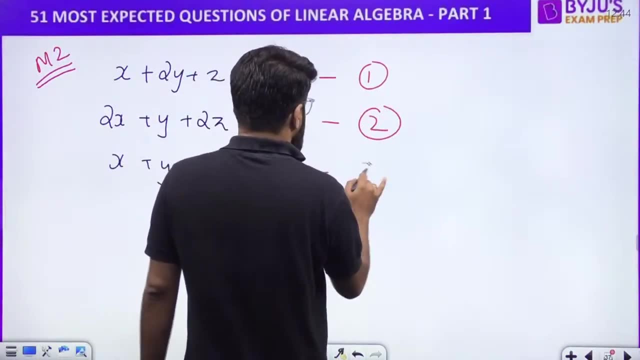 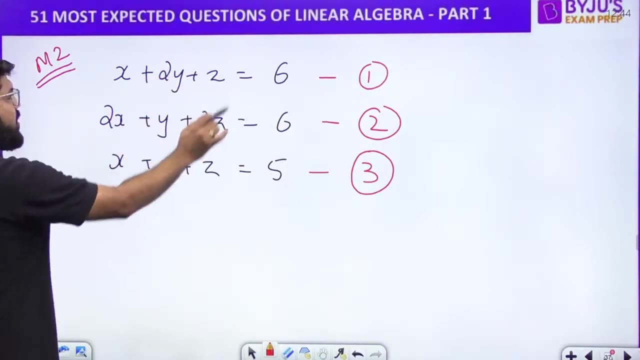 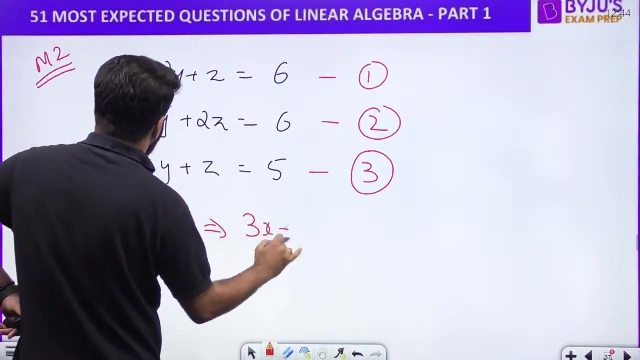 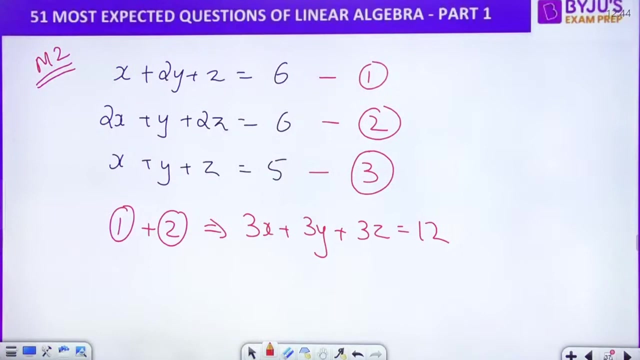 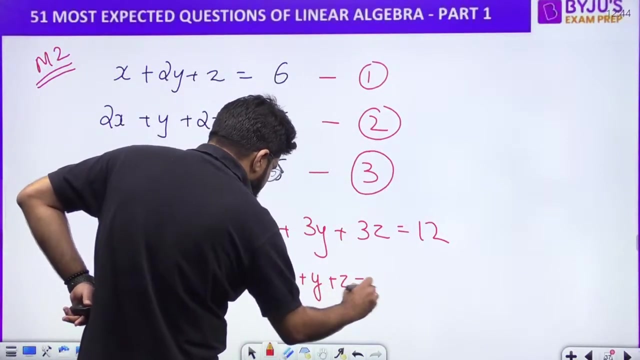 y plus z is equal to 5. okay, see, if I add equation number 1 and 2, na dependency, like the rank shortcut was dependency. yahaan, pe bhi dependency dekhenge. when you add these two, so 3 x, 3 x, 3, y and 3 z, all of them becomes 3, 3, 3, right? so when you add 1 and 2, you get x plus 2 x, 2 y plus y, z plus 2 z and right hand side, 6 plus 6, equal to 12. 3 x plus 3 y plus 3 z, equal to 12. 3 x plus 3 y plus 3 z, equal to 12. what is going to be x plus y plus z? what is going to be x plus y plus z? 12 is divided by 3 and that is 4. 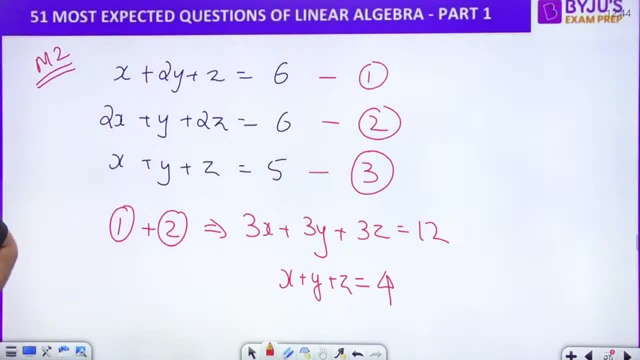 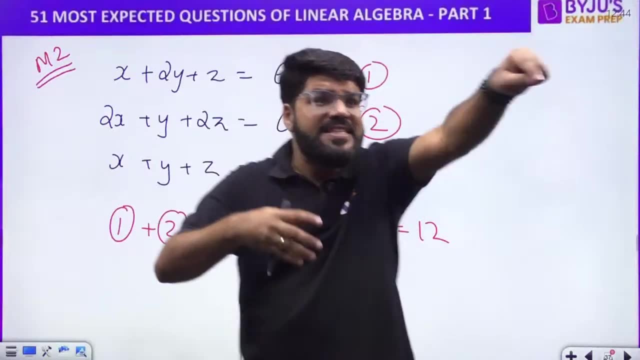 12 is divided by 3 and that is 4.. Now equation number 1 and 2, look into this Equation, number 1 and 2, when you combine they say. they say x plus y plus z should be 4.. 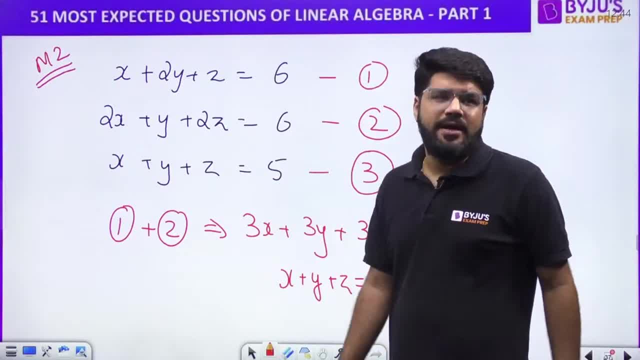 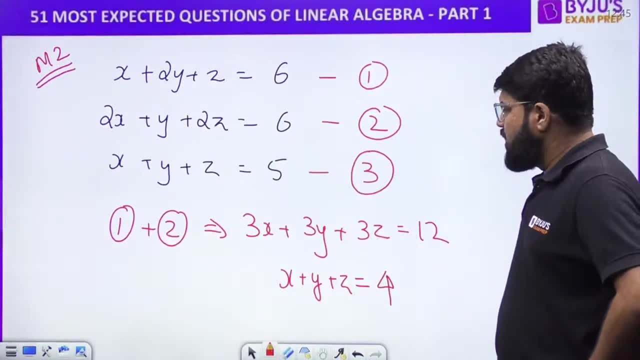 Sum of x, y, z should be 4.. But equation number 3, what does it say? Equation number 3 says that no, x plus y plus z should be 5.. So you are wrong. Okay, You are wrong. 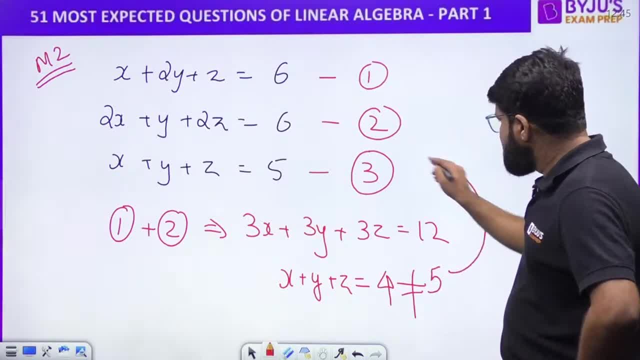 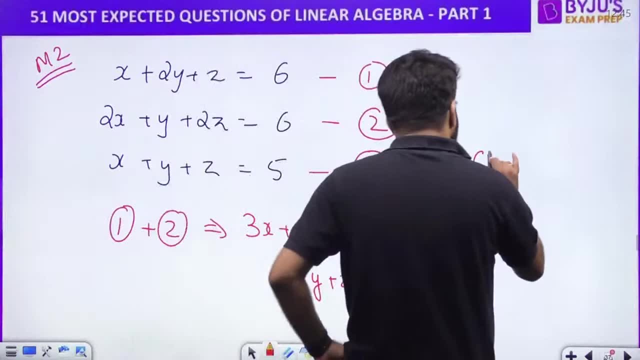 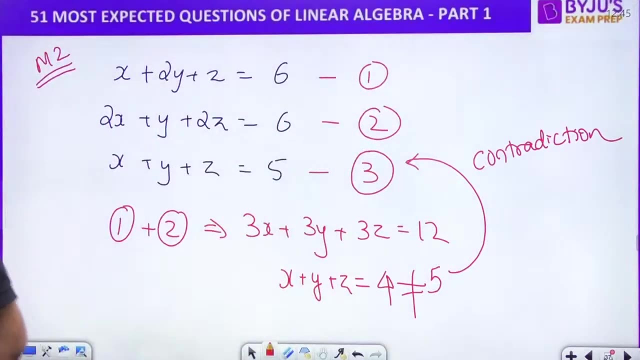 You are wrong, because equation number 3 says that x plus y plus z should be 5.. So what is this? This is known as the case of contradiction. Everybody? this is known as the case of contradiction. Right, This is what is known as the case of contradiction. 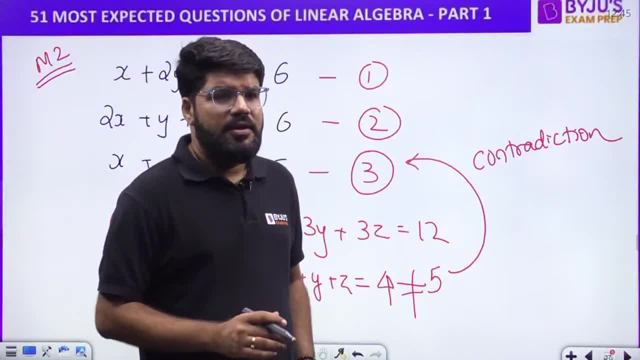 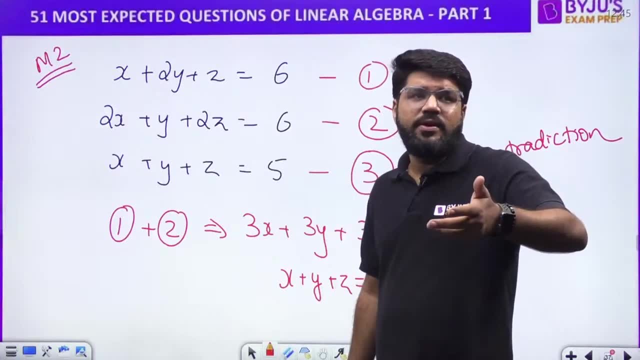 This is what is known as the case of contradiction: They cannot agree to each other. Okay, So if, what is the meaning of linear system simultaneously solving linear system of equation? That means we need to find x, y, z. 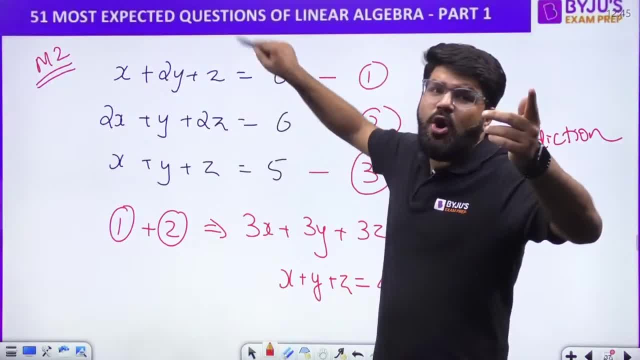 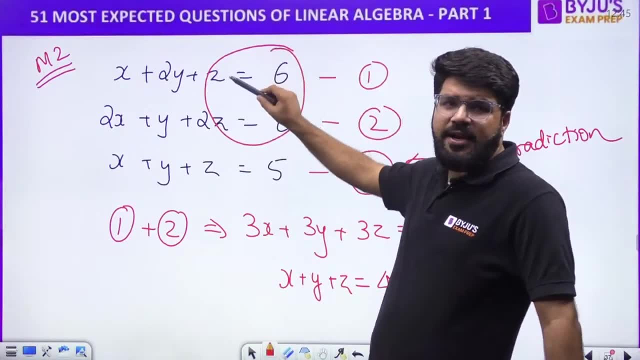 That means we need to find x, y, z which will satisfy all the three equations, Which will satisfy all the three equations. So if you have x, y, z, which satisfy first and second equation, it can never satisfy the third. 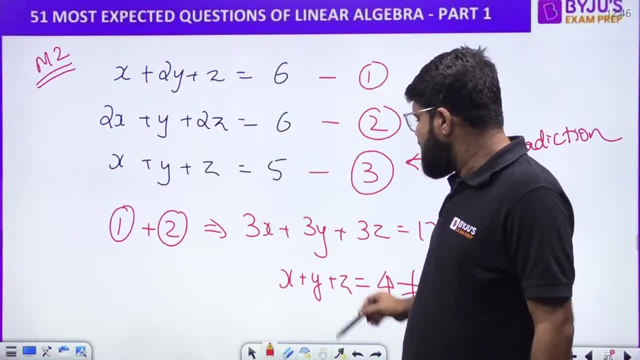 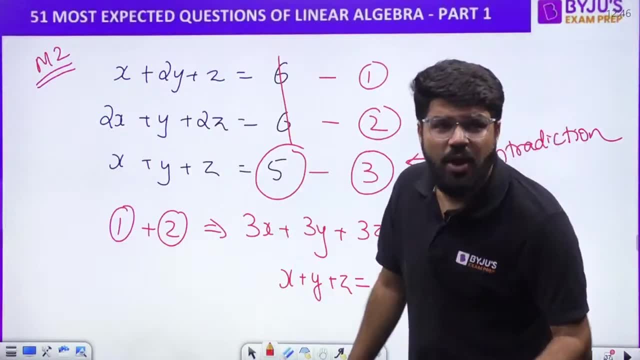 Or if you select x y z. if you select x y z, satisfying the third equation, it can never satisfy first and second. That means there is no value of x y z which can satisfy all at a time, because they are contradicting. 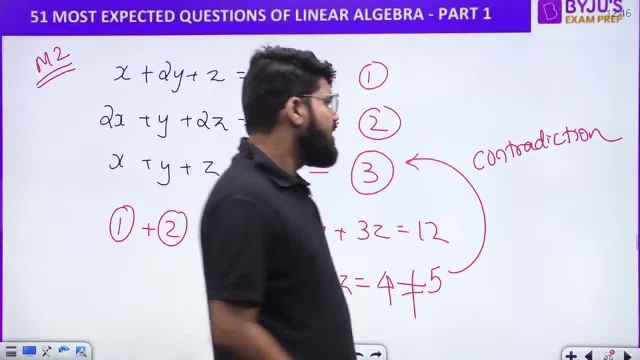 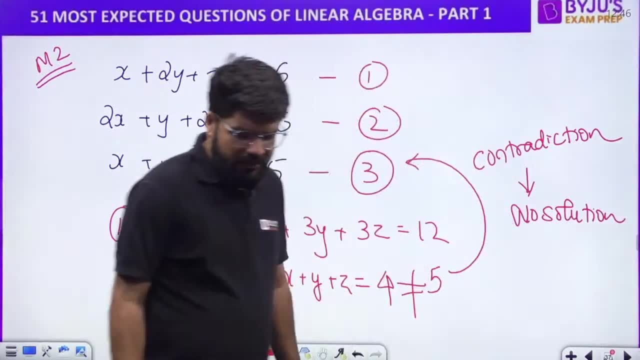 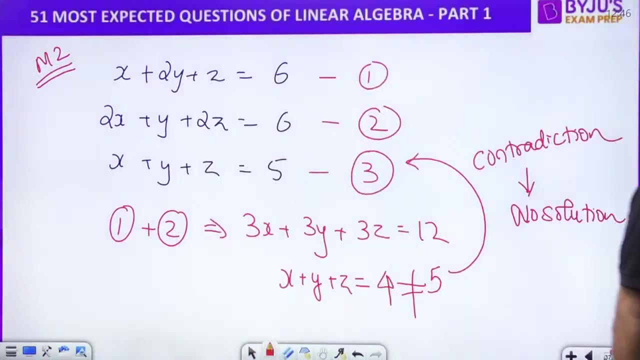 They are fighting each other, They are contradicting, They are fighting each other And whenever you have the contradiction, you have no solution. Whenever you have contradiction, you have no solution. Right, Whenever you have contradiction, you have the no solution. 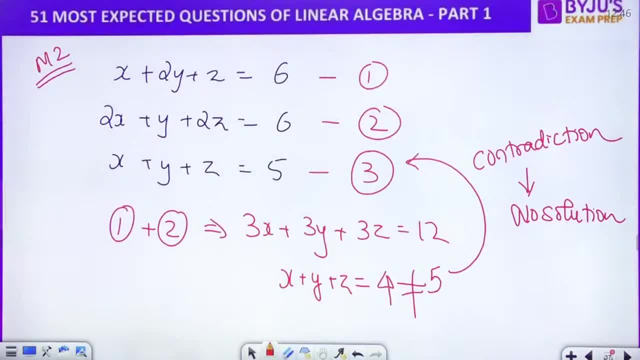 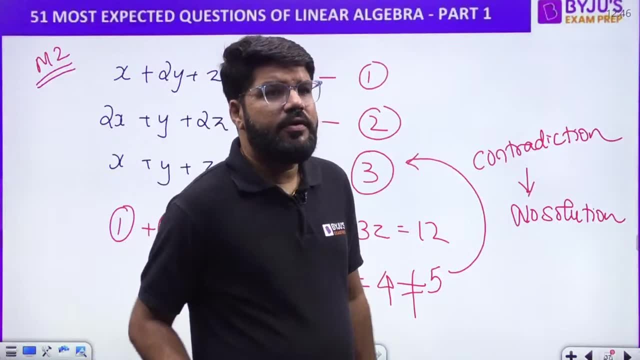 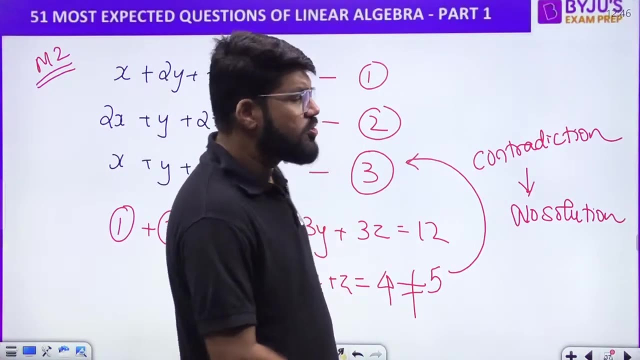 You have the no solution, Right. Whenever you have the contradiction, you have the no solution. All okay For contradiction. you have no solution, Chalo, Right. Remember, this is also a direct way of solving it. This is also a direct way of solving it. 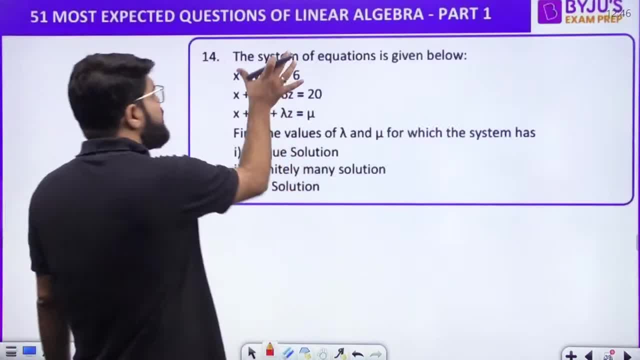 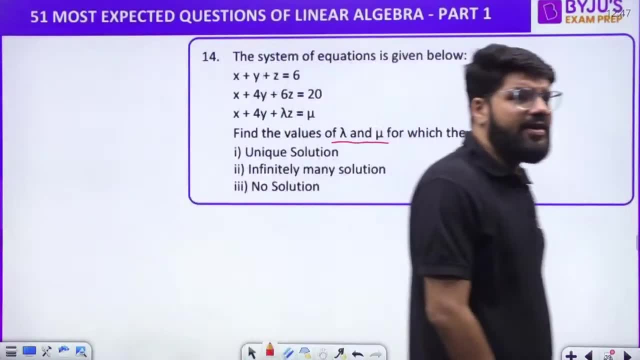 Chalo. Now guys, take up this question. With this question, let us find out the values of lambda and mu, for which the system has unique, infinite, no, All the three cases. let us quickly revise through this question And then we will come back to it. 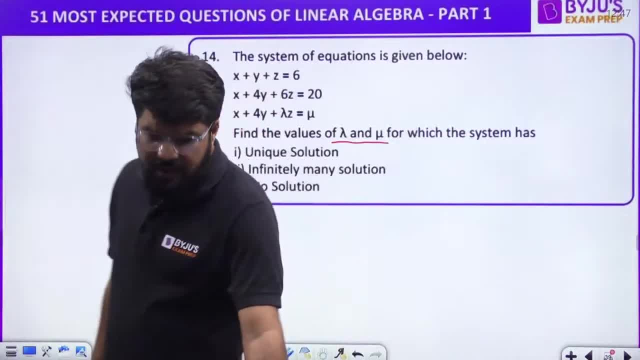 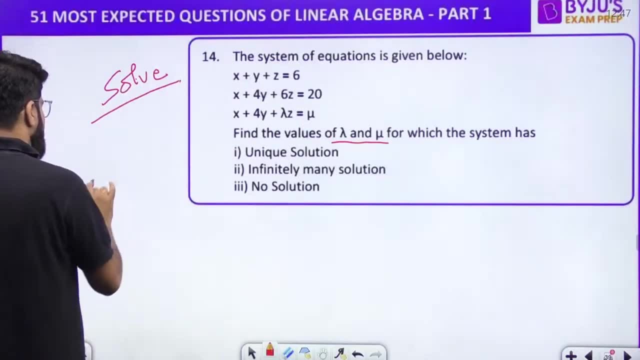 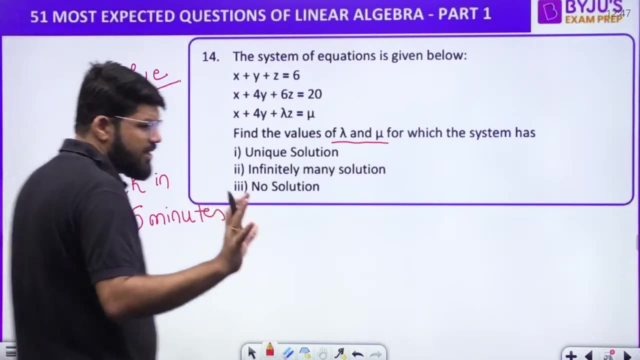 And then move to the next category. Then move to the next category. Guys, I just need five minutes of time, So please solve it up. I'll be back in five minutes. It's not a break or it's not a halt, but I'll just need four or five minutes. 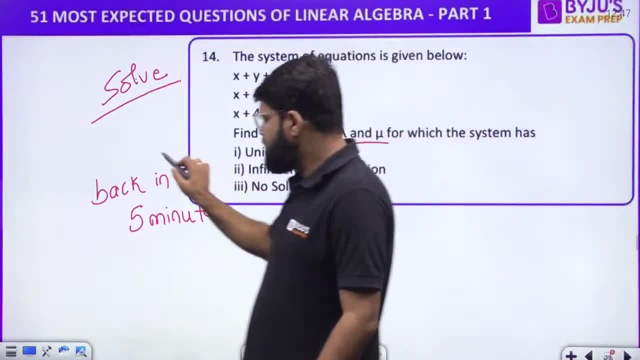 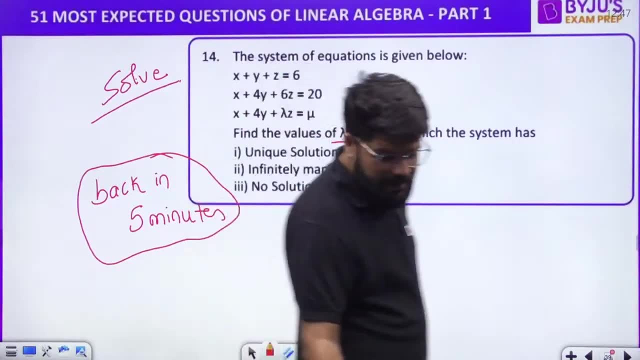 I'll come back. I'll just have some coffee or something. I'll just come back. I'll be just back in five minutes, Stay tuned. I'll just have some coffee or something And I shall come back very shortly. I need something. 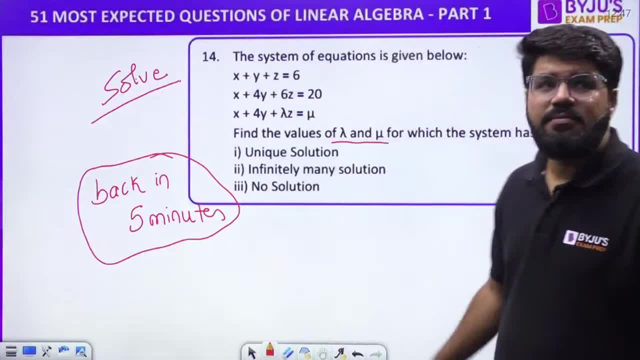 I need something for my throat Right. Five minutes, Just five minutes maximum. I'll come back. Okay, Please solve it up. I need your answers by that time. I'll come and start solving immediately, So please solve it up. 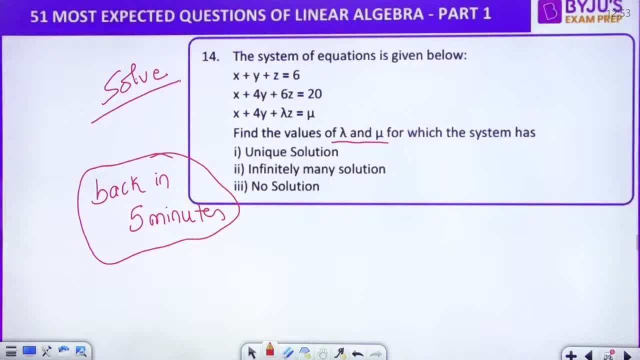 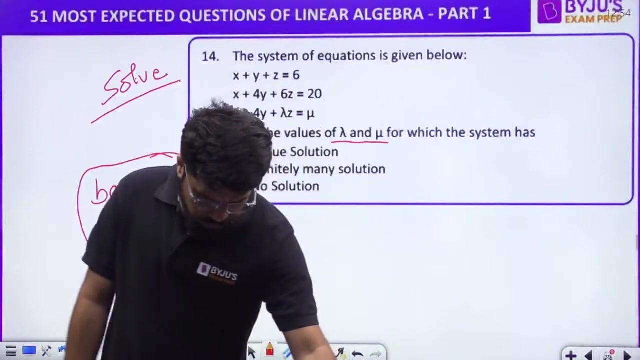 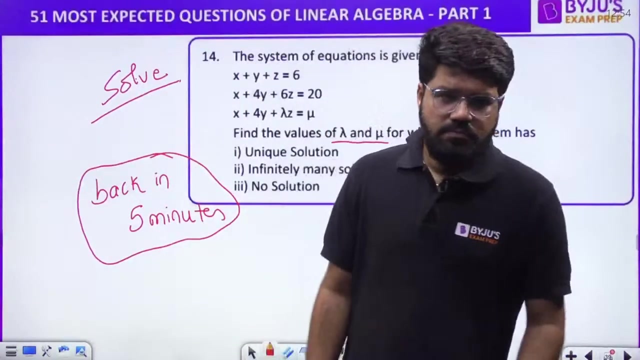 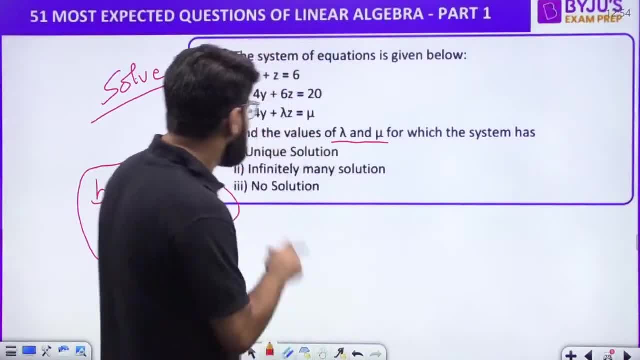 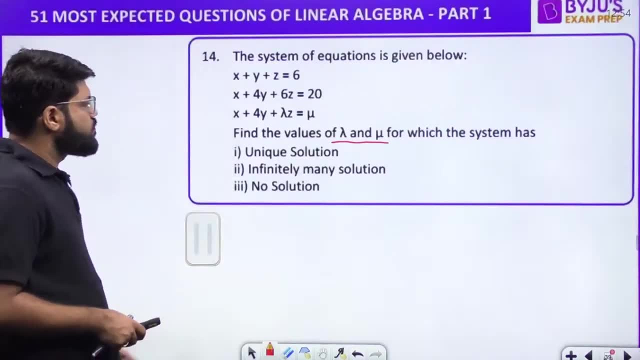 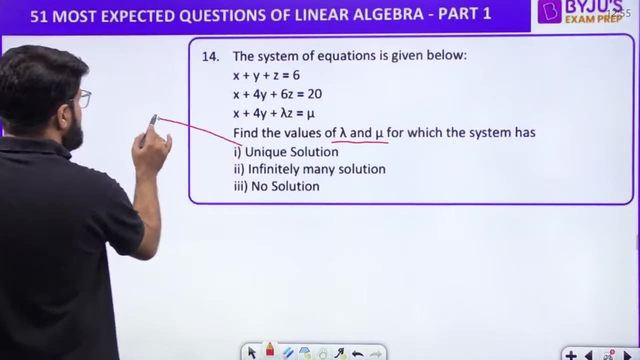 Some students lost the track in between, Some students left, or what Check? Unique? infinitely many solution and no solution. Unique is the first and the simple case. Okay, Unique is the first and the simple case. Unique, Unique, Unique. 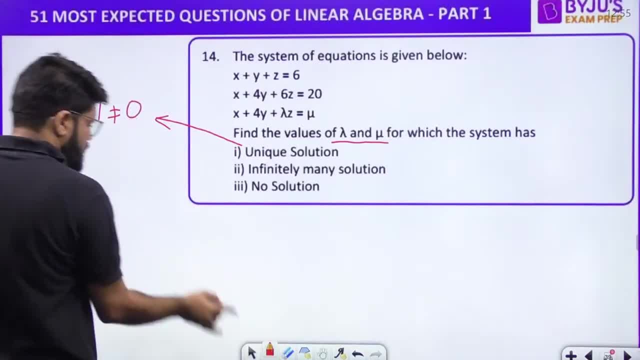 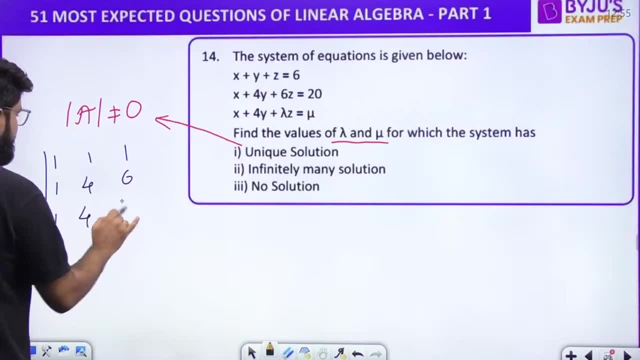 Unique, Unique directly determinant not equal to 0. determinant not equal to 0 means you have 1- 1- 1, you have 1- 4- 6 and you have 1- 4 and lambda the determinant of this not equal to 0. determinant of the. 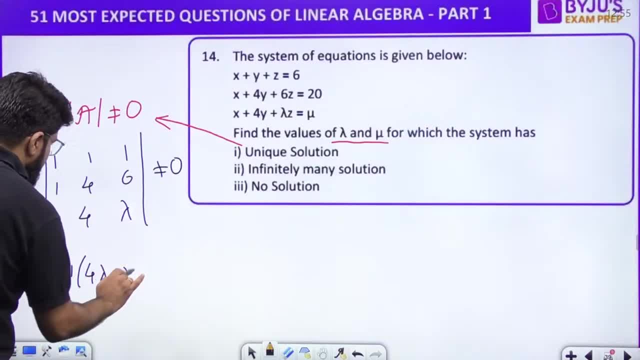 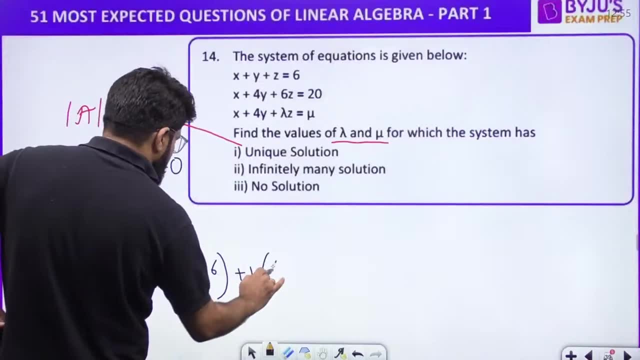 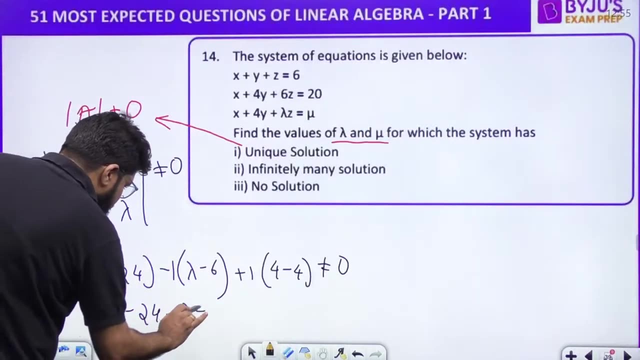 coefficient matrix. so it is going to be 1: 4 lambda minus 24 minus 1 lambda minus 6 plus 1 into 4 minus 4. this is total, not equal to 0. so 4 lambda minus 24 minus lambda plus 6, not equal to. 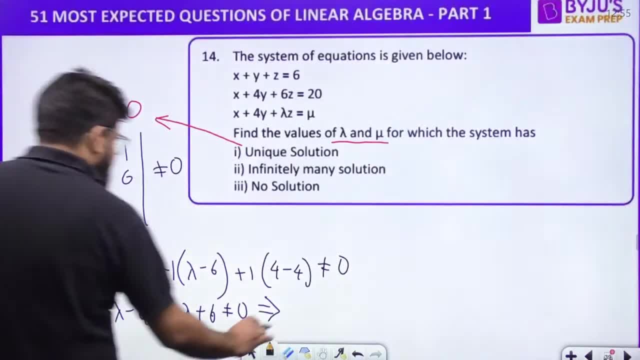 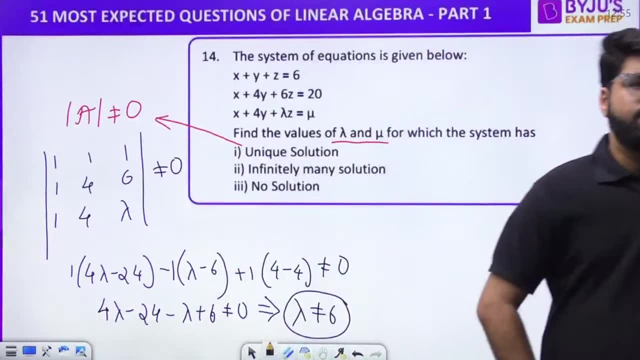 0, so 3. lambda not equal to 18. lambda not equal to 6. please check out the answer: lambda not equal to 6, right? lambda not equal to 6. is it the answer for unique solution? for unique solution? lambda not equal to 6. what about? 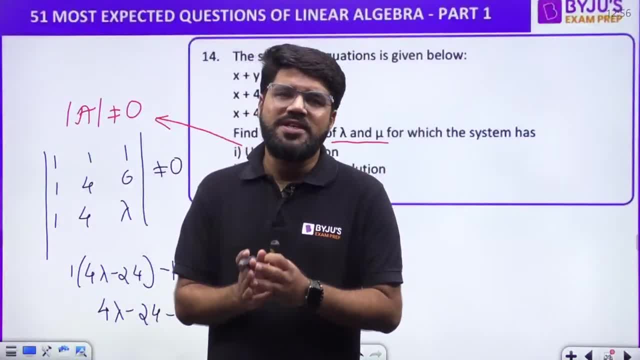 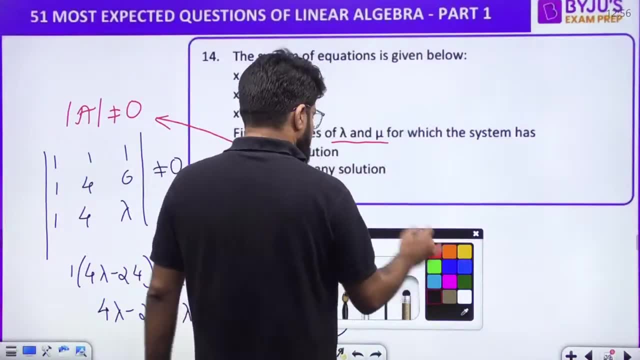 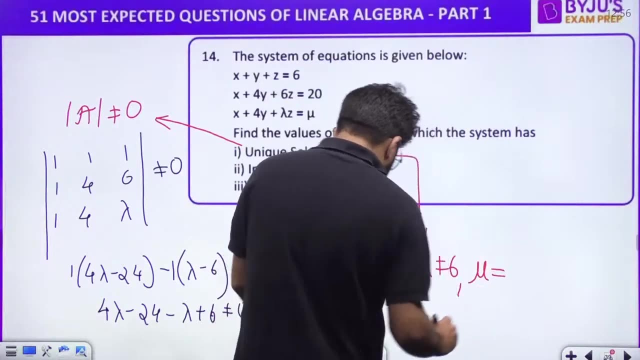 mu sir for unique solution, only coefficient matrix, determinant with will matter. there is no role of the mu right. so what is the answer for unique? what is the answer for unique right? lambda, not equal to 6. mu can take any value. mu can be any real value. 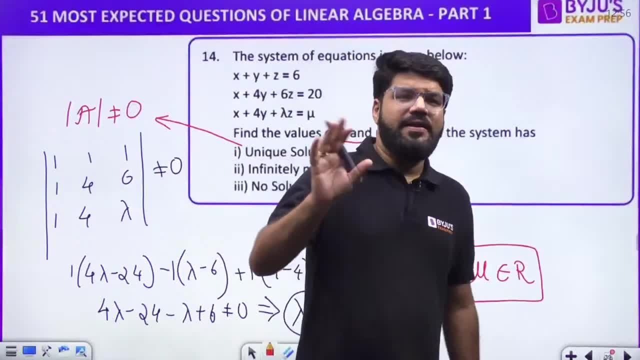 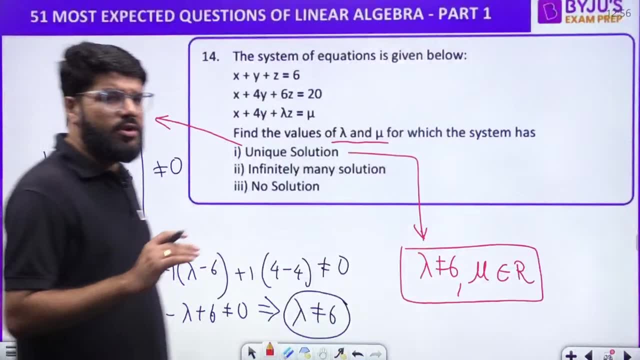 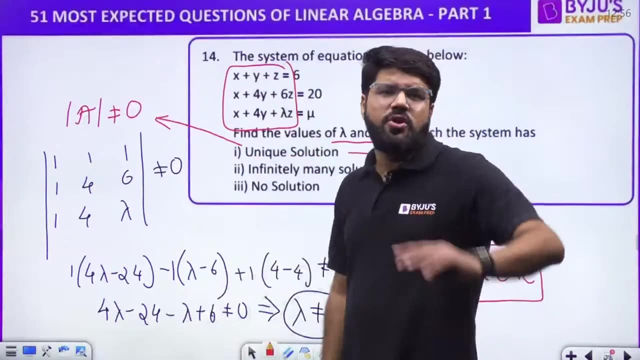 mu can take any value. no, no, it is not that mu same. no, no, no. there is no condition on mu. no guys for unique solution. there is no condition on mu. it only depends on the coefficient matrix. if the determinant is non-zero hundred percent, it is a unique solution, case mu can take. 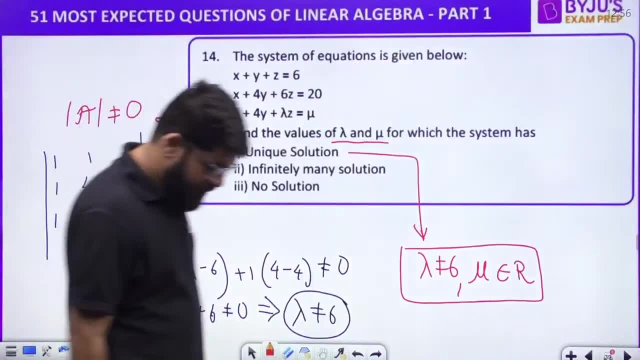 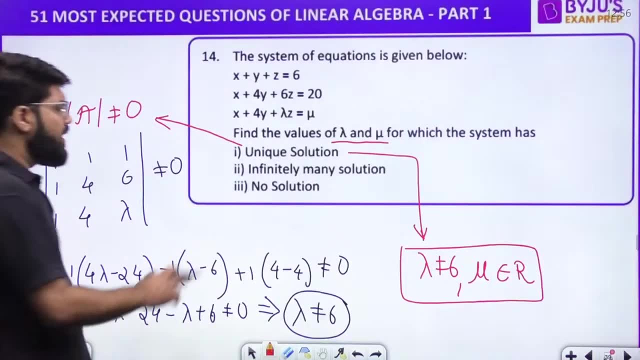 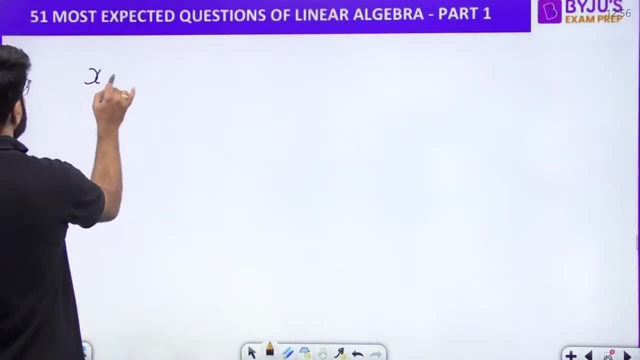 any, any value mu can take the any, any value. mu can take any possible value. everybody mu can take any possible value. great, let's go to the next. infinite and no solution. infinite and no solution. let me rewrite the numbers. i'll solve it up together: x plus y plus z, equal to six. i'll 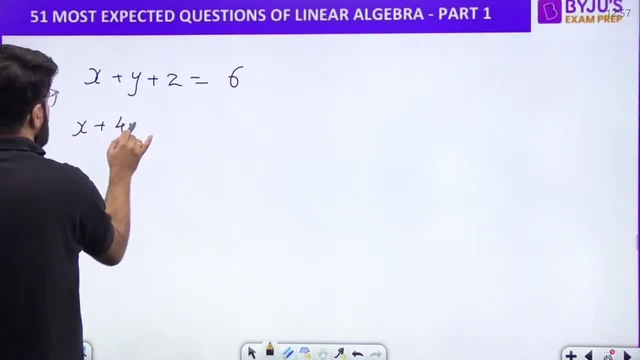 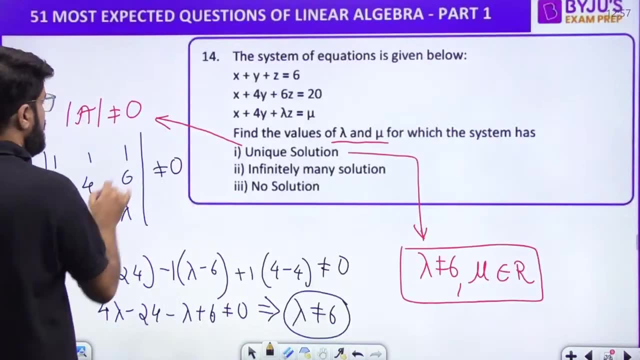 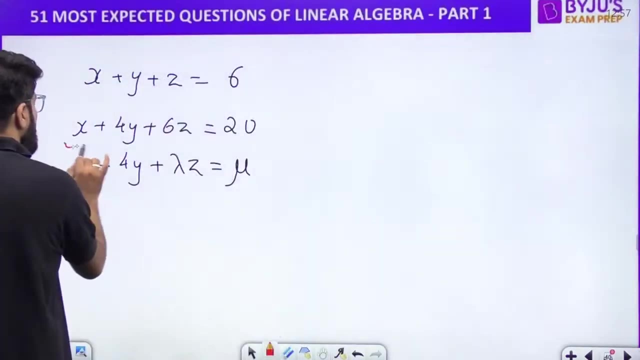 solve it through the shortcut now, which we have already discussed: x plus 4y plus 6z. x plus 4y plus 6z is 20, and next is x plus 4y plus lambda. z is equal to mu up right: x plus 4y. x plus 4y. 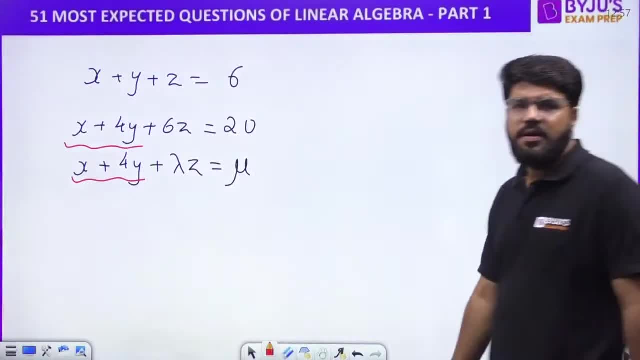 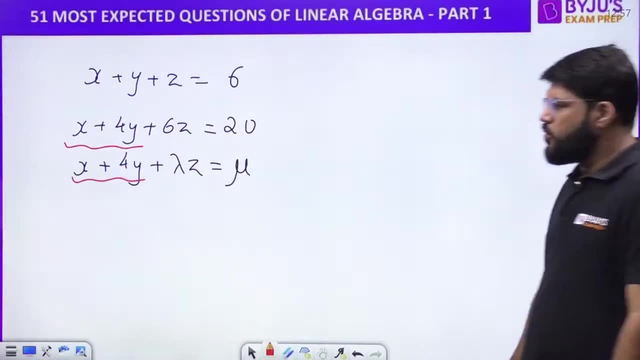 this much of the portion is common to both right: x plus 4y, x plus 4y. this much of the portion is common to both. this much of the portion is common to both right. suppose if this is common, the left hand side will be totally equal. suppose, if this is common. 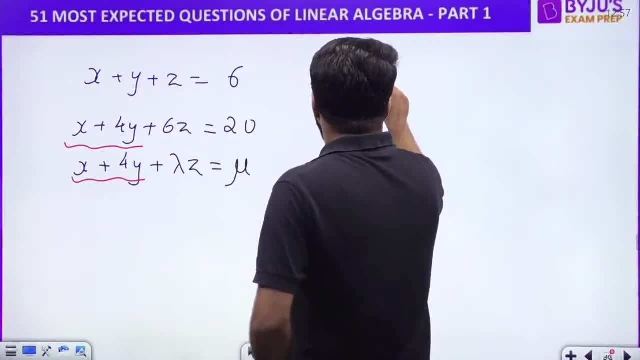 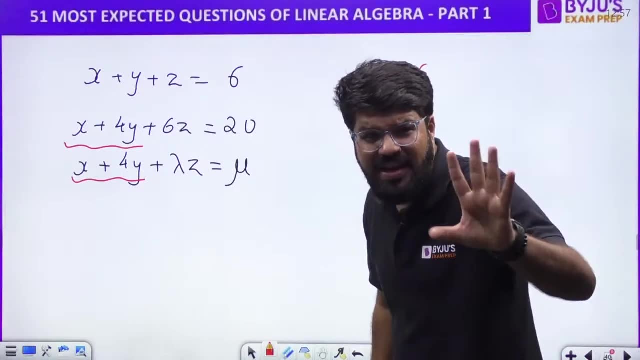 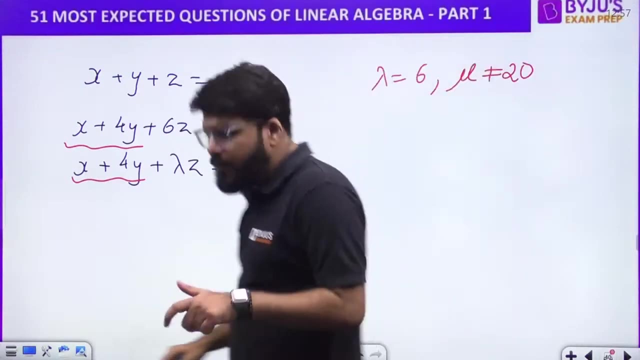 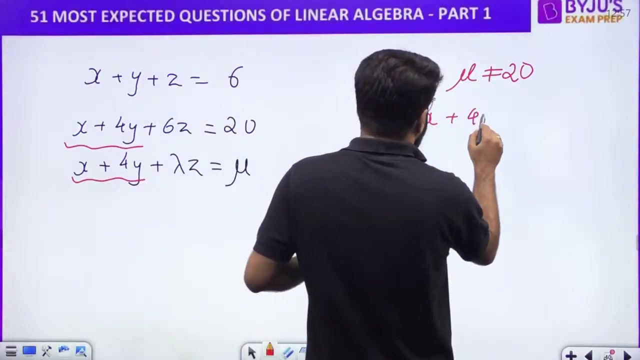 right understand through a simple logic. okay, so if lambda, i take it as six, if lambda, i take it as six. logic is all current, no need of any rank calculation. logic shortcut: lambda equal to six, but mu not 20. so if lambda is equal to six, x plus 4y plus, what will be the equation number three then x plus 4y plus lambda. 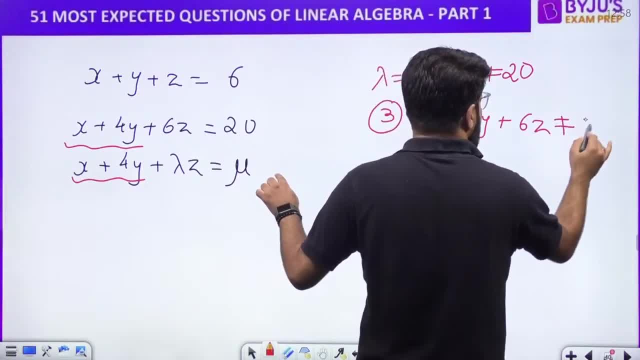 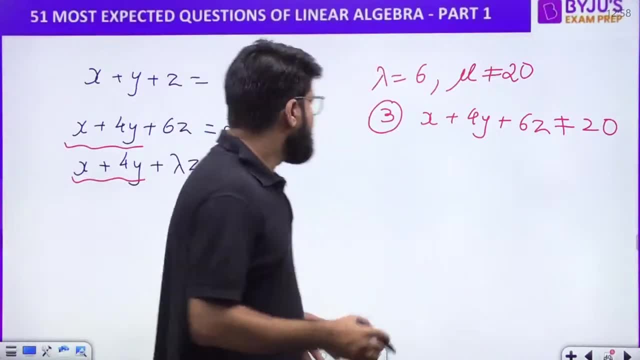 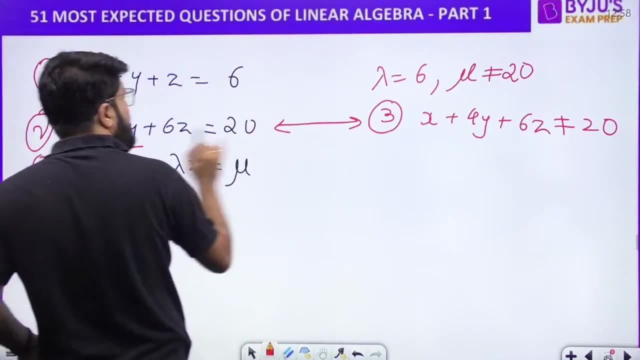 z, that is plus 6z equal to mu, but mu is not 20. so right hand side is not equal to 20. equation number two equal to 20. equation number three: there is not equal to 20, right? what will happen? what will happen, right? this is one, two, three. what will happen? it becomes the case of contradiction again. 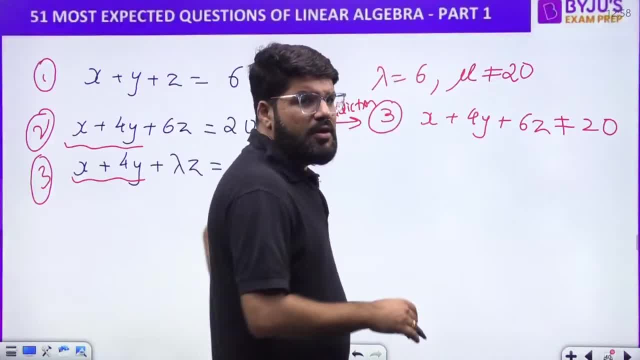 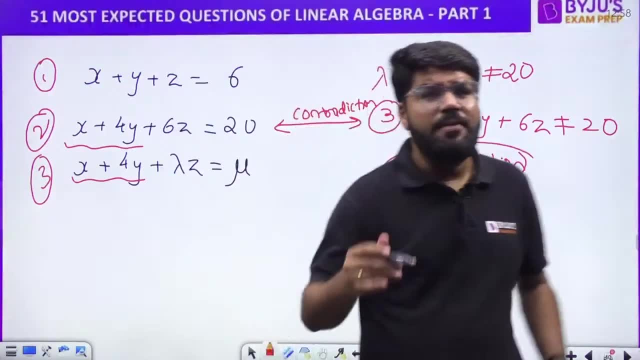 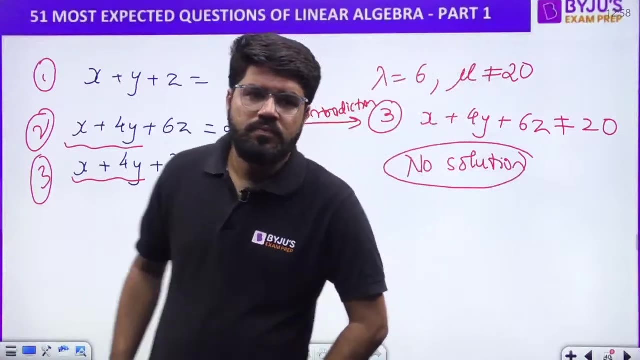 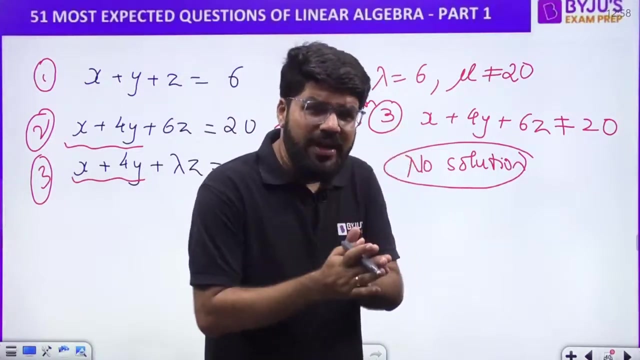 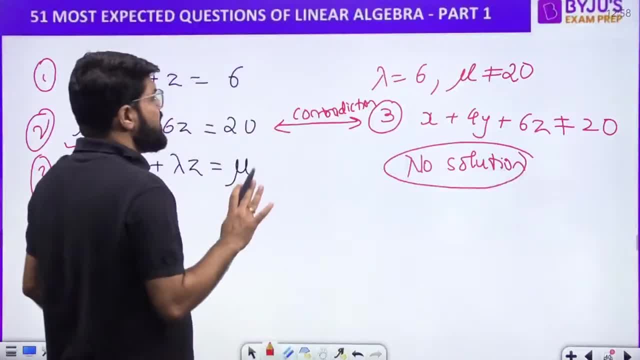 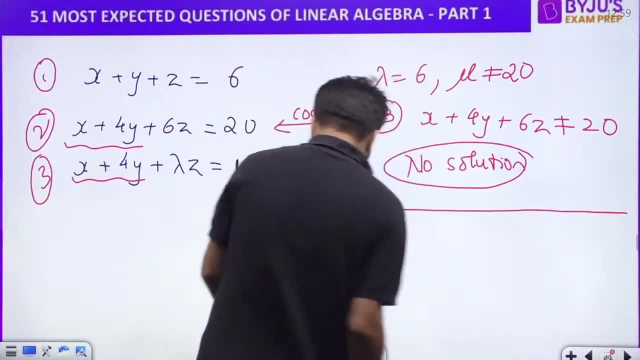 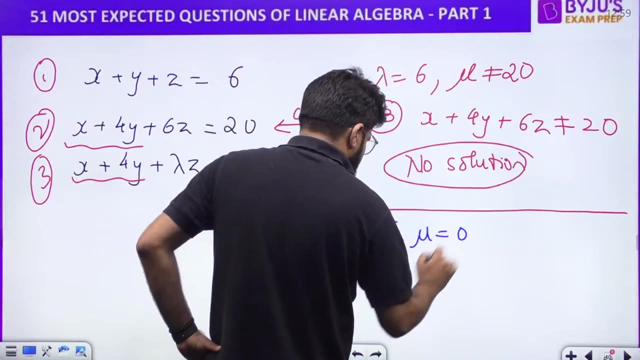 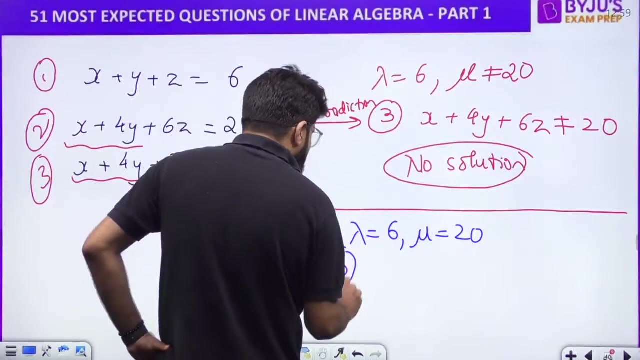 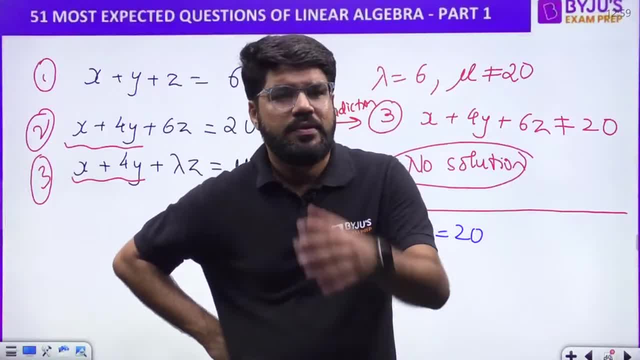 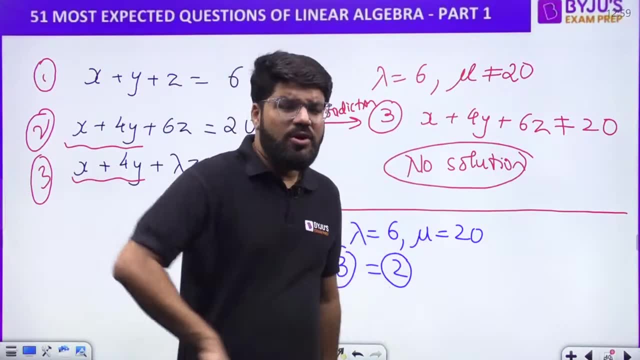 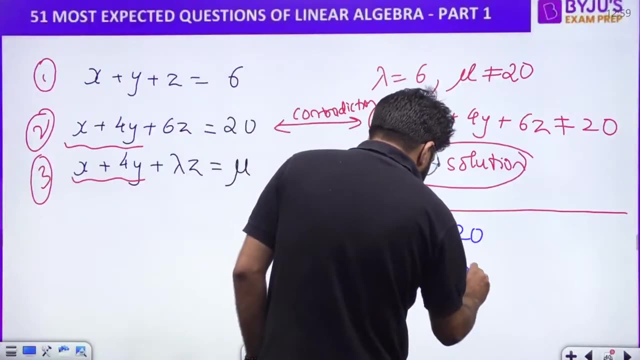 number two. So there are only two equations, right, Okay, Yes, yes, yes, Prashant, This is non-homogeneous. only Tanjai Surya. Okay, So there are dependent equations. Total equation. 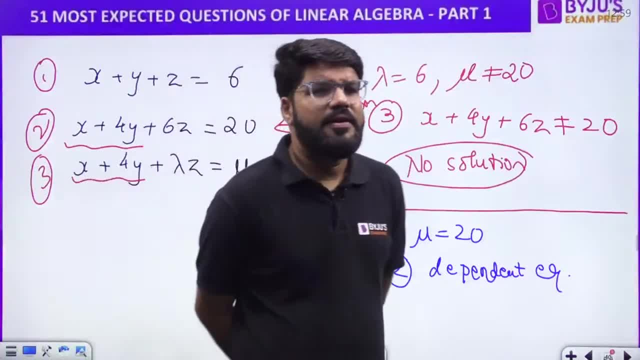 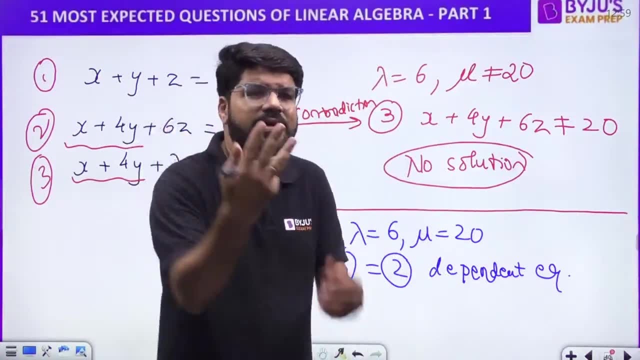 is dependent. Total equation is dependent, Correct? So what is the race? What is the result? What is the result? Okay, There are three variables, but there are only two equations. Third, there is no third equation. The third equation was just written to fool you. If 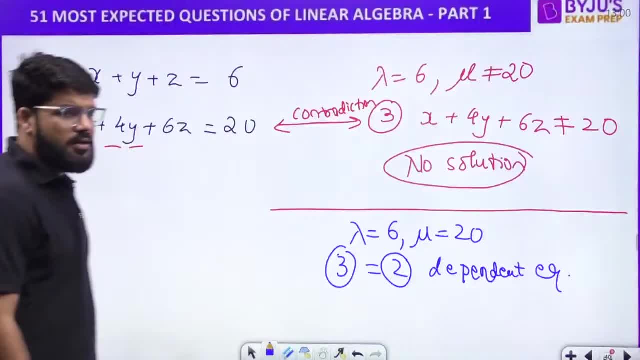 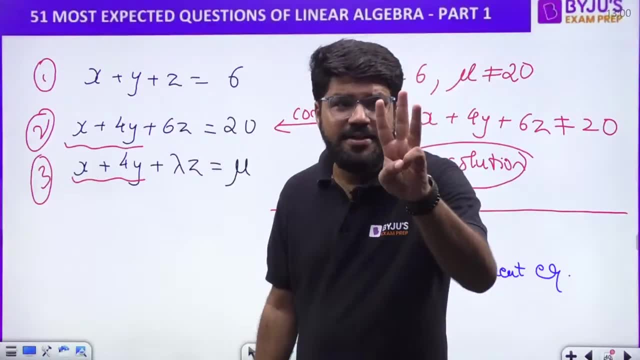 lambda is 6 mu, equal to 20, there is no third equation. There is no third equation. So system will give you infinite solutions. right To solve for three variables. you need at least three independent equations, So system will give you infinite solutions. So dependency. 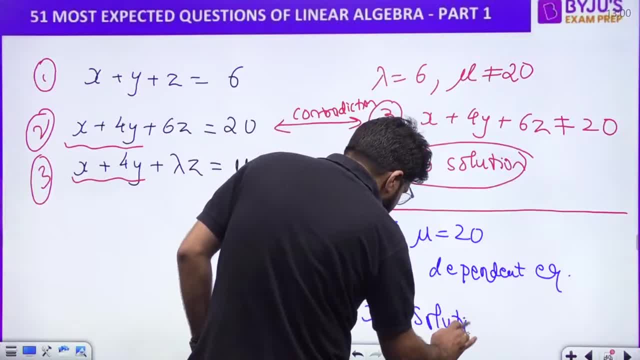 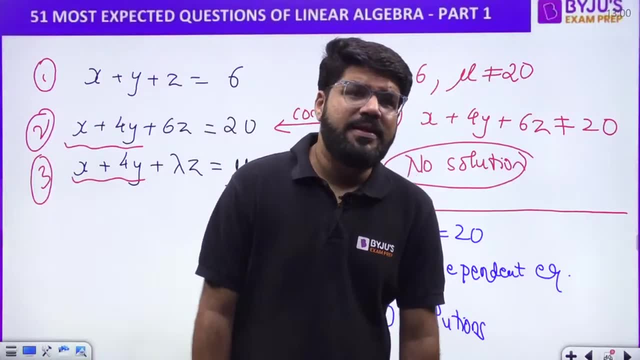 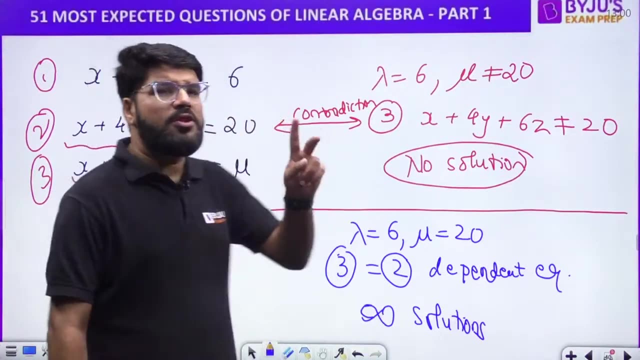 meh system will give you infinite solutions. Infinite solutions If you go by the rank method. if you go by the rank method, right, If you go by the rank method, then what you can say- Rank of A and rank of A- is to be. both will be equal and 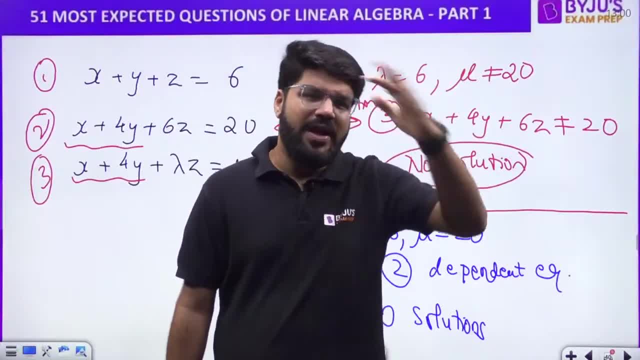 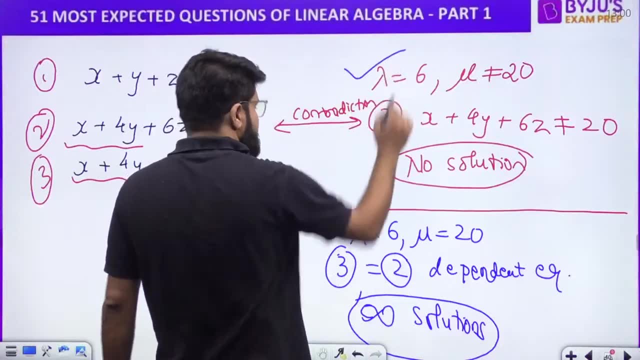 equal to 2, equal to less than number of variables, But no need of rank method. Apply the shortcuts, Apply the shortcuts. So for infinite solutions. this is the answer For no solution. this is the answer For unique solution. determinant method. that is the answer. All three answers. 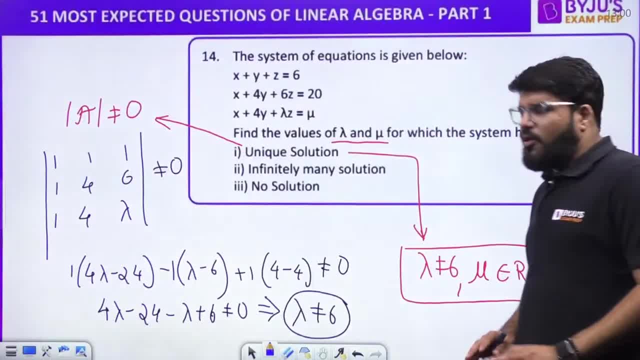 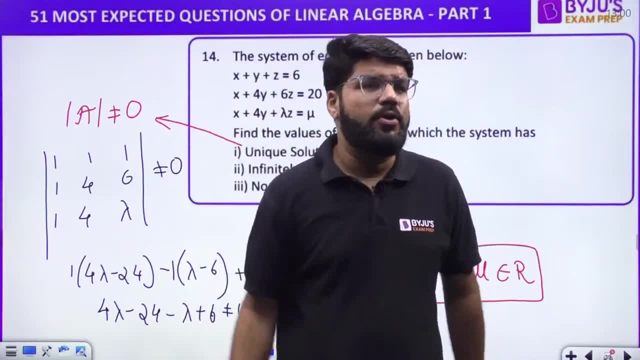 are written right. So, guys, now for most of the questions, I have made the process simple. Everybody just quickly recall: revise, unique solution, only one calculation, determinant not equal to zero, No solution, contradiction, infinite solution, dependent equations. If you apply these three tricks, 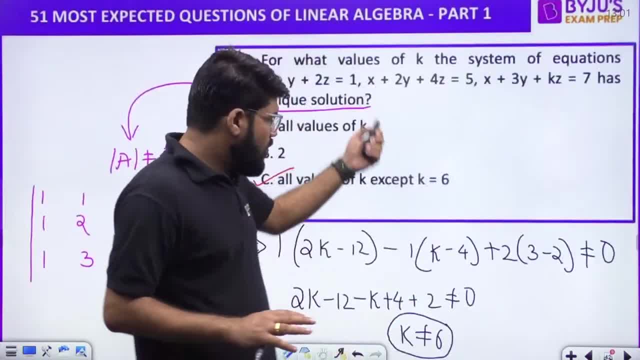 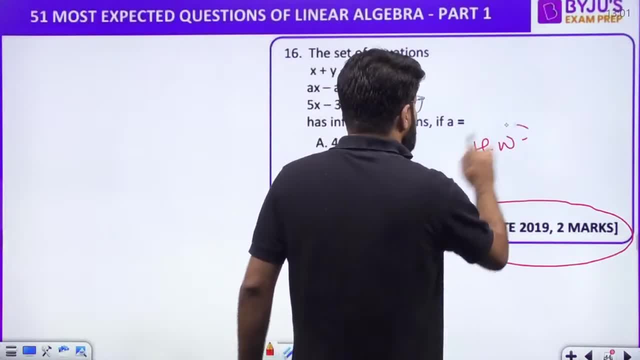 and these three logics, then most of the questions are simple. Okay, although we have solved in details. also Okay, now I'll give you it's a gate question for reference, just to show you how easy it is. Please take this as homework. Infinite solutions. Think about. 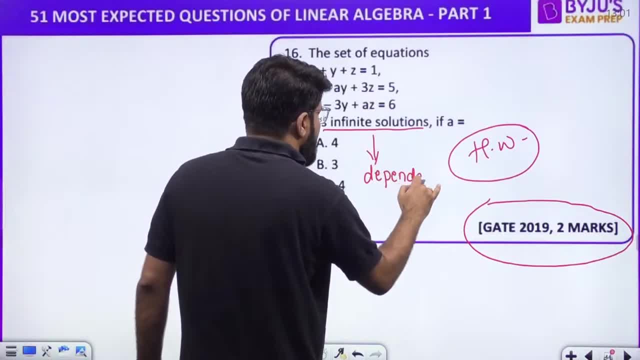 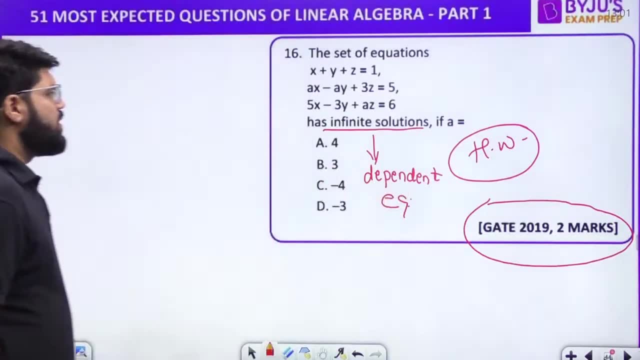 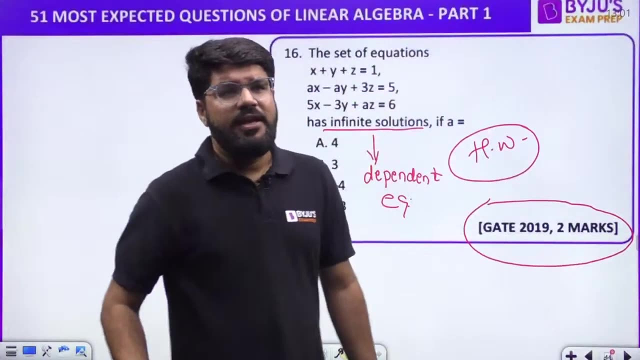 dependency. Kaise solve karenge? The trick is not about the rank method. Trick is dependency, Dependent equations. Try to see dependent equations. Try to make dependent equations Very clearly, very clearly. you will get the answer within few seconds If you think about dependency. 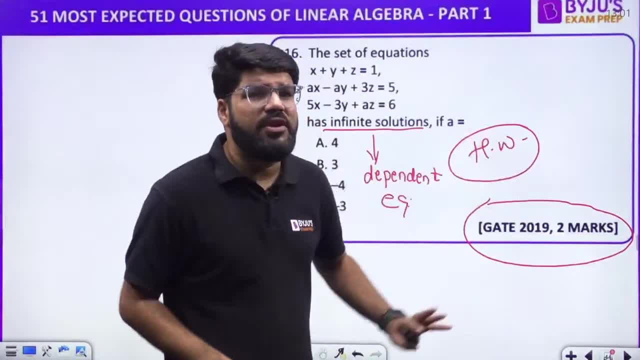 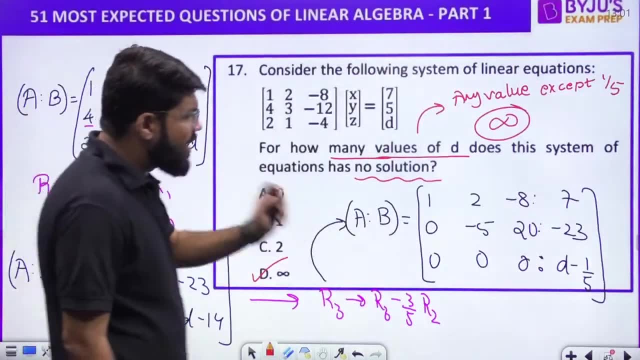 it's a two mark question. I want you to try. That is why I'm not discussing and intentionally I'm giving you a gate question as homework for reference. Otherwise rest were different questions. This I have shown you by the proper rank method: Yeh pura rank method. 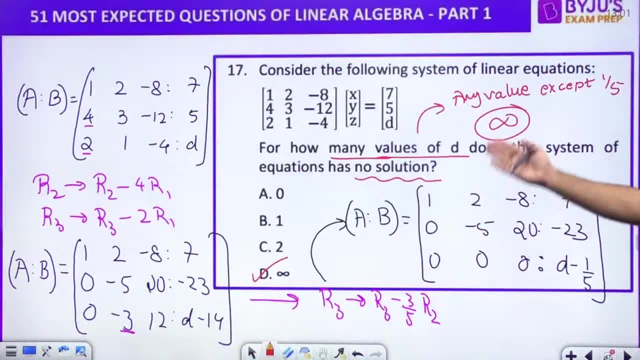 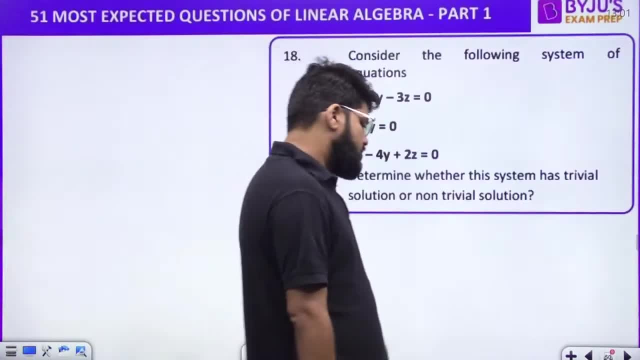 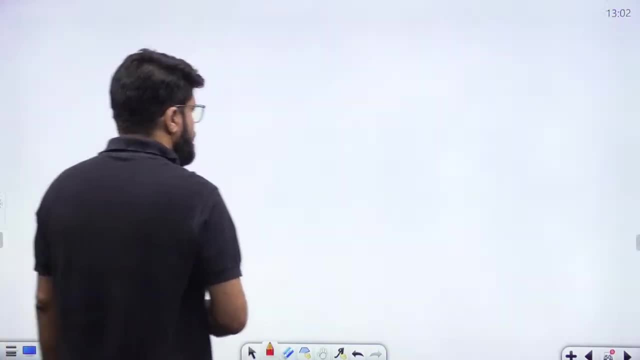 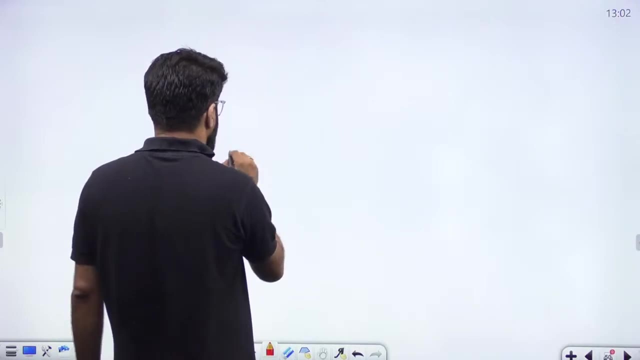 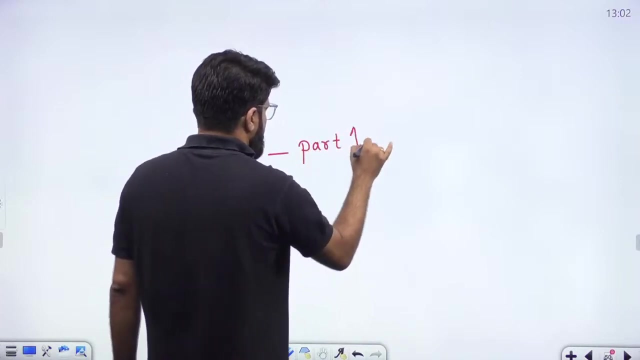 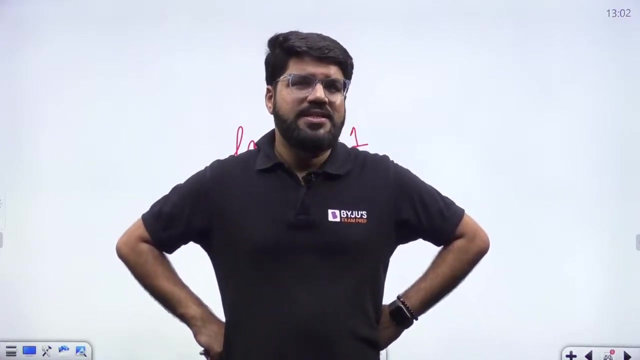 to next question. Let me also tell you the password for today's PDF. There are many few more questions left for today, but before that I will share you the password for today's PDF. Yes, guys, I am going to share you the PDF. 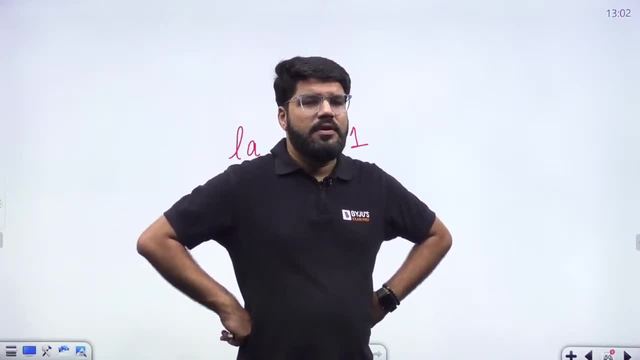 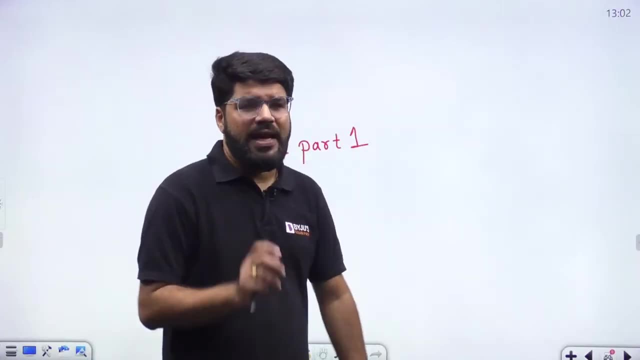 I am going to share you the PDF in my telegram group. The PDF is going to be password protected and the password is going to be LA underscore part 1.. A simple password I have framed today, LA underscore part 1. For tomorrow- does not mean that it is going to be password as part 2, tomorrow it will. 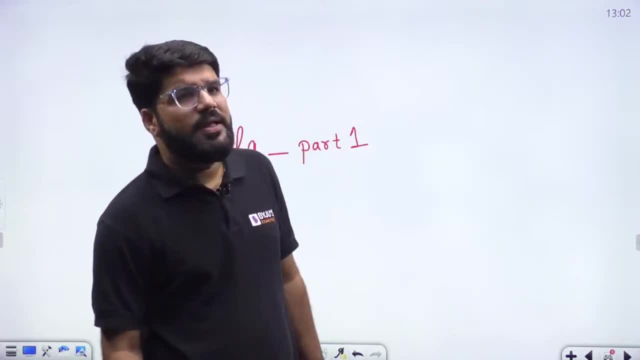 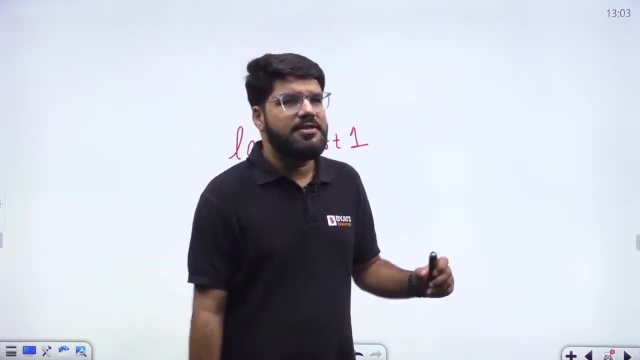 be something else, But for today, LA underscore part 1 is going to be the password for today's PDF. You can download from my telegram, put the password and then you can access the PDF. Without the password you cannot access the PDF. Next question: 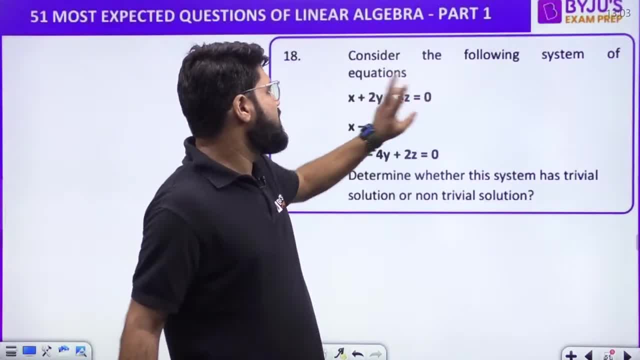 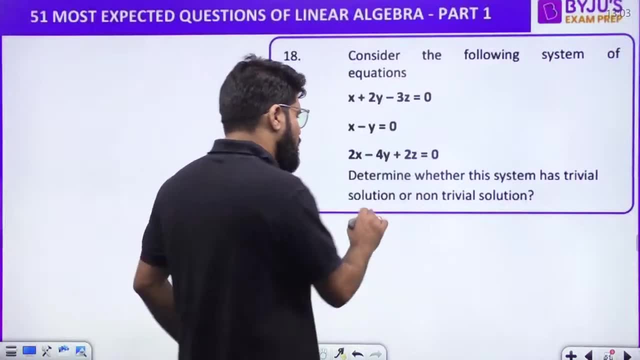 Consider the following system of equations: x plus 2y minus 3z equal to 0, x minus y equal to 0, 2x minus 4y plus 2z equal to 0.. And whether the system has trivial or non-trivial solution. 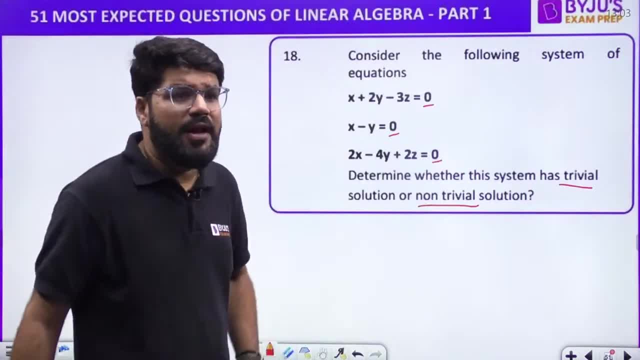 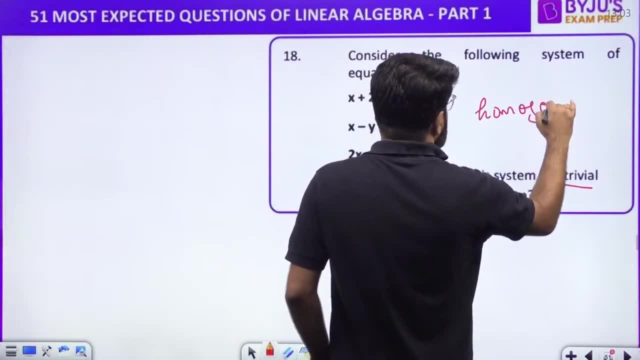 So see 0,, 0,, 0,. right hand side, everything is 0. So I am turning now to when all the right hand side coefficients, all the right hand side constants are 0, we call the system as homogeneous. Already I defined in the beginning this is known as homogeneous system of equation. 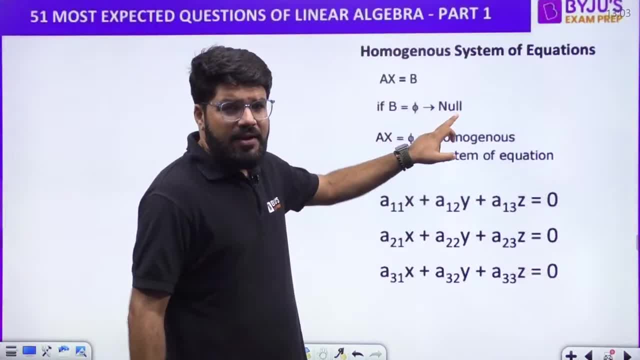 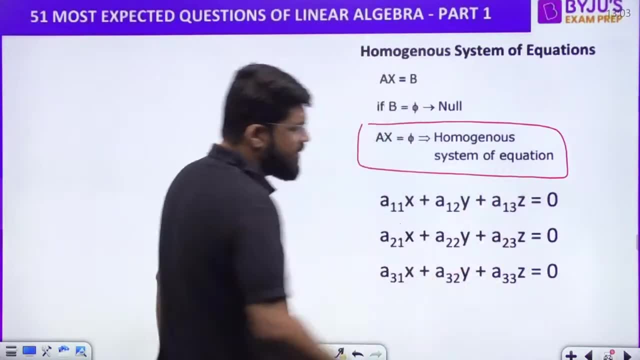 Have a look into this: Ax equal to b if b is null. if b is null, we get ax equal to 0 and ax equal to null, and that is what is known as homogeneous system of equation. Okay, All right hand side coefficients are 0. 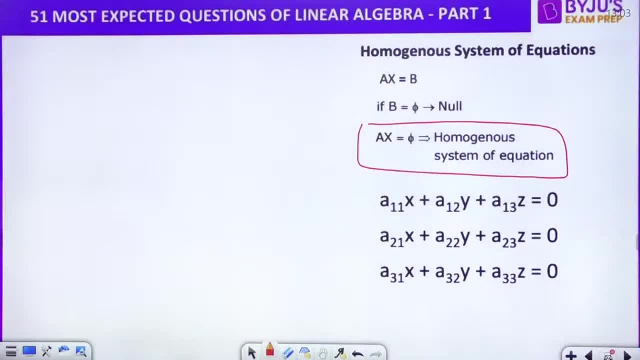 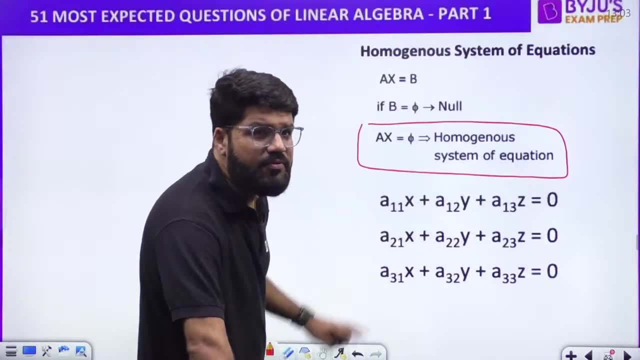 All right hand side coefficients are 0.. So what all you need to know about the homogeneous, What all you need to know about the homogeneous system of equation- We will understand that here- What all you need to know about the homogeneous system of equations. 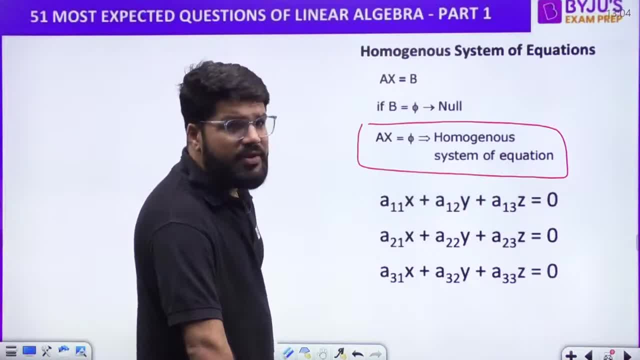 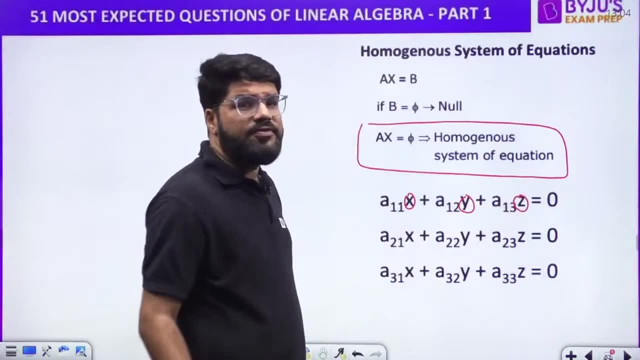 Please have a look at this. This is homogeneous system of equation. Now put x y z equal to 0.. What is the meaning of solution? Solution means the value of x y z which will satisfy all the three equations. 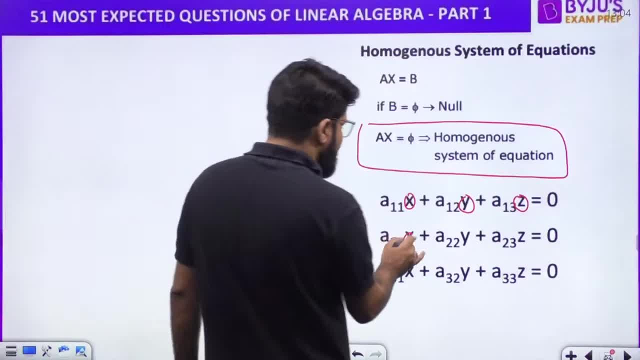 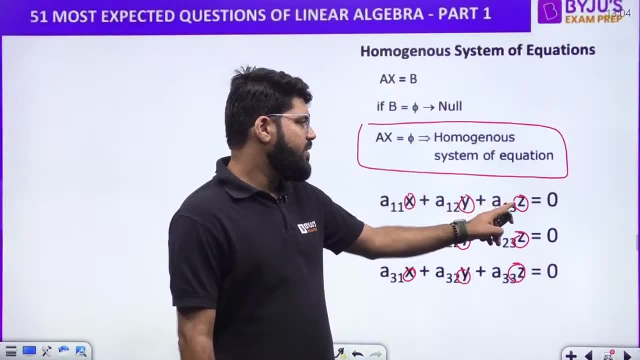 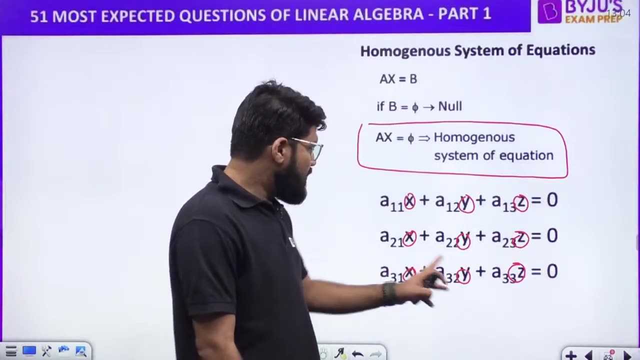 Let us see: Solution means the value of x, y, z, which will satisfy all the three equations. So I am trying 0, 0, 0.. Okay, So 0 into a11 into 0, a12 into 0, a13 into 0. 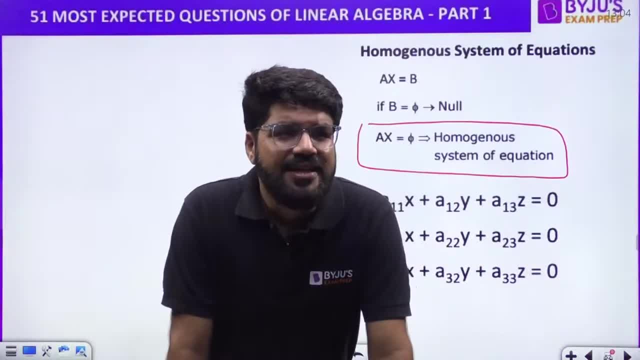 It is all 0 right hand side, 0 satisfied. Similarly, here also: 0 plus 0 plus 0, equal to 0, satisfied. 0 plus 0 plus 0, equal to 0, satisfied. So if I take x, y, z, 0, 0, 0, it satisfies all the three equations. 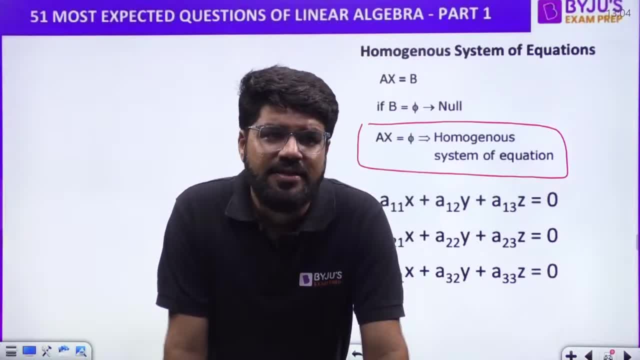 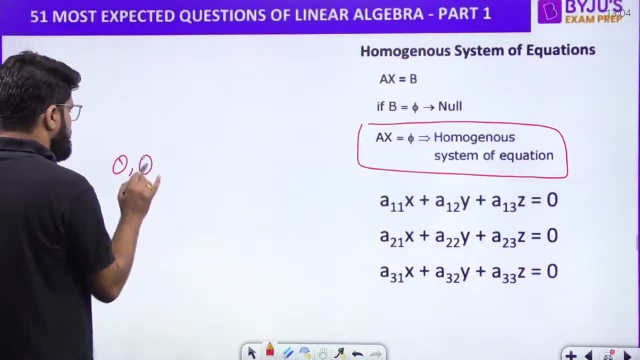 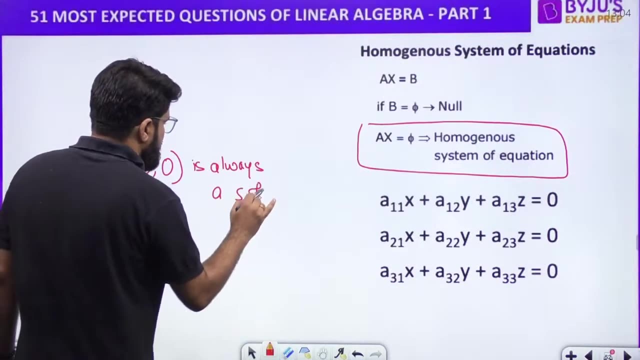 It satisfies all the three equations and hence it is a solution. 0, 0, 0 satisfied all the three equations and hence it is a solution. Hence it is a solution. Can I say na? 0 0 0 is always a solution. no matter what Matlab, this system can never be inconsistent. 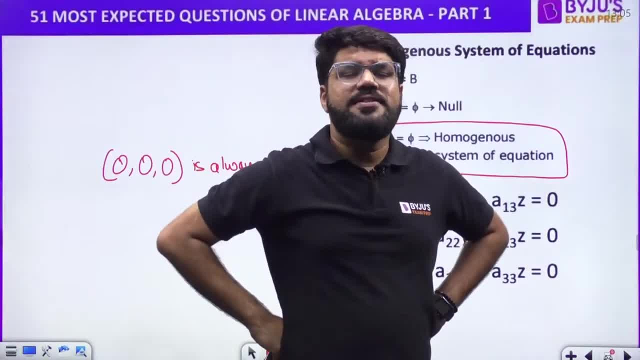 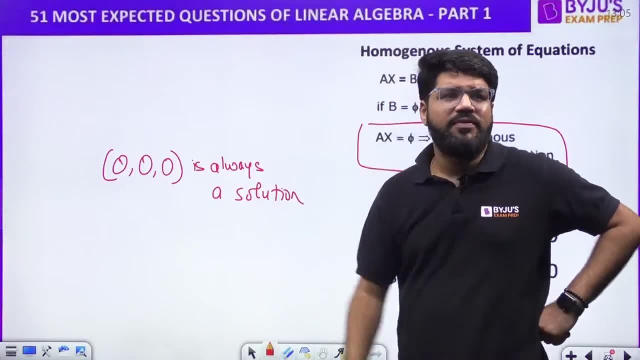 What is the meaning of inconsistency? What is the meaning of inconsistency? The system has no solution. But here it is not like that. 0 0, 0, always one solution, minimum. I am giving you, Guaranteed, confirmed. one solution is always given to you. The system is never. 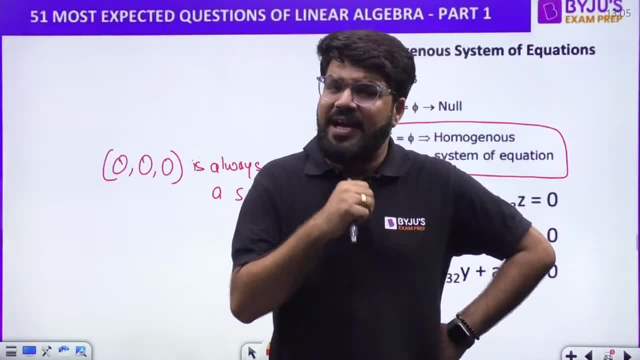 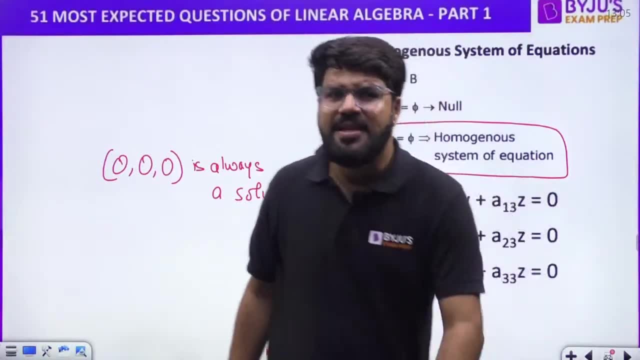 inconsistent System is consistent. Now the question is whether it has only one solution- 0 0 0- or it has more than one solution, or it has more than one solution. Now, everybody listen. if it has only one solution, if it is unique solution, listen to me clearly. if it, 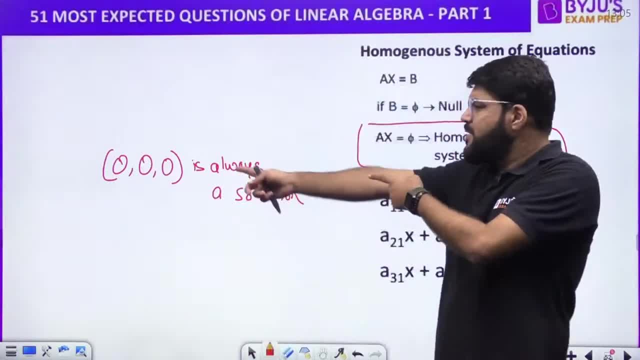 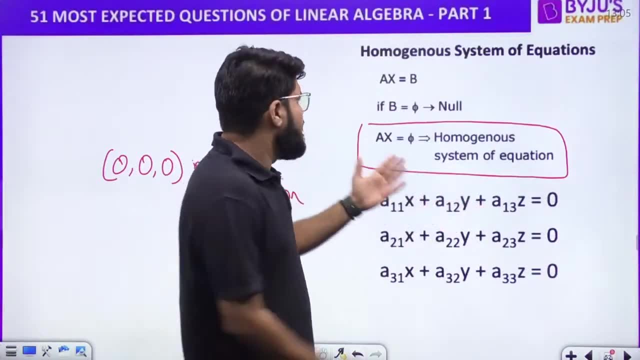 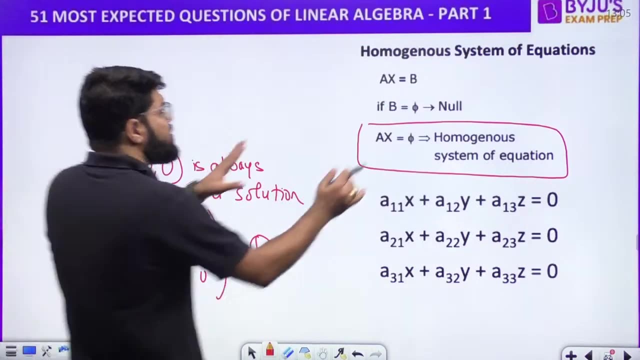 has unique solution means it has only one solution. But what is that one solution? 0 0 0.. That is always a solution. Does this solution depend on the system? Right? 0 0 0 means x is 0 0 0.. So x is also a null vector. So it is very logical na You take a matrix. 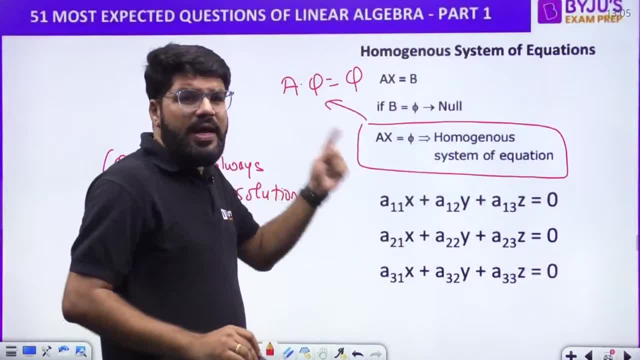 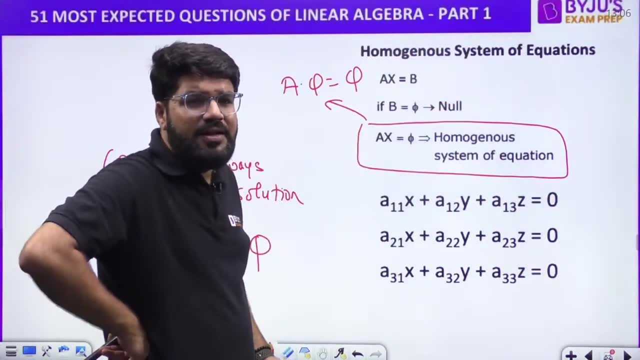 you multiply by null, you are going to get null. Null means zero. A into zero is always zero. A into zero is always zero. Is there any new discovery, a new discussion here? That is what you know from the childhood: Multiply anything by zero, you get zero. 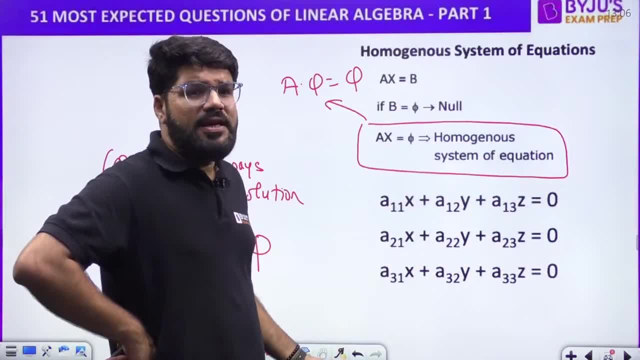 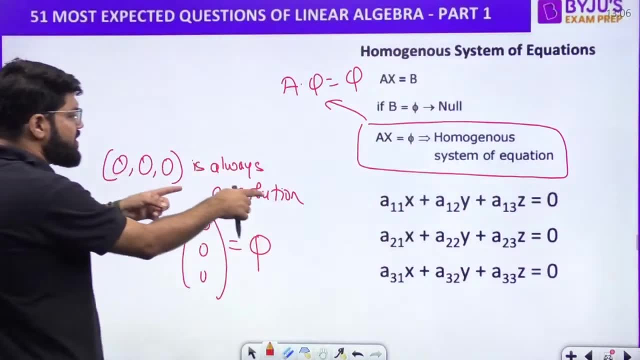 So what is new here? That is meaningless. That is meaningless. So if the system has unique solution means the system has only one solution. But we also know that 0 0, 0 is always a solution. So what is that one solution? What is that one solution? 0 0, 0.. 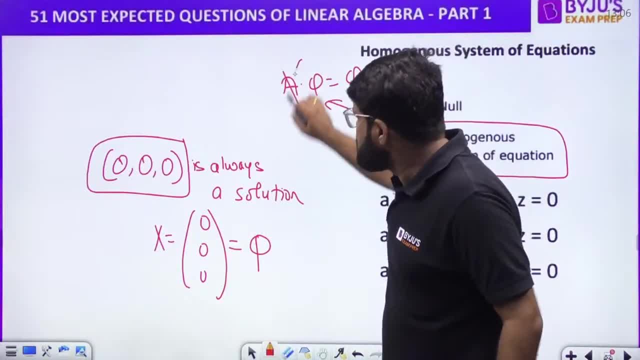 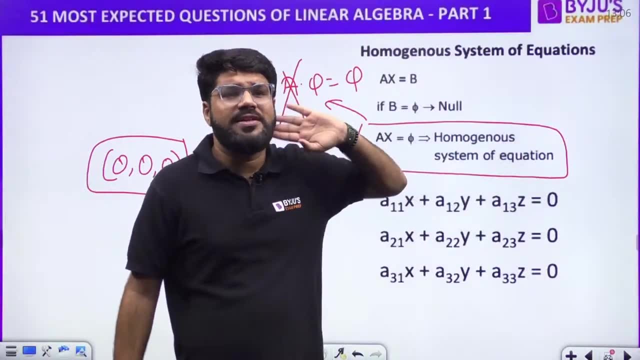 But that is meaningless. Independent of the matrix, say, there is no role of the system matrix here. There is no role of the coefficient. Whatever coefficients in the world you bring, this system always have 0 0, 0 as a solution. So whenever the system has 0 0 0 and 0 0 0. 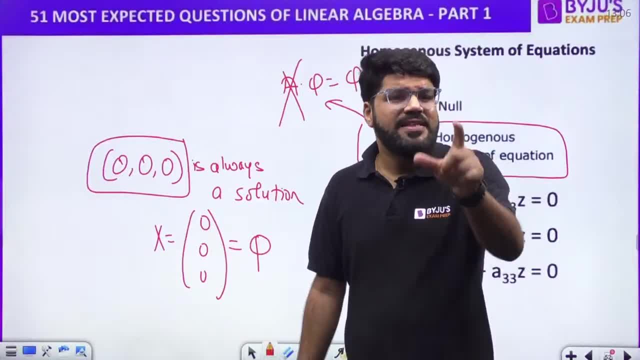 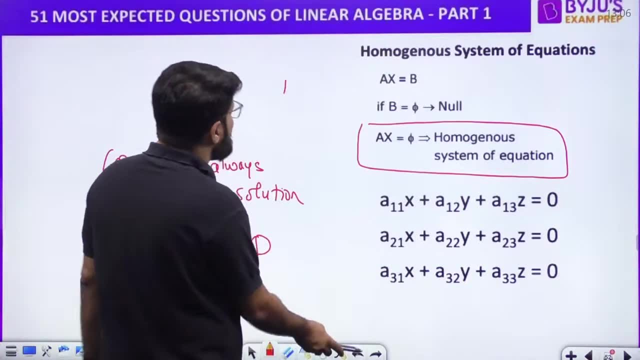 as the only solution. then the system is said to have, then the system is said to have trivial solution. Then the system is said to have trivial solution. What is the literature meaning of trivial? Trivial means something which is meaningless, which is of no additional value. 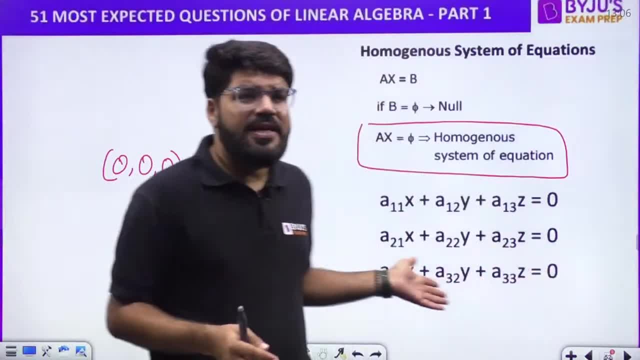 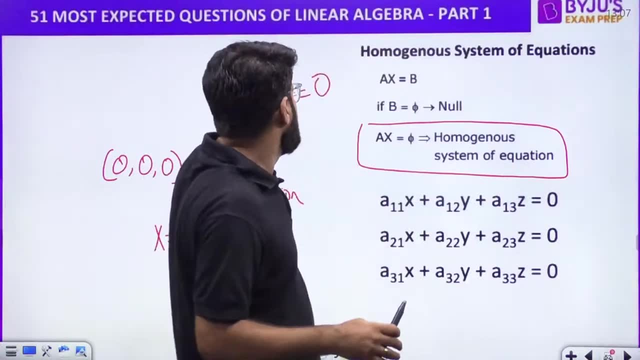 which is not of much use. Right, That is what is the case happening here. A into 0 is 0.. What is new? Nothing new, Meaningless. We all know from childhood that A into 0 will be 0. Right. So whenever the system has unique solution. 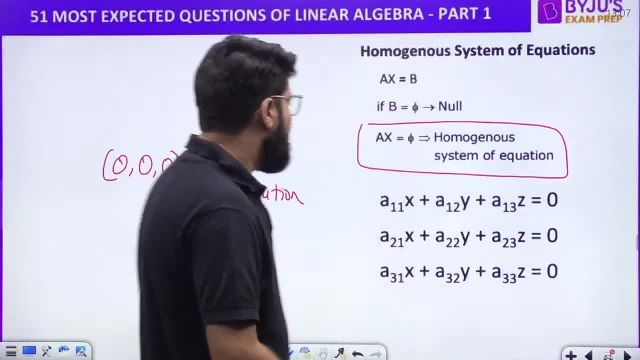 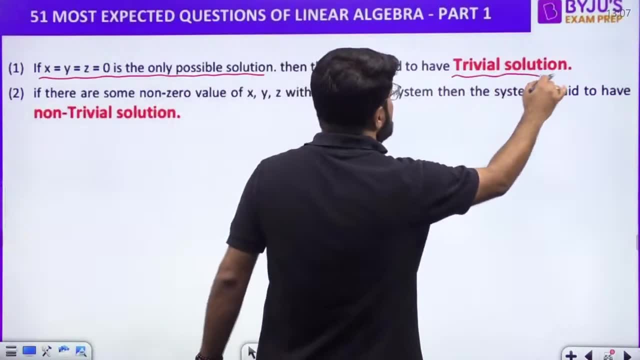 it will be said to have trivial solution here. It will be said to have trivial solution here. First, let us come to this: If 0 0, 0 is the only possible solution, then the system is said to have trivial solution. It is the only possible solution, Right? So this is related. 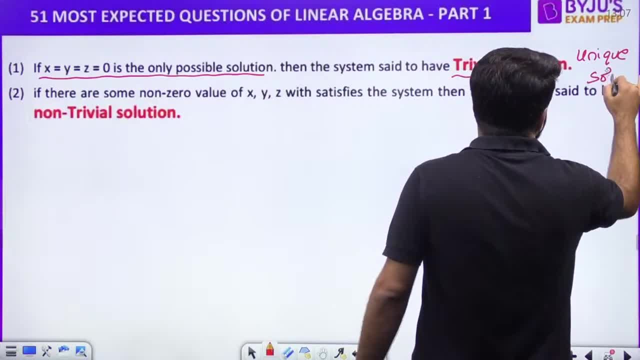 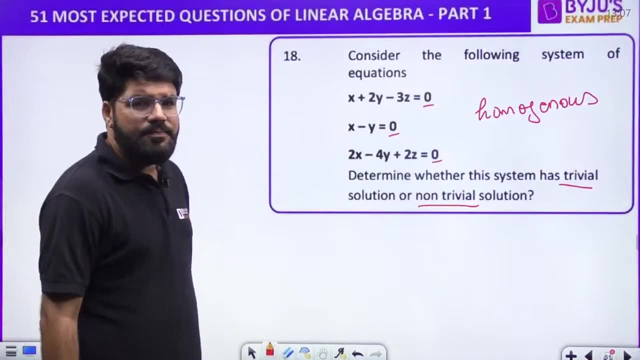 with unique solution. This is related with unique solution. Now understand some more things. Ok, This is one point. Ok, If I again turn back to the question, I have written the question here for you once again. Look into this. This is the question given to me. 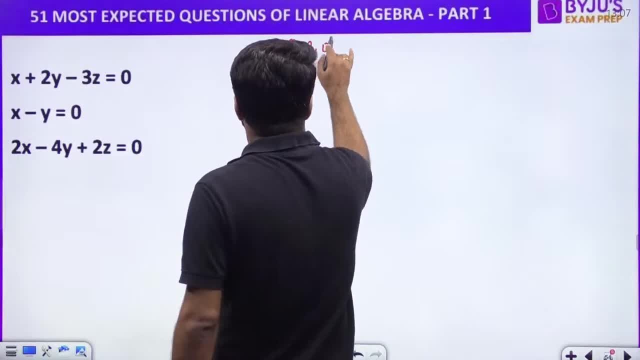 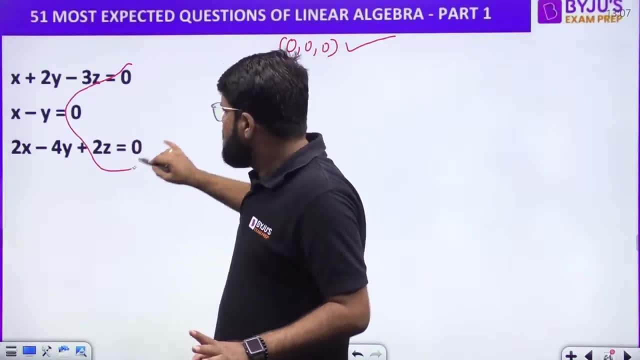 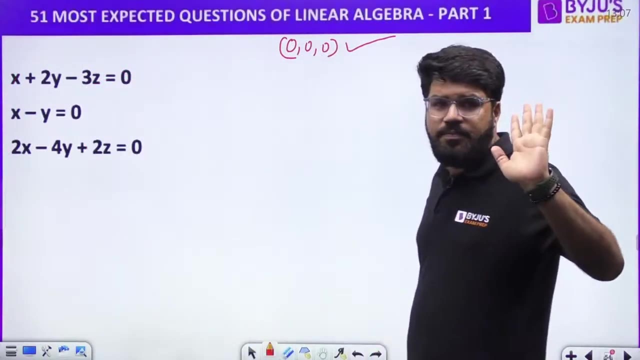 0, 0, 0 is always the solution. It is the solution. It is blindly. I can say See, blindly, looking into, you know, looking into the coefficients, I can say that without looking into coefficients I can say 0, 0 is the solution. Ok, That is waste, Ok, but here look into this, Here look. 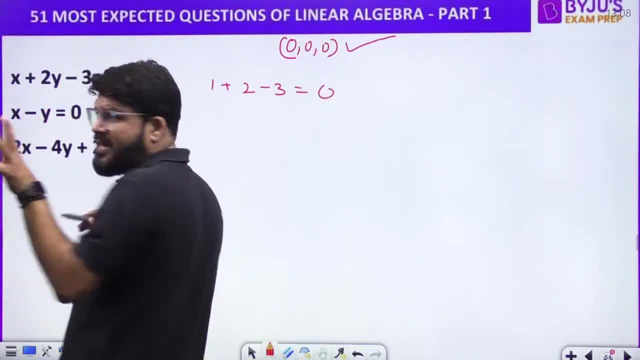 into this: 1 plus 2 minus 3 equal to 0.. Intentionally, these equations have been framed for easy numbers. Second, 1 minus 1 equal to 0.. Next, 2 minus 4 plus 3 equal to 0.. Next, 2 minus 4. 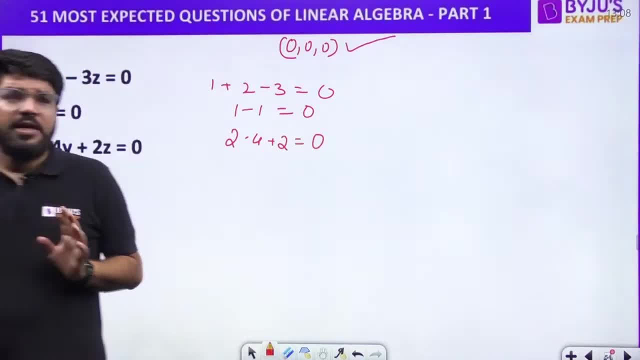 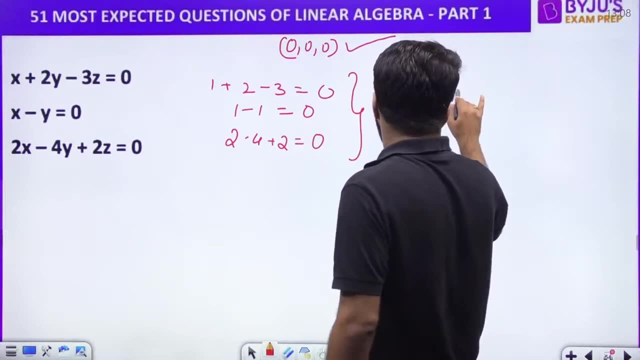 plus 2, equal to 0.. Satisfied, All are satisfied. So if I put x, y, z, all equal to 1, 1, 1,, still I get a solution. So what did I get from here? 1, 1, 1 is also a solution here. 1, 1, 1.. 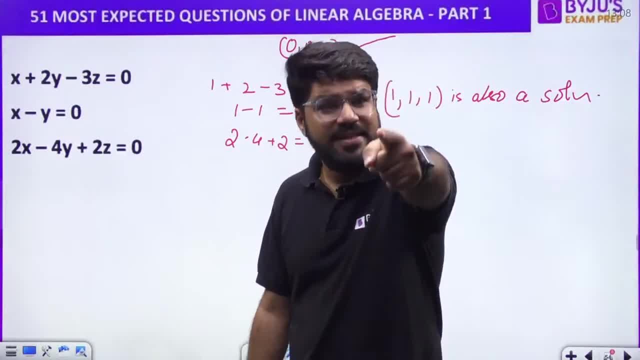 If you satisfy 1, 1, 1,, it is satisfying all the three equations. That means it is a solution of linear system of equation. So 1, 1, 1 is also a solution, right. 1, 1, 1 is also a. 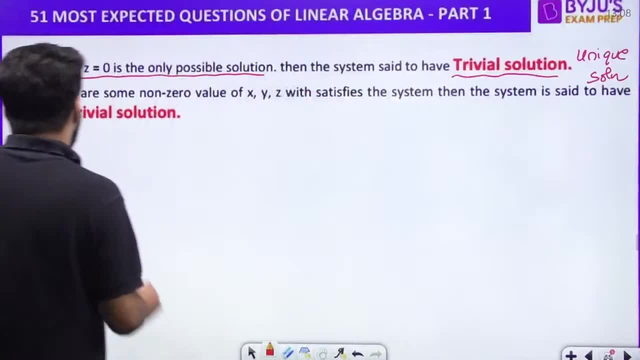 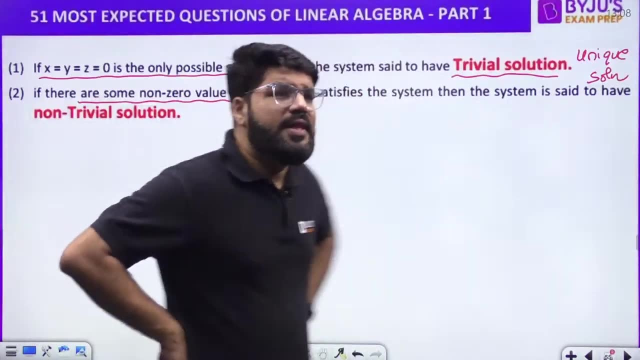 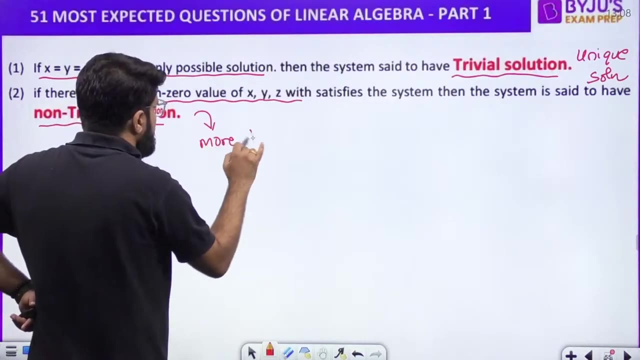 solution here. That means you have some non-zero solution here. If there are some non-zero solutions also, if there are some non-zero solutions also, then the system will have said to have non-trivial solution. Okay, So non-trivial solution means more than one solution. 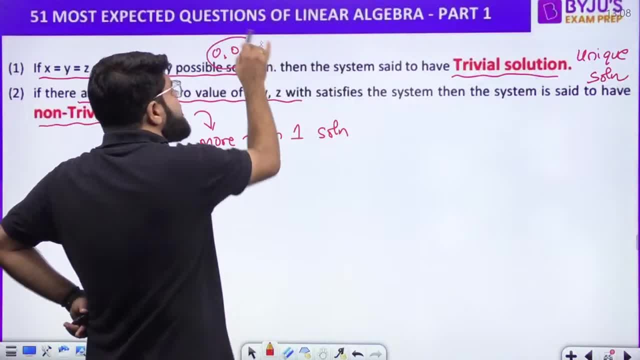 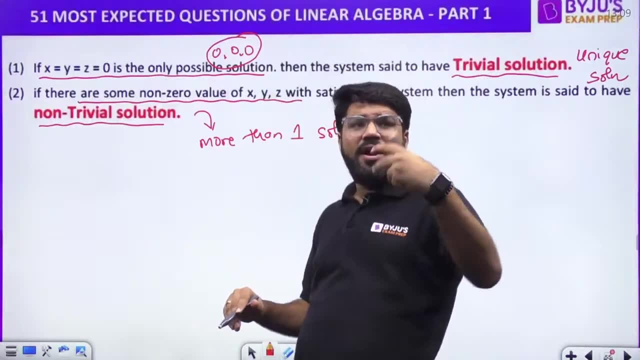 because this is always fixed. You can't remove it. But other than 0,, 0,, 0, if you have some non-zero values, then you can't remove it. So if you have some non-zero values, then use also Matlab. you have more than one solution. You have more than one solution, More than one. 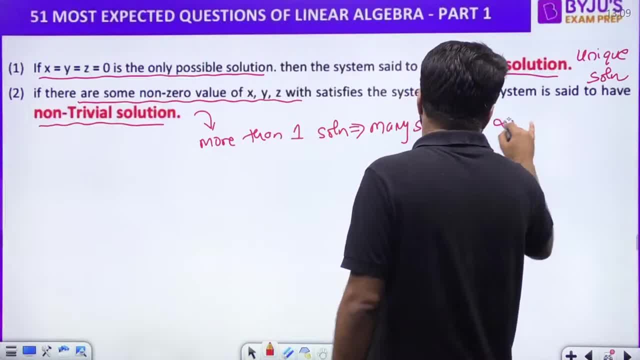 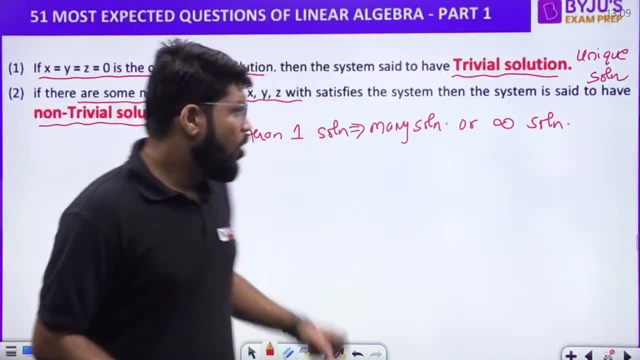 solution is referred to as many solution or infinite solution. Whenever a linear system of equation has more than one solution, it will always have infinite solutions only. Okay, So non-trivial solution is related to what? Infinite solution, then Infinite solution, So have. 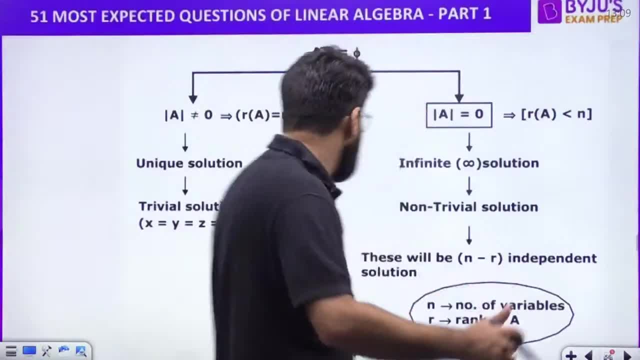 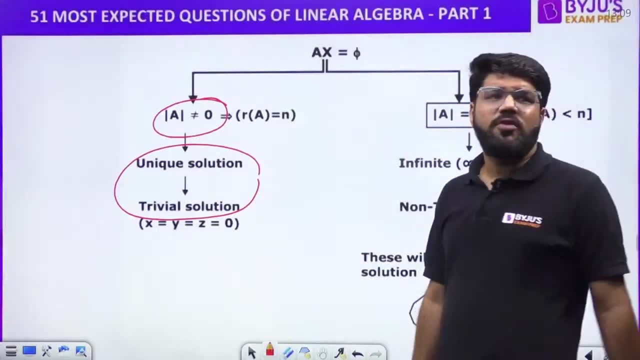 a look into the summary. Question is asking you: trivial, non-trivial. The summary is trivial: unique. What is the condition of unique? You already have studied. You already have studied What is the condition of unique? Mod A not equal to zero, Mod A not equal to zero. But then we 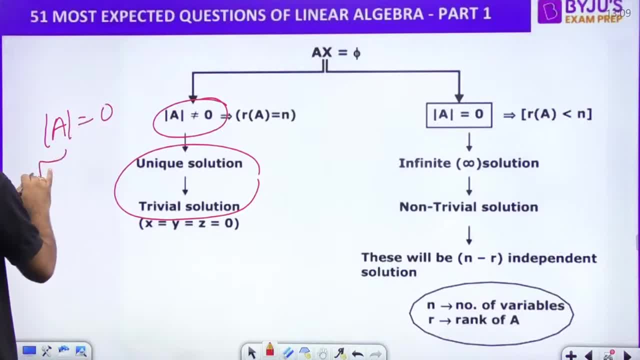 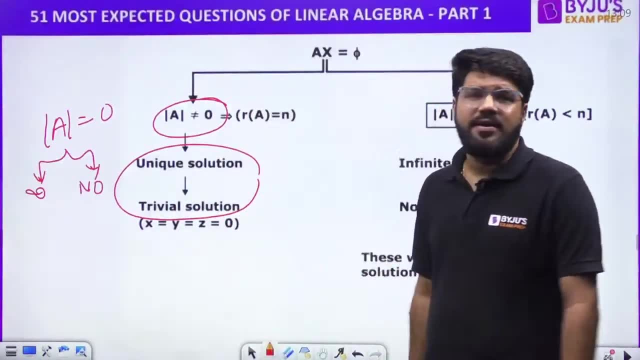 learned. but then we learned: if mod A equal to zero, then the system can have infinite solution or no solution. Mod A not equal to zero is unique. Confirm Unique means trivial here. But if mod A equal to zero, system can have infinite or no solution, But in homogeneous system of equation. 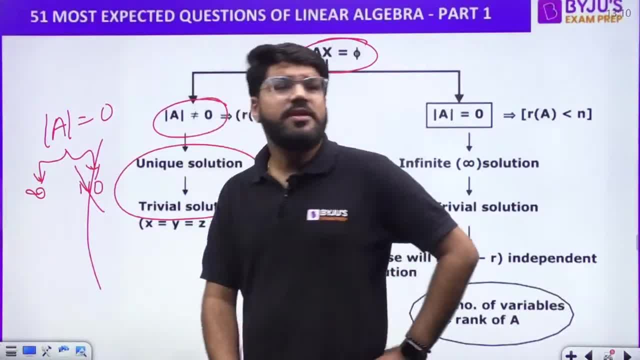 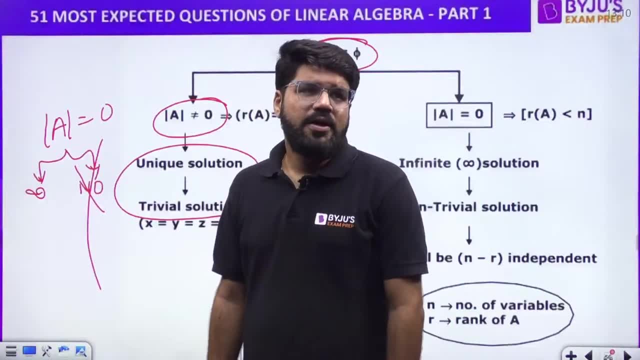 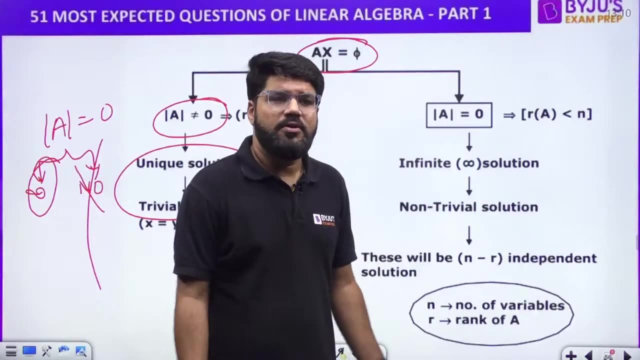 but in homogeneous system of equation, no solution discarded. Already explained the first thing: There is no possibility of the inconsistency Right. So if mod A equal to zero, what is the only thing left? Infinite solution. Infinite solution related to non-trivial solution Question. The whole story is over, So trivial or? 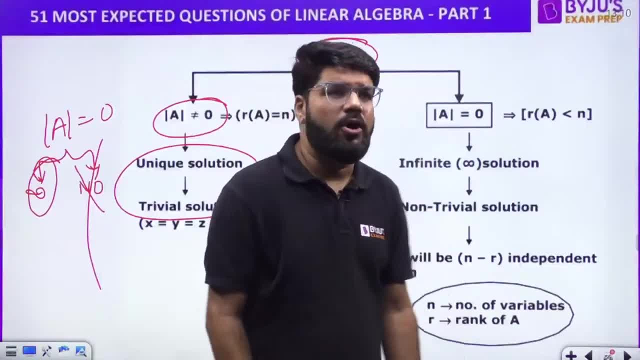 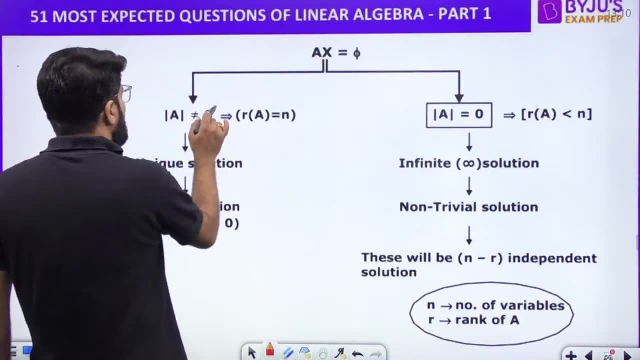 non-trivial. it is just one determinant, No rank. This is much more easier than the non-homogeneous. also. It is much more easier than the non-homogeneous also. Right there. So determinant of A not equal to zero. 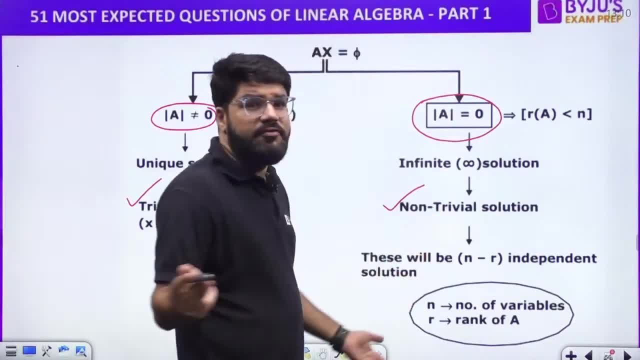 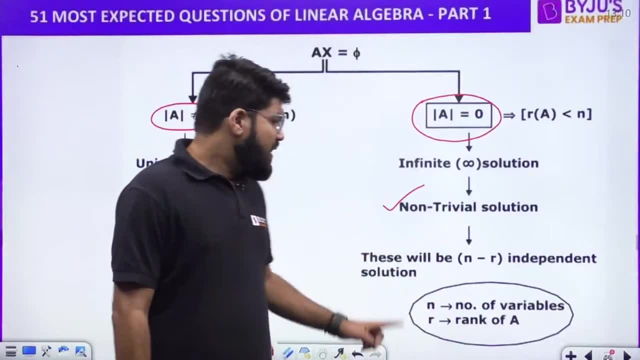 Non-trivial solution. Deternant of A equal to zero. Non-trivial solution: Finished, The story is so simple. as compared to non-homogeneous. also, Right, If the system is non-trivial. just note down one more formula: The system will be having n minus r independent solutions. Right, There will be. 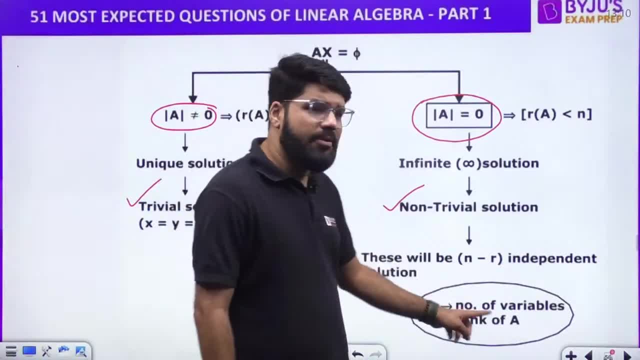 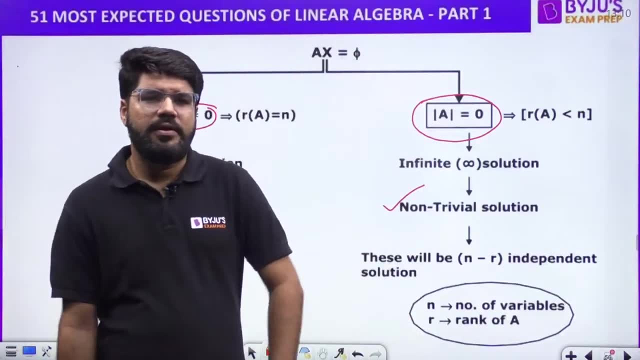 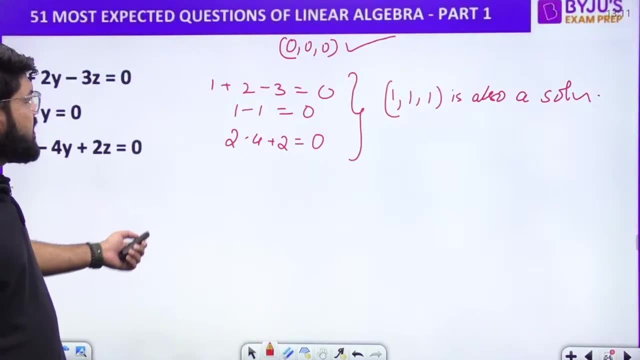 non-zero solutions, out of which n minus r will be independent. n is the number of variables, like three in the previous case. r is the rank of the matrix which you know to calculate, Which you know to calculate Right. So yeah, So this is what I say, This is also a solution. So here you have non-trivial. But how do? 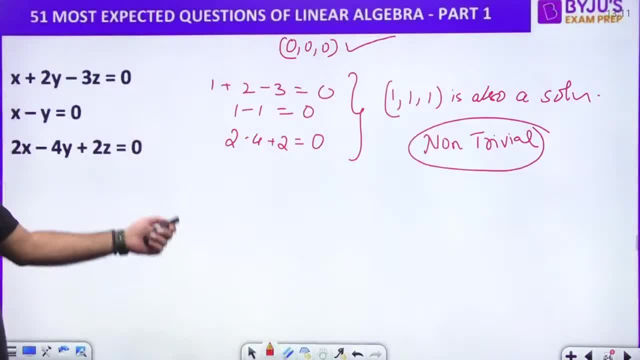 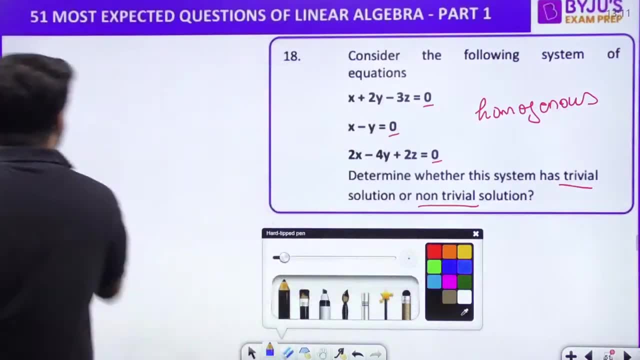 you check by the method. This is explanation. How do you check by the method? Let us go back to the question. Let us go back to the question. Question: Trivial- non-trivial. I will only check the determinant of A. I will only check the determinant of A Whenever I see the question. 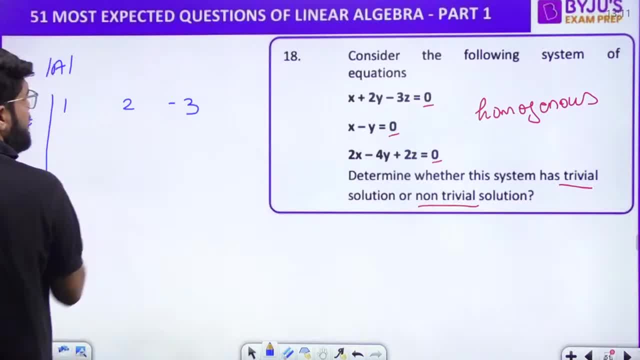 I only need to check the determinant of A, So 1, 2, minus 3.. 1, minus 1.. Z, absent, is zero, 2 and minus 4.. Okay, Let us check this determinant. This is becoming 1, minus 2, minus 0.. Minus of 2.. Minus of 2.. 2 minus 0. 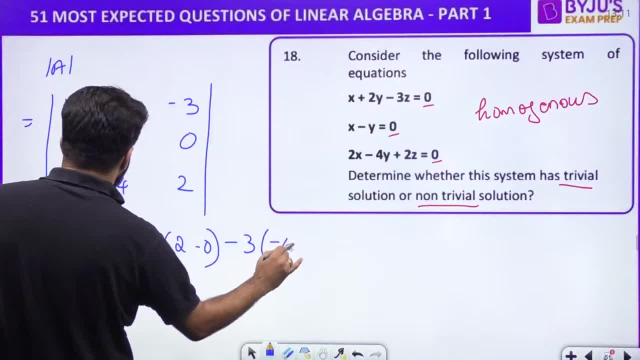 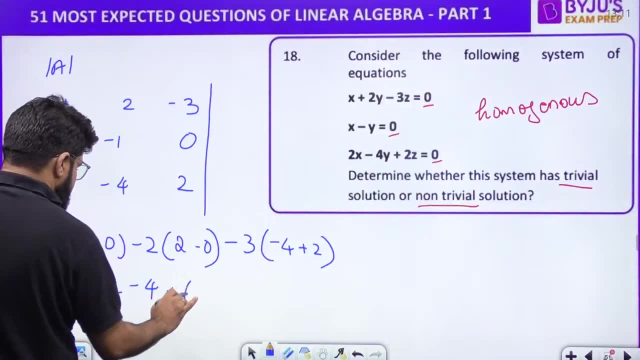 Correct: Minus of 3.. Minus 4. Plus 2.. Ketna huba, ye, This is minus 2.. This is minus 4.. This is minus 2 into minus 3 plus 6.. Yeah, It is equal to 0.. Because the determinant equal to 0. 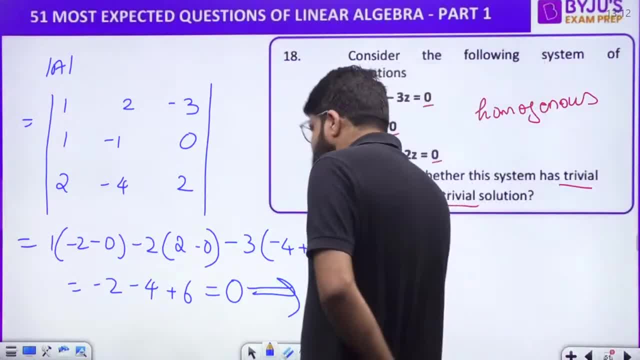 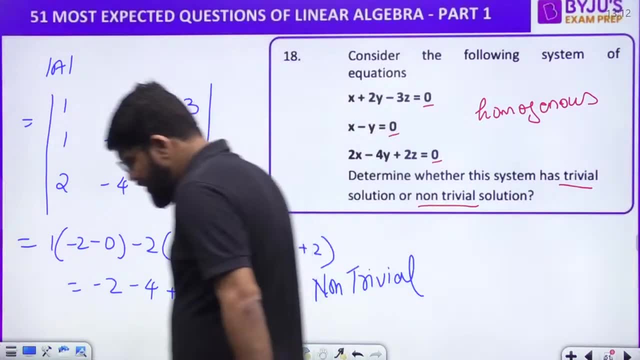 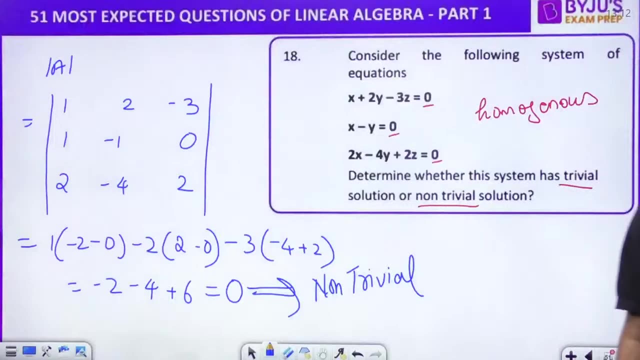 Because the determinant equal to 0.. System is said to have. System is said to have infinite matlab non-trivial solution. The system is said to have infinite or non-trivial solutions. Right, The system is said to have infinite or non-trivial solution. That is it, Question closed. The system is said to have: 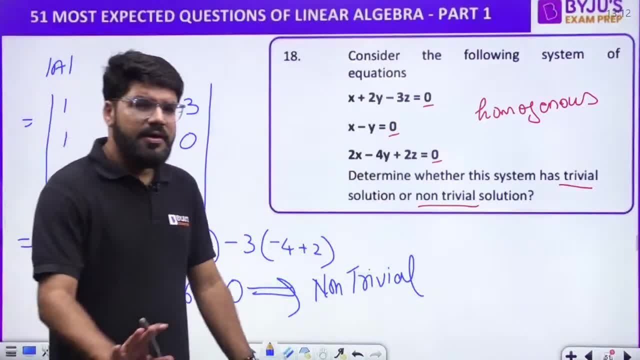 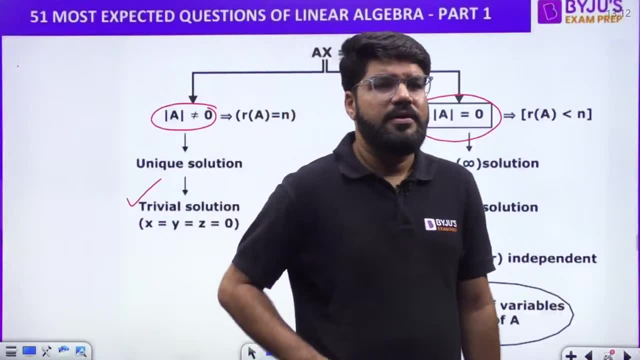 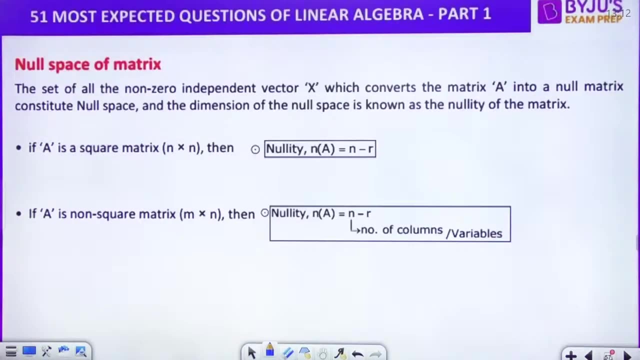 infinite or non-trivial solution. As simple as it could be. Okay, That is why this procedure is much simpler. Okay, This procedure is much simpler, Right? Yes, Yes, This is only for homogeneous Hania, Correct, Right. Null space of a matrix, Just few. 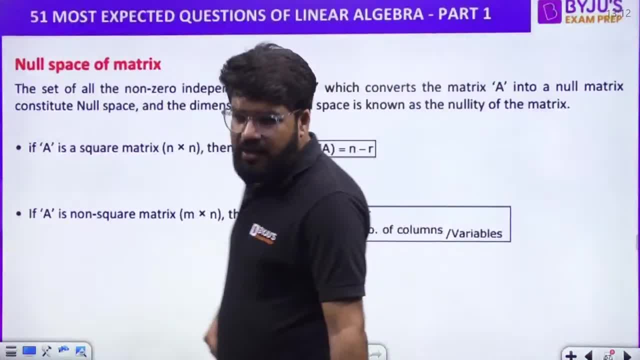 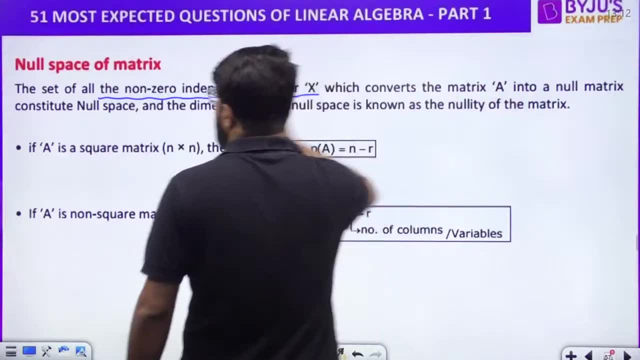 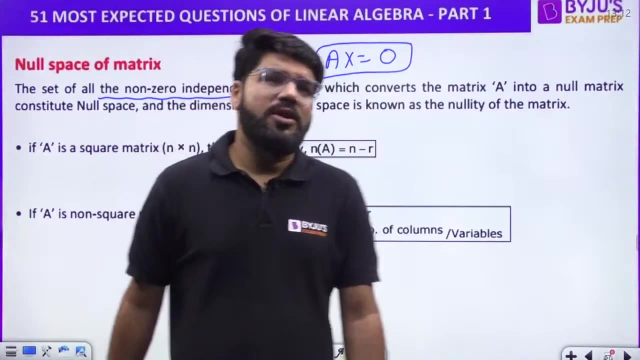 more definitions and then we will complete all the questions for today. Okay, Few more questions are left. All non-zero independent vectors: x which will convert the matrix A into null space. Right, So they go. We are solving homogeneous system of equation A, x equal to 0.. We are solving 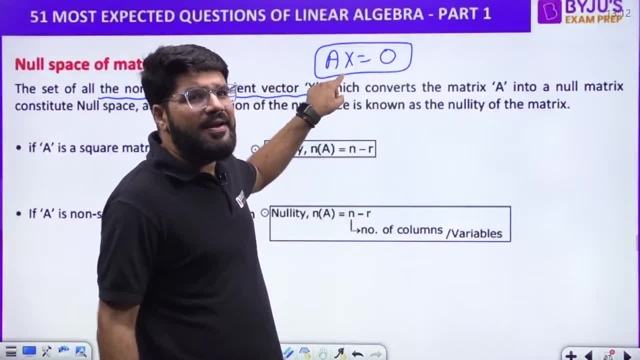 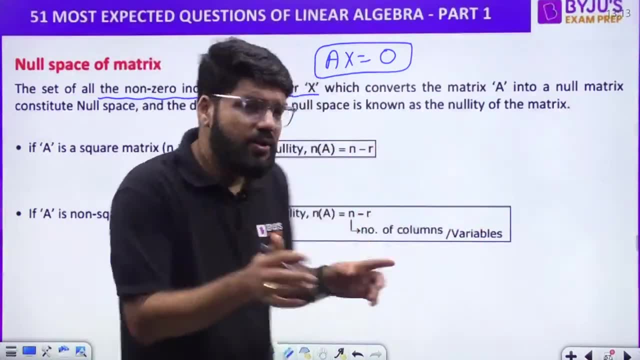 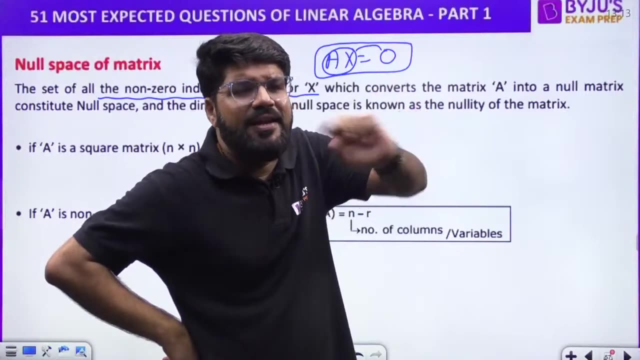 homogeneous system of equation, All those non-zero independent vectors x which will satisfy x equal to 0.. If they satisfy x equal to 0, that means what they are doing. What they are doing, They get multiplied by A and convert them into a null matrix: The x vector multiplied by the A. 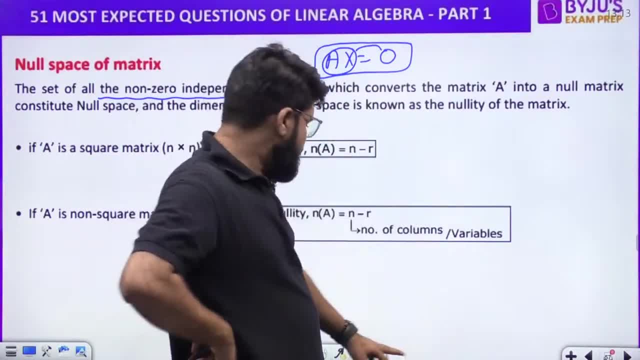 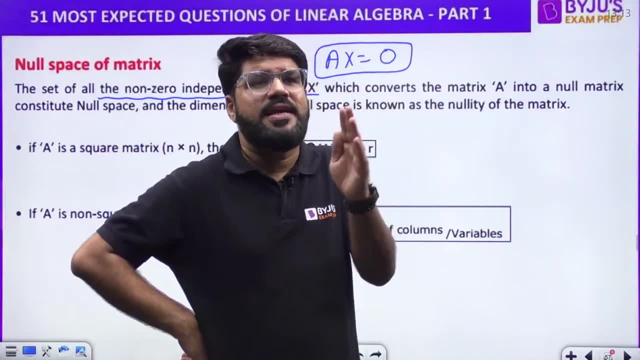 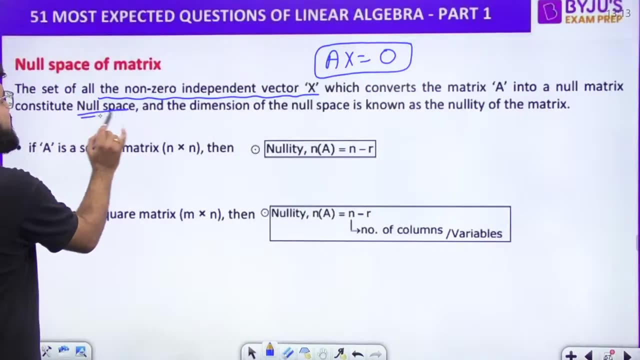 convert the matrix into null matrix. Convert the matrix into null matrix. All those vectors which will convert the matrix A into null matrix are said to form null space. The set of all those independent vectors which convert the matrix A into null matrix will form the null space of the. 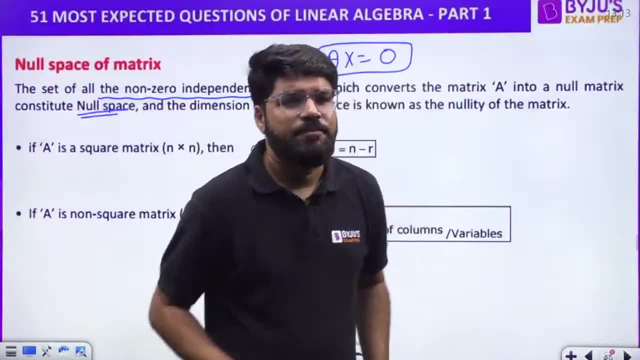 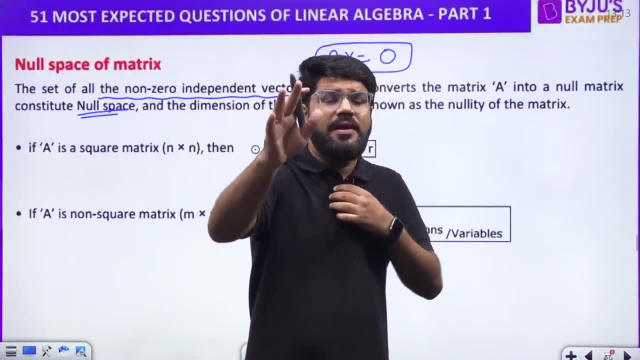 matrix And dimension. Dimension means the number of elements, Dimension means the number of elements And, in brief, I am explaining, because this is the question session Right? No, No, How many. how many independent solutions they can ask? Sivaraman? How many solutions means infinite. 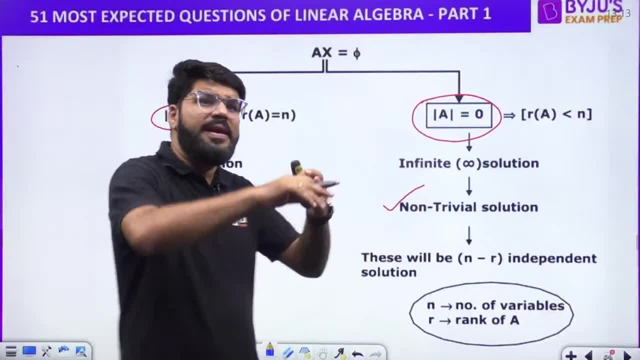 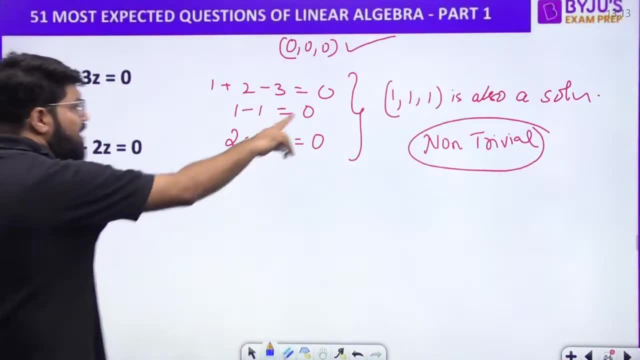 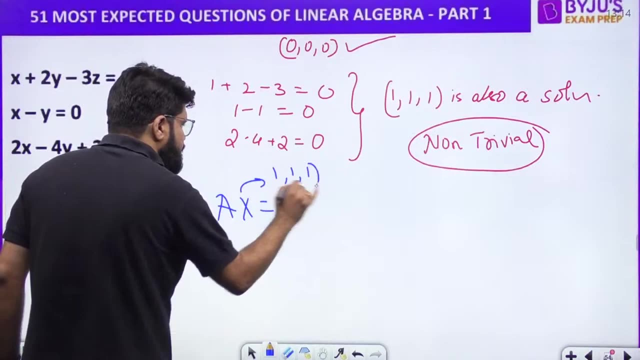 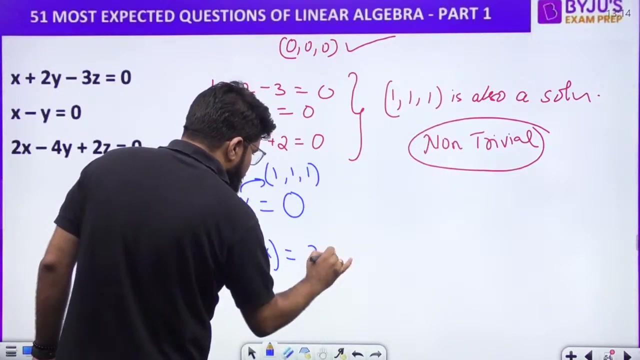 solution. See: Non-trivial means infinite. There will be infinitely many solutions, but how many of them are independent? I will explain you like this. Look, If there is any confusion: 1 1, 1 is 0. x is 1 1, 1.. But, dear, if x is equal to solution, A into 2. x is 2 into 0. But what is? 2 into 0. That is. 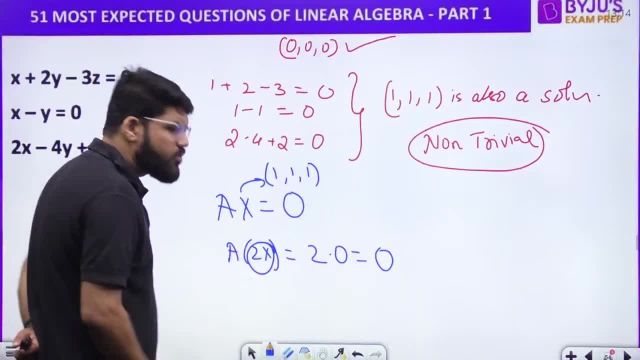 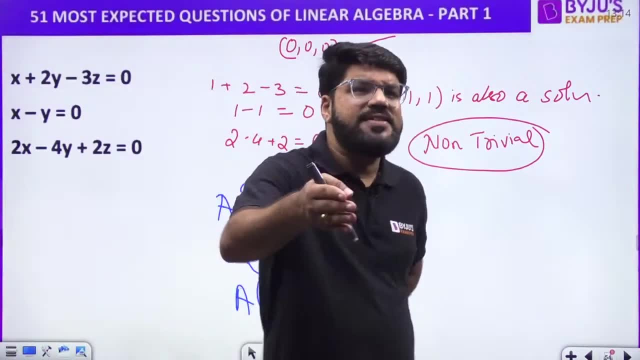 also 0.. So if x is a solution, 2 x is also a solution. If x is a solution, 5 x is also a solution. A into 5 x, This will also become 0. So if x is a solution, 2 x, 3 x, 4 x, 5 x, 100 x, 1000 x, all of them are. 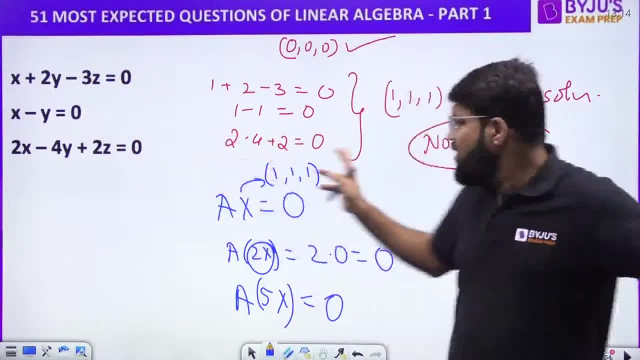 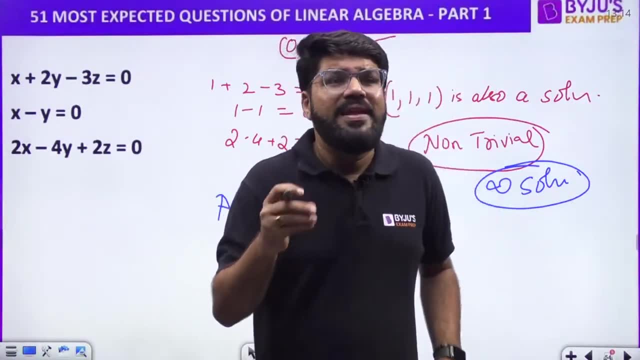 solution. Okay, So there are infinite solutions. Non-trivial means infinite solutions. So there are solutions. Non-trivial means infinite solutions, But but how many are independent solutions? They can ask that question, Sivaraman. Okay, Total solutions to infinite. So you have to be very. 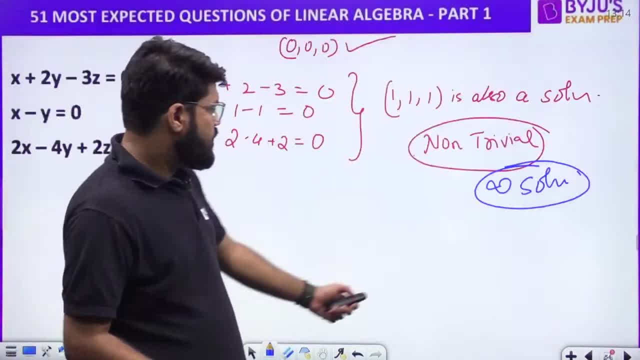 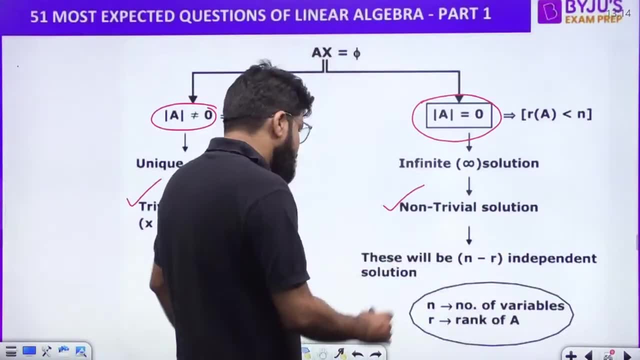 carefully reading that, And that is why I have given you this result, This one. Where is that gone? Yeah, We have. we are not deriving right now, but I am giving you this result directly. There will be n minus r Important word. There will be n minus r independent solutions, Total solutions. 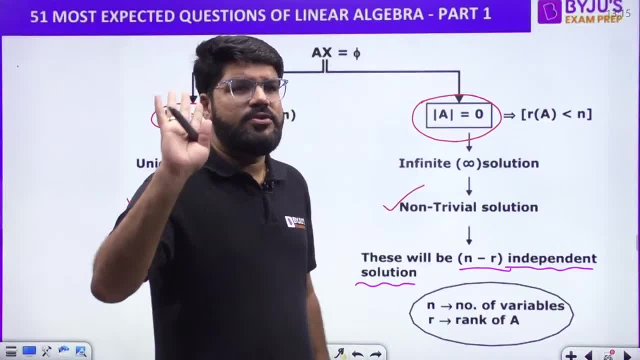 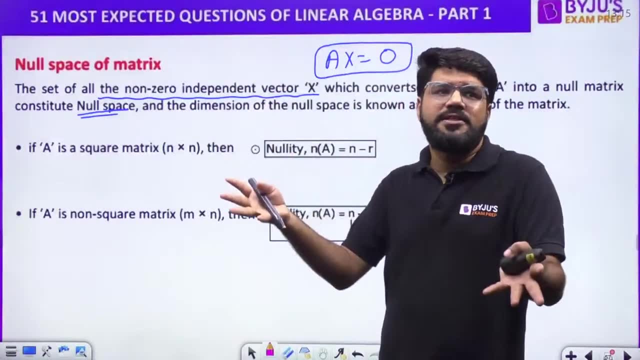 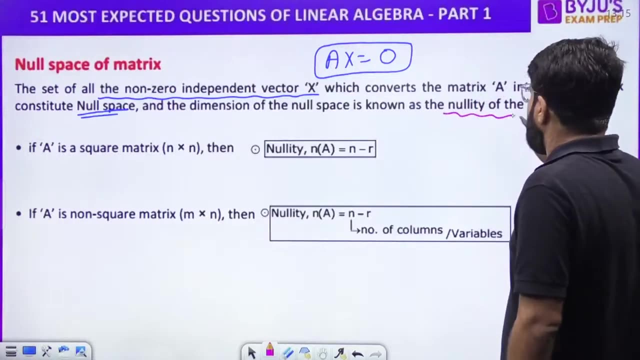 to infinite, But n minus r will be independent, And those independent solutions, when put together, they form the null space. So what is the dimension of null space? How many vectors are there in the null space? That number of vectors in the null space is known as the nullity of the matrix, So same formula will come up here, Okay, So what is? 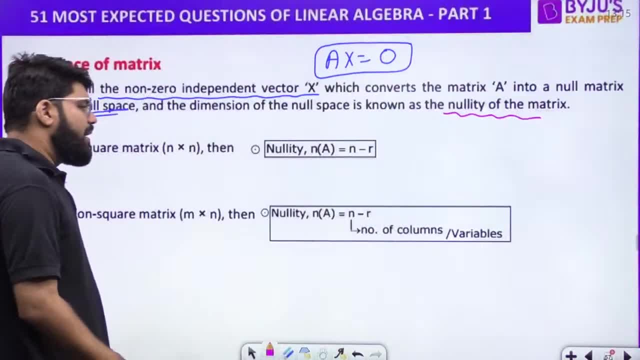 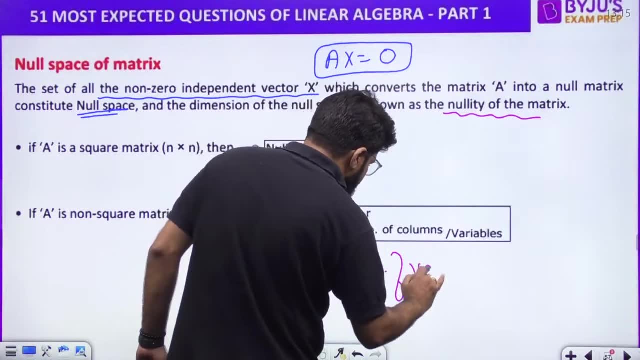 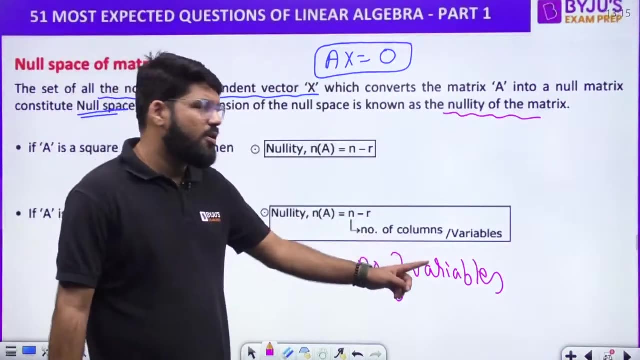 the nullity of matrix: N minus r Right, N minus r Right. So whether it is square or non-square, you just have to remember n is the number of variables. So both the formulas are okay. The nullity of the matrix is given by n minus r. N is the number of variables, R is the rank of. 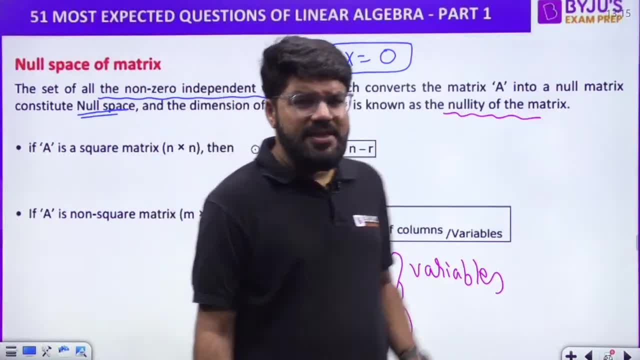 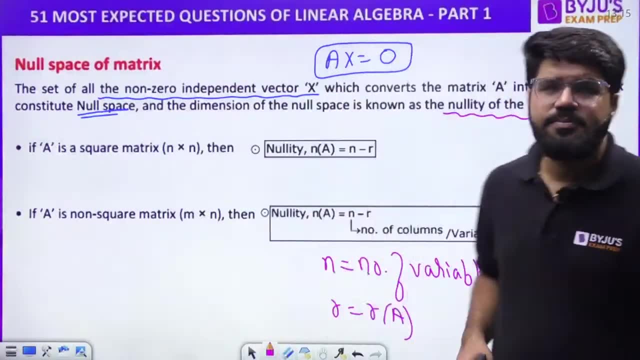 the matrix A. R is the rank of the coefficient matrix. Since this is question session, I am giving these definitions in brief, Right? If you have any more doubts, you can refer to the detailed sessions of that or you can ask. discuss me later on. Okay, Chalo, Now look into this. 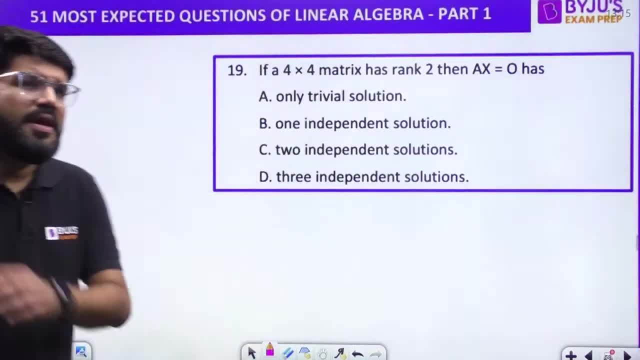 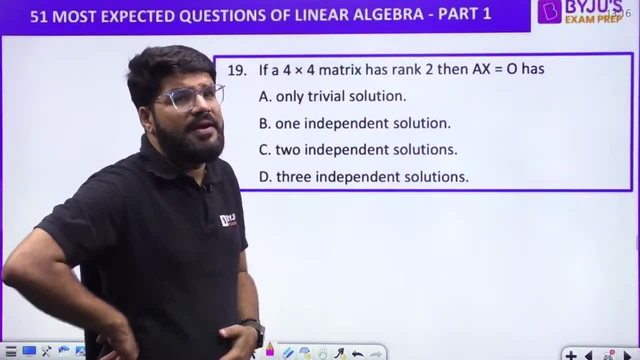 question. Look into this question. If a matrix, If a 4 cross 4 matrix, has rank 2, then A x equal to 0 has how many? See Shiva, that is what You can ask- how many independent or dependent solutions? Or does it have only trivial solution? 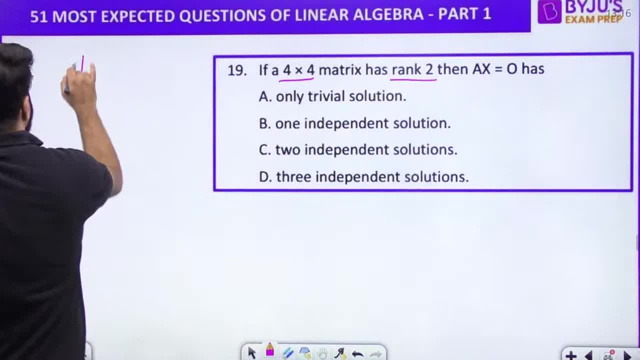 Right, 4 cross, 4 matrix rank 2.. Right Matrix is 4 cross 4.. Right Rank of the matrix is equal to 2. That is less than 4.. So determinant of A must be 0.. Okay, Determinant of A must be 0.. 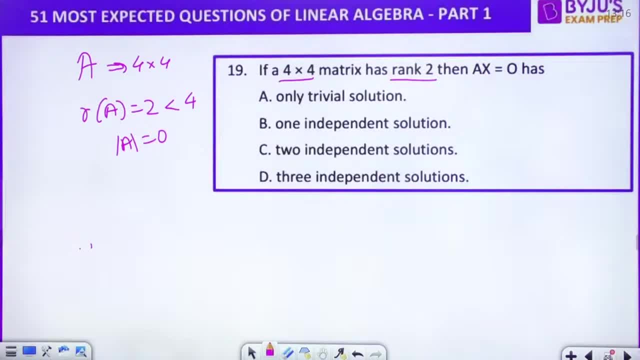 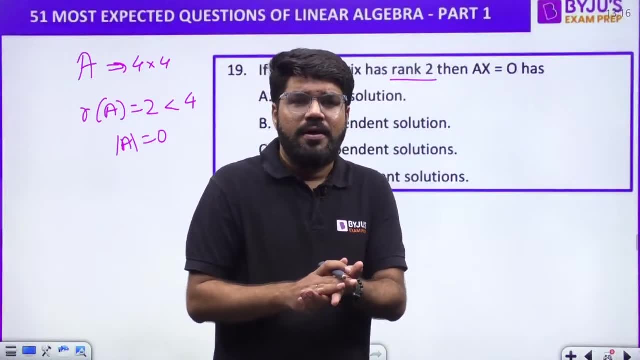 Determinant of- Oh, I am sorry, Determinant of A must be 0. Because if determinant is non-zero, No, No, No, Setupati. If determinant is 0. Then the system will have non-trivial solution. How will it be trivial, Right, So determinant? 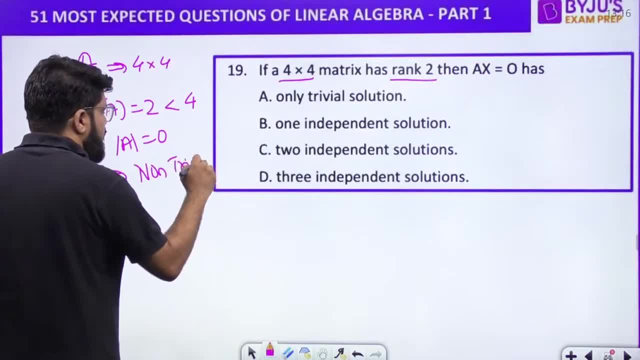 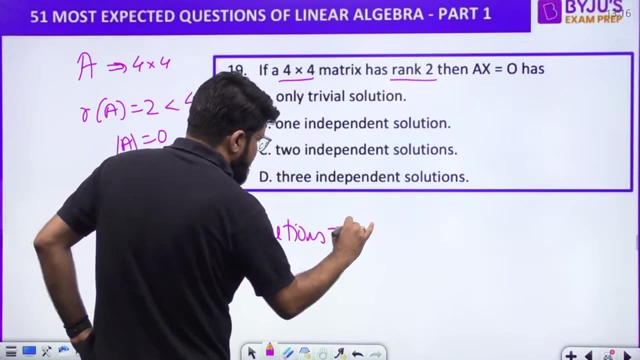 not equal to 0.. So non-trivial solution: Okay, So A is wrong. But in the non-trivial, how many independent solutions? How many independent solutions? Number of independent solutions is given by N minus R. N is the number of variables. So what is the number of variables? 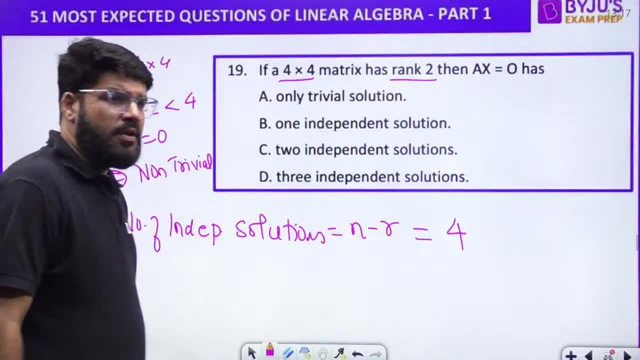 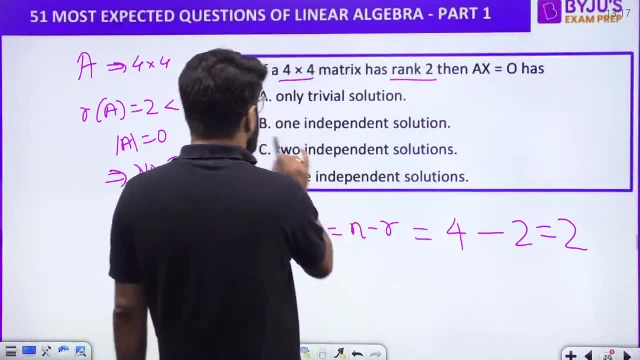 4 cross 4 matrix. So number of variables will be 4. Right Minus rank of the matrix they have given directly. So this is a direct, actually formula based question. So answer will be 2. 2 independent solutions. Option number. 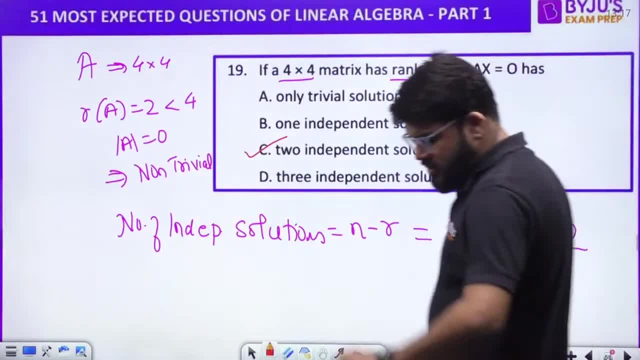 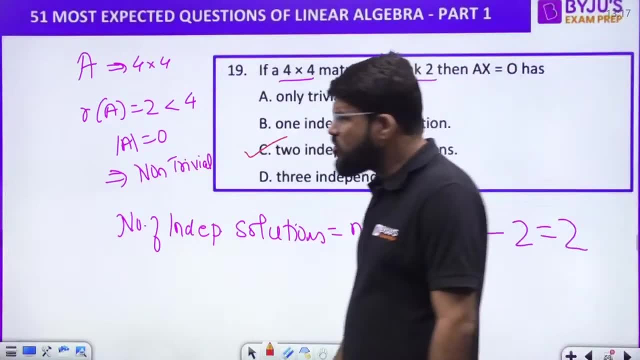 C 2 independent solutions. Right, I think around almost 2 hours of session is about to be done. Many people are tired Now the attendance has got dibbed. Should we stop? If you are tired, How can I gain that energy? always Students are tired so early I am. 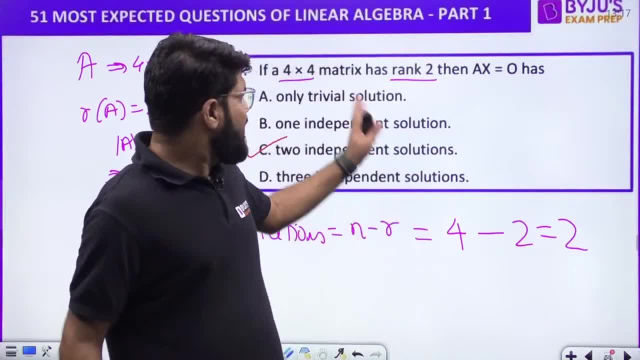 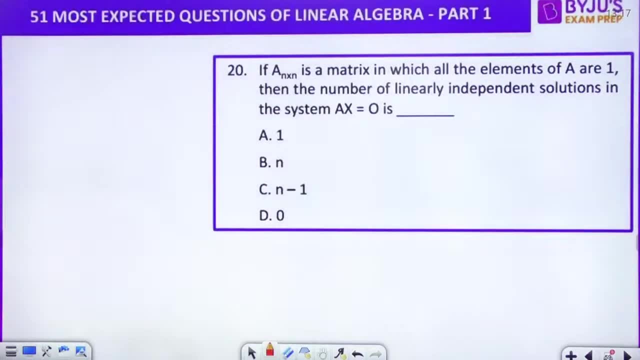 there with full energy. Right, I think we have around 25 questions For today. exact number I do not remember, But should we stop at 1920.. If A is a matrix in which all elements of A are 1., Then the number of linearly independent solutions of 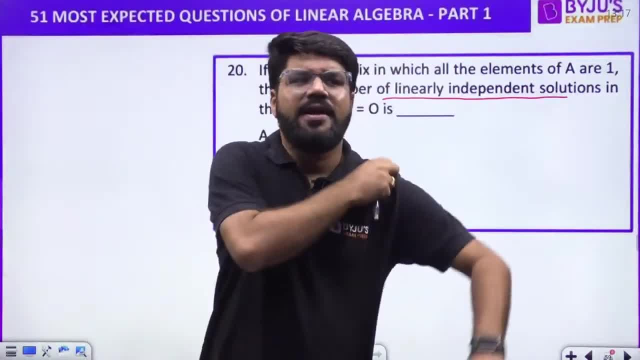 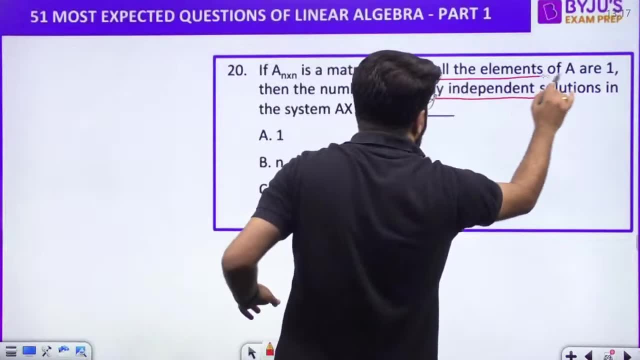 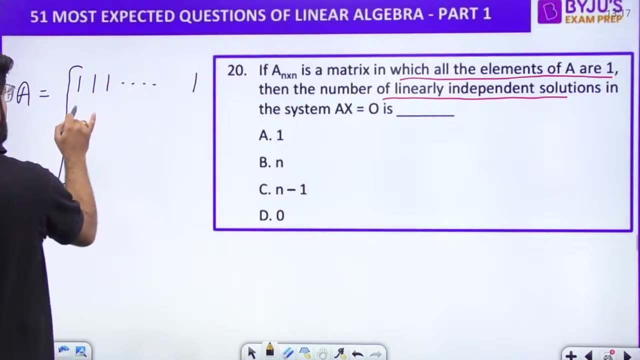 the system. Little indirect question, but very simple. Little indirect, but very simple Right, In which all elements of A are 1.. A is a matrix in which all elements of A are 1.. Very simple na. A is a matrix in which all elements of A are 1.. 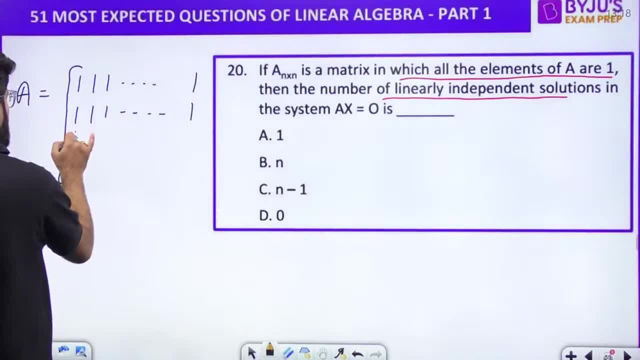 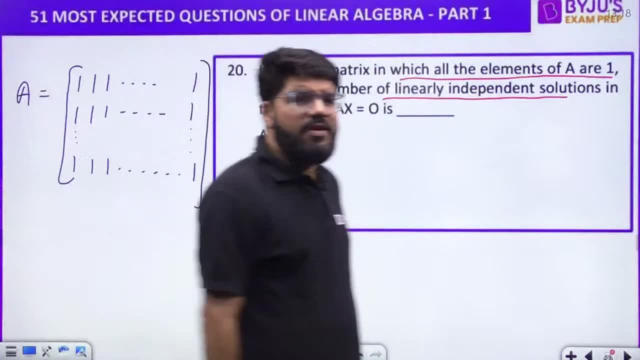 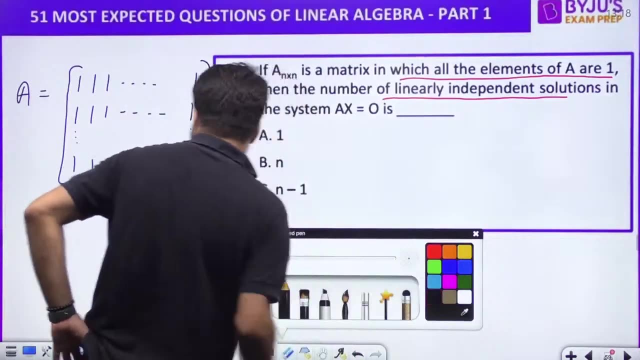 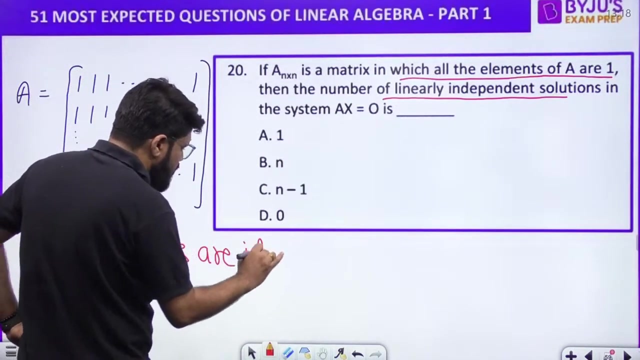 So what is the rank of the matrix? What is the rank of the matrix? All elements of A are 1.. What should be the rank of the matrix? Tell me Right. This simply: all elements are 1.. That means all rows are same. All rows are identical to each other, And if a matrix 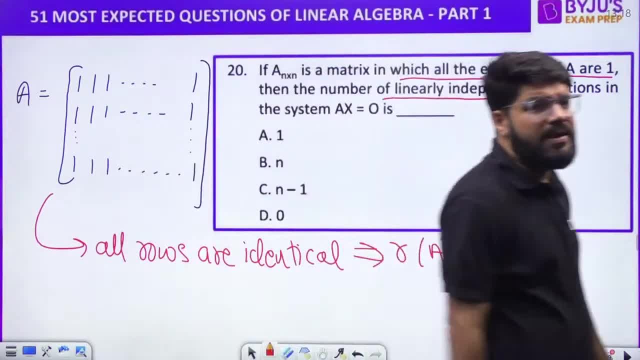 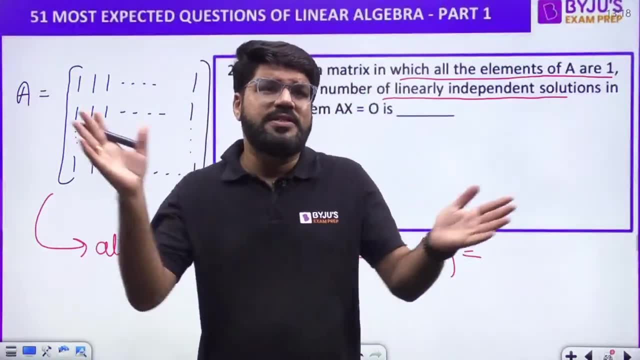 has all the rows identical to each other, Then it is a matrix in which all elements are equal to each other. What is the rank of such matrix, Everybody dear, What is the rank? That is why see all these topics rank, homogeneous, non homogeneous, system are totally. 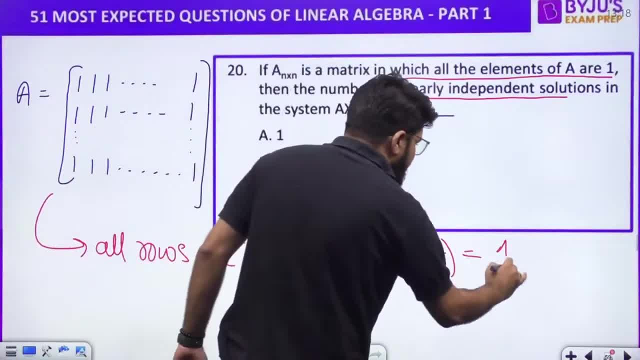 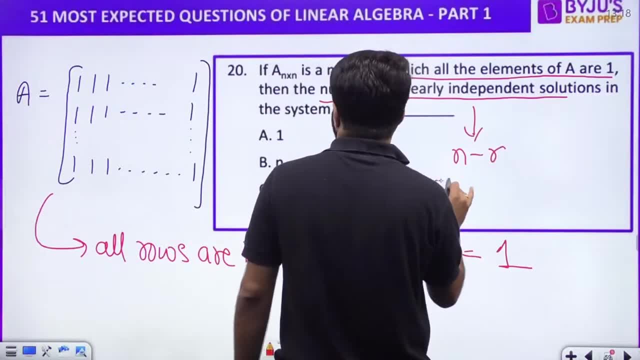 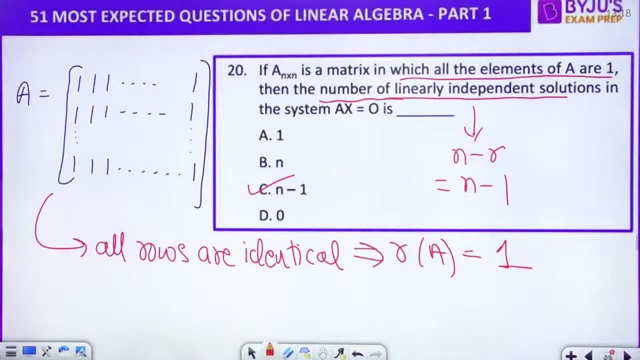 connected Right. We have studied this point today only in the rank. Rank of A is equal to 1. Right. So what is the number of? what is the number of linearly independent solution? It is given by the formula n minus r, n minus 1. r, ka, value 1.. Answer: number C Or they. 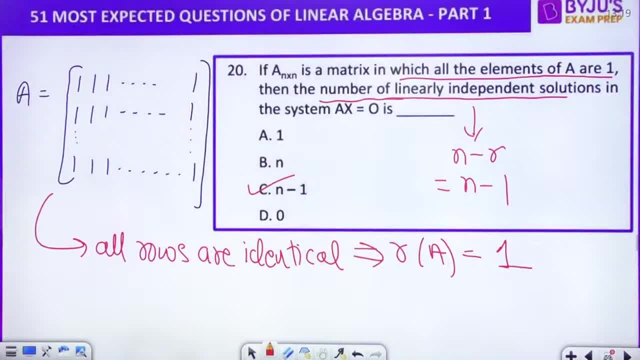 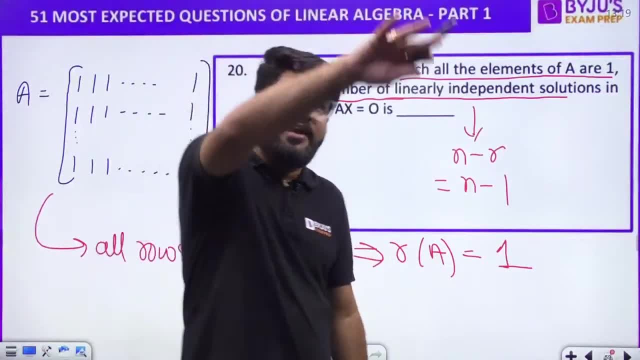 can give the value of n as well. They can specify the value of n. So the answer is n minus 1.. See, a good question. It is very simple, but I will call it as good question. It is using some concepts related with the. 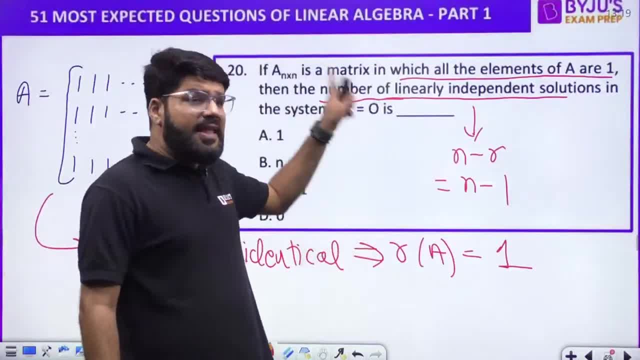 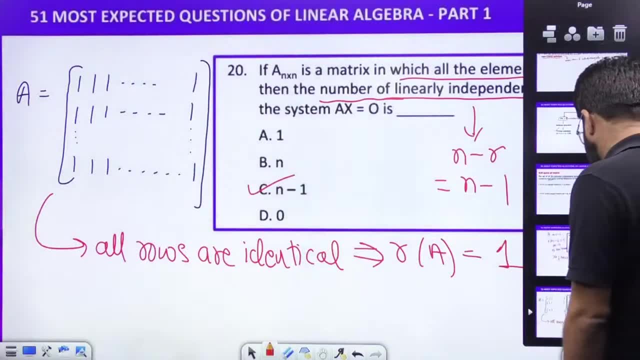 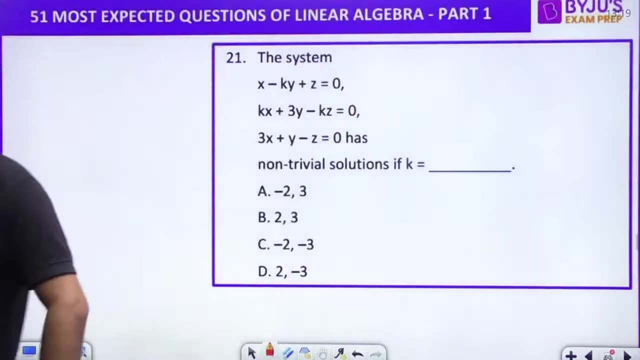 rank. also, All elements are 1.. So you should be able to relate rank as 1.. Then you should be able to apply the formula number of linearly independent solutions Correct. That is why I call this as a better question. Chalo, next, number 21.. This system has non trivial solution. if This system has non trivial 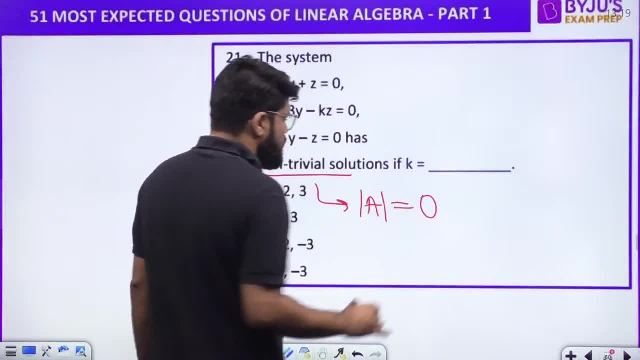 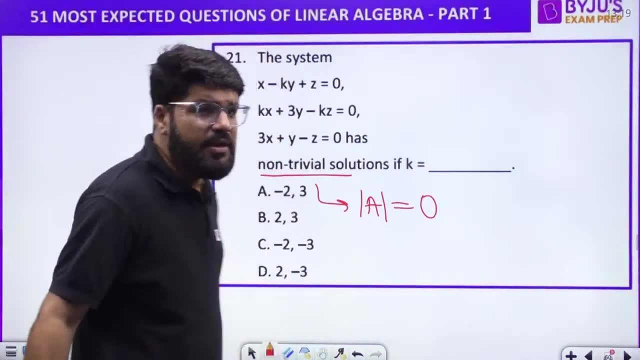 solution. what is the condition for non trivial solution? Modulus of a equal to 0.. Trivial means unique. unique means non zero, determinant. Non-trivial means infinite. infinite means zero. determinant. simple and sweet memories. OK, So determinant equal to zero, How simple. 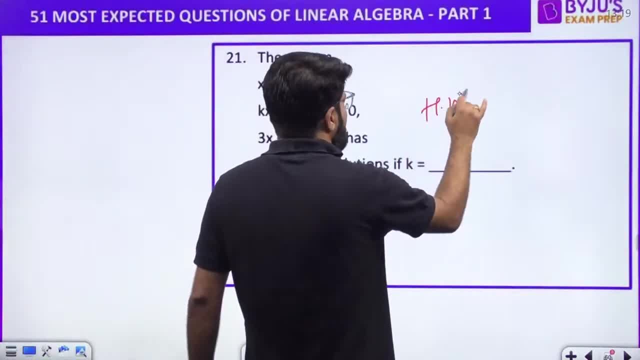 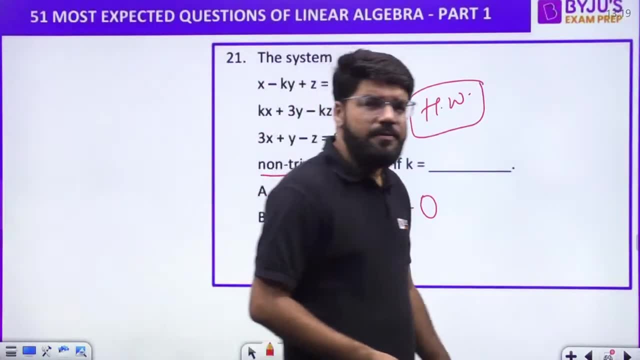 is that going to be? Kindly complete this as homework? na yaar, It is a repetitive calculation, So better. determinant equal to zero: everybody can do it. Everybody can do it, Please do it. Determinant equal to zero: everybody can do it, So please. do it and calculate it Correct, amazing guy. So now the teorization time for the limitations of non trivial solution is time: 1.1.1 is 5.25 and third: 1.5 is also 0 minute and 5 minute It is 3. another hurt pepper 화. 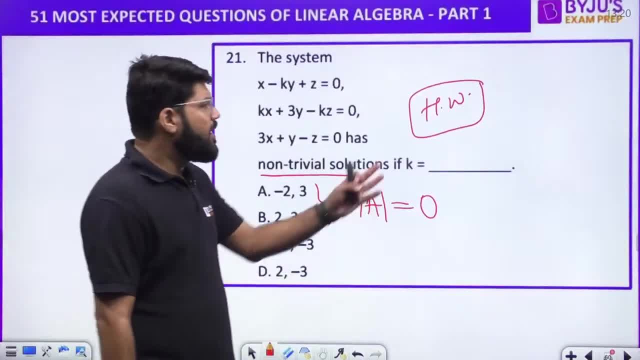 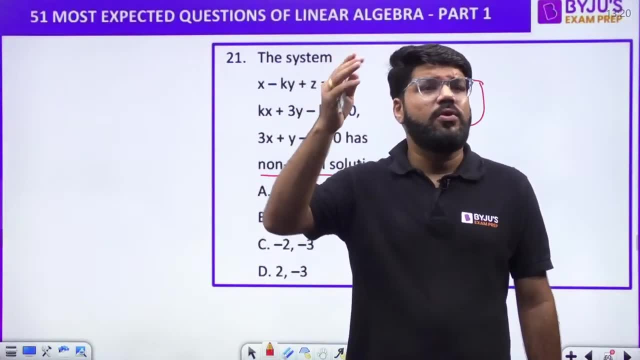 complete it, okay, i hope you will be able to do it. i'll put it as homework. everybody will be able to do it. please complete this, okay, and whatever three, four homeworks i have given, do not forget to comment your answers in the comment box after the video gets over. please do comment, please do. 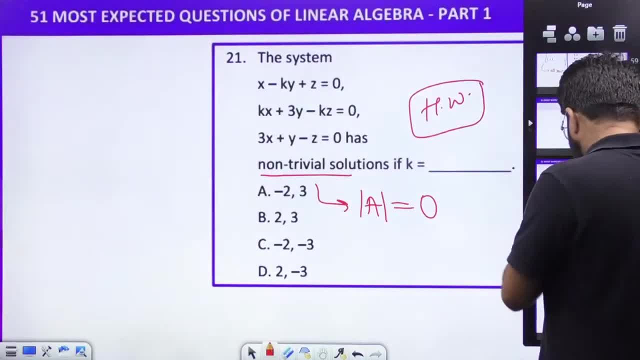 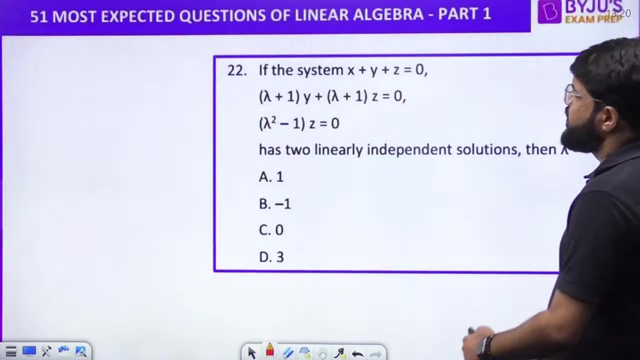 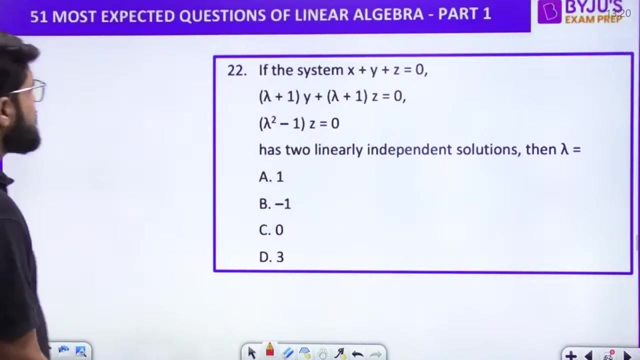 comment. okay, next question, let us first, let us first jump to, let us go in sequence. only, no issue, this one is homework number 22, number 22: here: if the system x plus y plus z equal to zero lambda plus one y lambda plus one z, equal to zero lambda square. 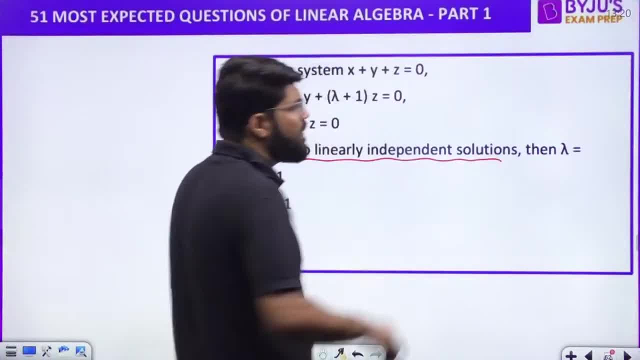 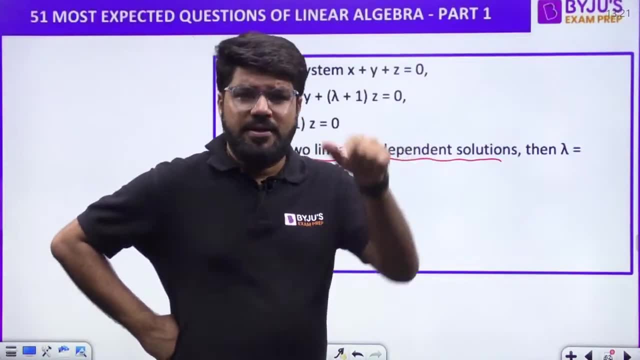 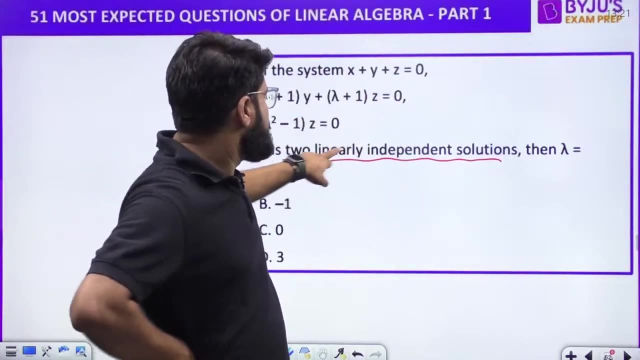 minus one z equal to zero. has two linearly independent solutions. some indirect question: yeah, i'll share sanjeeva, i'll share. okay, don't worry, has two linearly independent solutions. today i'll share up. today i'll share both this video and the digital one. okay, has two linearly. 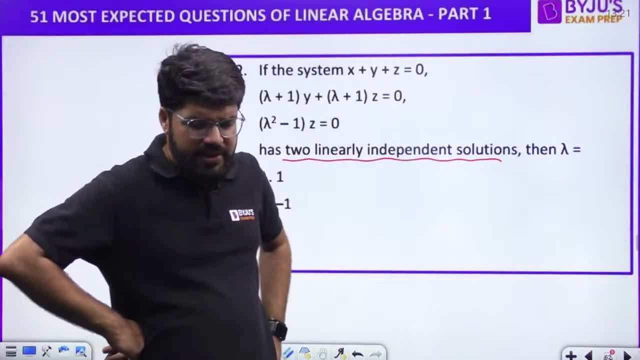 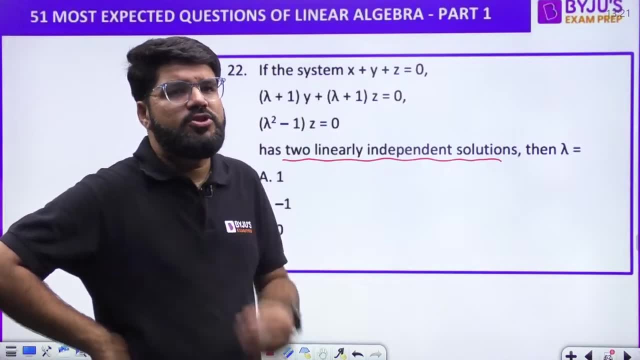 independent solutions. what is the value of lambda? this has two linearly independent solutions. what should be the value of lambda? two linearly independent solutions. what should be the value of lambda? now? number of linearly independent solutions? n minus r is given to be 2, where n is equal to number of. 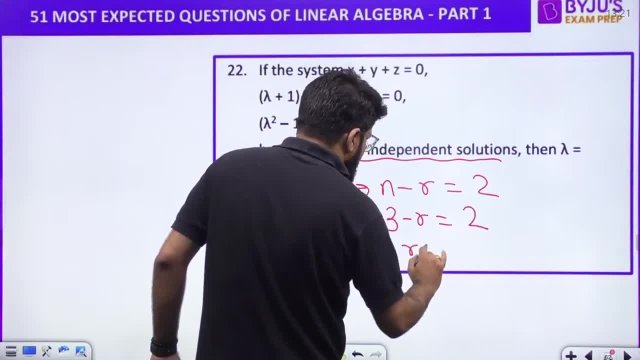 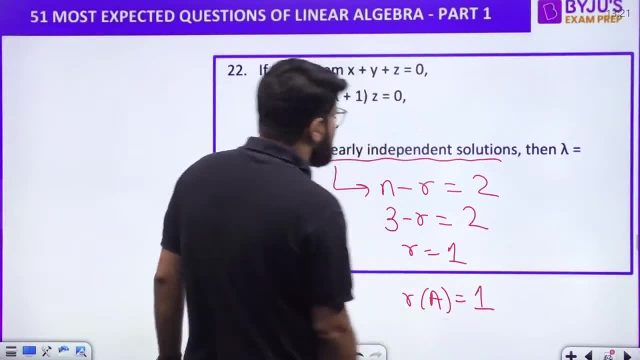 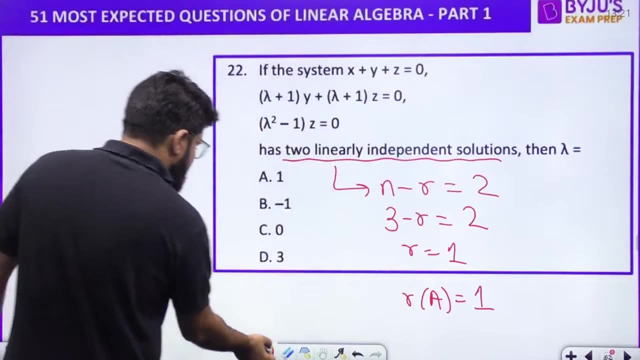 variables. so n is 3, so 3 minus r is equal to 2. r should be 1, r matlab r, matlab rank of a should be 1. then what is the value of lambda? the question is indirectly related to rank. again, the question is indirectly related to rank. rank of a equal to 1. what is the a matrix? what is the a matrix? 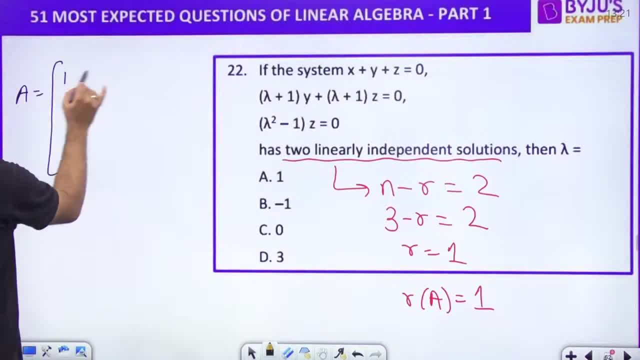 What is the A matrix here? 1, 1, 1.. Then you have 0, lambda plus 1, lambda plus 1.. Then you have 0, 0, lambda square minus 1.. What should be the value of lambda? Here? identical rows cannot be applied. 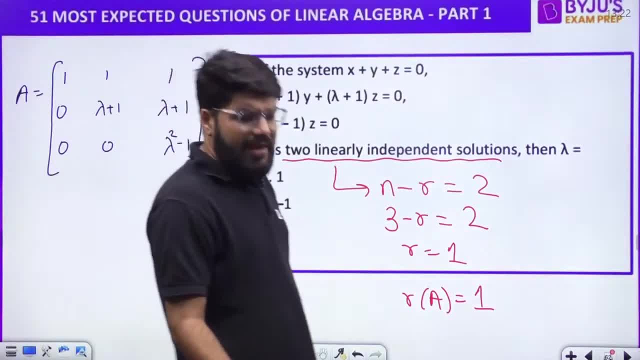 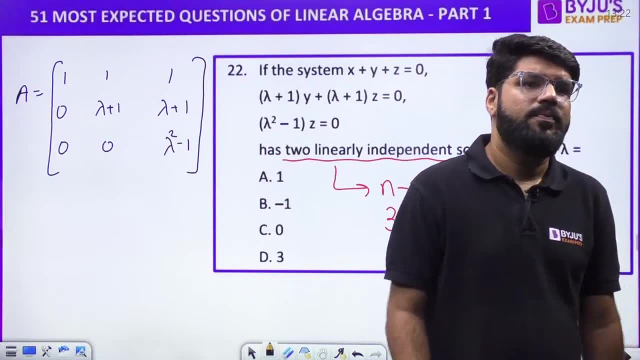 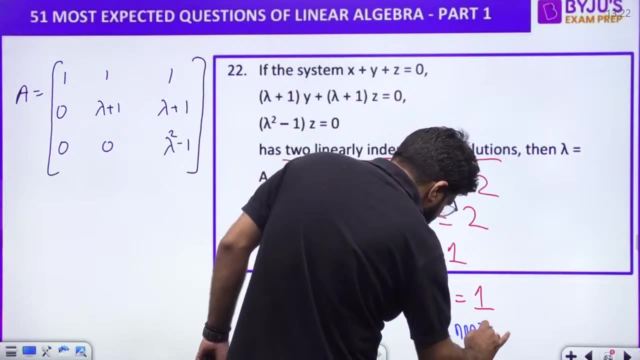 because anyways, this is 0.. 0 cannot be identical to 1.. So rank is equal to 1.. You can say: only one non-zero row in the equivalent form. The matrix should have only one non-zero row in the equivalent form, Rank equal to 1.. So I can say: the matrix should have one non-zero row in the equivalent. 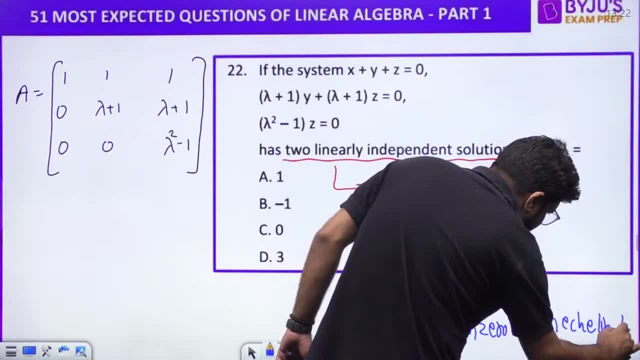 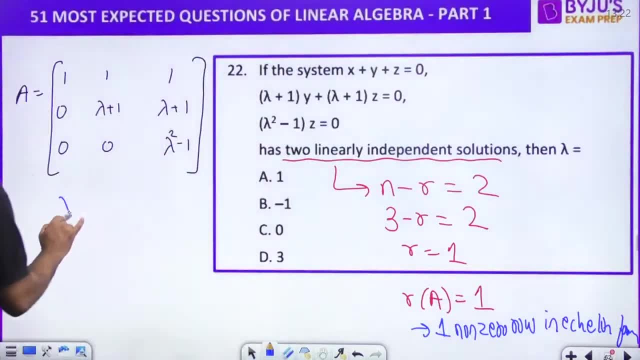 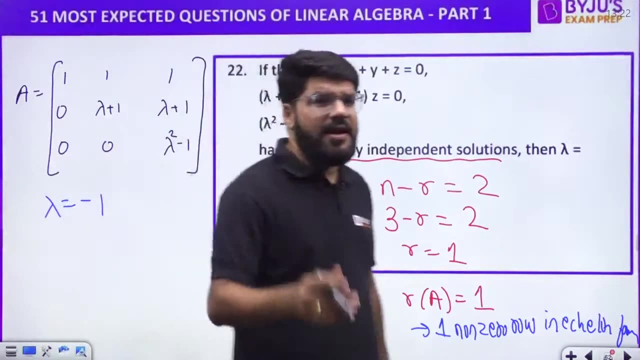 form. Non-zero row method. only for equivalent form. Only for equivalent form. So it should have only one non-zero row for the equivalent form. Simple logic, Simple logic: Lambda plus 1 ko 0, kar do, So lambda is equal to minus 1.. It's a crystal clear answer in the mind. 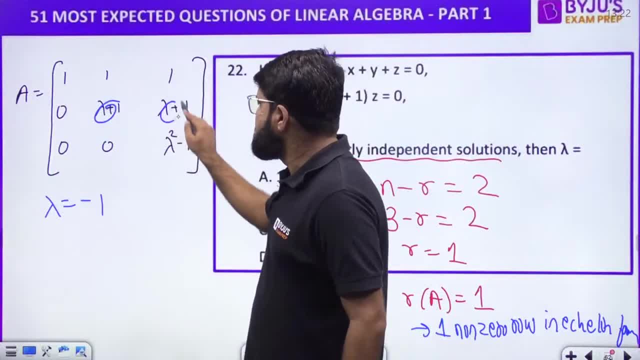 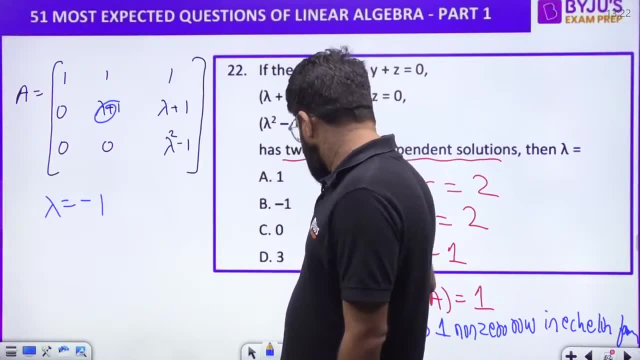 because it's a simple logic. If I take lambda equal to minus 1, this is 0, this is 0. and lambda square minus 1, this will also become 0. Both these rows will become 0. Both these rows will become 0.. So if lambda is equal, 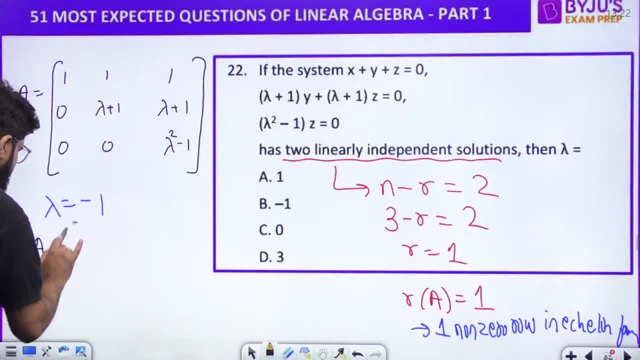 to minus 1,. what does the matrix A looks like? Matrix looks like: 1, 1, 1, 0, 0, 0, 0, 0, 0.. Both the row of 0 is at the last, So it is the equivalent form. Number of starting zeros. 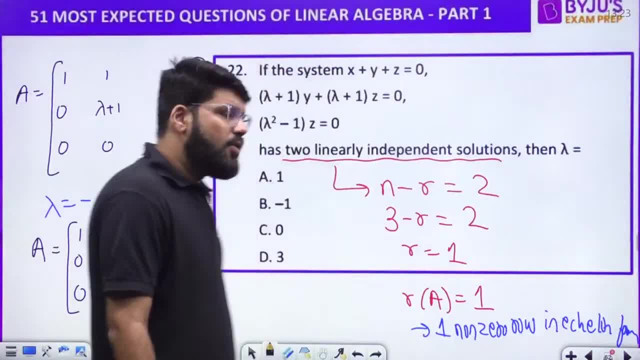 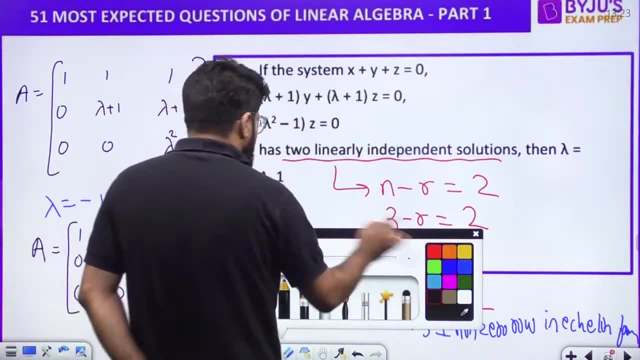 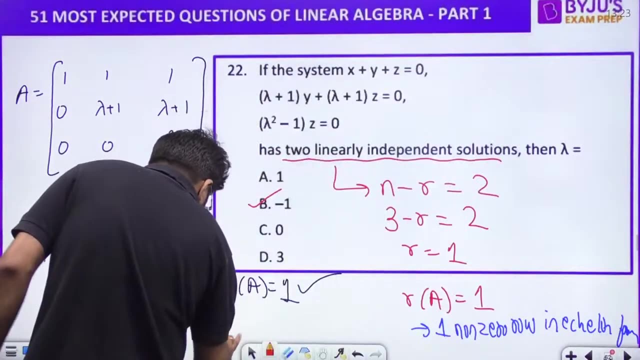 ek hi row ka dekhenge. Don't count the number of R0s. Okay, So this has the rank equal to 1.. And that is what I want. So for what value of lambda Minus 1.. For what value of 0? Minus 1.. Okay, This is equivalent form. This is: 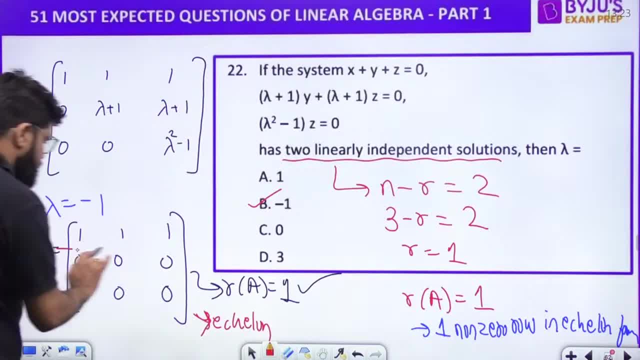 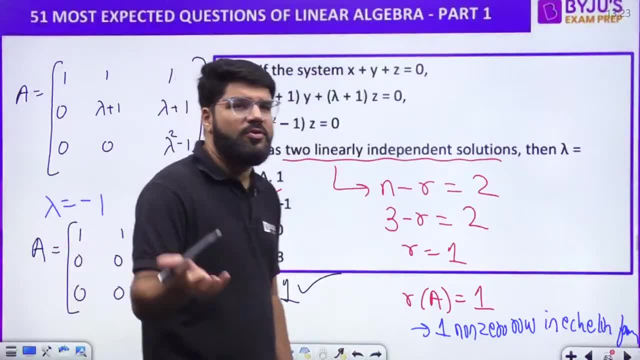 the equivalent form Row of 0s should be at the last. Now, other than the row of 0s starting 0,, only one row is there, So we can say it is increasing order. There is only one number. There is no sense of comparing increasing, decreasing. The question is solved here itself. 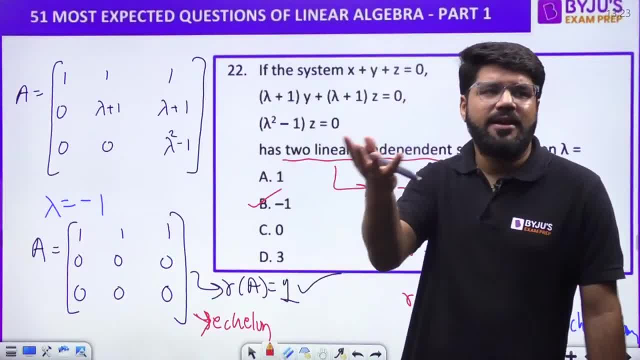 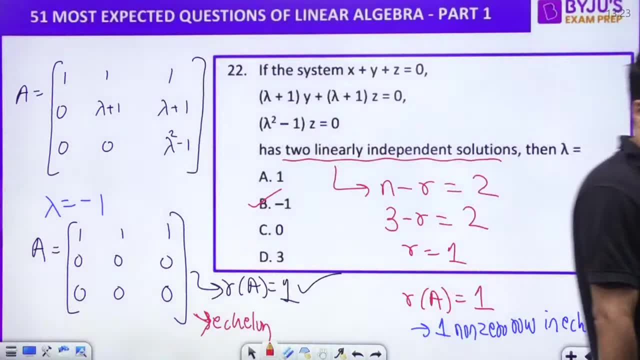 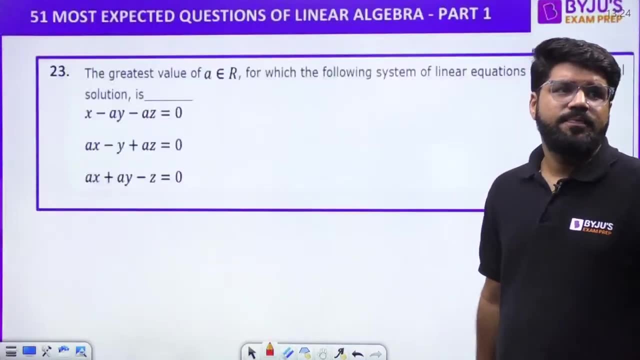 only Rank is equal to 1.. Or you can even solve by the determinant and minor method: rank 1 aega, Simple one, Rank will be 1.. Simple one, All great. Next question: So this is again a good question. Indirect connections, Number 23. The greatest. 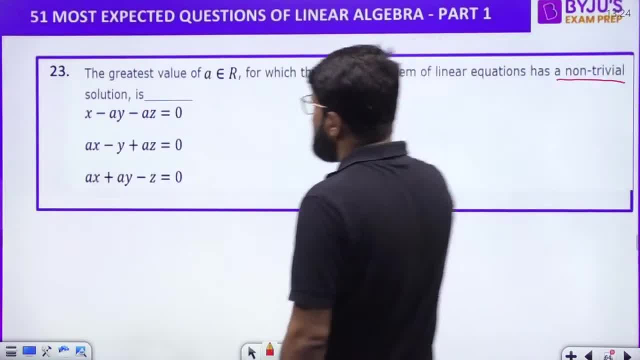 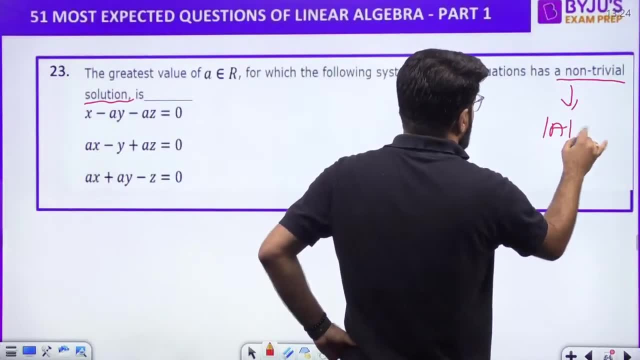 value of alpha, for which the following system of equations will have: non-trivial solution, Non-trivial solution. Once again, non-trivial, Non-trivial solution. Let's do this: If non-trivial is said, mod a equal to 0.. Determinant equal. 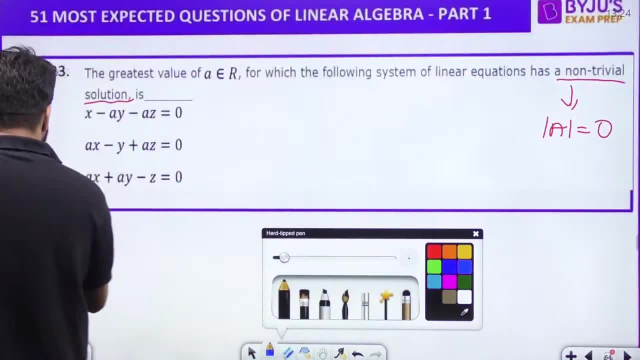 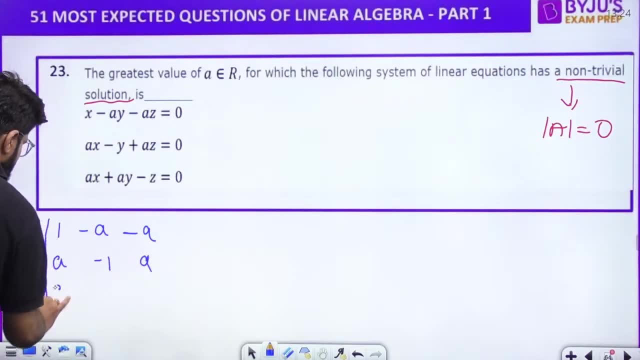 to 0.. Okay, So determinant equal to 0 means you have 1 minus a minus a a minus 1 a a a minus 1.. Let us see what is this. Is there any significance? of the greatest value here? 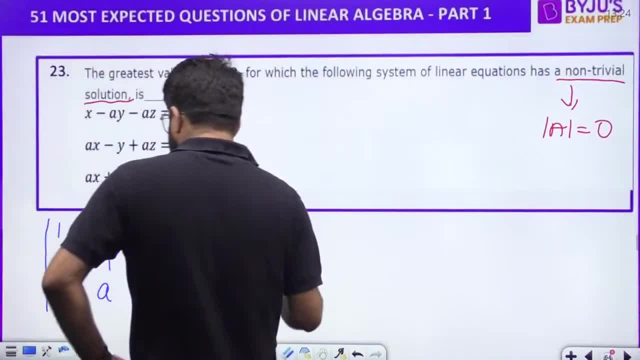 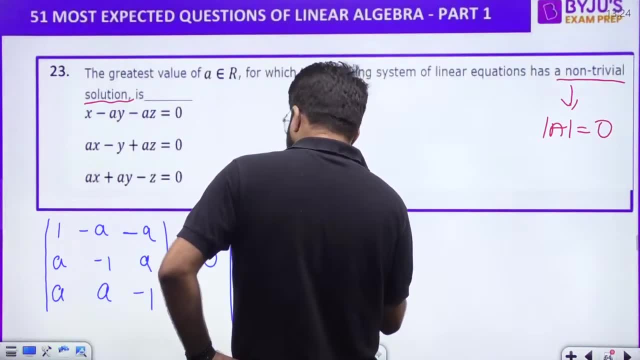 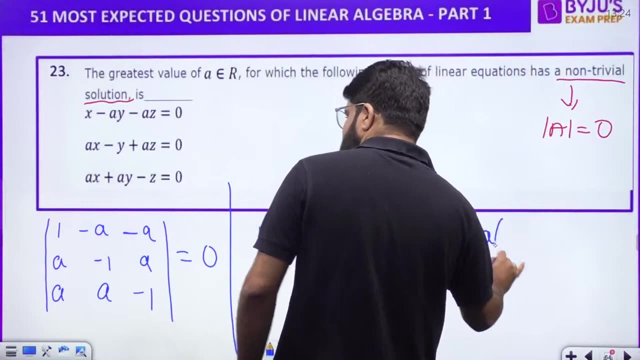 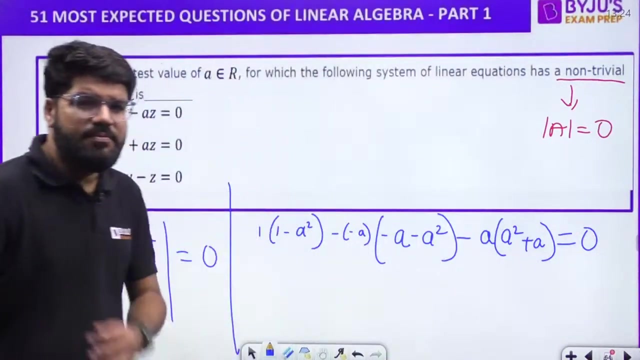 Let's check Right. So this determinant equal to 0.. So 1 into 1, minus a square, minus minus, It will become plus a Plus a of minus a minus a square, Then eventually minus a. Then you have a square minus minus plus a. This should be equal to 0.. Let us just scroll and simplify. 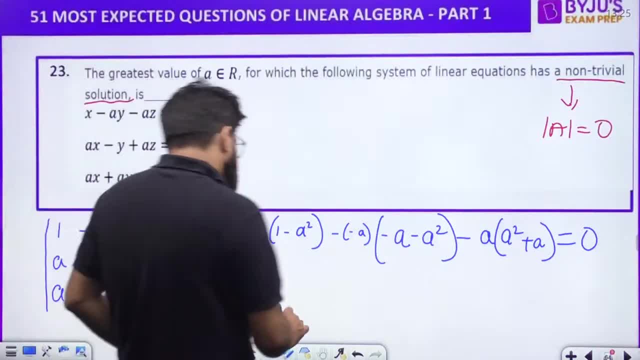 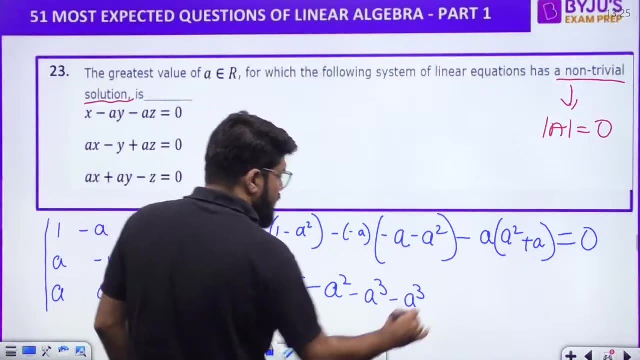 this Right. Yes, Yes, Yes. So this is 1 minus a square. Right Minus, minus plus a And eventually minus. So minus a will remain Minus a square Minus of a cube, Minus of one more a cube Minus of a square equal to 0.. Right Minus. 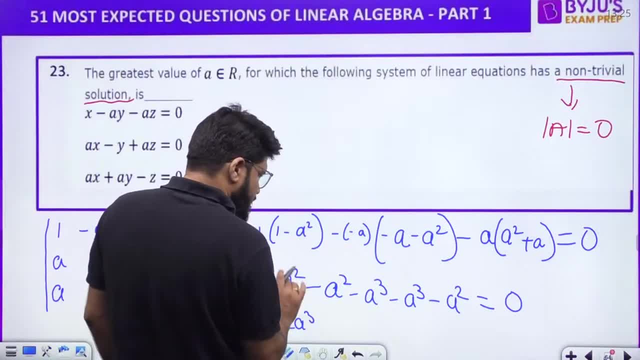 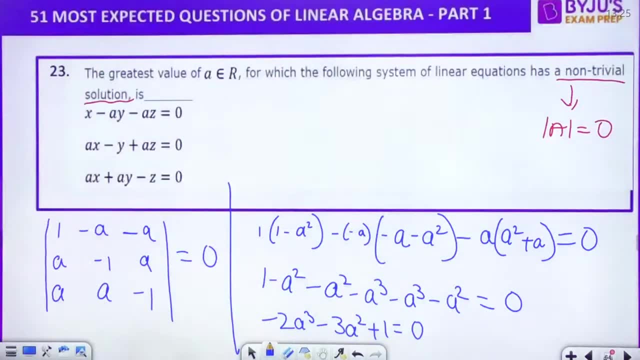 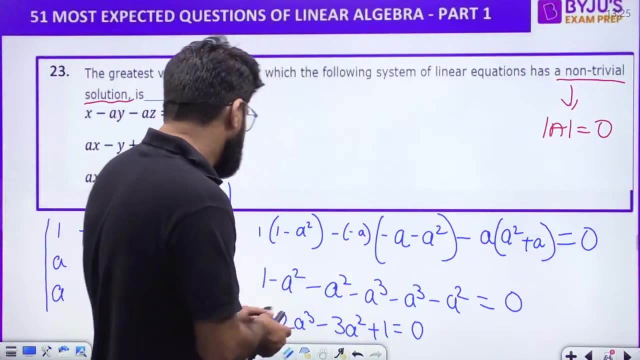 a cube minus a cube minus 2 a cube, who are total: a square. a square a square 3 times minus 3, a square plus 1 equal to 0.. What should be the greatest value of a? now, to satisfy this Right, Minus 2 a cube, Correct 1, 2, 3 minus 3 a square. Let us write this here: 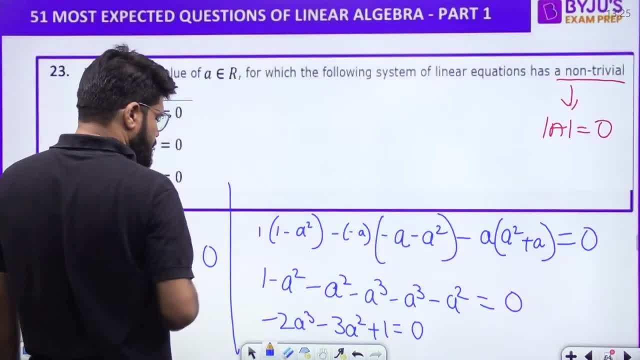 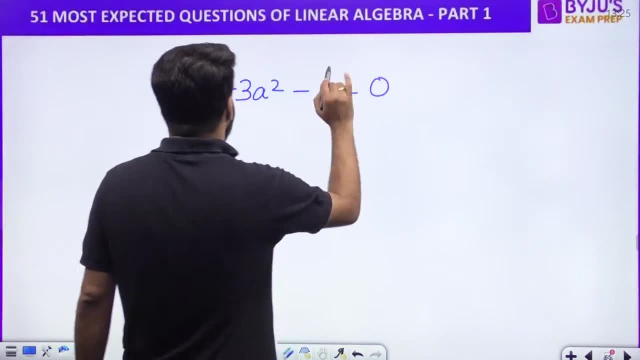 Minus. if I separate 2 a cube Right Minus 2 a cube Correct, 1, 2, 3 minus 3 a square Minus, sorry, plus 3 a square minus 1 is equal to 0.. Is equal to 0.. Right: 2 a cube plus. 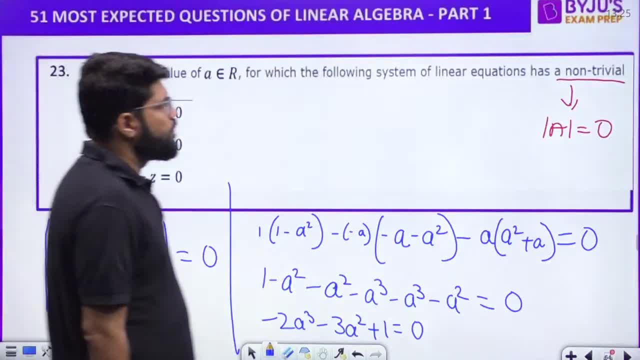 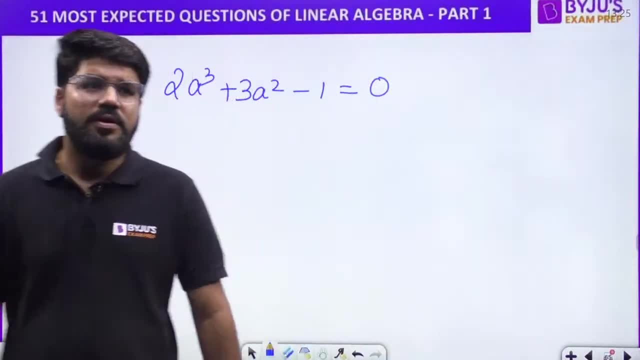 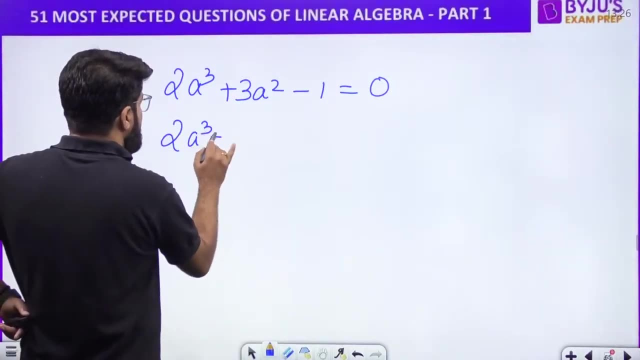 3 a square minus 1, equal to the 0.. Okay, so can we factorize this? Can we try and factorize this So I have 2 a cube Plus 2 a square Plus a square minus 1.. this is going into minus. 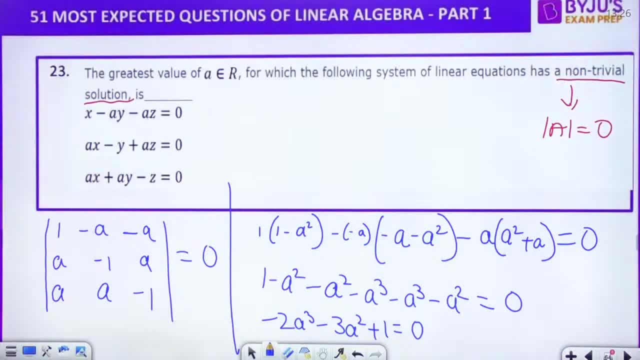 Tucme 11. Why? Because 0, because no 1.. Singapore just went in to minus Right, So I am writing. that is, I think, the problem. now, 1 into 1 minus a square minus of minus 1, then you have minus. 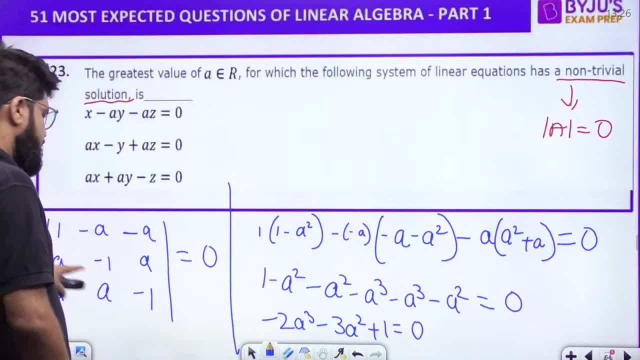 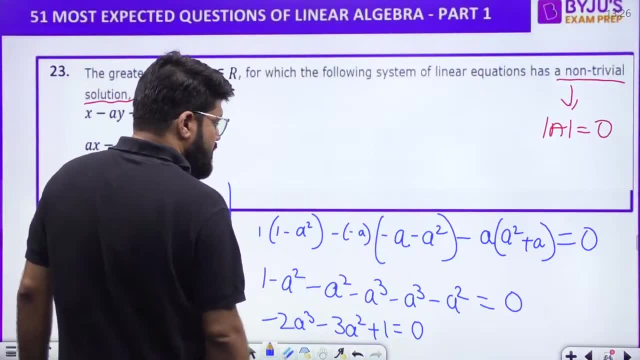 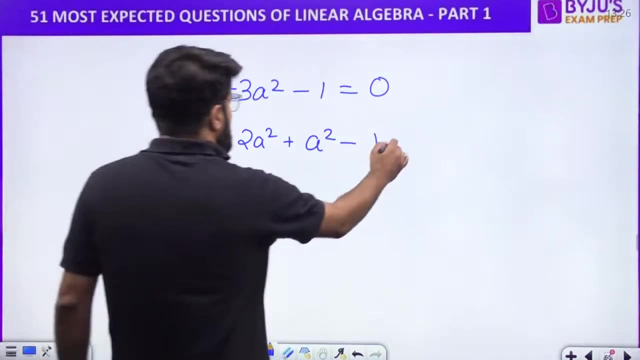 a minus a square. perfect minus of a a square minus minus plus a, so 1 minus a square. 1 minus a square minus a cube. minus a cube minus a square equal to 0. so minus 2 a cube. minus 3 a square plus 1 equal to 0. perfect up to this point. and this is equal to 0. this is: 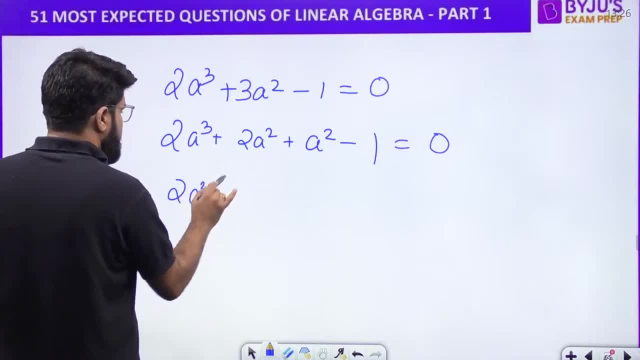 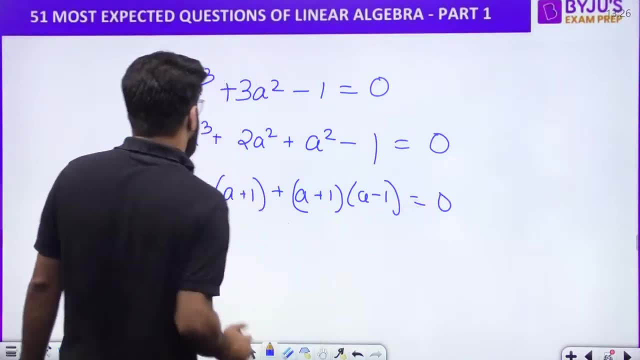 equal to 0, right? so if I take 2 a square outside, I have a plus 1 plus. this is factorized as a plus 1, a minus 1 equal to 0, right? in dono ko club, kya club? these two right, then I have. 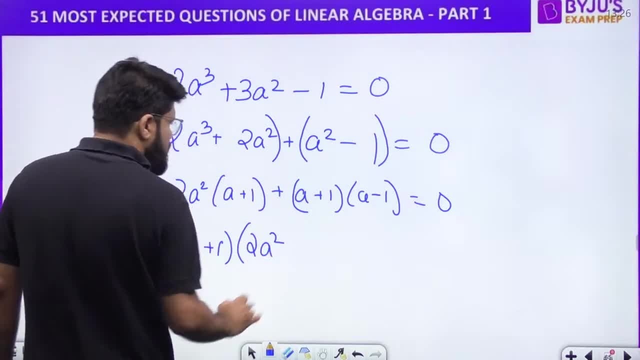 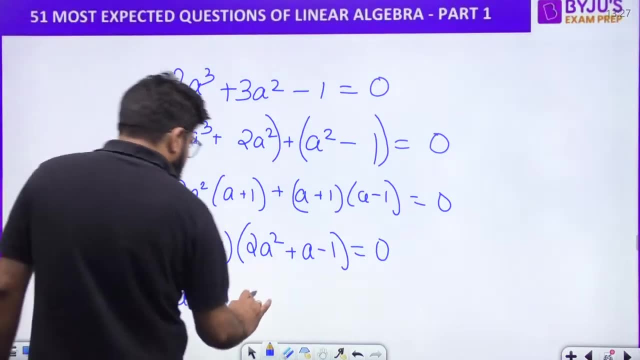 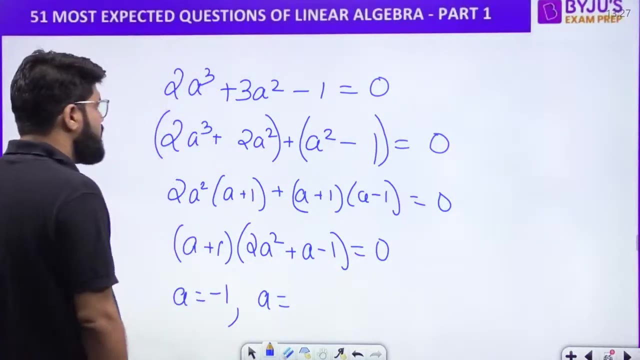 a plus 1 common, then I have 2, a square, plus a minus 1, equal to 0. so a is minus 1. that is one of the solution from here you will get. it is a quadratic roots. right, it is a quadratic root, It is a quadratic root and for quadratic root you have minus 1 plus minus root over. 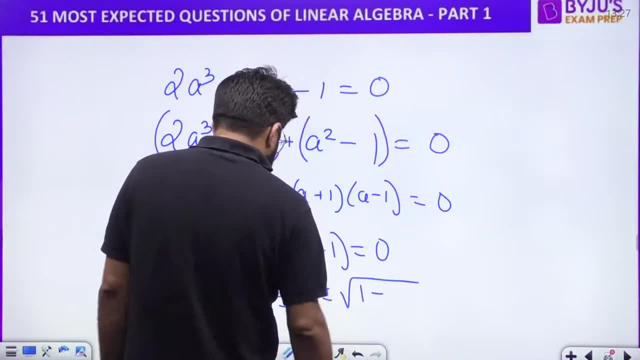 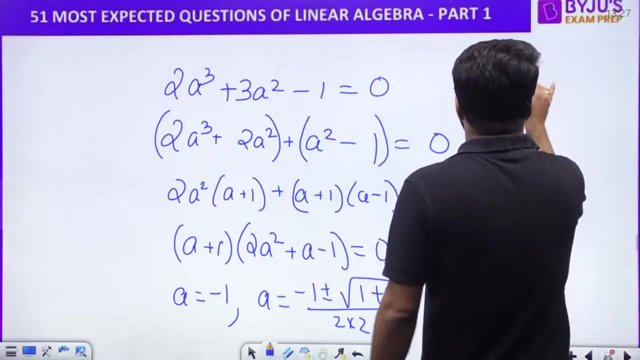 b square. that is 1 minus 4 ac, so that will become plus 8 is divided by 2 into 2. so what are the values of a coming up? a is minus 1, then minus 1, plus minus under root of 9, that. 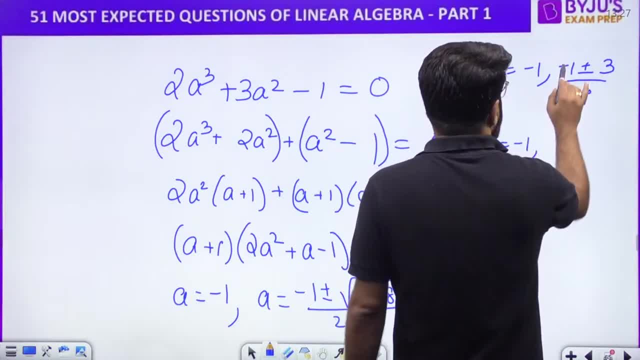 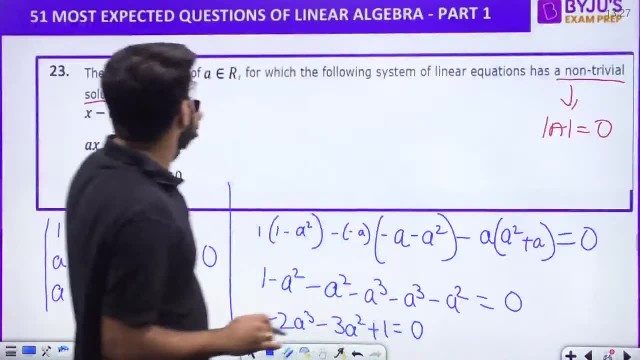 is 3 and then divided by 4, so a is eventually minus 1 minus 4 by 4 is again minus 1, and then you have 3 minus 4.. 3 minus 1, 2 by 4, that is 1 by 2. what is the greatest value of a? what is the greatest value? 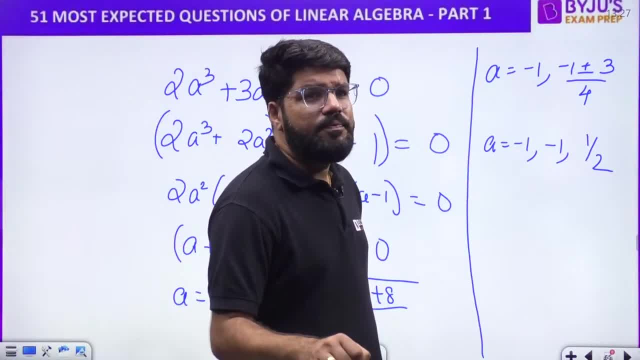 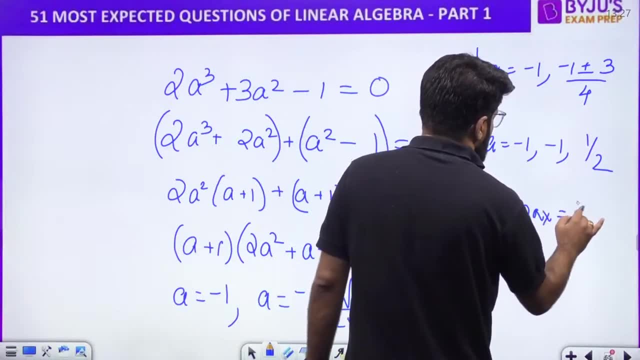 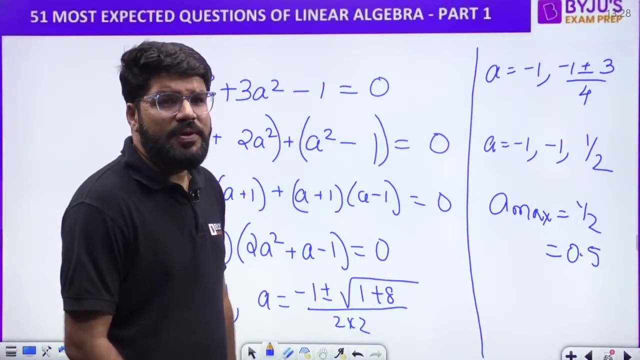 of a modulus of a, b. nahi pooch hai. what is the greatest value of a, 1 by 2? what is the greatest value of a? guys, check out the calculation: 0.5. it should be 0.5. yes, sethupati akji correct. 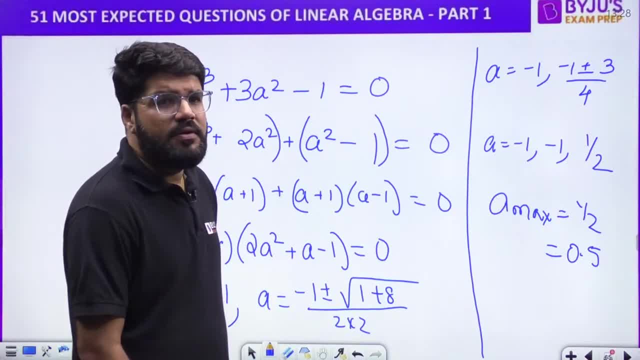 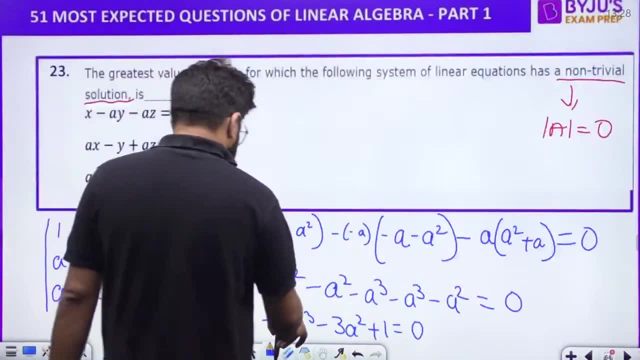 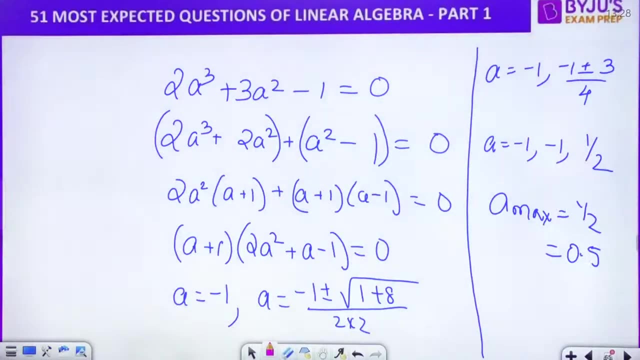 answer right: 1 by 2, all ok, I think so. Some of you are commenting minus 1 or some other thing. please check it up. 1 by 2 should be the answer. correct answer is 0.5. the correct answer is 0.5, right, everybody the correct. 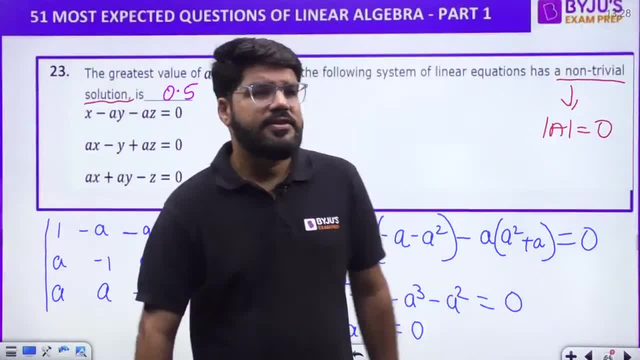 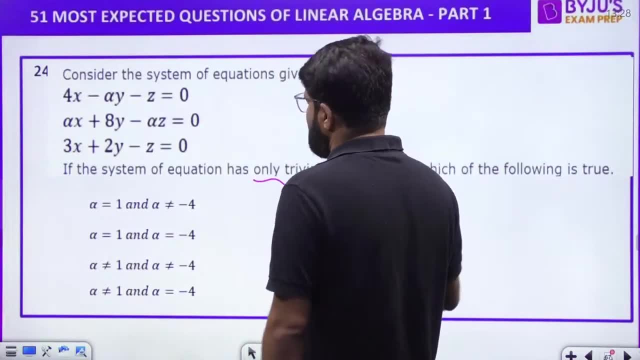 answer is 0.5. ok, non-trivial solution. next question, number 24: ah, guys, again, again. you know this is this is very simple trivial solution. so one more homework. all similar questions you can try as homework, Because only calculation part is what we are going to do. 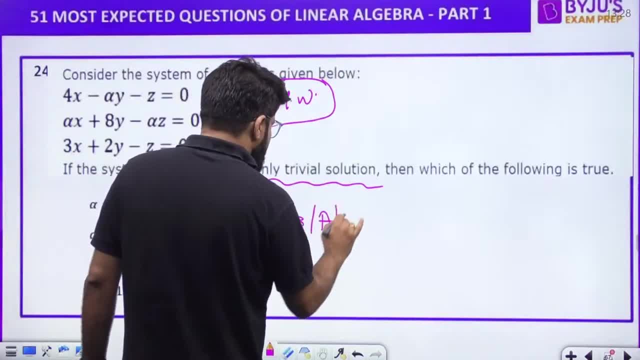 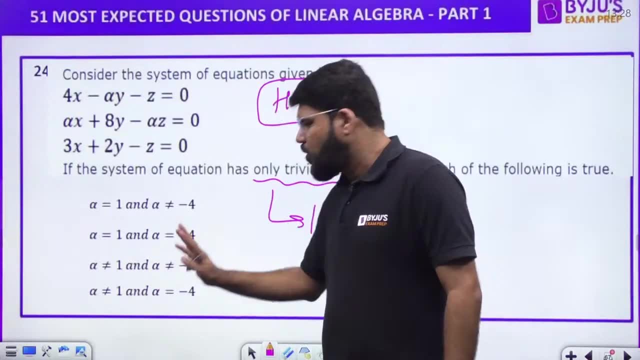 Ok, We are discussing in a in a similar question, trivial solution. so mod a not equal to 0. that is why options are in the form of not equal to options, not equal to formula. see actually both non-zero aayega, both not equal to aayega, right? ok, yeah, we will plan some basic sessions. 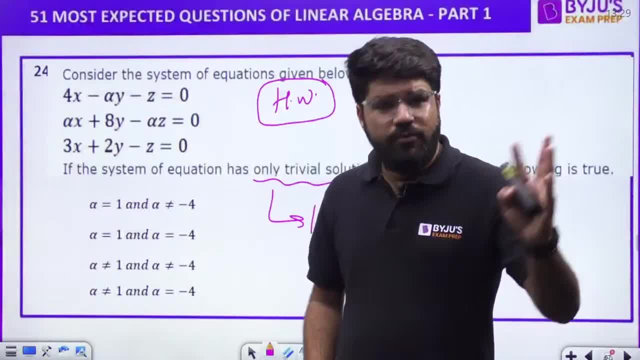 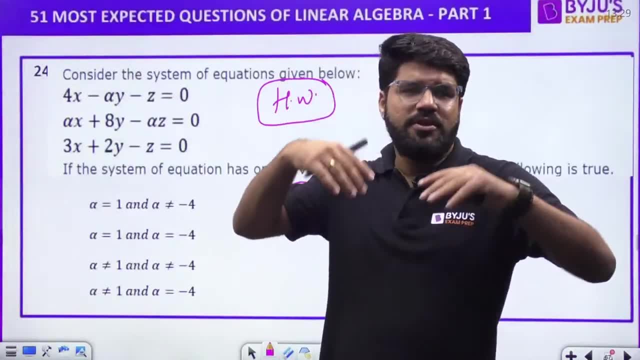 also of linear algebra, but hanumanth, this can also help you. if you follow this session from starting, this can help you. but yeah, this is not from the basic, this is from the questions. reverse methodology: first we take questions and we discuss the properties and the related. 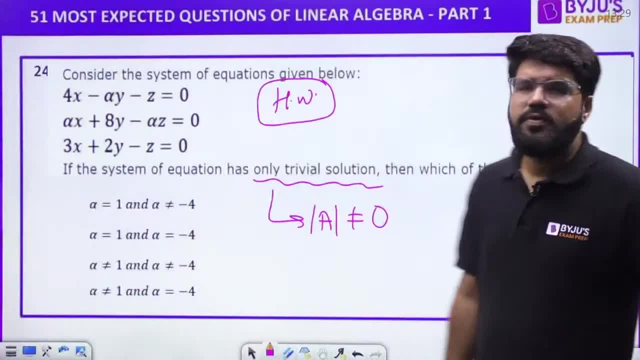 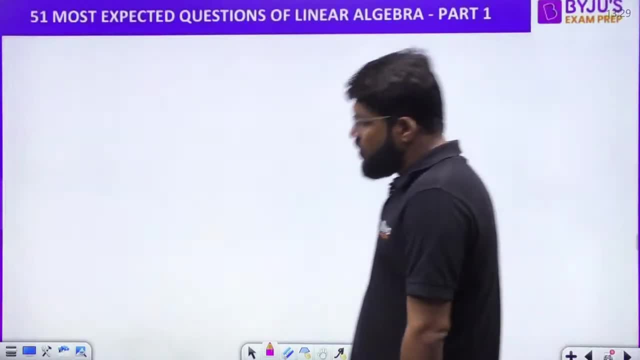 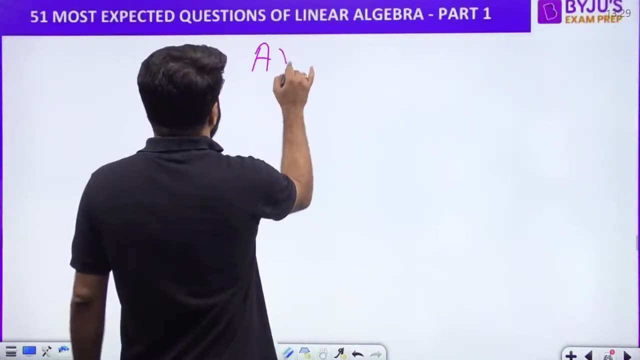 concepts. so this is next homework for you guys. this is the next homework for you. this is the next homework for you, right, ok now look at one thing. normally, let us go back to ax equal to b, right, right, normally we have ax equal to b. let us go back to the non-homogeneous. 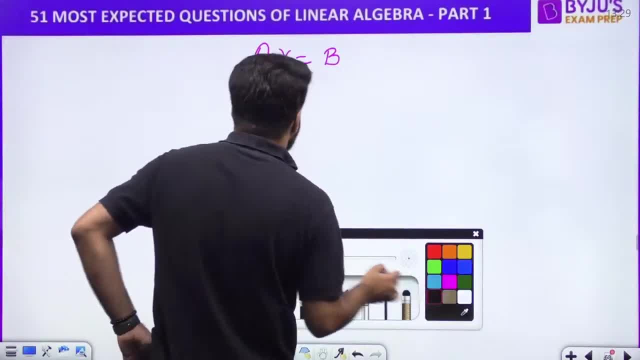 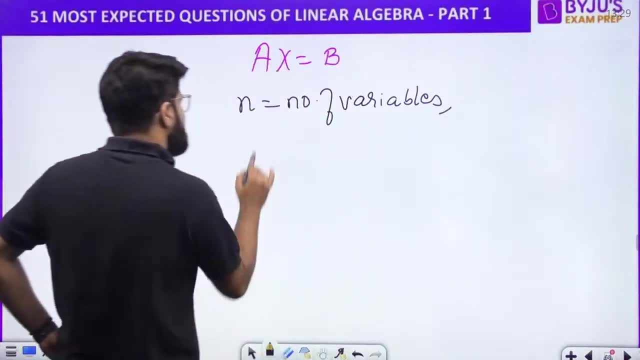 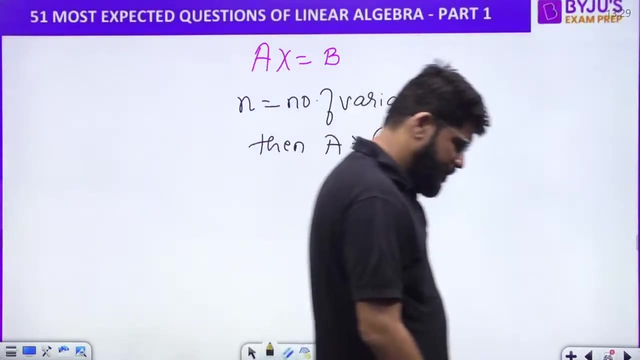 system of equations. only right, non-homogeneous system of equations, right, let us suppose n is the number of variables. Right, Right, Right. Let us suppose n is the number of variables. then, guys, what is the size of a? then a is a square matrix of size n, cross n. then a is the square matrix of size n, cross n. ok, that. 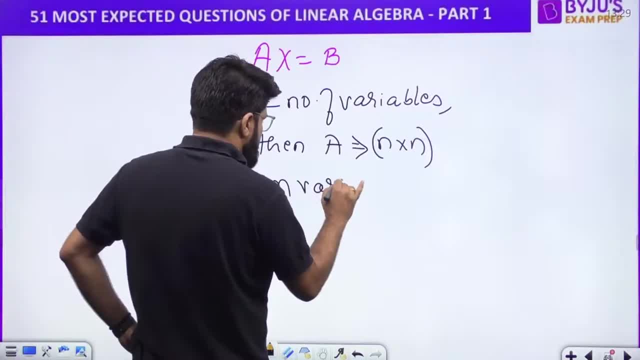 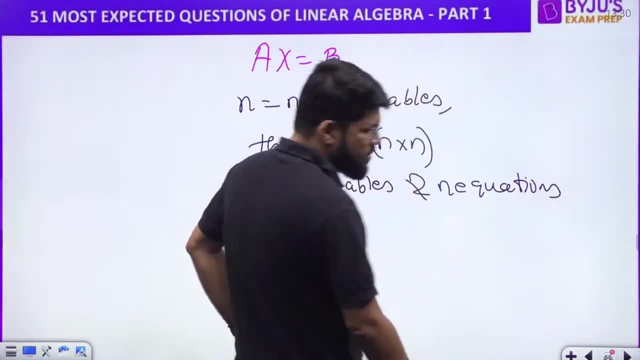 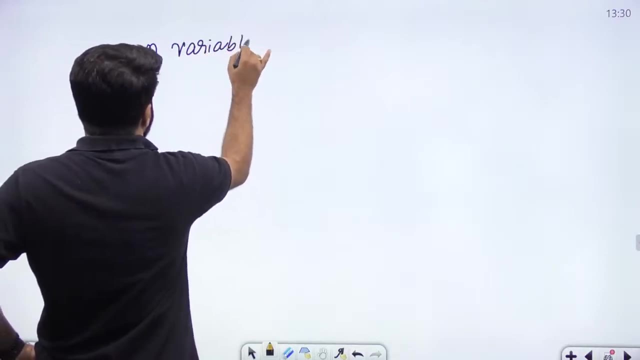 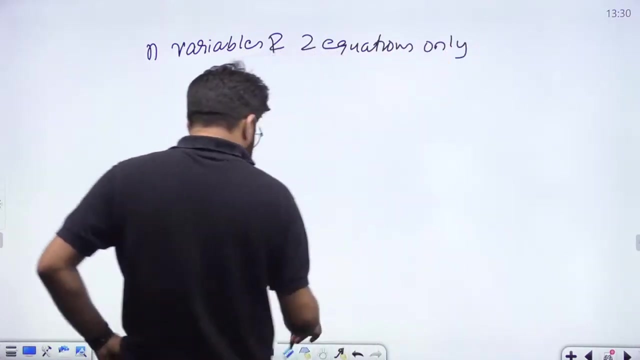 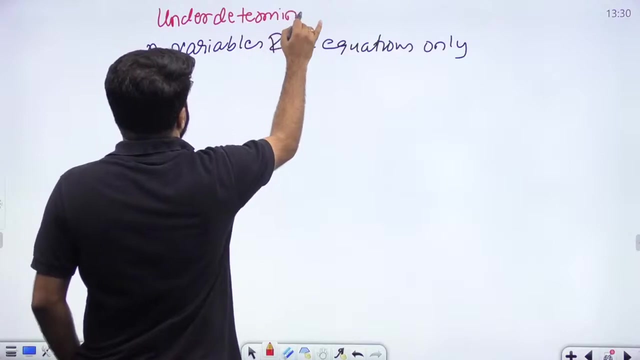 is known as n variable, n equations, that is known as the case of n variables and n equations. but suppose, but suppose, but suppose you have. You have n variables right and two equations. only such a system is said to be, such a system is said to be underdetermined system. underdetermined system, you are given three variables right. 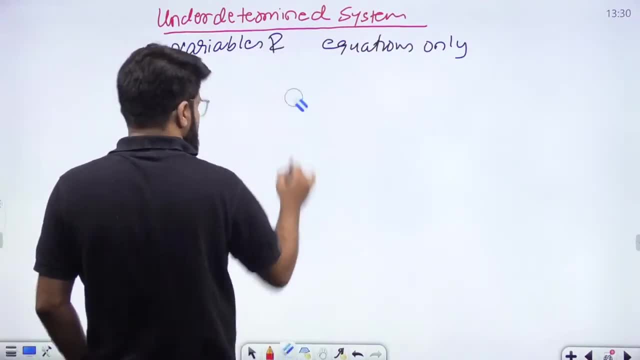 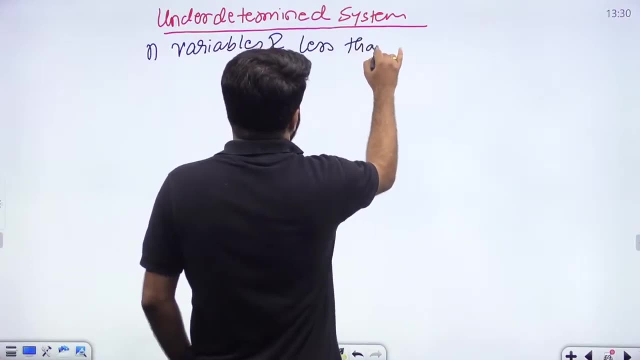 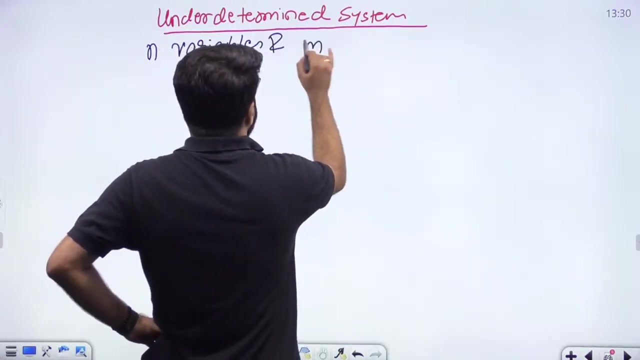 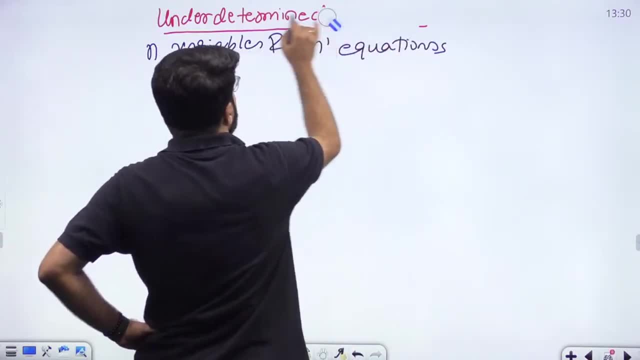 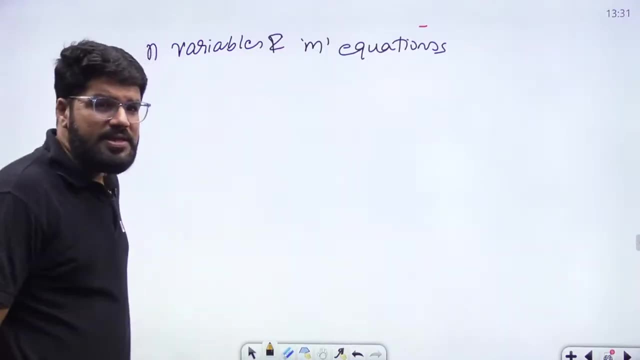 Two equations: and And. Let us generalize just one more. while. Let us generalize one more. whiledem tut two, dizendo te suppose you have n variables, can? I will generalize this in a single shot. you have n variables, You have n variables, and. Okay, but 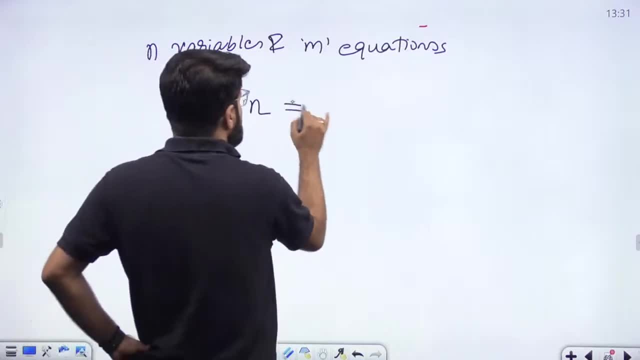 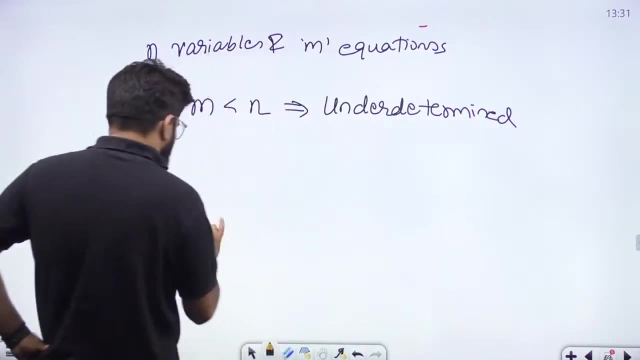 You have n equations and number of equations which are less than the number of variables. 時候이리AKEorta다 underdetermined. Such a system will be underdetermined right. And if m is greater than n, such a system. when more number of equations are given, such a system is said. 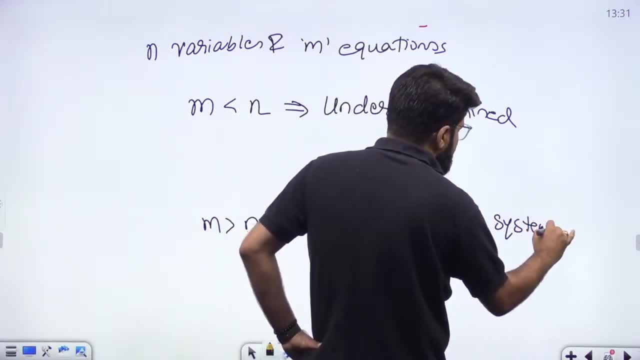 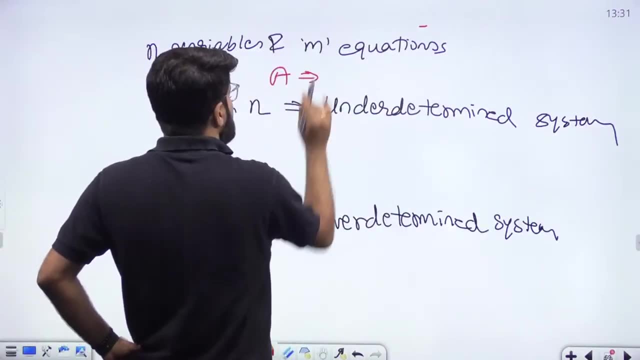 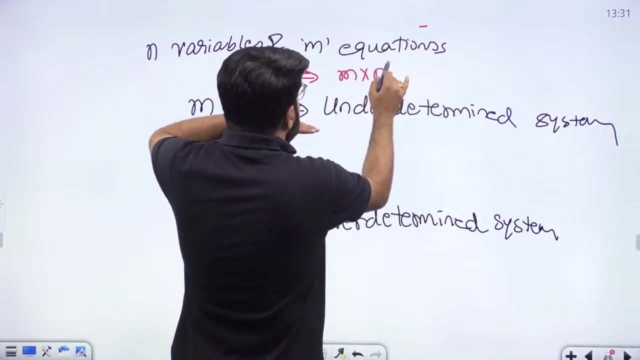 to be overdetermined. system when more number of equations as required. right The size of the matrix. the size of the matrix: see how many rows are there in the matrix depending on the number of equations. right How many columns, depending on the number of. 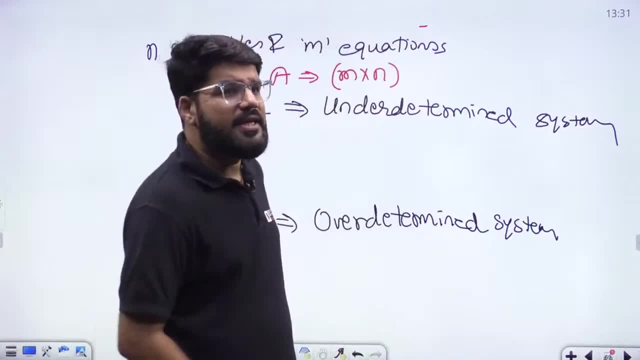 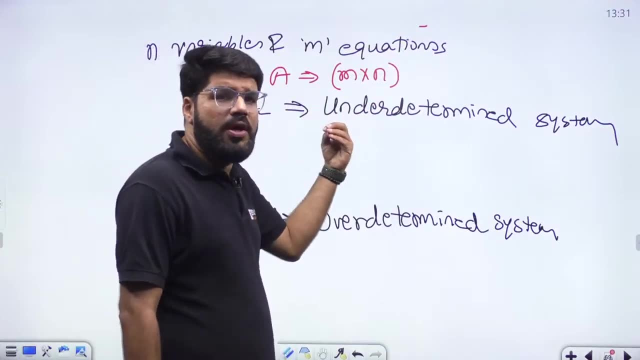 variables. As an example, I will explain you right. As an example, I'll explain you How many rows in the matrix: First equation. second equation, third equation converts to the first row. second row, third row. So how many equations, m equations to m rows, How many variables You. 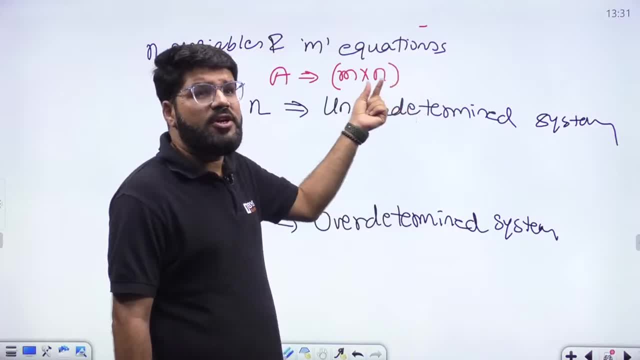 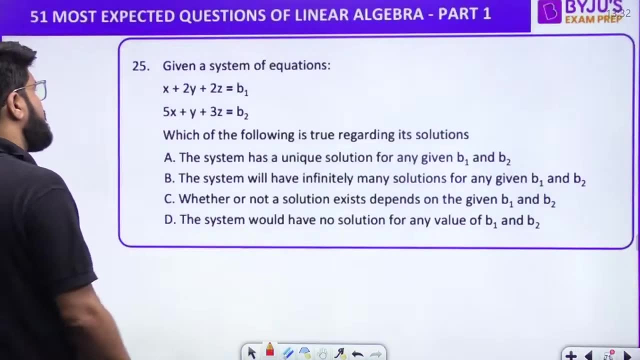 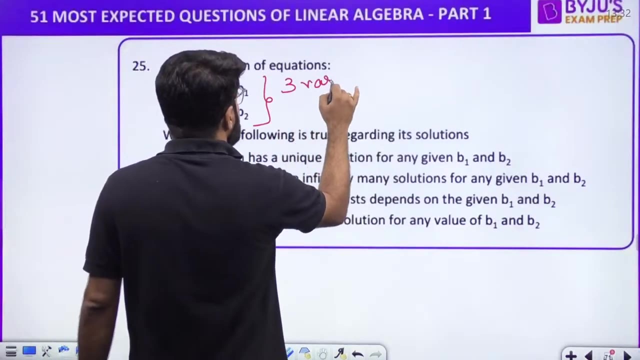 need in every row, you need how many numbers, You need the coefficient of every variable, How many variable. n variable. This is m cross n. Have a look into this example first. This example goes like this: This is x plus 2y plus 2z is b1, 5x plus y plus 3z equal to b2.. So this is three variable case. 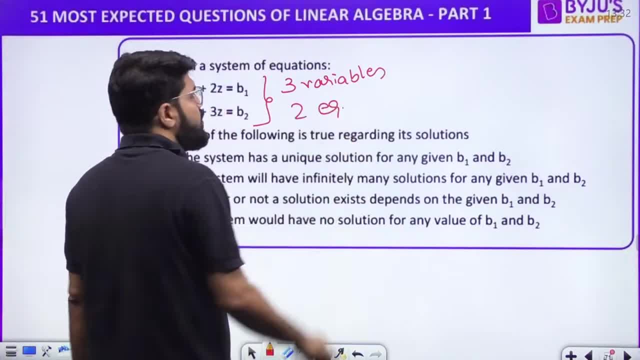 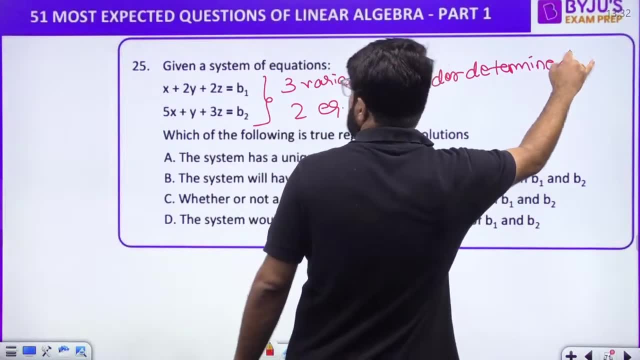 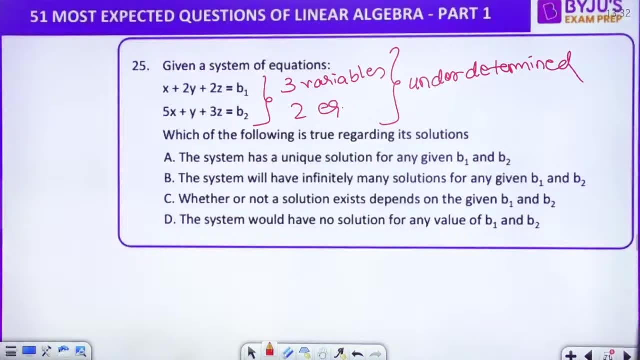 right, But this is only given two equations. This is known as underdetermined. This is known as underdetermined. This is known as what? This is known as underdetermined type of system. This is known as underdetermined type of system. What should be a, a will be m cross n. 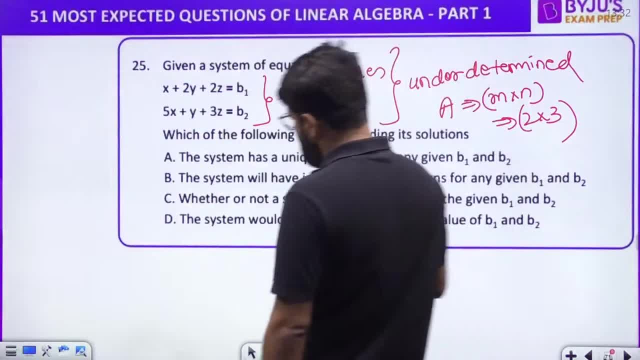 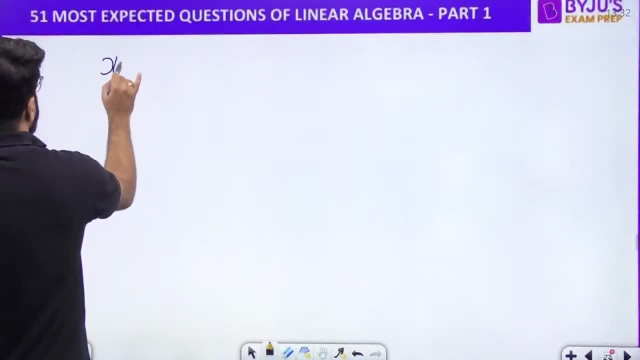 right, That means a will be a 2 cross 3 matrix. That will be. a will be a 2 cross 3 matrix. How a is the 2 cross 3 matrix? Let us understand in this next slide. Okay, so you have x plus 2y plus 3z. 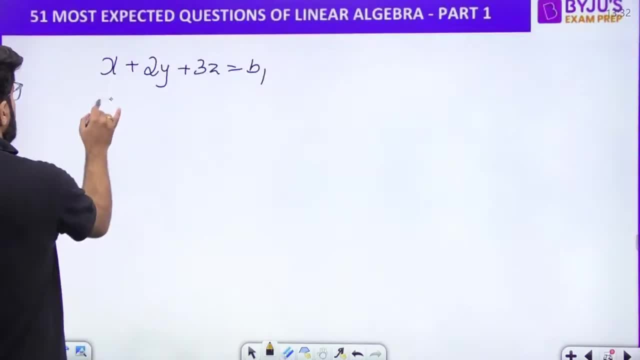 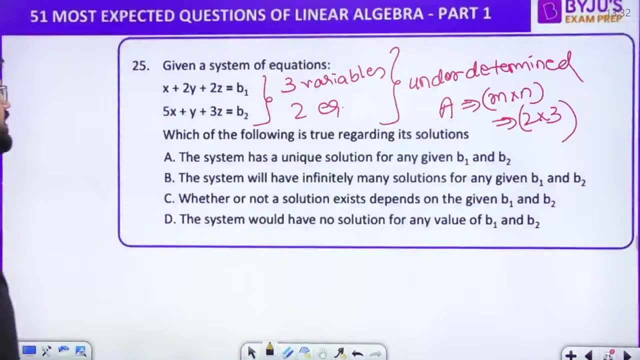 is equal to b1, right. And then you have 5x plus y plus 3z is equal to b2.. This is given, right. How do you write down this system? in the matrix form, You will have 1,, 2,, 3,. 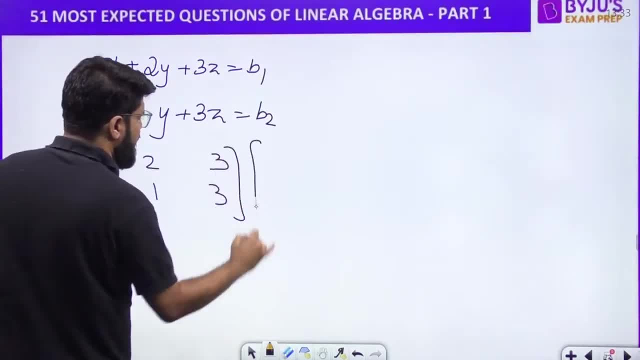 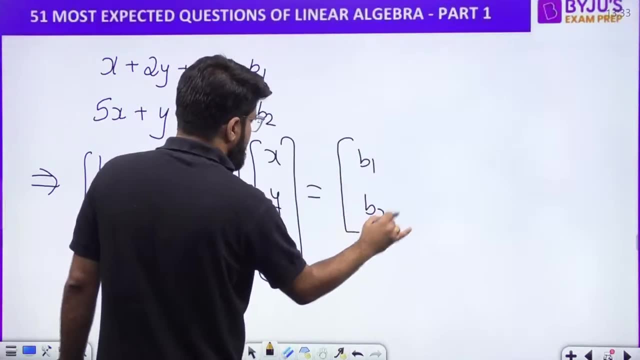 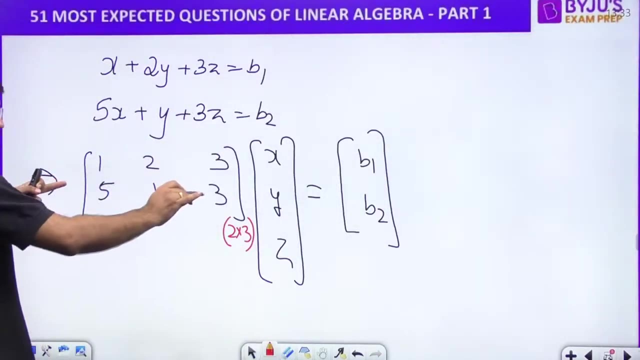 5, 1, 3 multiplied by x, y, z Variables are still: 3 is equal to b1, b2, right. So what is the size of this matrix? This is 2 cross 3.. Automatically, this is 2 cross 3.. Only two rows to fill up, but. 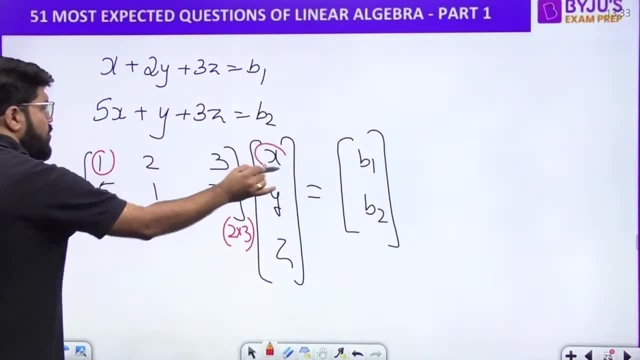 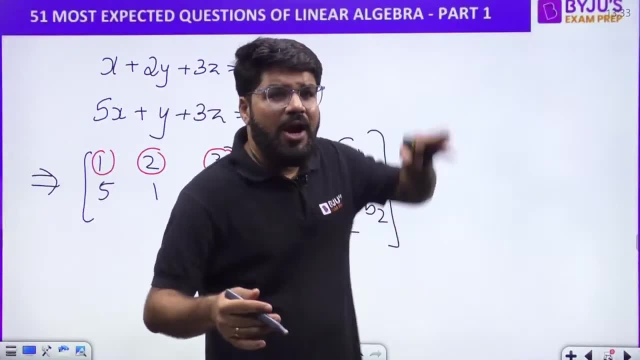 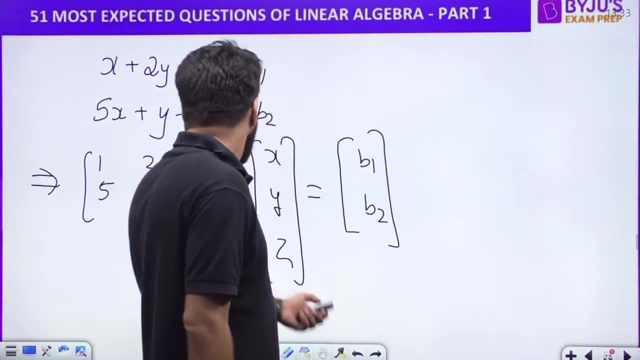 number of entries in each row, number of columns: x coefficient, then y coefficient, then z coefficient. So how many columns, Number of variables, How many rows, Number of equations given. So that is m cross n. That is why, in general, I have written this as: 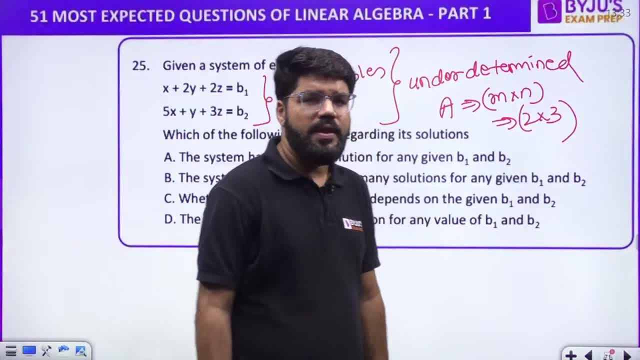 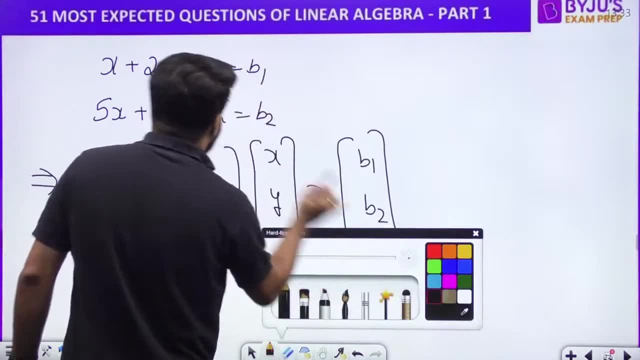 m cross n, And this is an underdetermined system. It is 2z. It is 2z. Oh, sorry, I will just make the correction. That was a reading error. I will write this as 2z Here also 2.. But even if it is, 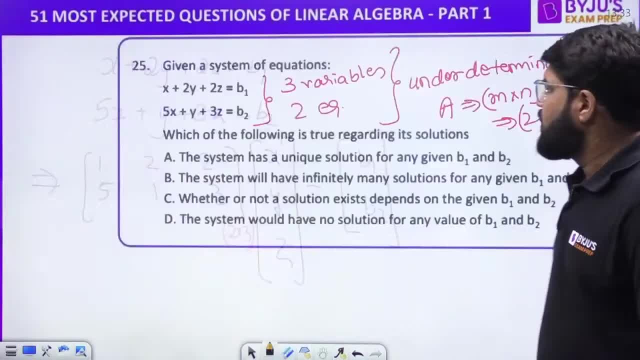 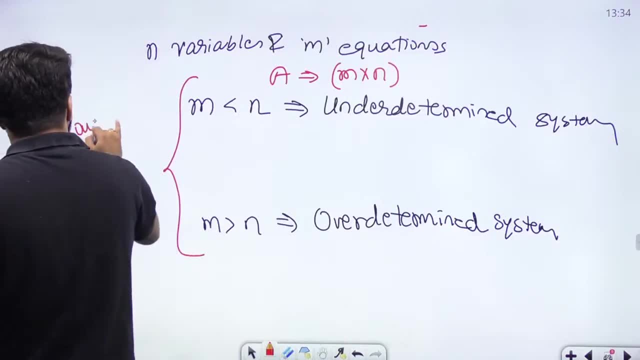 underdetermined or overdetermined. the method remains the same, Guys, even if it is underdetermined or overdetermined for both. right, For both Rauch's theorem, That flowchart you have discussed, right, That flowchart, that I told you, that Rauch's theorem. 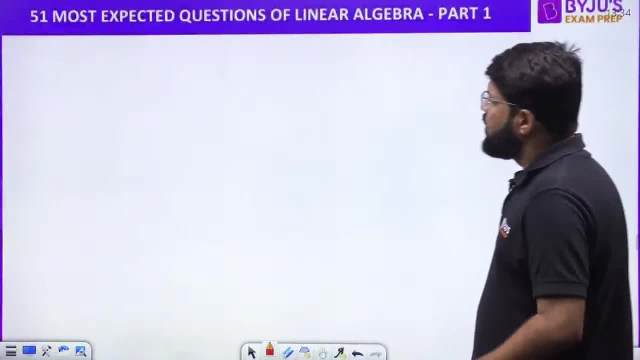 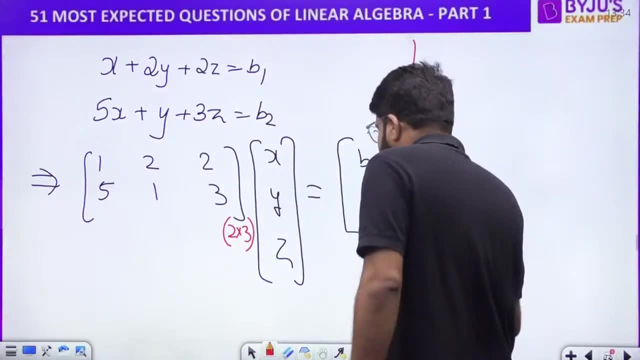 it is still applicable as it is. There is not going to be any change in the method. There is not going to be any change in the method. So what is that Rauch's theorem? What is that Rauch's theorem? Let's pick it right. What is the a? and what is the a is to b. 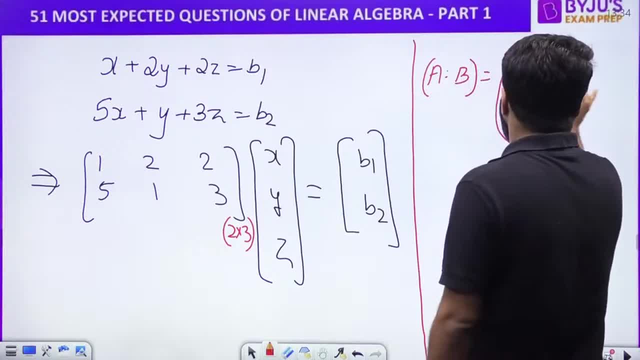 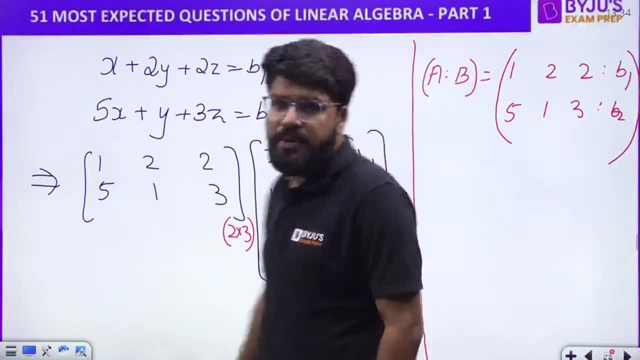 What is the a is to b matrix, Combined matrix. So 1, 2, 2 is to b1.. 5, 1, 3 is to the b2.. 5, 1, 3 is to the b2.. Okay, Now pick up any one minor. 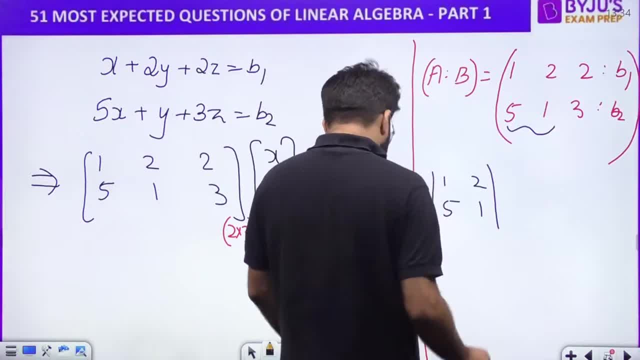 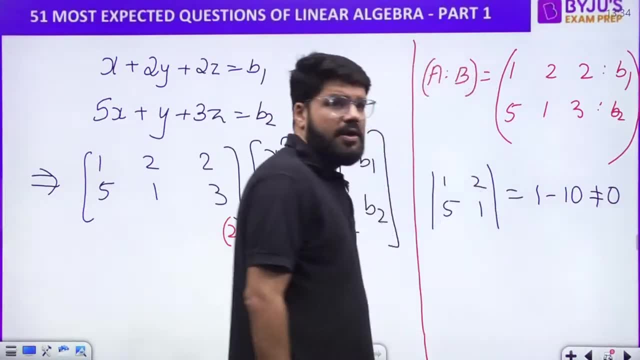 1, 2, 5, 1.. Pick up any one minor from here. right. Calculate the value 1 minus 10.. This is not equal to 0. That means that means you have a 2 cross, 2 minor non-zero. 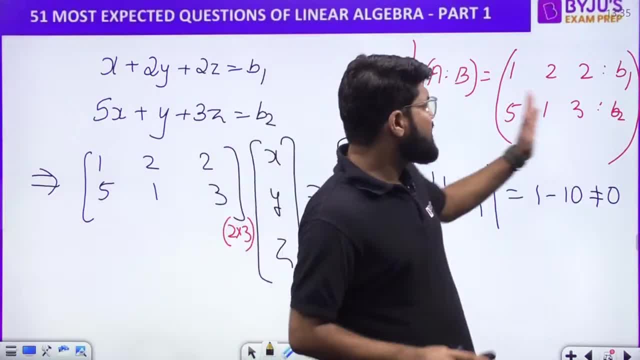 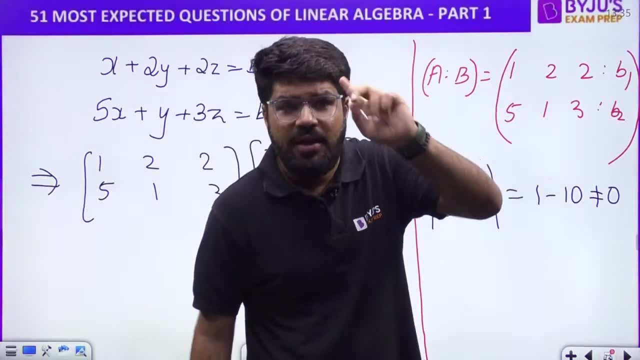 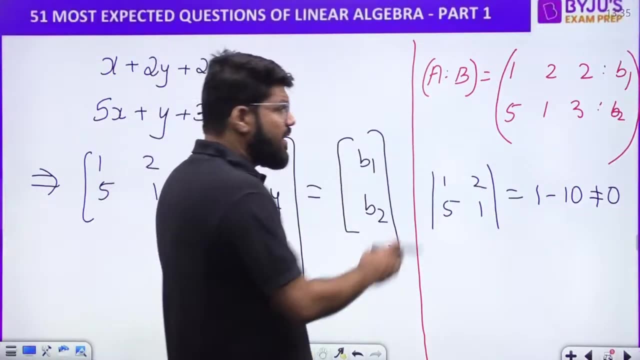 You have a 2 cross, 2 minor, non-zero. What is the total size? of A is to be 2 cross 4.. What should be the maximum possible rank? 2. What is the maximum rank? Minimum of Mn, Remember. minimum of Mn right, Minimum of Mn right. So there. 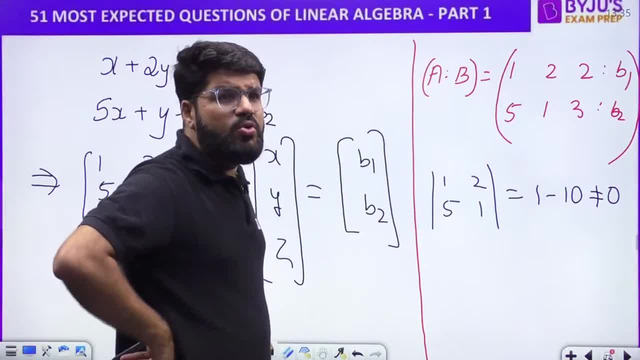 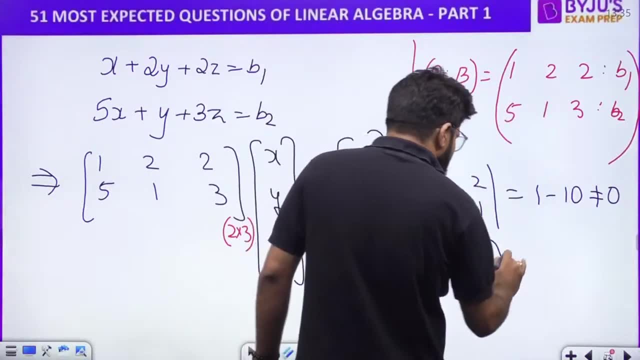 is a 2 cross 2 matrix not equal to 0.. There is a 2 cross 2, there is a 2 cross 2 minor not equal to 0. So rank will be 2.. Now, this is a minor of A. This is a minor of A is to: 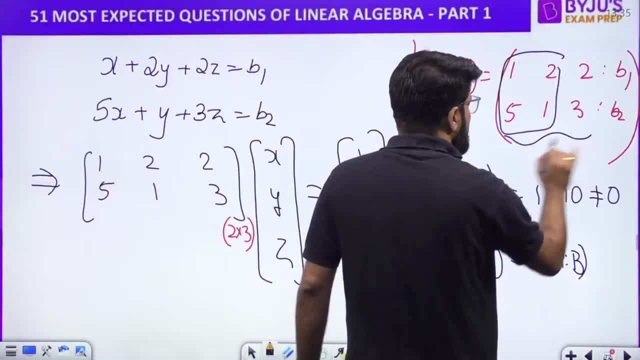 be also The same minor. it is a part of A also. it is a part of A is to be also. So if I have found one non-zero minor which is common to both A and A and B, so I can say: 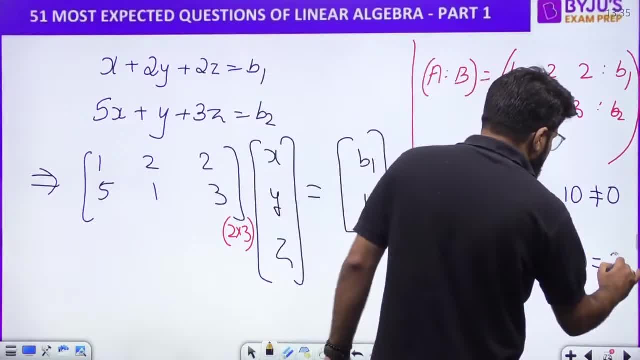 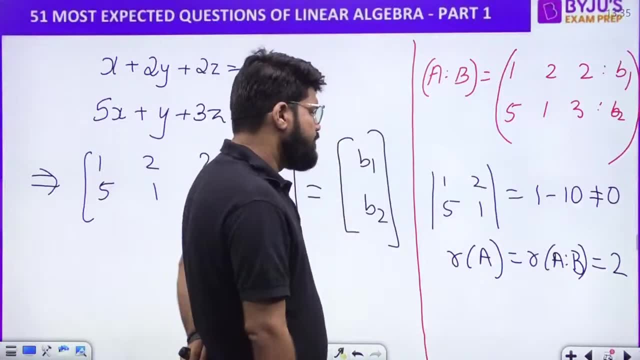 that I can say that rank of A and rank of A is to be both- is equal, equal to 2.. No need to convert to echelon form. Directly, I am able to feel. If you want, you can convert to echelon form, but directly I am able to feel. So both the ranks are equal and equal. 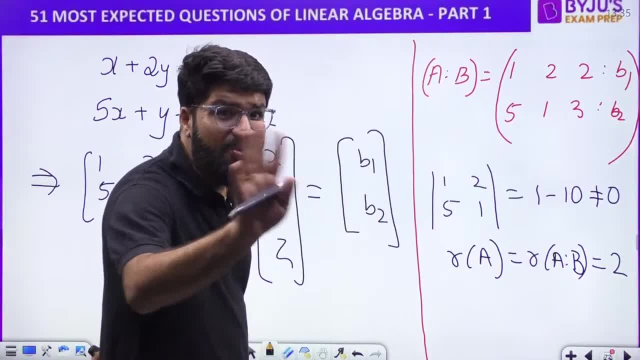 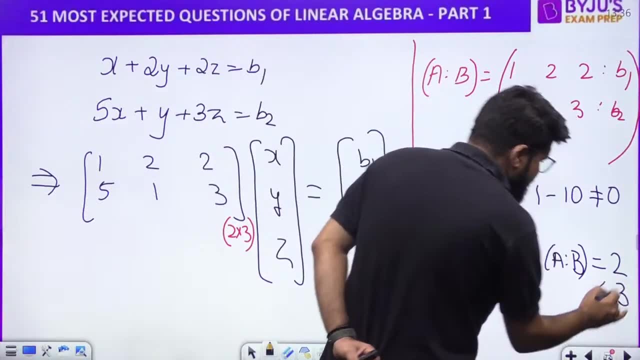 to number of variables. Is it equal to number of variables? No, Both the ranks are equal to 2.. Less than the number of variables, This is less than 3.. Both the ranks are equal, but less than 3.. So how many solutions you? 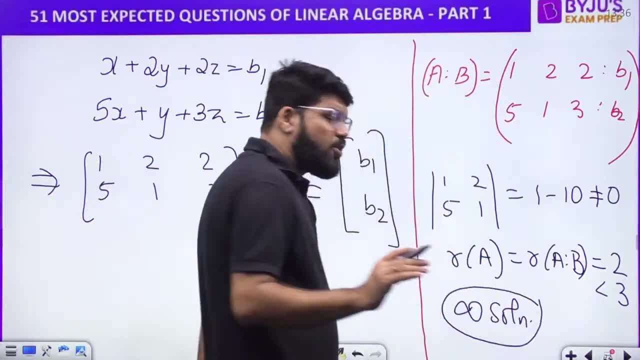 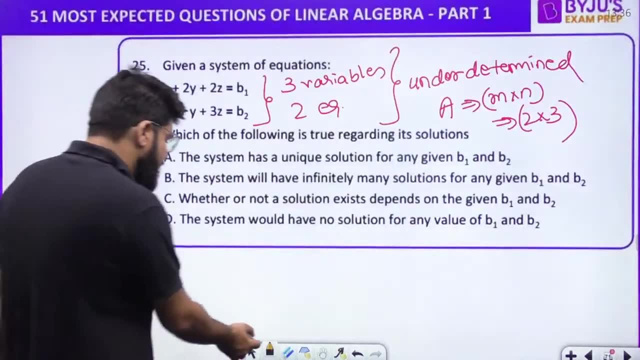 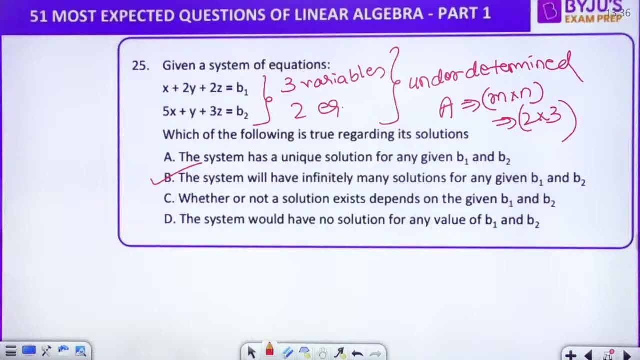 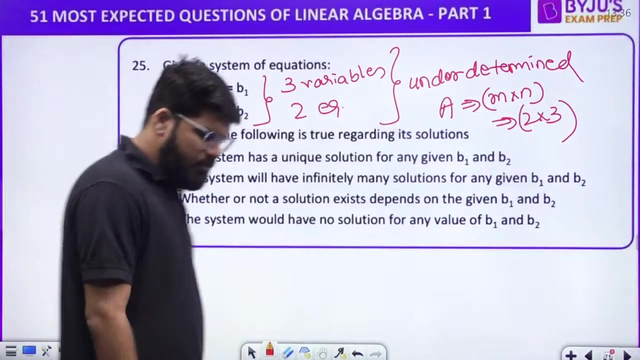 will have Both. the ranks are equal less than number of variables. So infinite solutions, Infinite solutions. The system will have infinitely many solutions. The system will have infinitely many solutions. Unique solution is not possible. That means it can be either infinite or no solution. 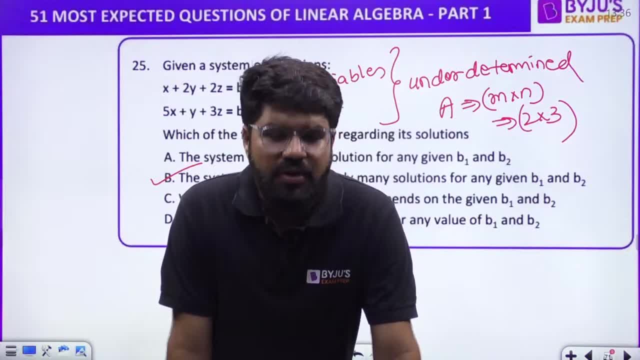 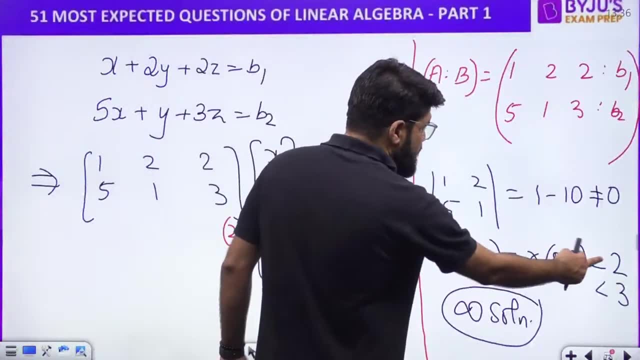 For under-determined, you cannot find the unique solution. For under-determined. it clearly means you cannot find the unique solution. You cannot find unique solution because rank of A- rank of A is to be- is always equal to minimum of MN and M is less than N. Under-determined. 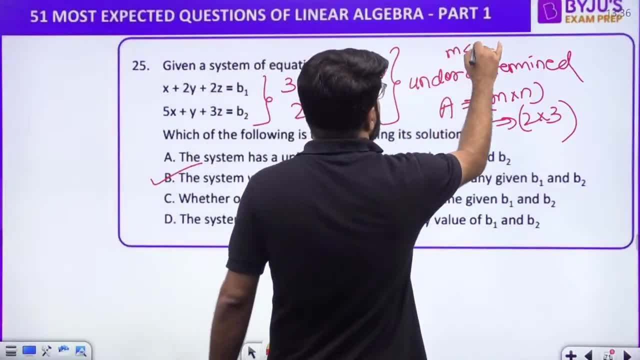 means M less than N. Under-determined M less than N. So what is the minimum of MN? It is M. So rank of A. rank of A is to be equal to 2.. So rank of A is to be equal to 2. So. 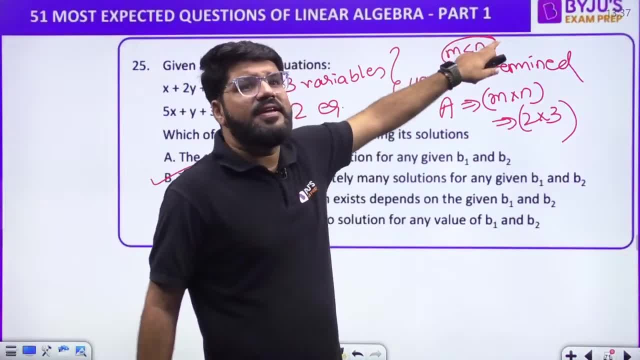 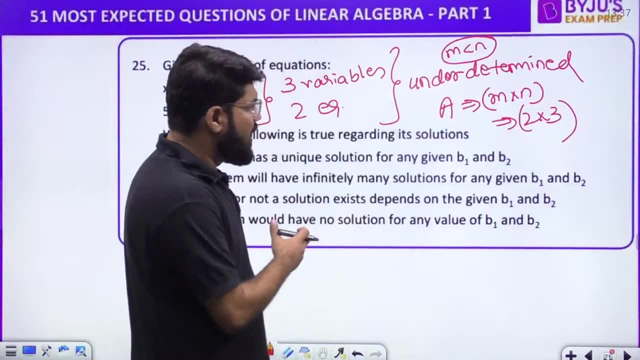 rank of A is to be even. if it is equal, it can be maximum M. It can never touch N. And if it can never touch N, it cannot have unique solution, No, possible. That, depending on the, that depends on the jumbling of the numbers, That still may be possible, but unique solution. 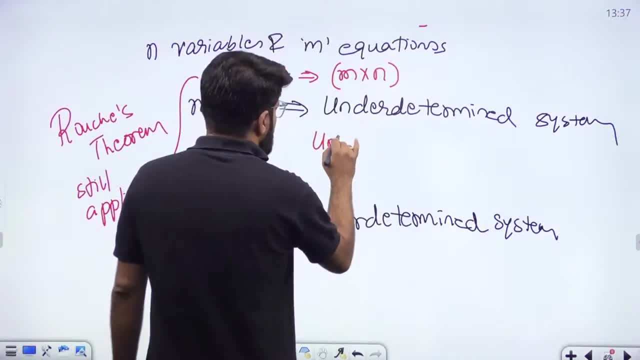 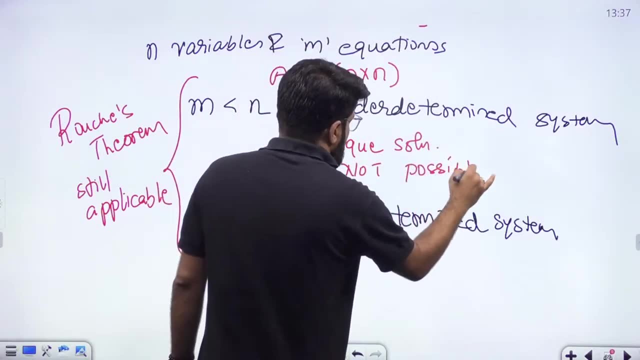 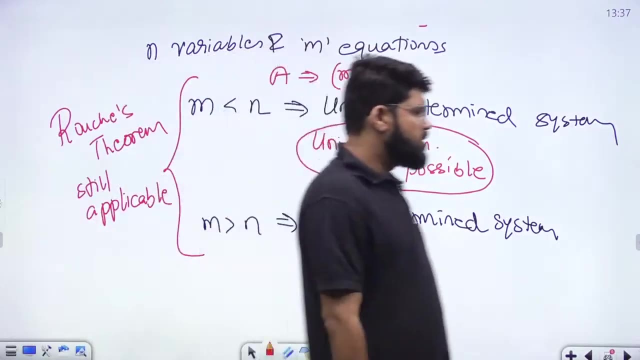 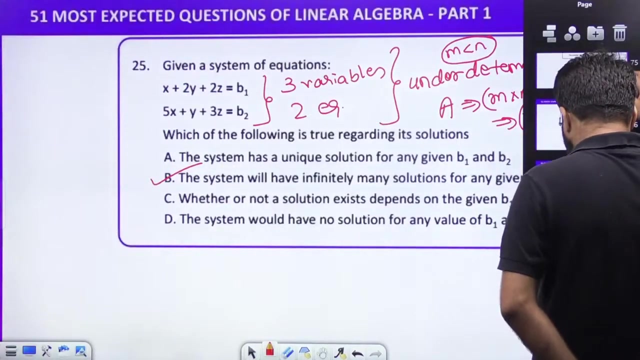 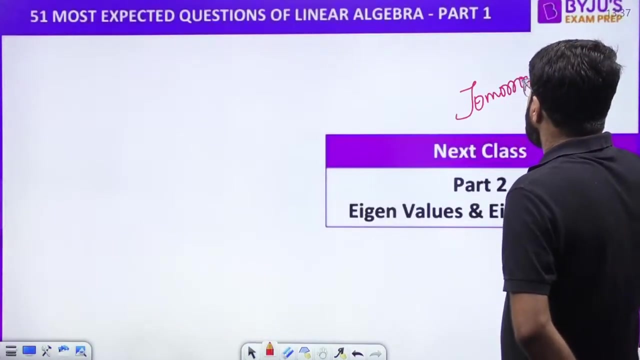 never possible. So for under-determined unique solution, not possible. For under-determined unique solution, not possible. For under-determined unique solution, not possible. So this was the question number 25 for the day And guys, now tomorrow at the same time. 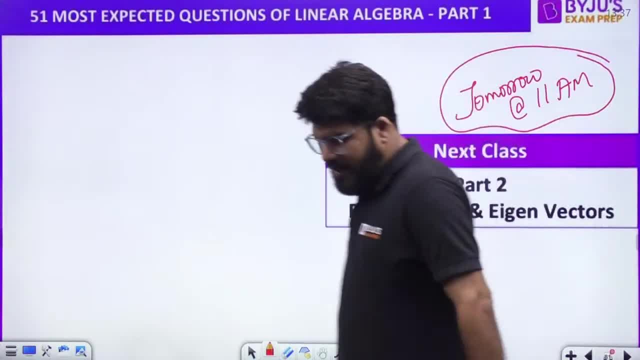 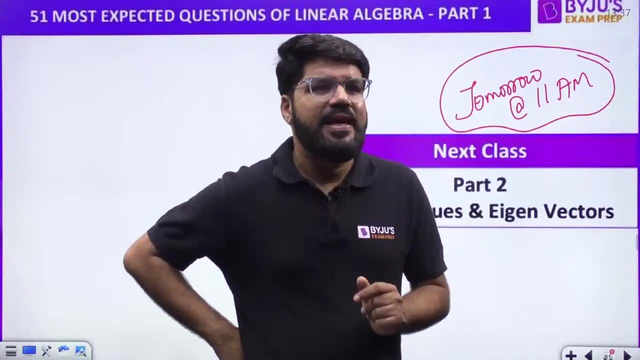 of 11 am. all, dear students, tomorrow, at the same time of 11 am, tomorrow, very same time of 11 am, we are all going to connect once again And discuss the Question number 2.. Question number 2.. 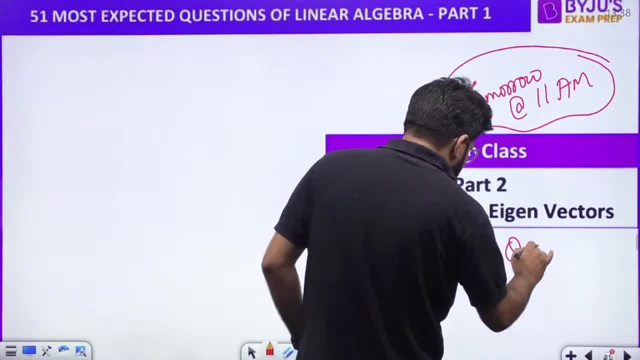 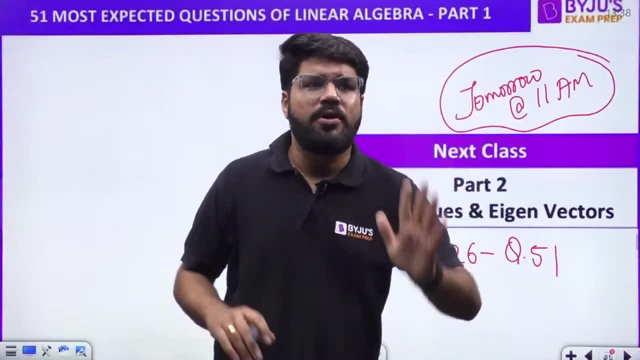 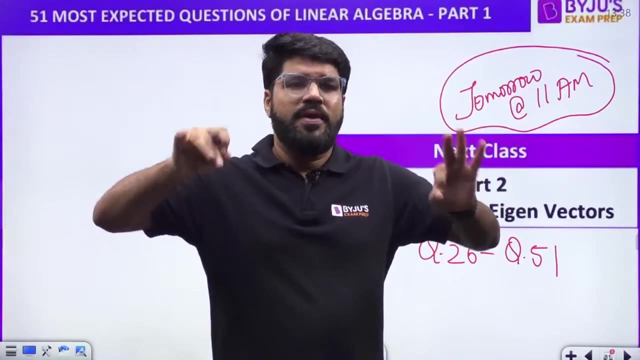 Right, That means That means question number 26 to question number 51. All 51 questions. I will have promised 51, I will give 51 questions, But the very and the most important topic you can say of linear algebra, eigenvalues and eigenvectors, just like today, It is not only questions. 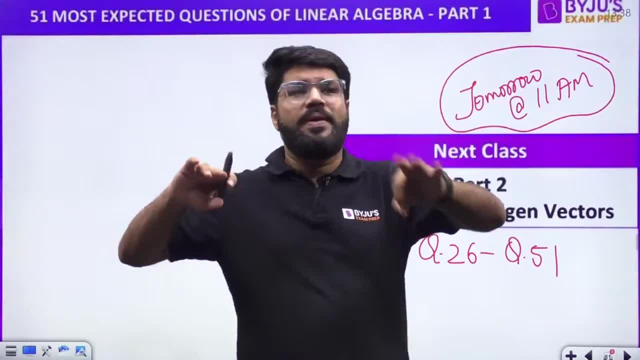 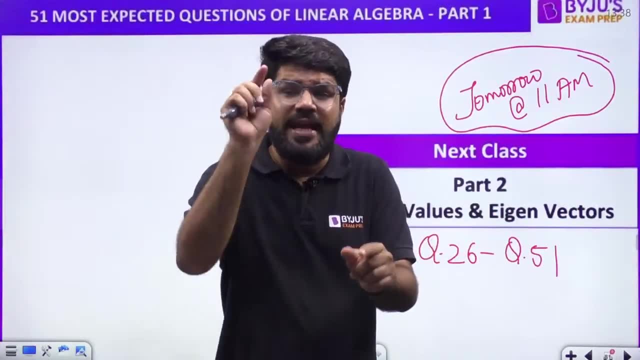 It is not only questions, But if you have attended the today's complete session, you might have felt that we are discussing the concepts, the properties, no detailed theory, no derivation. But we are discussing the techniques, the formulas, the revision, important points and the concepts, along with 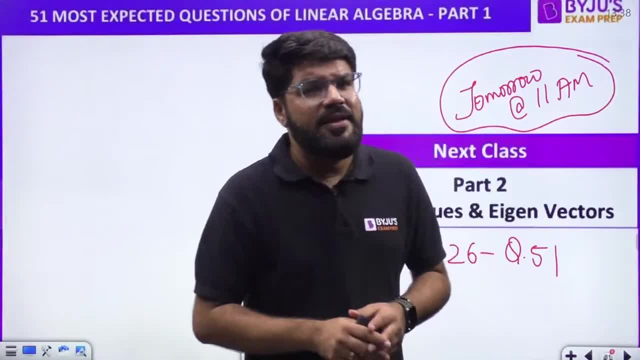 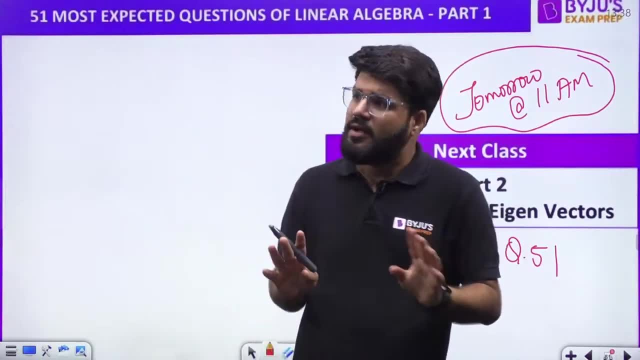 the question. So it is going to be similar tomorrow. Please do mention in the comment box, right? Yeah, Kylie Hamilton will also come up tomorrow with eigenvalues. only right, PDF password is given in the middle of the session, right? So, guys, PDF password is there in the middle of the. 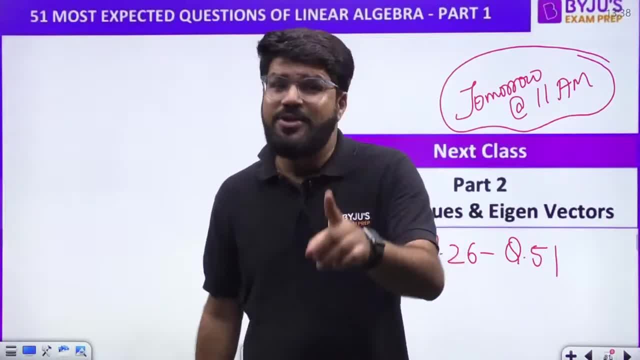 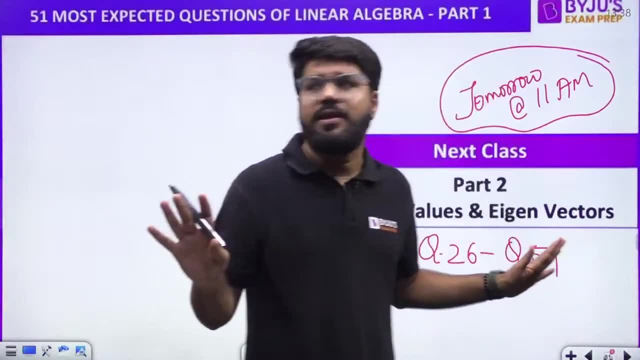 session. So, guys, please do mention in the comment box how much you enjoyed the session. right? If you feel that you have enjoyed, I will plan some more on the weekends. I'll plan some more sessions on the upcoming weekends, Don't worry regarding to it. okay, So tomorrow, 26 to 51 question. 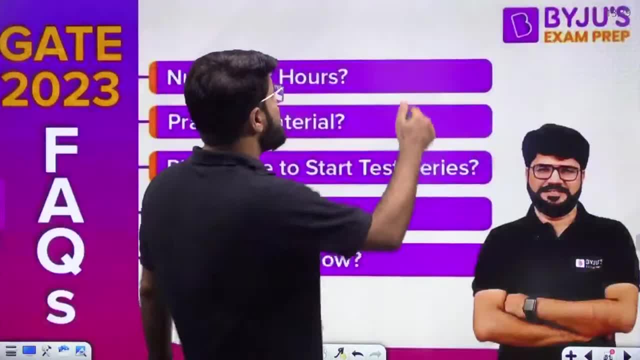 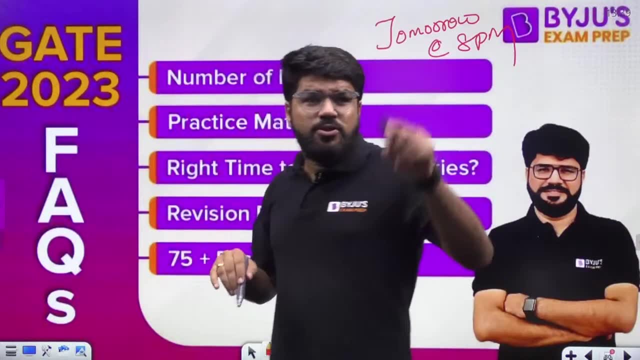 eigenvalue eigenvector. tomorrow at 11 am. and tomorrow you have one more session right For all the GATE 23 aspirants, tomorrow 8 pm. Also join me tonight. same Byju's exam prep YouTube English. 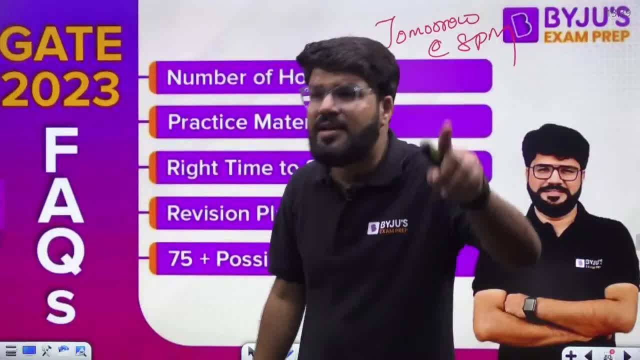 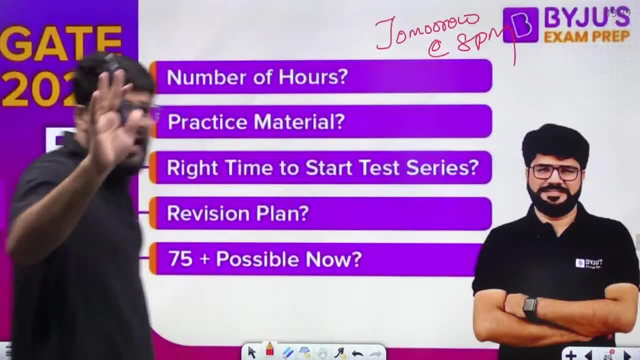 channel. Do not forget to subscribe. In case you are not subscribed to the channel, do subscribe so that you get notified. you are updated about all activities of the session. So tomorrow: GATE 23,. last three months. last 100 days left. 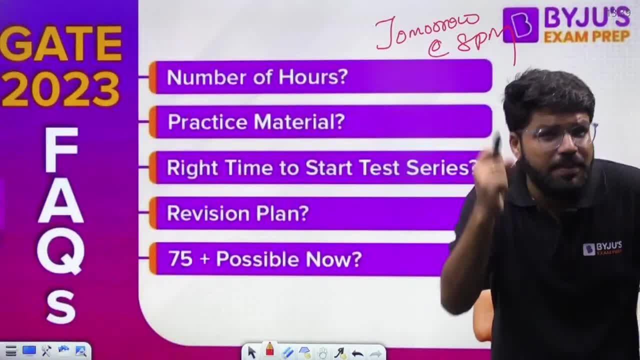 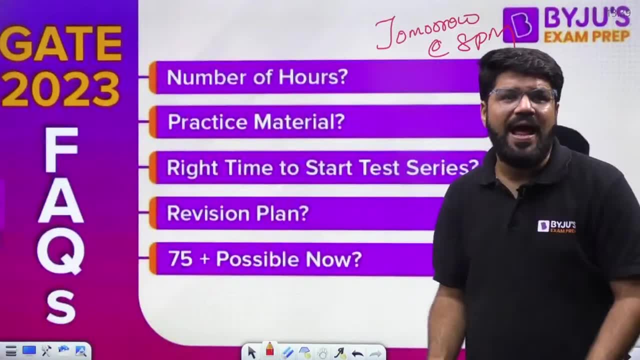 What are the frequent doubts in any aspirant's mind right? How many number of hours now From where to practice? What is the right time to begin test series? Where is the revision plan right? And is 75 plus still possible? Let's get an answer to all of these tomorrow, 8 pm, Same. 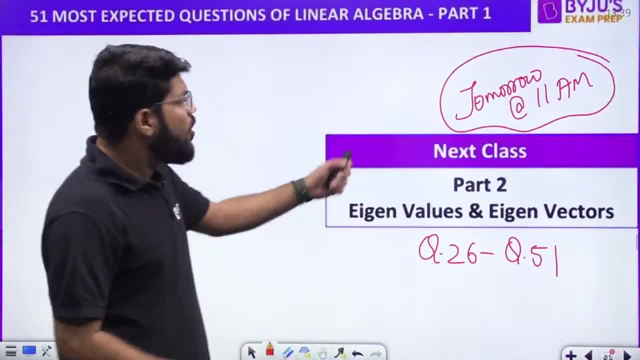 channel. Keep subscribed to the channel. Hit the subscribe button if you have not subscribed, okay, And let's connect. tomorrow 11 am. Yes, tomorrow 11, 1, 1, 11.. Bye-bye, See you tomorrow. 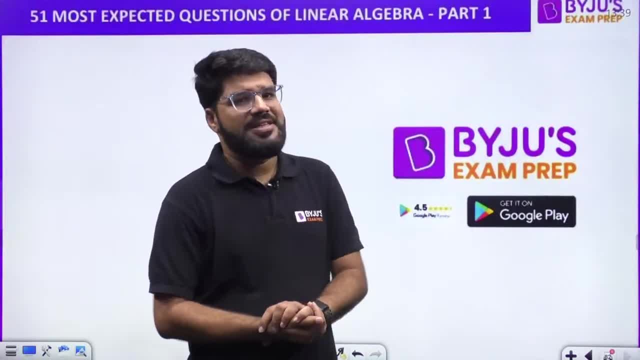 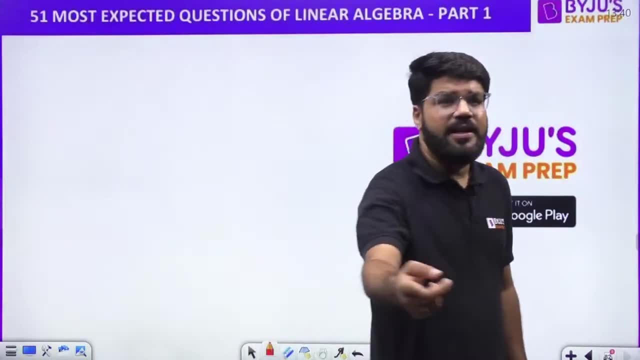 and do not forget to download the Byju's exam prep app also. Bye-bye, See you tomorrow. PDF will be shared in the Telegram group. PDF will be shared in the Telegram. I'll share you the Telegram right now. I'll just share you the Telegram right now.